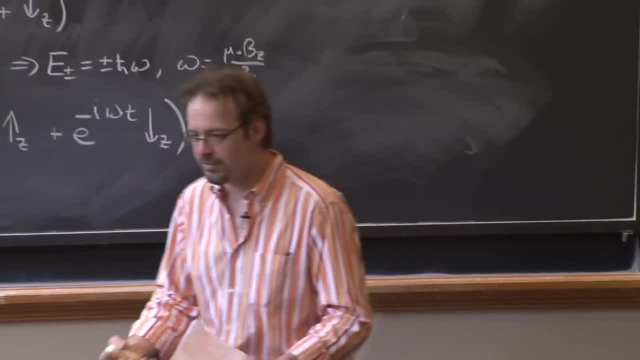 So to finish up. so today I want to finish up a couple of loose ends in the class. The first is I want to pick up- by the end of the day we'll talk about EPR that we've picked up in the last couple of lectures. 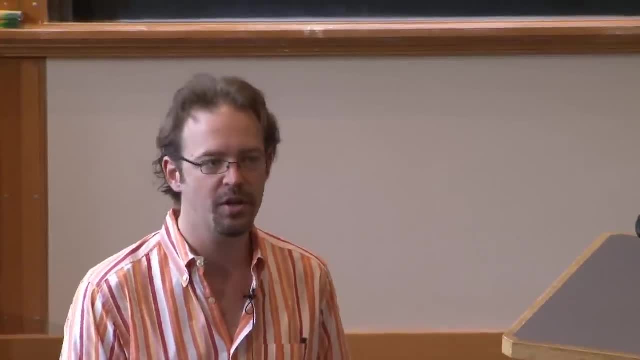 We're going to close up Bell's theorem from the very beginning. So we talked about Bell's inequality and we'll re-prove Bell's inequality and then we'll see what quantum mechanics has to say about it. But first I want to show you something neat. 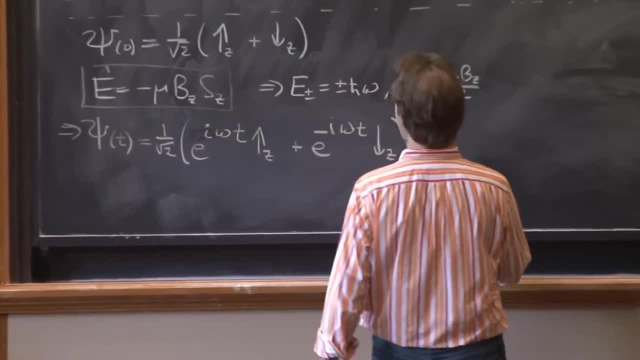 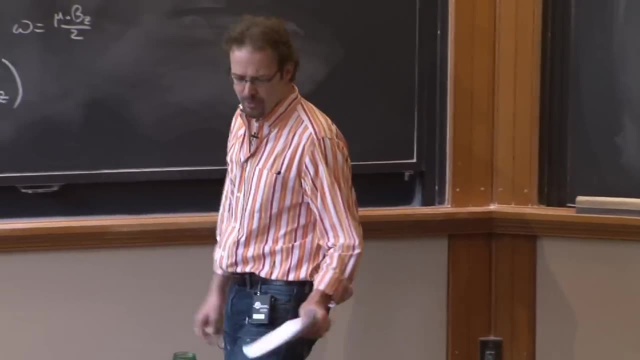 So a couple of times we've talked about entanglement and what it can do, And I want to spend the first good chunk of the class talking about what entanglement can do and also what it can't. So before we get started, I want to remind you. 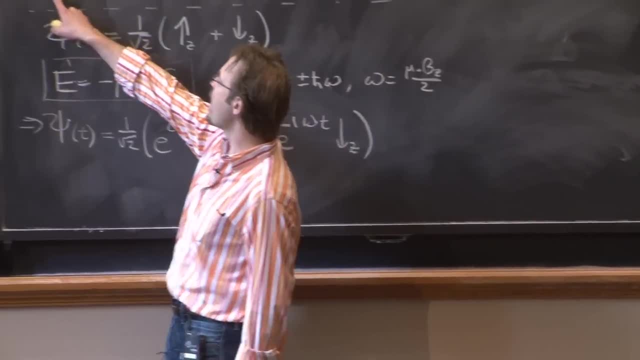 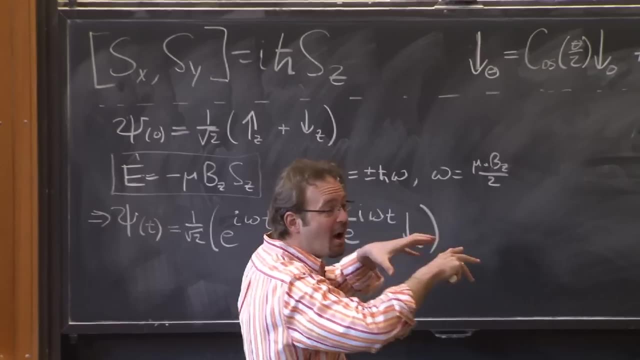 of a couple things from the last lecture. So the first is: We have- so particles can have spin- half integer intrinsic angular momentum. that has nothing to do with being a rigid object that rotates, but it's just an intrinsic property of angular momentum. 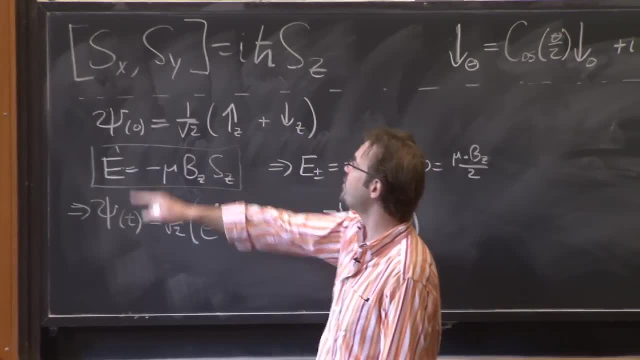 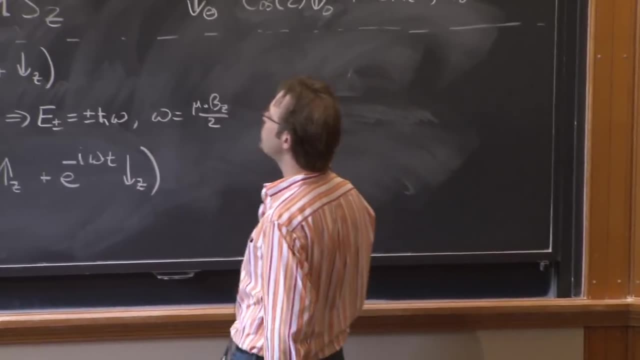 And the spin is represented, it's observable, it's represented by an operator. In fact, a vector of operator says x, x, y and a, c that satisfy the same commutation relations as the orbital angular momentum. Now, last time, one thing we showed: 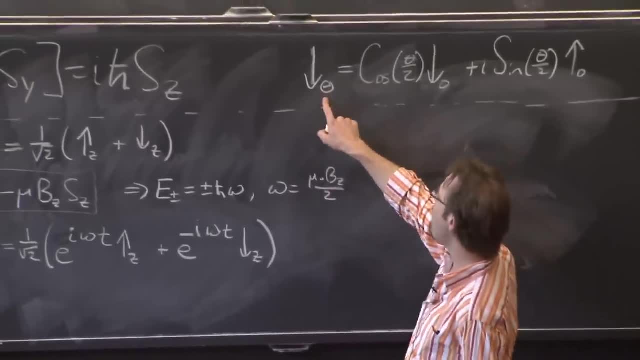 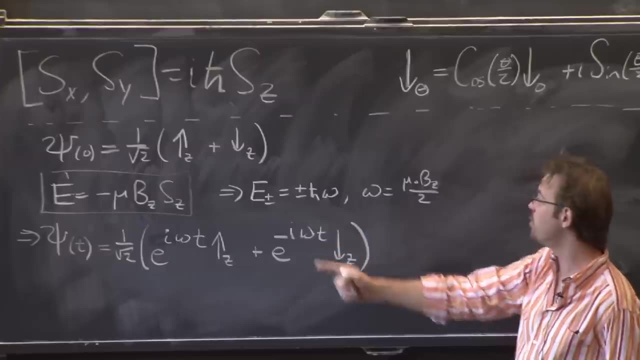 is that a state which is up or, for example, down at an angle theta. So if I measure the spin along this axis I will always find It's either up or down. Spin 1 half, either plus h bar upon 2 or minus h bar upon 2.. 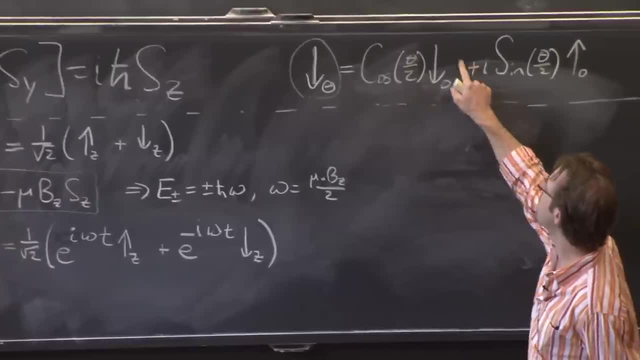 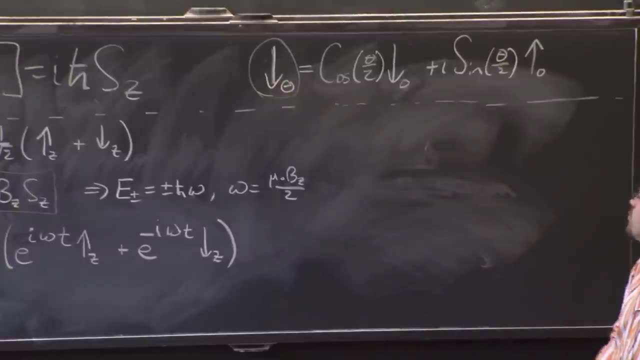 But I can express this state in terms of the states with spin which are up or down along the z axis, And we found, or we gave, an expression, and I challenge you to follow the logic given to derive this expression, an expression for the state which 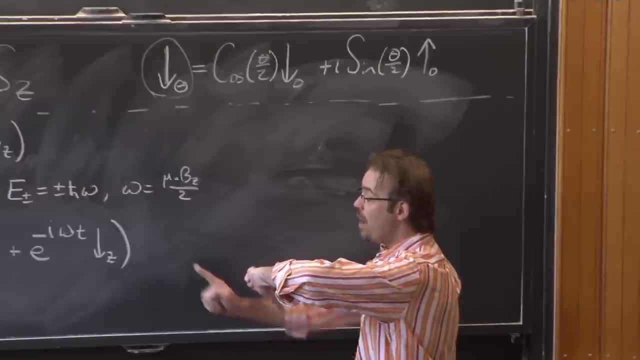 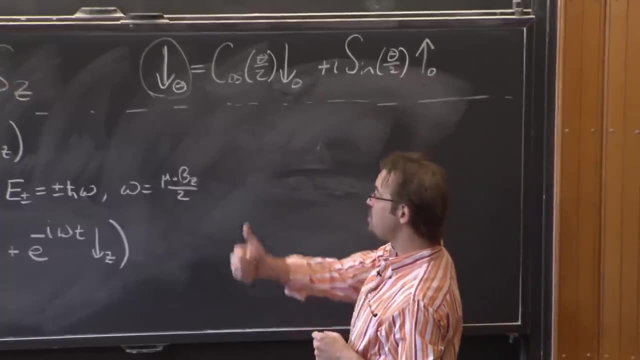 is, in this case, down along the angle theta down when measuring spin along the angle theta in terms of up and down, along, Of spin along the z axis or along the angle 0, theta here being the declination from the vertical. 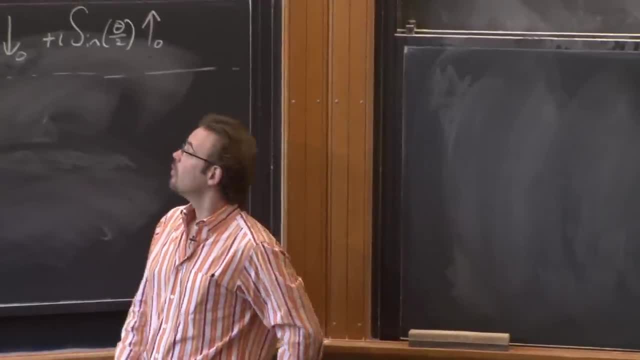 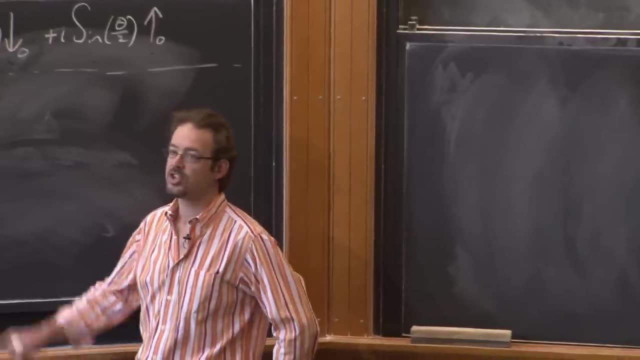 OK, Yeah, So that is for angle theta in the z x right. Yes, Isn't there a relatively simple formula for the angle? Yes, Yeah, there's a general thing for this that says for a general angle, and it's actually. 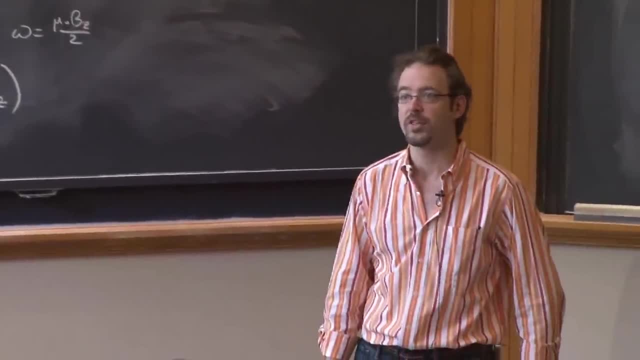 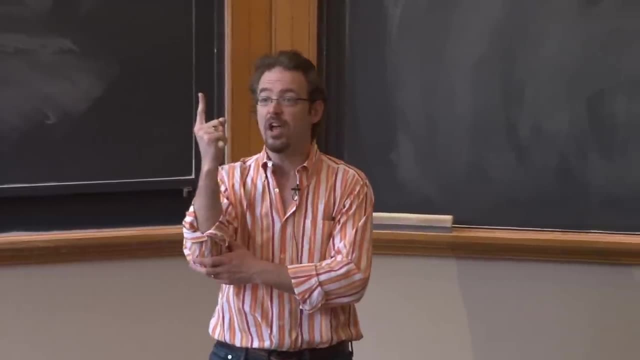 in the notes, which I guess weren't posted from last time, But it's in the notes And it's also easy to derive, right? You know what the so what's the point here? The point is You have a spin vector. 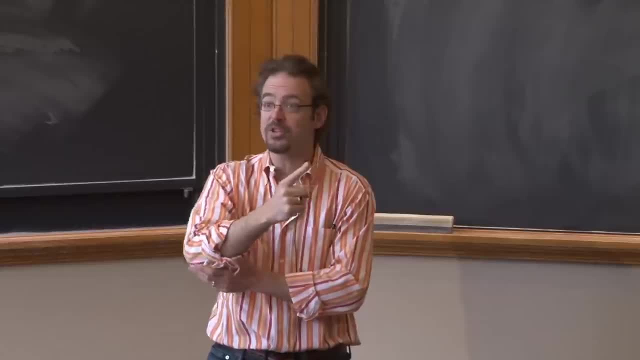 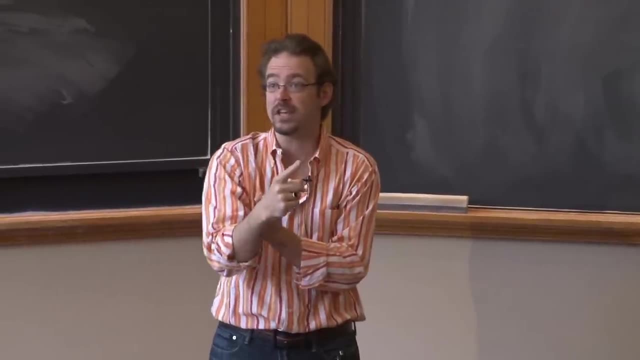 And it's a vector- s, x, s, y, z- And you can compute the operator representing spin along a particular direction by taking the unit vector in that direction and taking the dot product. So that gives you a particular linear combination of s, x, s, y and a, z. 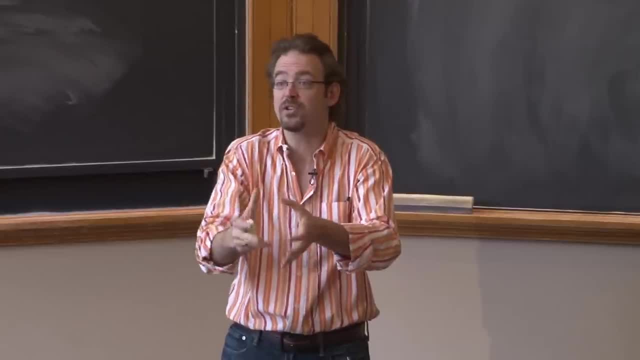 But from last time you know that's just some stupid matrix And you can express that matrix in any basis. you want, For example, the basis of up and down in the z direction, which is what we used last time, And then you can find the eigenvectors of that. 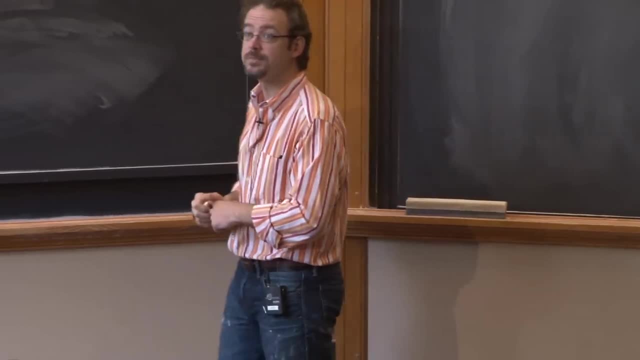 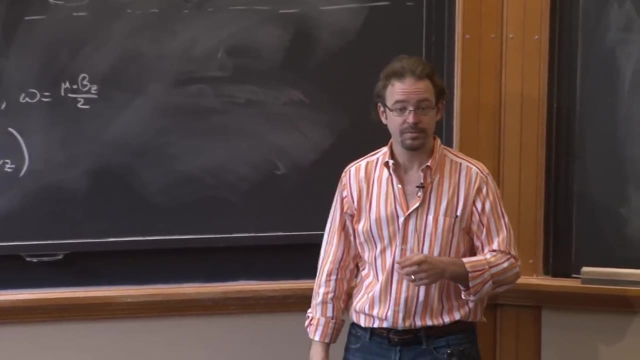 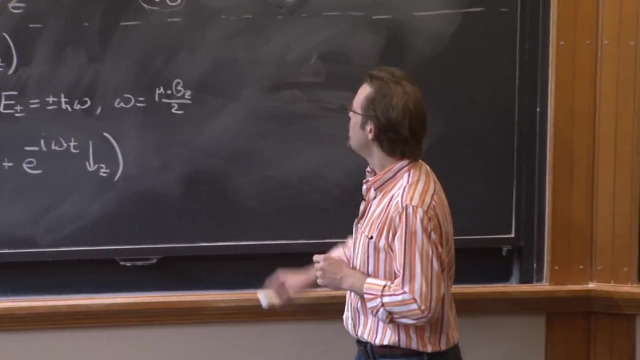 And that's how you find these states. So there's a very simple generalization. It just involves an extra angle, theta, which is the angle around the equator. OK, Sorry, phi, My extra angle phi. So we then did the following thing: 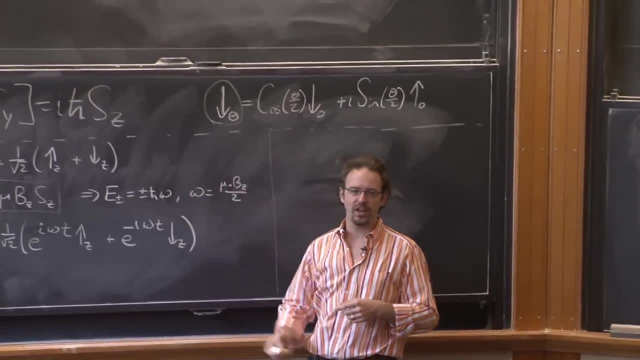 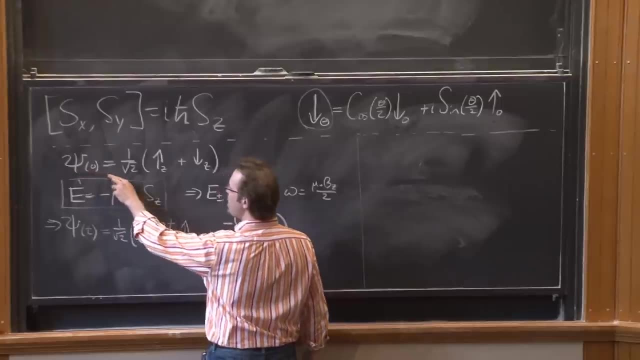 I talked about the Stern-Gerlach experiment, And here I'm going to abstract away from the Stern-Gerlach experiment. the core of the nugget, the core of it And the core of it is this: Suppose I have some spin. 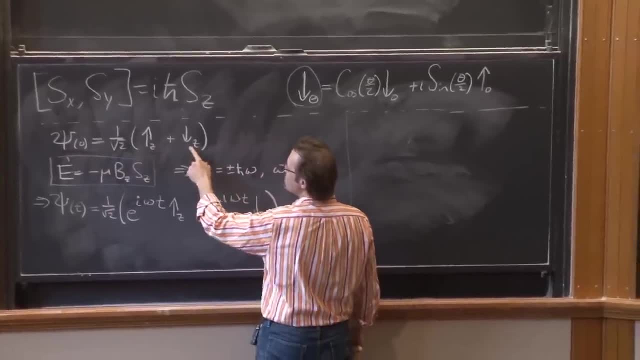 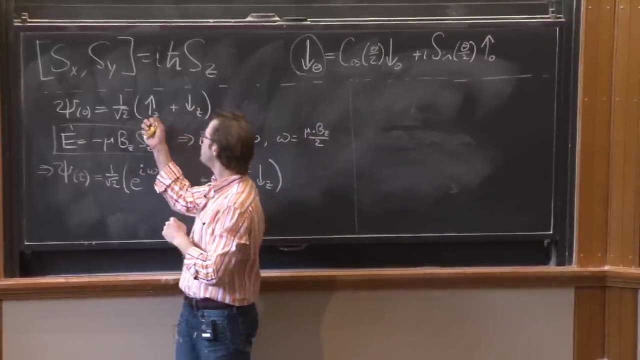 And I put it in a particular state. Let's say, for simplicity, up in the z direction plus down in the z direction, with equal amplitudes, So they're equally likely to be measured, And then these two states should be degenerate in energy. 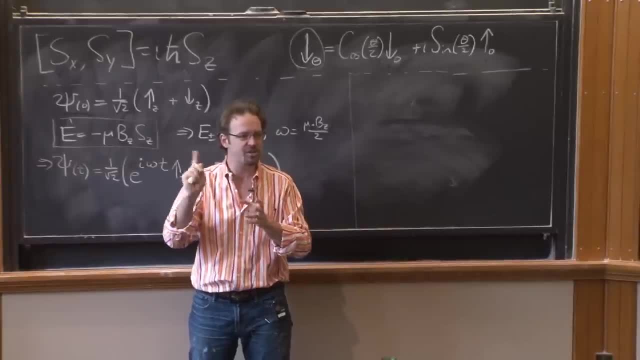 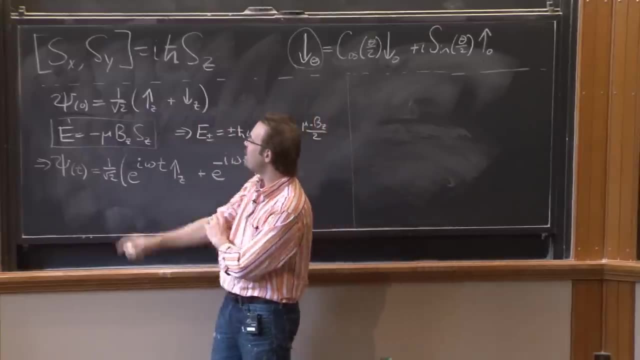 because the system is rotationally invariant. It's just a spin sitting there. There's rotational invariance. So we know that the energy can't depend on the z component of the angular momentum. But we can break that symmetry and break the degeneracy. 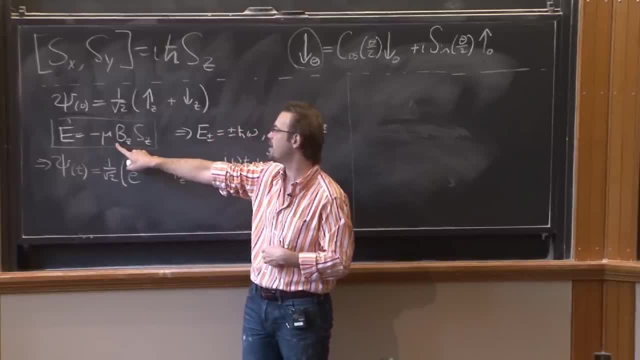 by turning on a magnetic field. So for a Stern-Gerlach experiment we turn on a magnetic field. that had a gradient, But I just want to look at a constant magnetic field for the moment and see what it does. So we turn on a constant magnetic field. 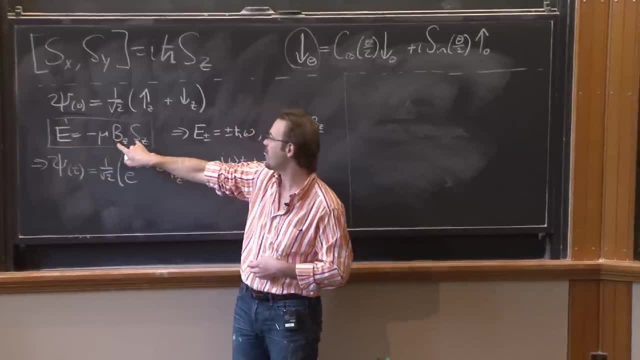 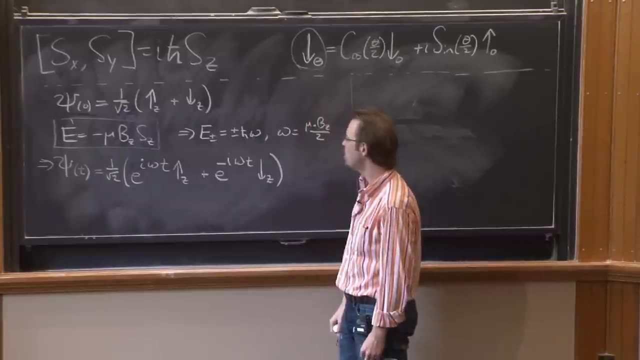 That's a contribution of the energy, which is minus the magnetic field dot, the magnetic moment, which is a constant, That's the spin. But if the magnetic field is in the z direction, then this is just bz sz. So we then found yesterday that this: 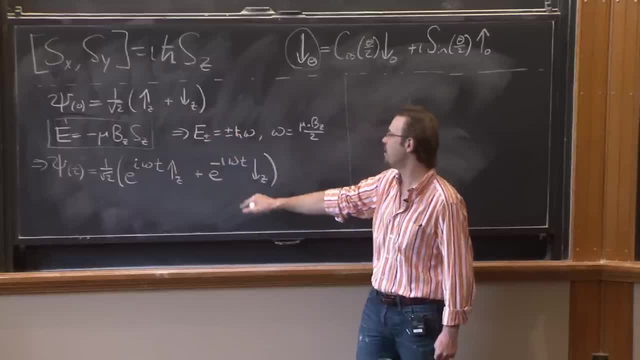 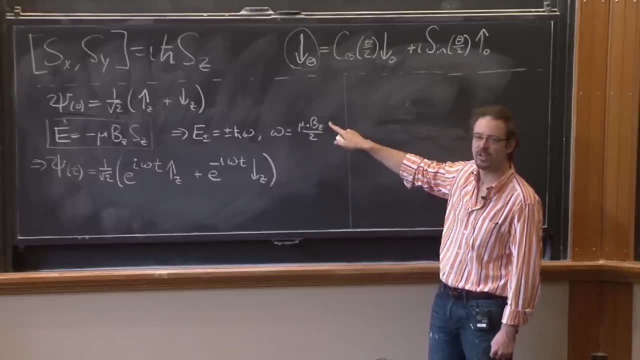 led to a splitting that the up state had energy plus h bar omega and the down state had energy minus h bar omega, where omega is given by mu 0 bz upon 2.. Yesterday we had an additional term which involved the z dependence, the beta z term. 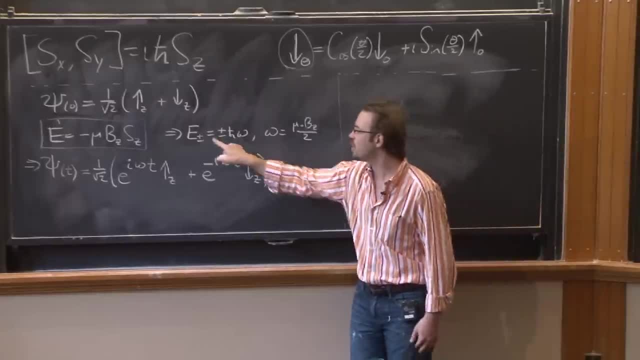 But here I'm just looking at a constant magnetic field. But if we know what the energies are, these are still the eigenstates of the energy operator. If we know what the energies are, we know how the system evolves in time. Here's the initial state. 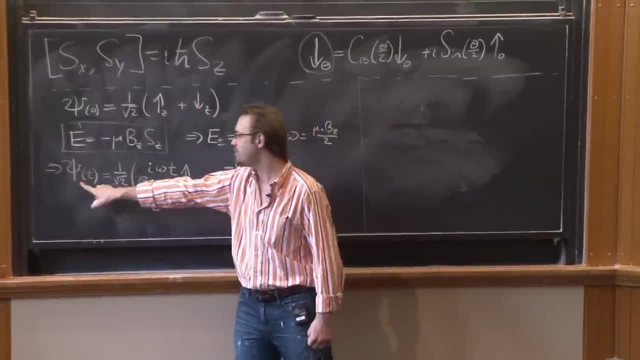 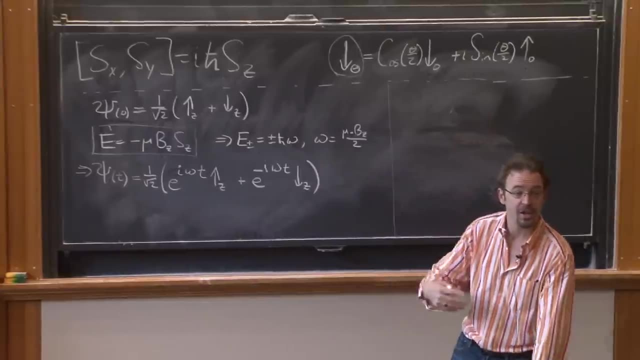 These are the eigenstates, The energies are these. So we can let the system evolve in time And we find that all we do is we evolve the system with phases. This is as usual in quantum evolution, If you have an expansion of a state in energy eigenstates. 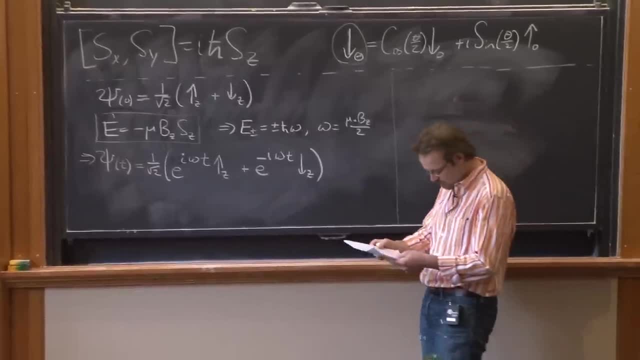 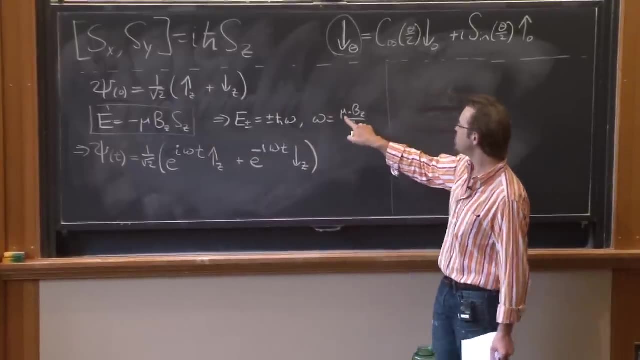 time, evolution is just phases for each term. But note that there's a simple thing, This omega, the thing that determines the rate of evolution of the phase, is controlled by the magnetic moment, which is something intrinsic to the spin, and the magnetic field, which is something I can dial. 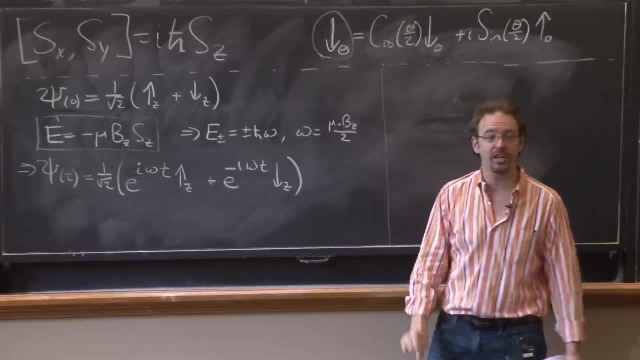 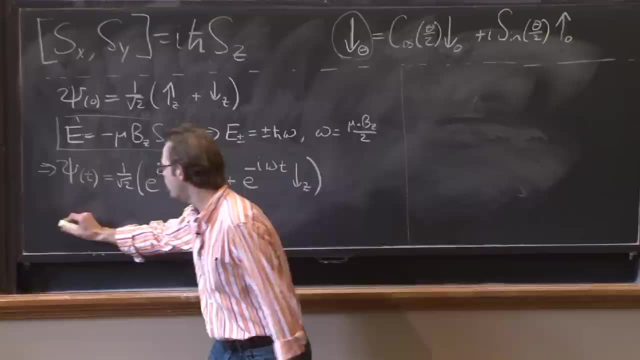 in an experiment I can really tune it. Meanwhile I can decide how long to leave the magnetic field on. I could turn the magnetic field on for a while. I could turn it off a while later. So suppose I leave the field on for a time t. 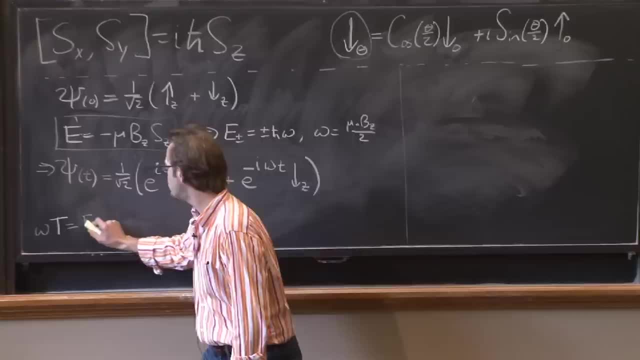 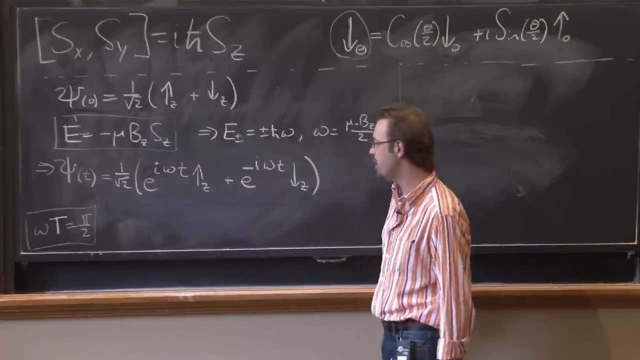 such that omega t is equal to pi upon 2.. So I turn on a magnetic field for a time t, such that omega t is pi upon 2, or t is equal to pi upon 2 omega. What is the state then afterwards? 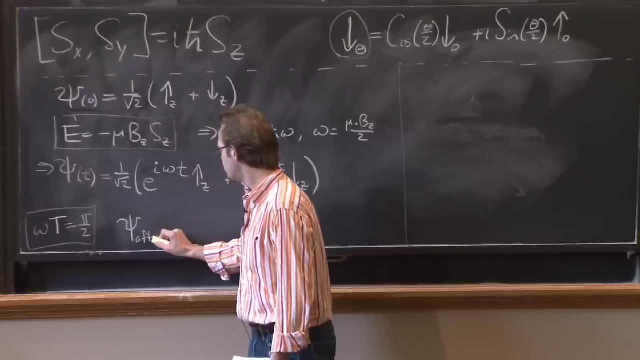 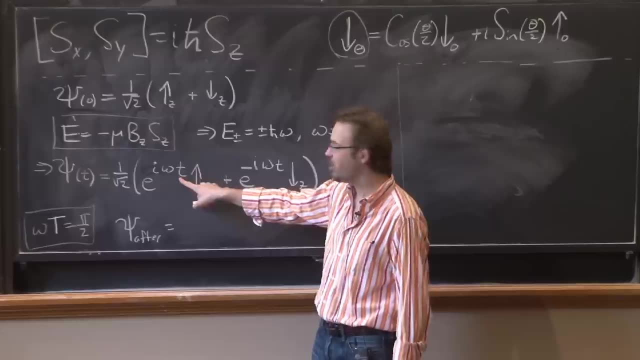 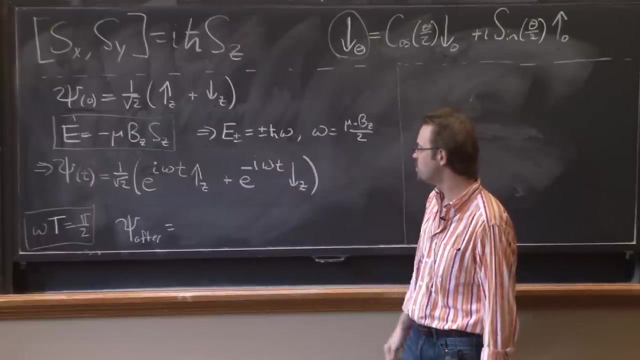 The state subsequently psi after is equal to. Well, It's this guy with omega t equal to pi upon 2.. But what's e to the i pi upon 2? i And e to the minus? i pi over 2 is minus i. 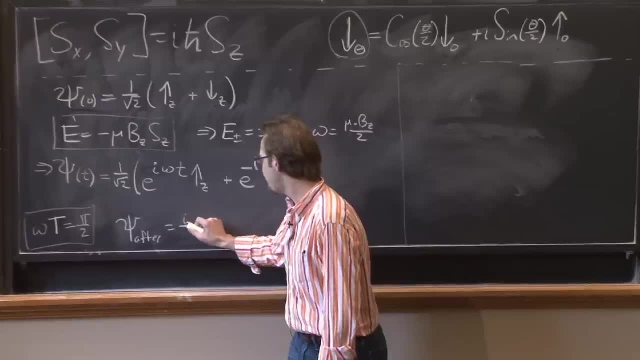 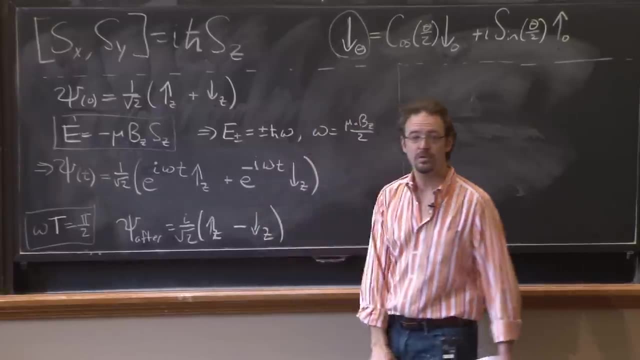 So this is an i and a minus i. I can pull out the i, So the phi after is i a phase upon root 2, times up z, minus, down z. Yeah, That's cool, And this is a state that we saw last time. 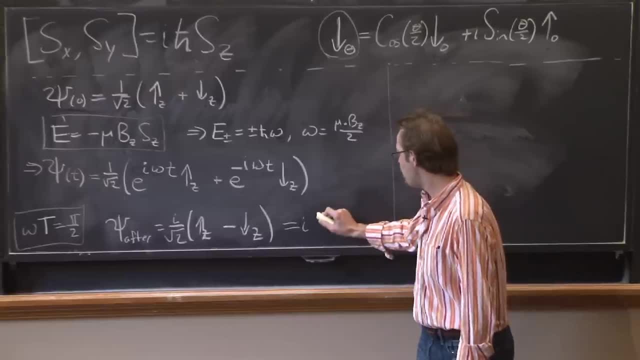 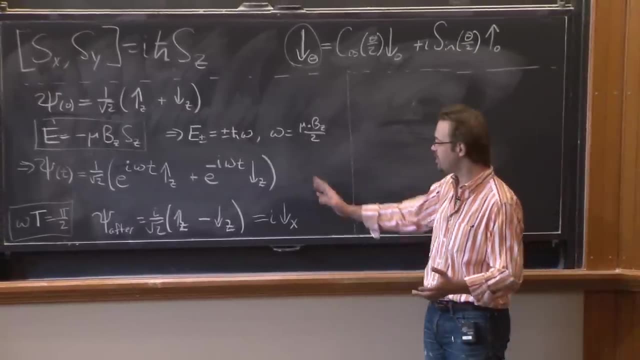 It's actually up to normalization, which is just an i up or down, x down in the x direction. So what this lets us do is something really quite cool. What this tells us and all these calculations are just the Stern-Gerlach calculation. 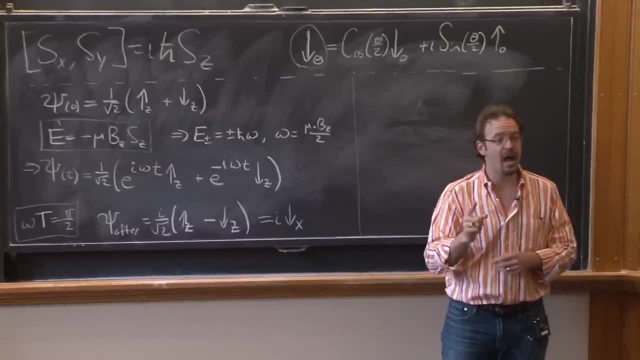 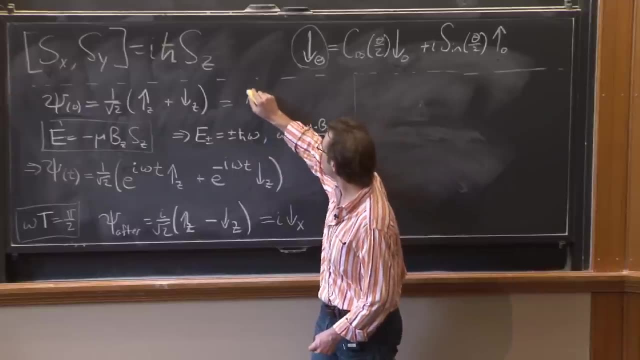 but even easier because we don't have a gradient. If we turn, if we have the spin in some superposition, which incidentally was initially up and down in the z direction, this is equal to up in the x direction And we turn on the. so we have in x, we have it up. 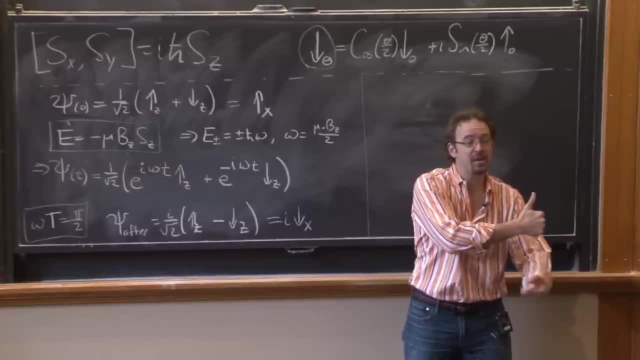 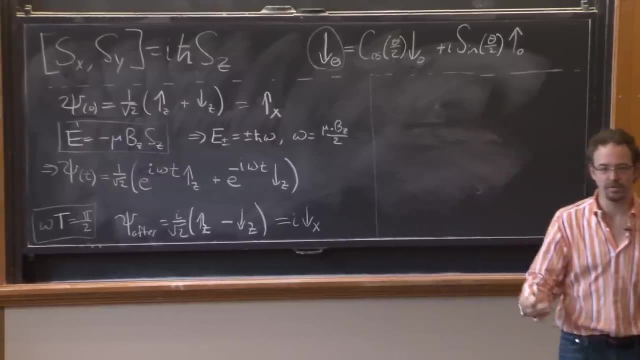 We turn on the magnetic field. We have the magnetic field in z And what happens is the spin precesses around the z-axis And we get down. We get precession. Here's the important point. The important point for everything that's going to follow is this: 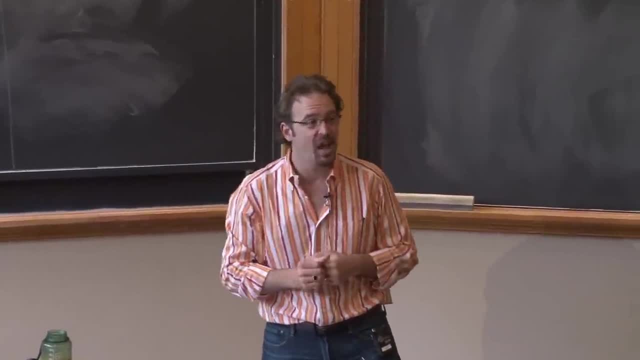 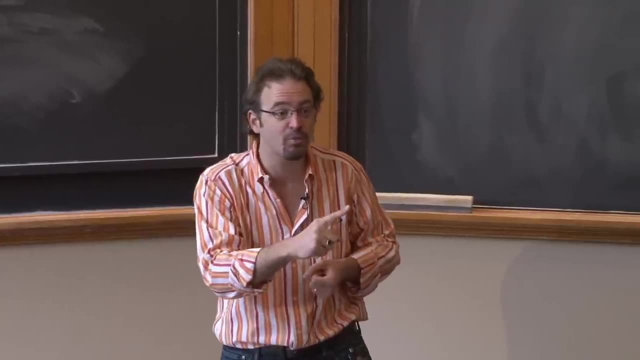 If I have some spin state and I want to take it to some other spin state, how do I do so? Well, I can build a machine that does it by turning on the appropriate magnetic field and having the magnetic field precess the spin. 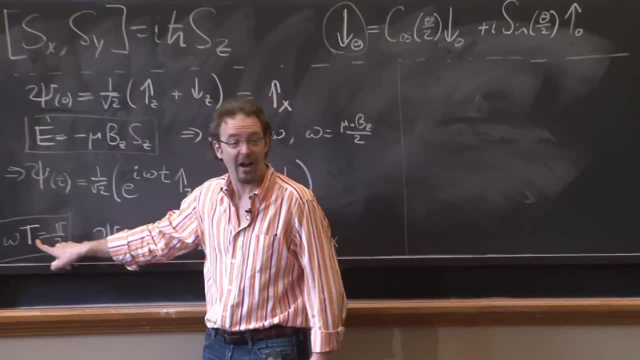 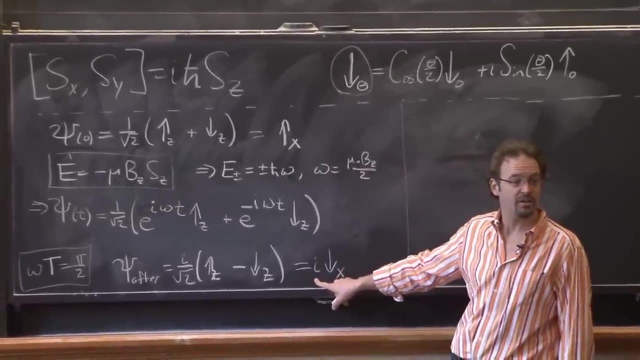 Here I found exactly what magnetic field I need to turn on, with what amplitude and for how long, Such that I take the state up x to down x with a known phase. i Everyone cool with that. So any unit. here's the thing I want to convince you of. 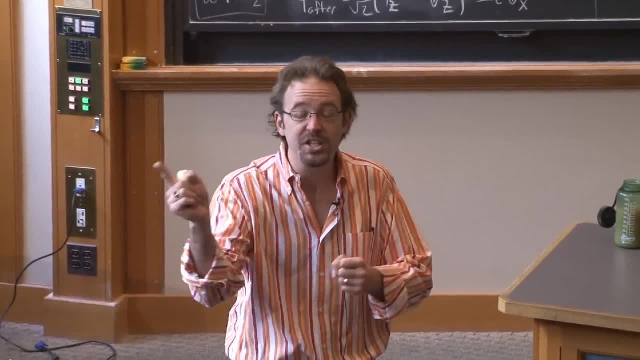 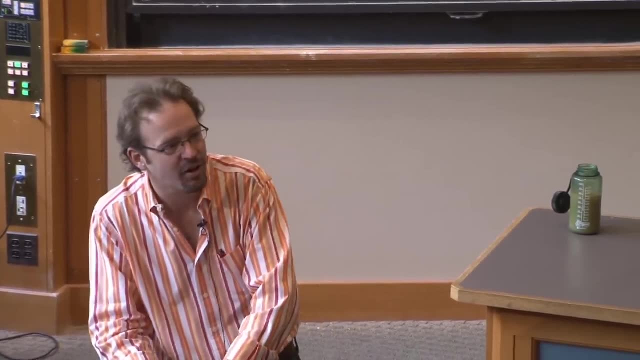 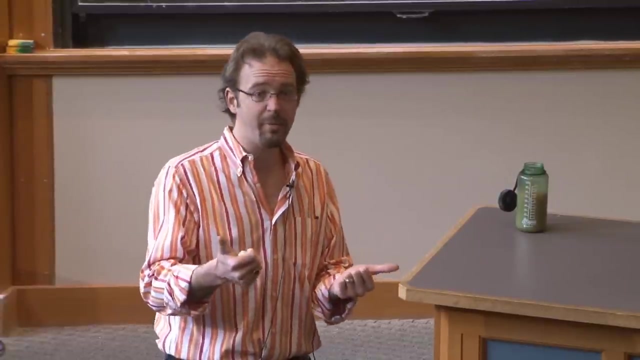 Any unitary operation that takes you from one vector to another vector or from one spinner to another spinner. up z, down, y. linear combination of up and down z. some particular linear combination of up and down x. Any such pair of vectors can be related. 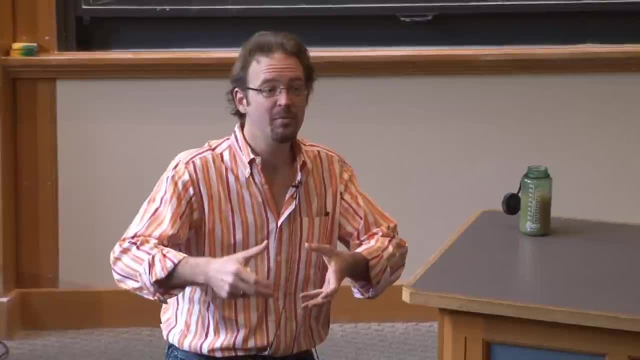 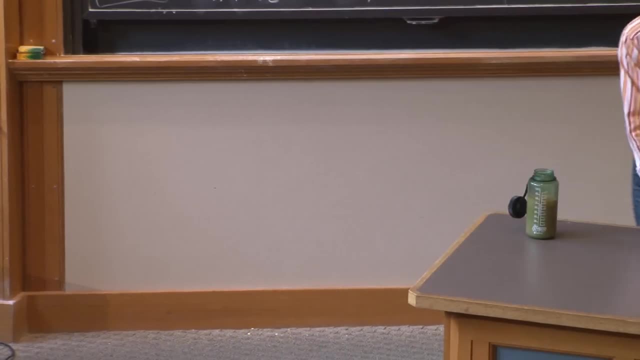 by unitary transformation And any such unitary transformation. unitary transformation can be built by some series of magnetic fields. That cool, And you can prove this to yourself quite quickly, but let me just state it. So now, this gives us the ability to do the following: 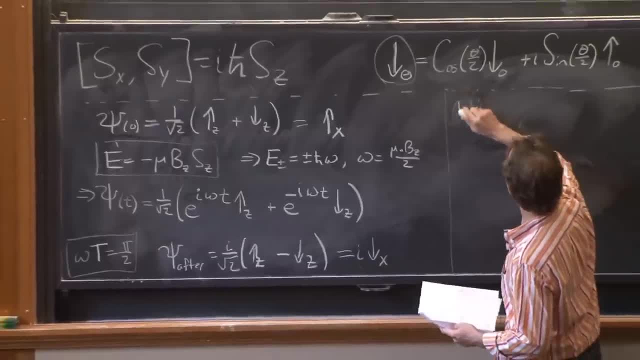 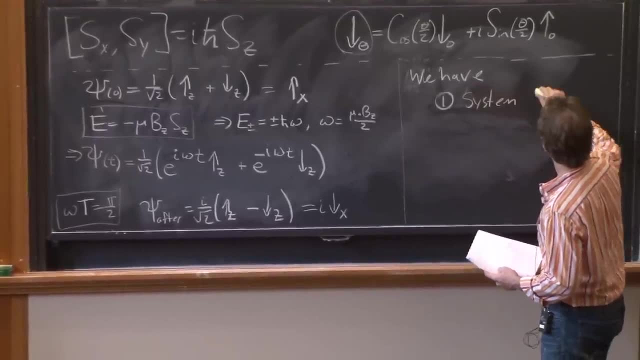 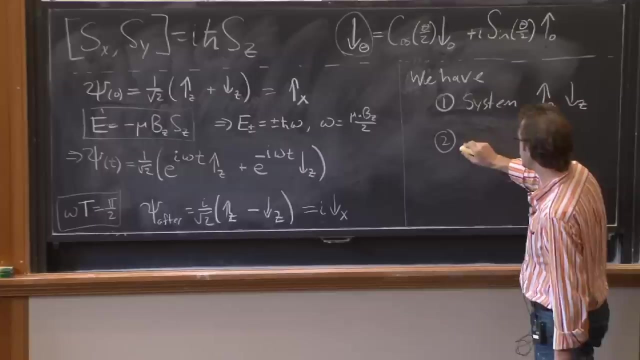 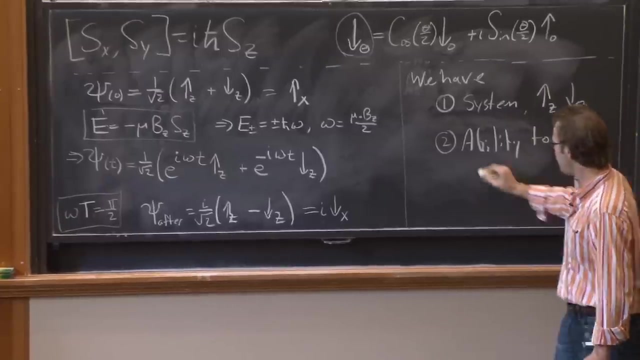 One we have. so what do we have here? We have when we have spins? one, spins that can be put in a system, that can be put in states like up, z and down z And two: the ability To rotate states, ability to evolve states from state. 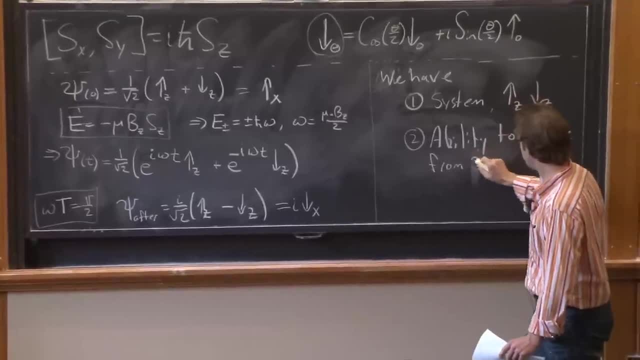 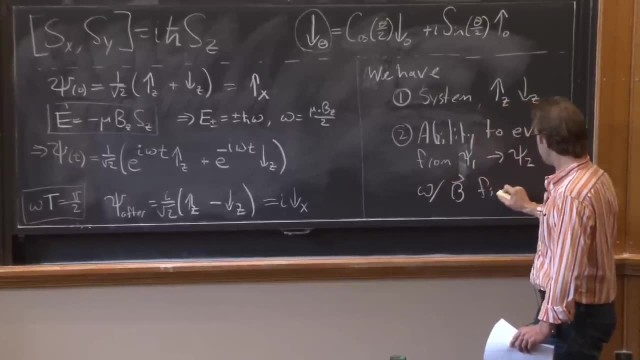 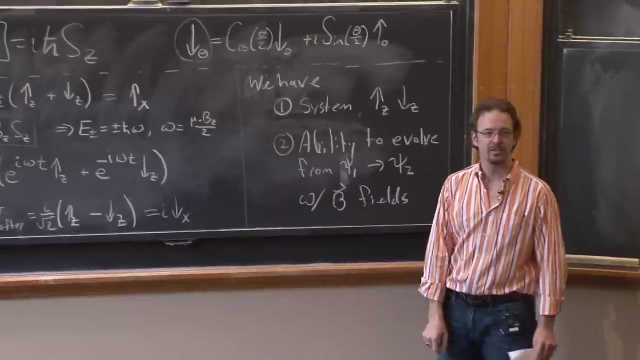 to state from spin state one, psi one to psi two, by turning on some magnetic fields, So by suitably choosing our magnetic fields. Everyone cool with that. So here's a question I want to ask: What do we do with this? 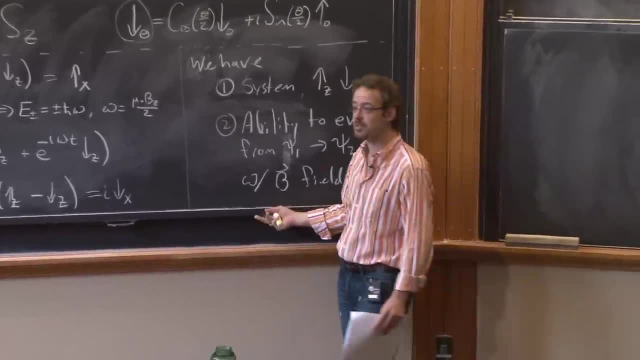 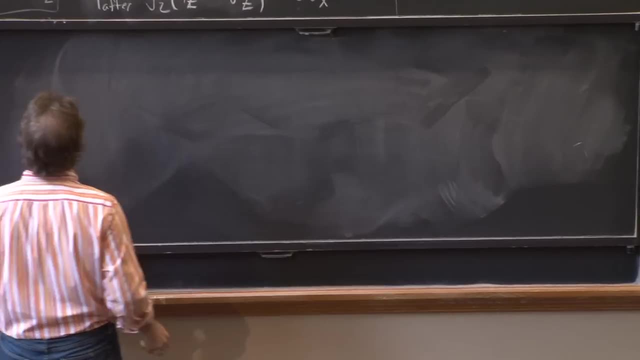 Imagine we really had this equipment in front of us. What power, What awesomeness could we realize? And this is the entry point to quantum computing. The answer to what can you do with this cool machinery is: you can build a quantum computer. 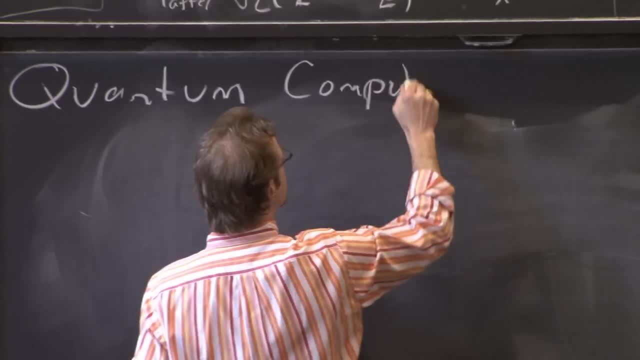 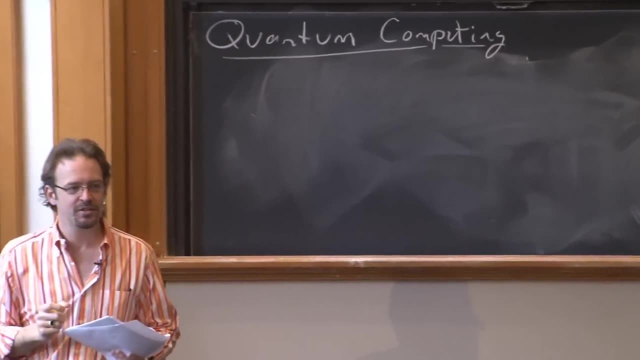 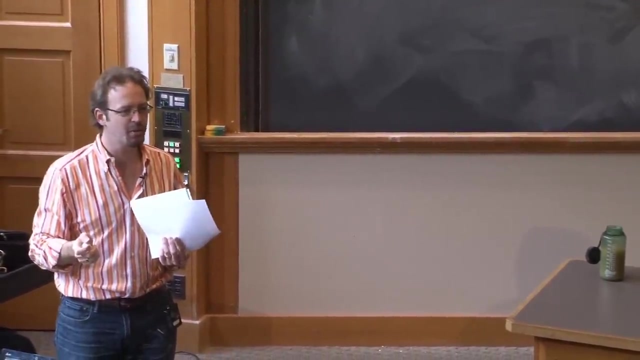 So let's talk about what that means. So quick question: do quantum computers exist? Yeah, are they very big? No, OK, the biggest quantum computer that's been built, to my knowledge, is one that has factored the number 15, although they might have done 21 at this point. 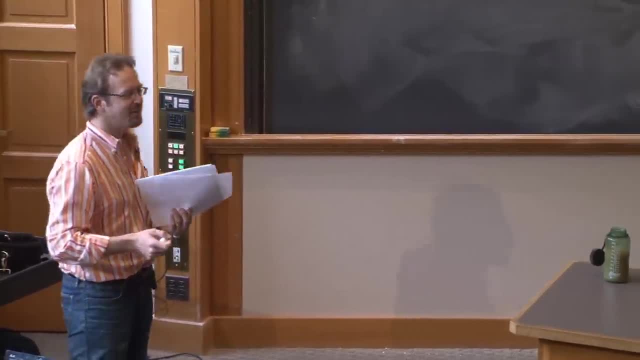 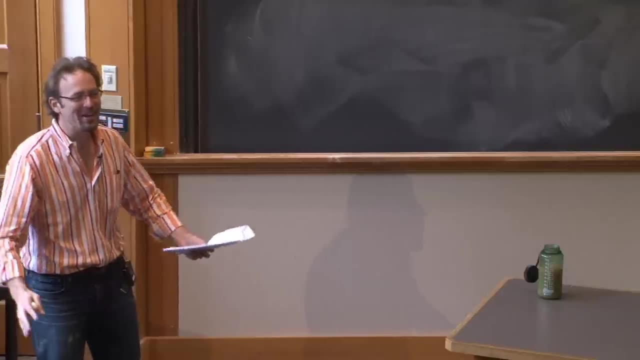 I'm not exactly sure. 21, done? Yeah, OK, 21's done. Good, so that's the upper end. Yeah, Well, they're large physically. It's true, they take up a room, or at least a large tabletop. 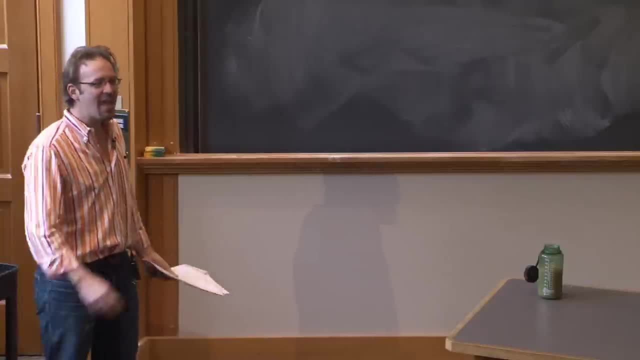 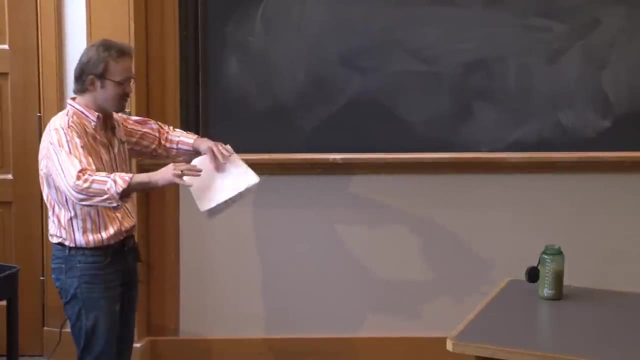 an optics table, But they're not very big in a useful sense. And there's actually interesting reasonable people, not just reasonable intelligent people And reasonable- that's a non-trivial- The people who live at the intersection of intelligent and reasonable. 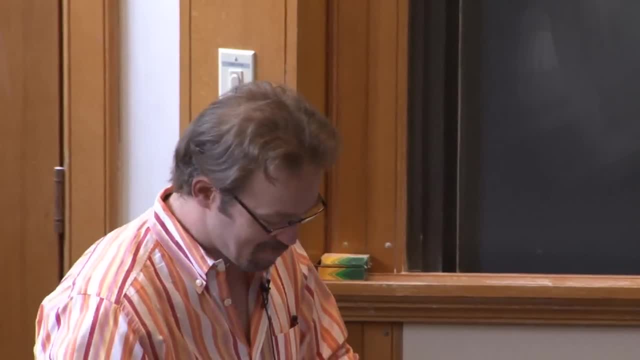 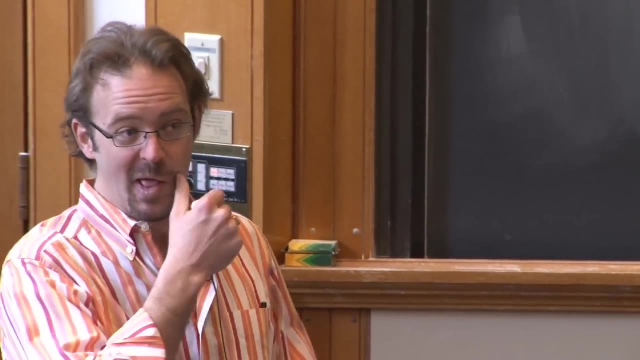 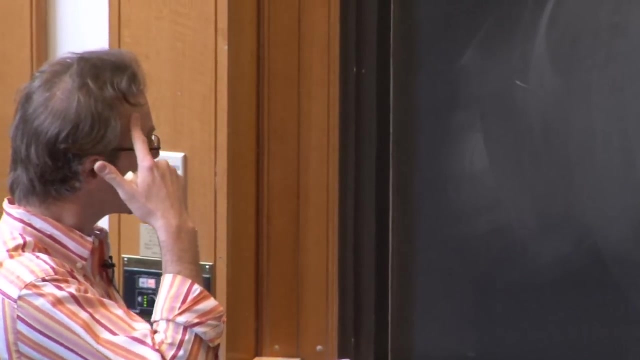 OK, Which admittedly, as my colleague is pointing out, is not a large overlap. There are people in that overlap who suspect that it's for some fundamental reason impossible to build a useful quantum computer in some deep, deep sense. I don't know whether that's true or not. 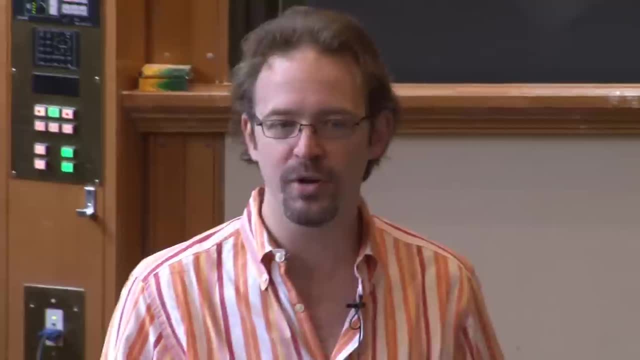 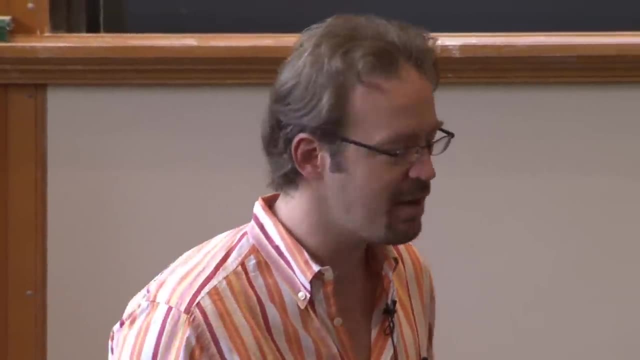 but we're about to engage in a discussion of what happens when you build quantum computers for n bits, where n gets large like millions and billions, as you need for codes or for studying images. And of course it's a little strange because such a computer doesn't exist. 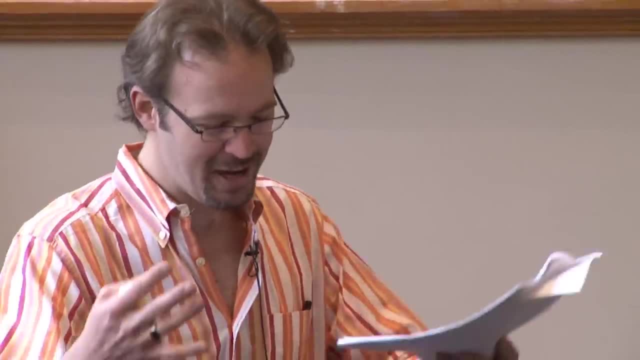 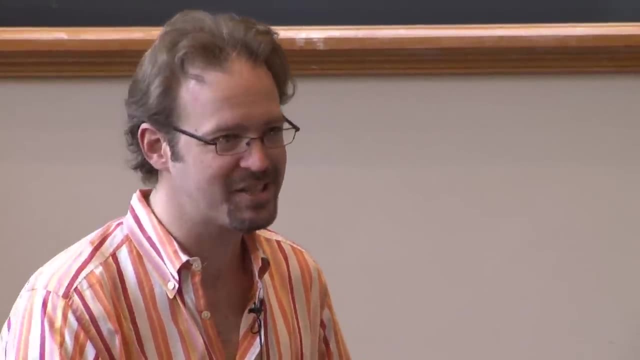 which leads to my colleague and friend Scott Aronson's lovely comment that his job as someone who studies quantum computers is to prove things that can't be done with computers that don't exist, which is what we're about to do. So let's talk about quantum computing. 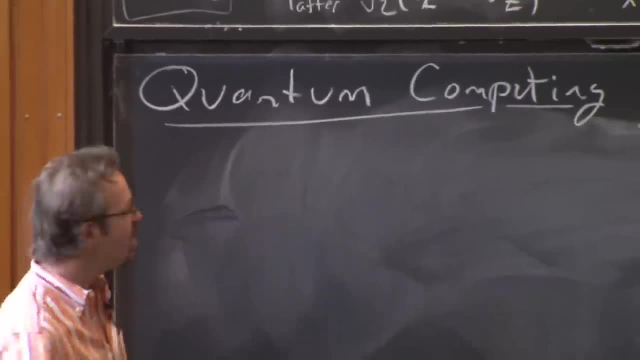 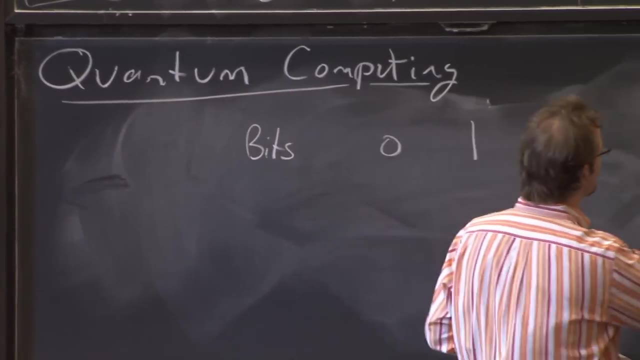 So what do I mean by quantum computing? Here's the basic idea. Let's talk about classical computing. Classical computing says I have these things called bits, which are binary objects that are either 0 or they're 1. And we realize them in a very particular way. 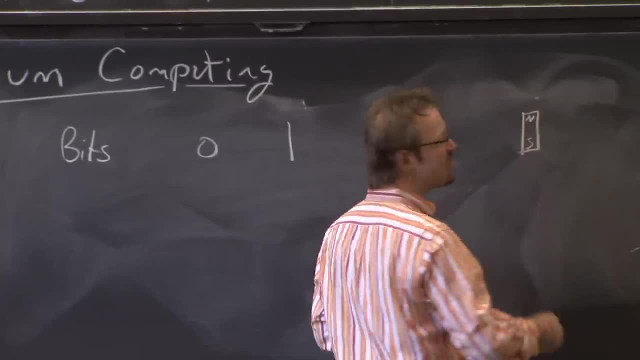 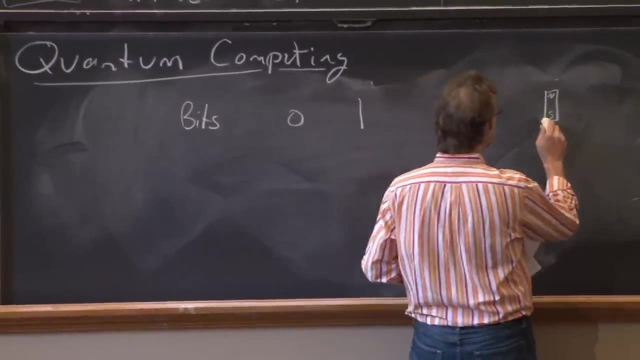 We realize them with a little magnet which points north or south. Now, it's not always exactly a magnet. It isn't like an old hard disk In your computer. it's something a little more fancy than just a magnet, but it's still basically a magnet. 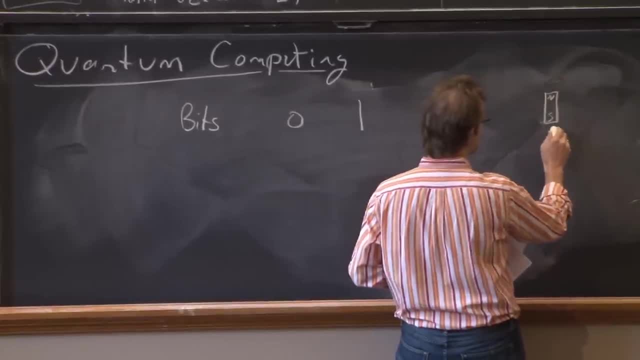 And you have something north south, And whether it's pointing south down here, which I'll call 0, or whether it's pointing north down here, which I'll call 1, determines whether you call this 0 or 1.. 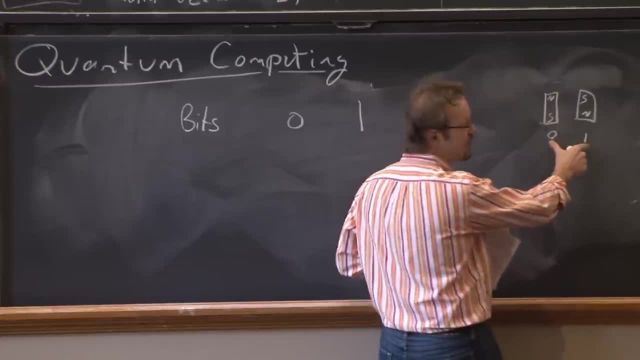 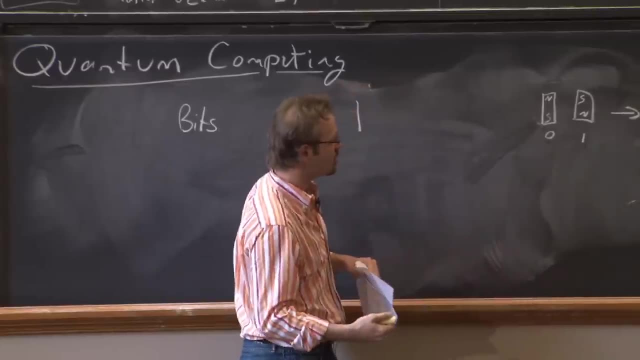 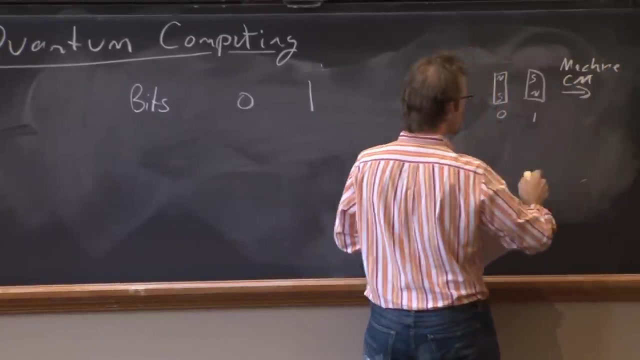 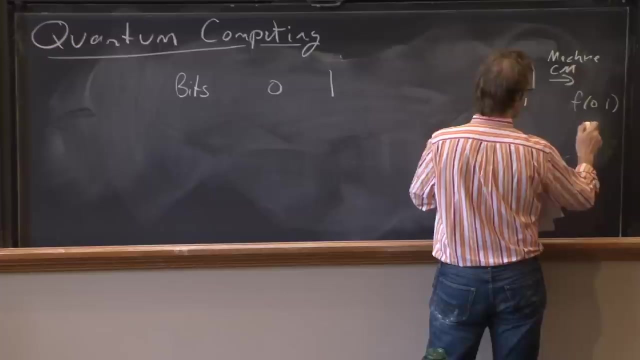 And classical computation is: your data are a set of numbers. what's pointing down? And quantum computing? The process of doing a classical computation is build a machine which is governed by classical mechanics, that takes this initial configuration and replaces it with a new one, f of 0,, 1, which is also some number. 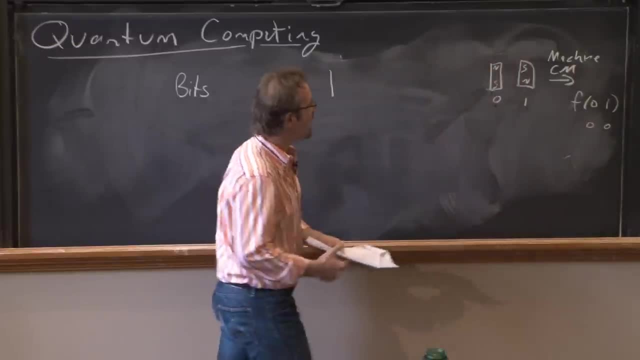 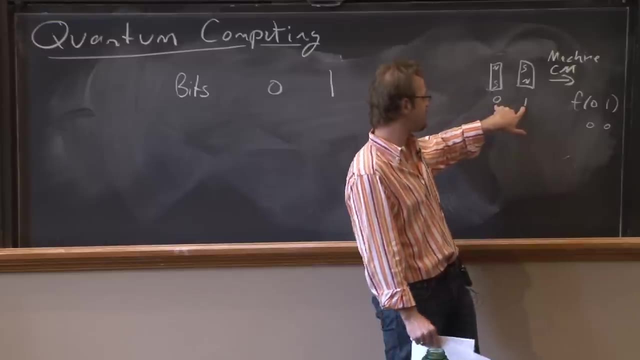 So maybe it's 0, 0. I don't know It's whatever f is, And what you want to do is you want to perform some calculation, which is some function, a known function of your input variables function, in this case, of two bits, which. 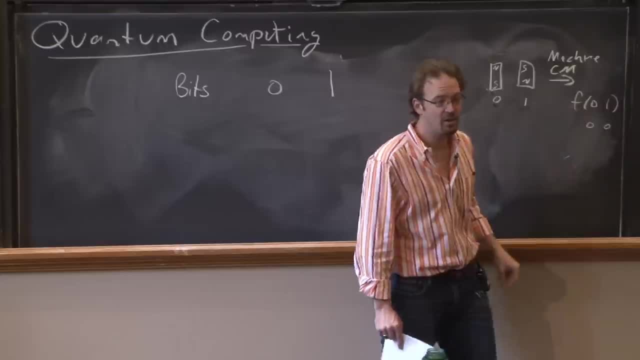 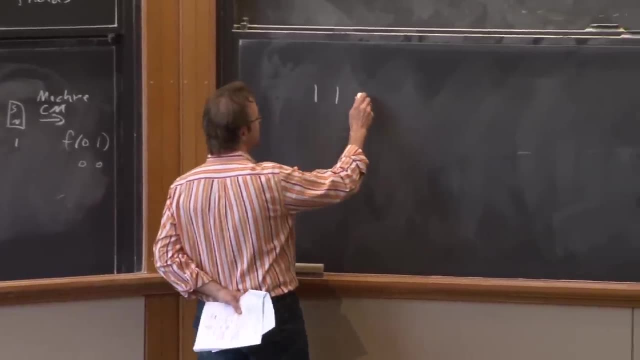 produces the output that you want, And you build a machine that does that. So let me give you an example. I want to build a classical computer that takes a string of binary integers: 0, 0, 1, 0, 0,. 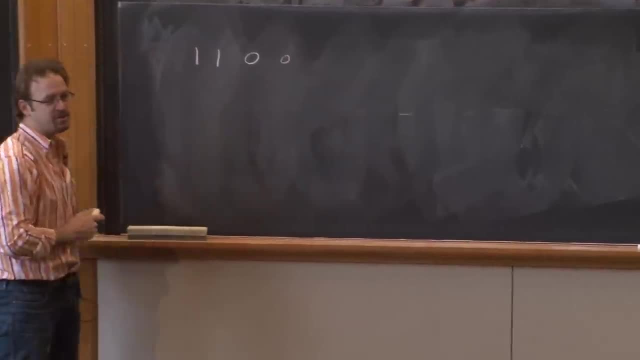 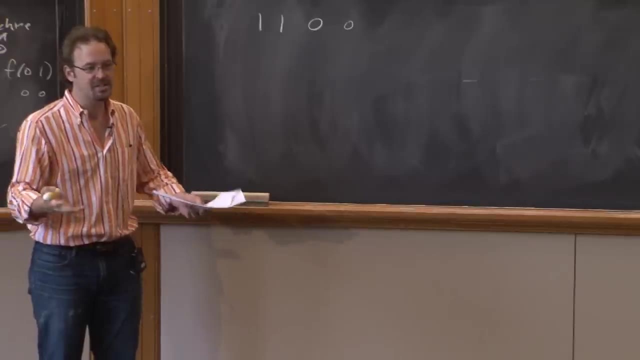 and performs a logical knot on each bit independently. So I need to build that computer out of objects available to me And I need to use nothing other than the laws of classical mechanics. That has to suffice to describe the system that I'm going to. 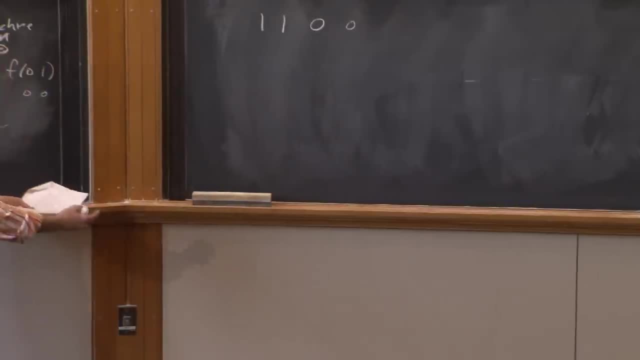 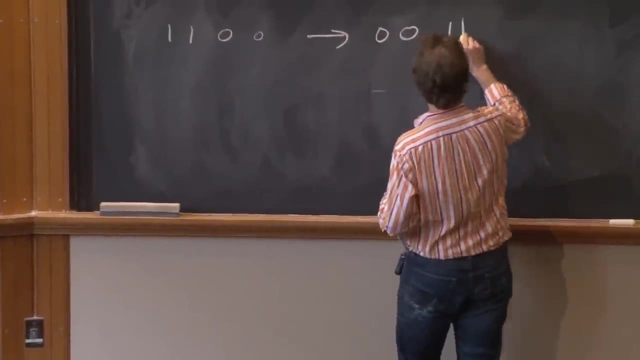 So let me give you an example of such a computer. Why, Alan, Why don't you do this calculation? So that's the input, And I am now the classical computer: 0,, 0,, 1, 1.. Now, that's not actually what you do in your cell phone. 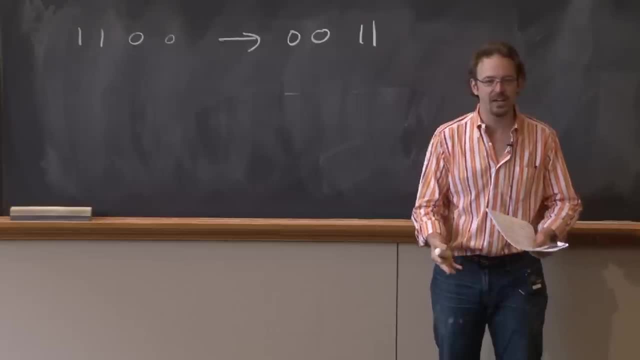 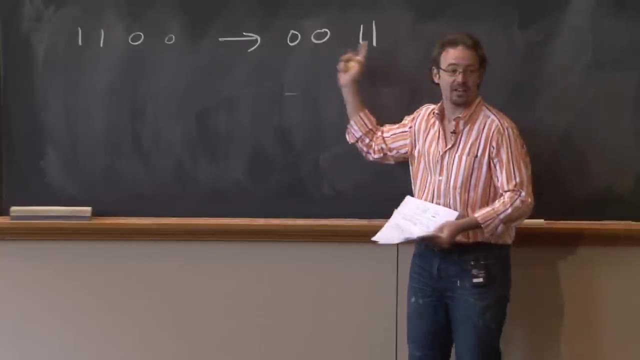 or on your laptop That uses transistors, But it's the same basic idea. You build a set of objects, magnetic fields, electric currents that affect this calculation, And so there's some relationship between what electric fields you turn on, what currents you induce to flow. 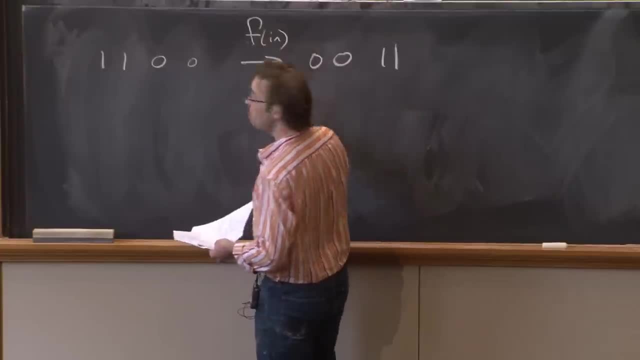 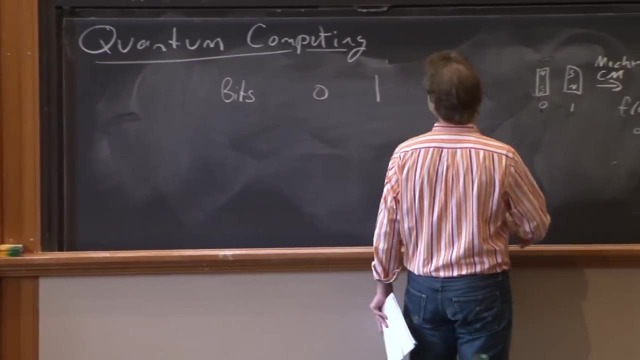 and the calculation you want to perform, f of the input. This is the basic idea of a classical computer With a quantum computer. we want to. oh, and one last thing. Suppose we have n bits, Suppose we have n classical bits. 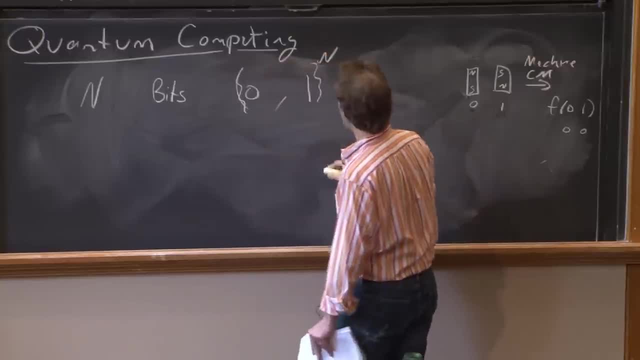 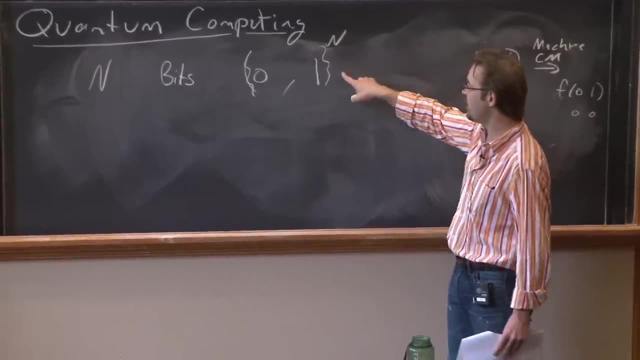 Then we have 0,, 1, the n, And how many numbers do you have to specify to specify the configuration of n bits? This is sort of No, you just need to specify the number of each bit. So we need n bits. 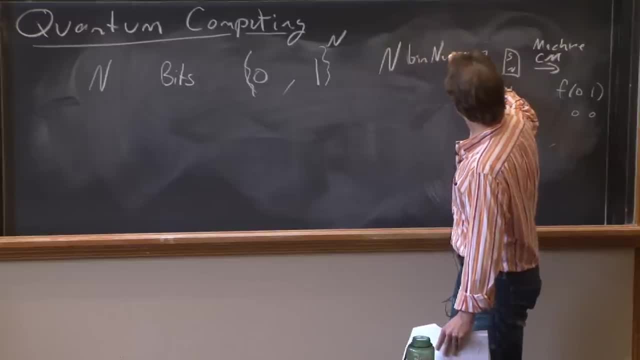 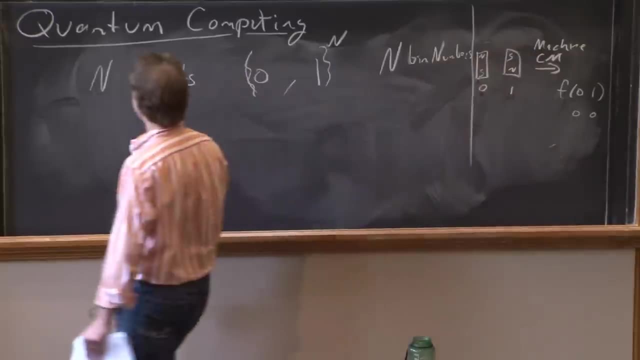 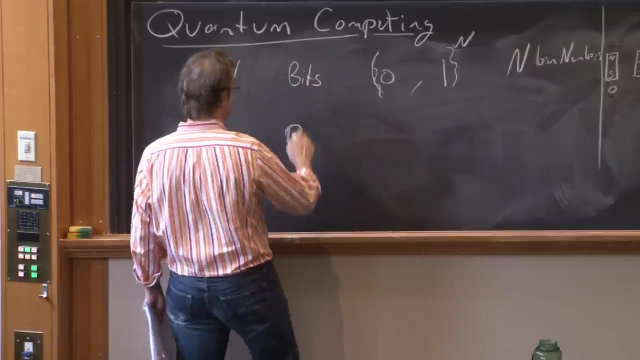 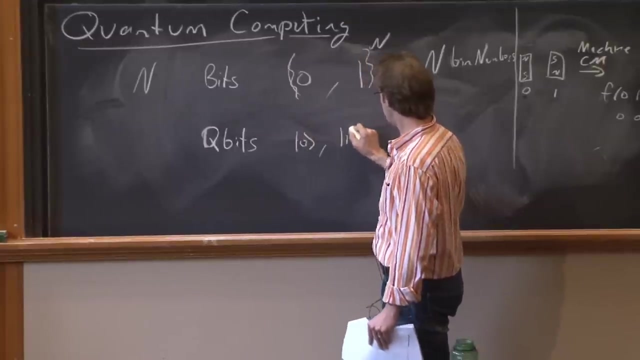 So n binary numbers. Remember that I specify what each register is and I'm done. Imagine this is quantum mechanical. Instead of having bits, let's take quantum mechanical bits, by which I'm going to mean a system that has two possible observable states: 0 and 1.. 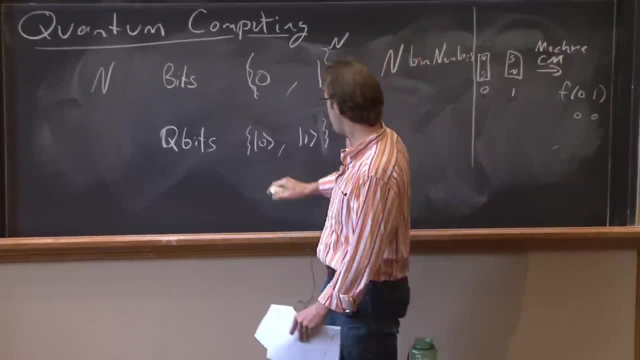 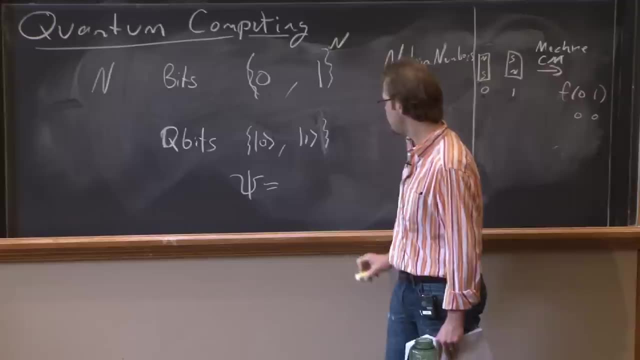 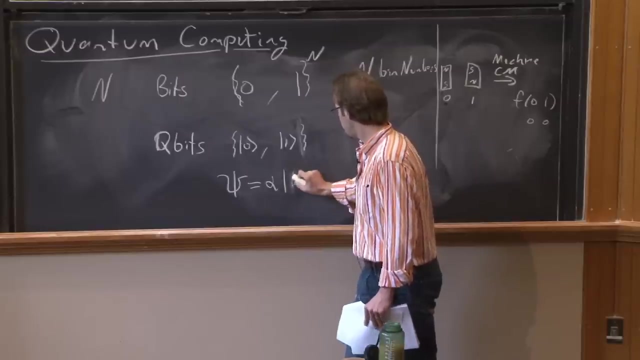 So these are the possible observable states And to specify a general configuration, I say that psi is equal to- and I'm going to represent this by well: psi is equal to some linear combination alpha 0 plus beta 1.. 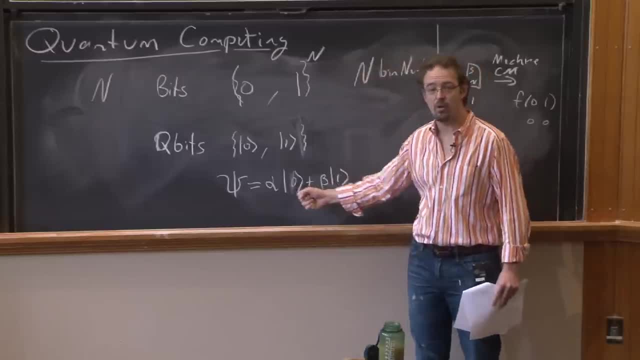 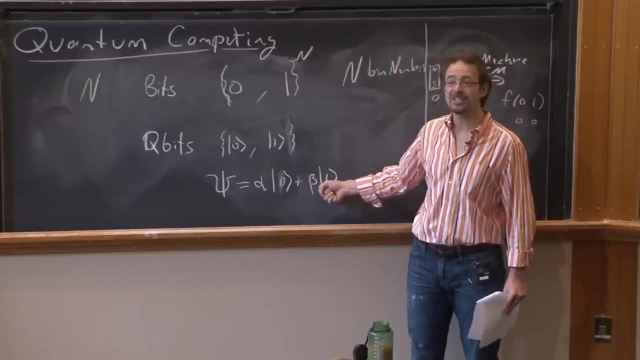 Now, if I measure, we know that we'll find either 0 or 1.. If we measure the spin in the z direction, we will measure either up or down. However, at a given moment in time, the system needn't be in a state corresponding. 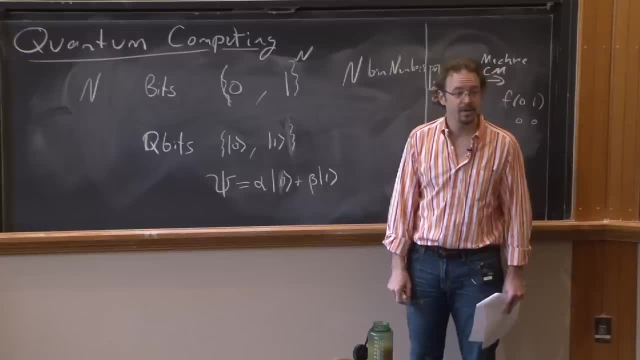 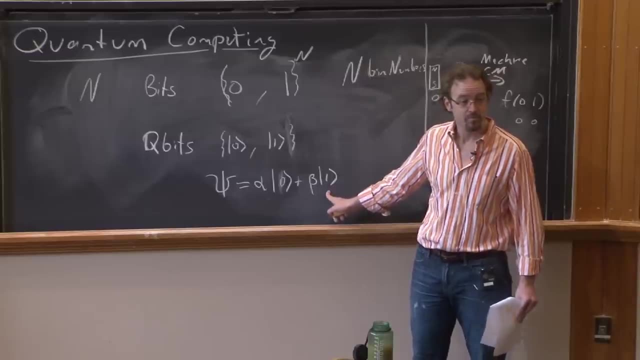 to a definite value of that It could be in a general superposition, Agreed. So now here's the question: how many numbers does it take to specify the state of a single quantum bit? Two complex numbers. It takes two complex numbers to specify the state of a bit. 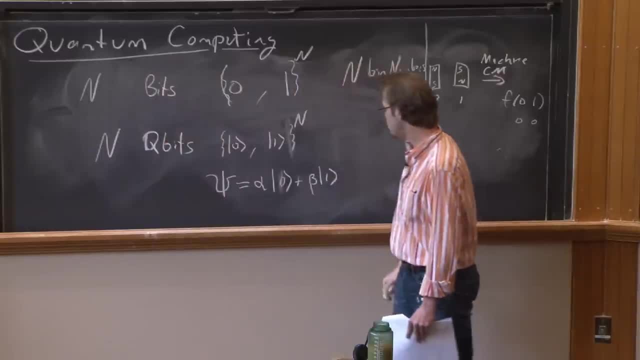 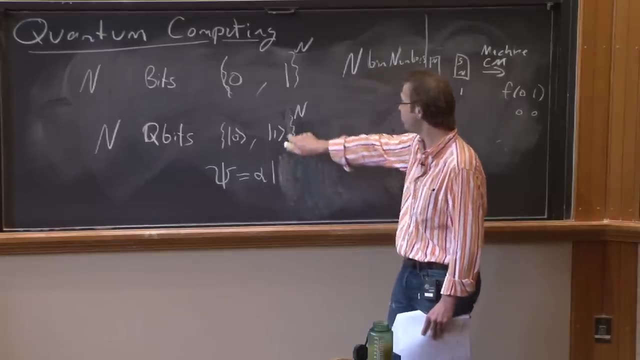 And if we have n qubits, then there are n of these guys. Well then, how many numbers does it take? Well, I have to specify the state of every possible. I have a possible superposition for every possible configuration of the system. 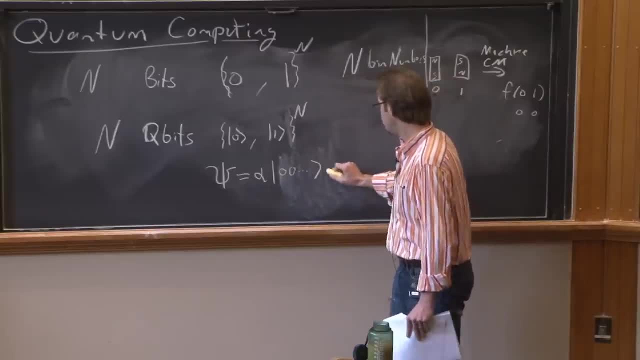 So, for example, they could be all 0,, 0, 0, dot dot dot 0, plus beta. the first one is 1 and the rest is 0, dot dot dot, plus. and how many terms are there? 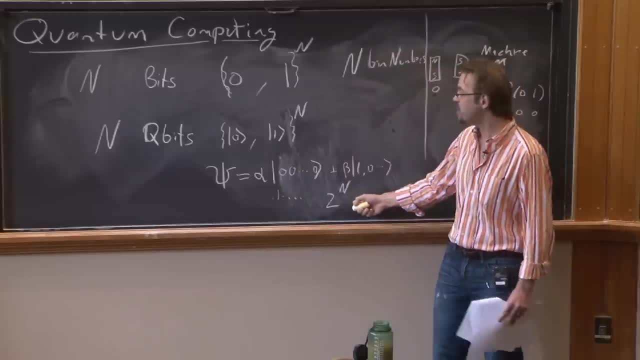 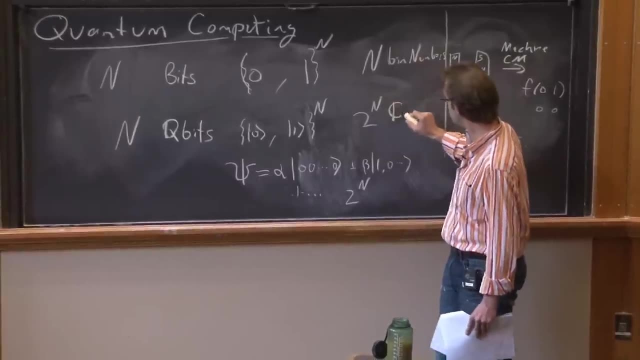 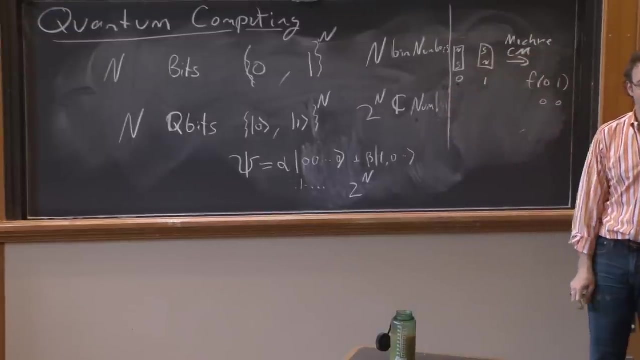 They're 2 to the n terms. So how many numbers do I need to specify the state of n qubits? I need 2 to the n complex numbers. Yeah, Everyone see that. So this immediately leads to a really frustrating reality we have to face. 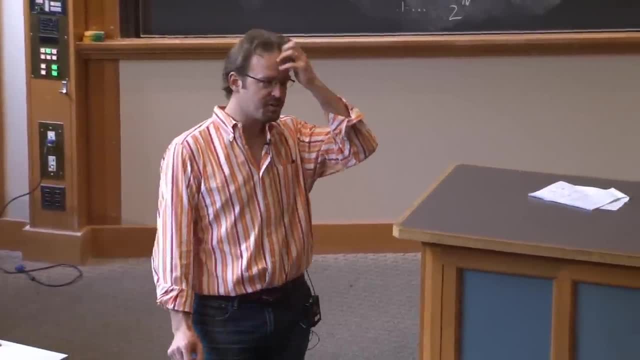 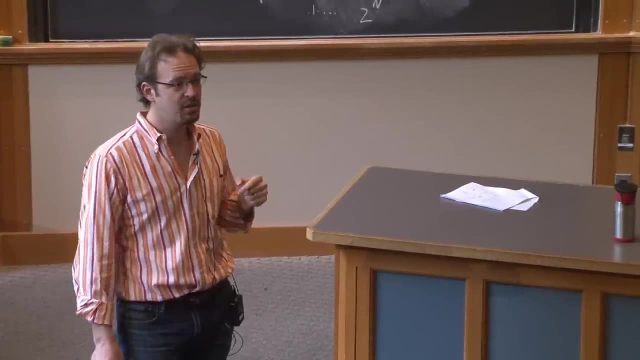 Suppose you want to simulate using a classical computer such as sits on my desktop. I wanted to simulate a quantum mechanical system of n bits or n spin. 1 half states evolving according to some energy function evolving according to some Hamiltonian. 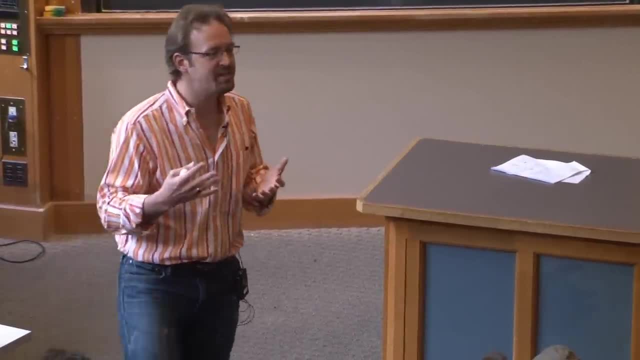 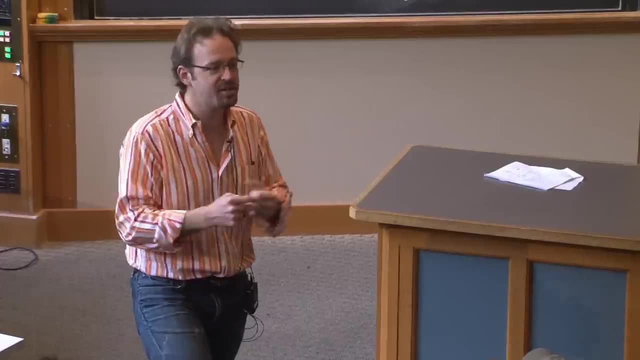 How many variables and how much memory will it take 2 to the n. If I've got n bits that I want to describe, it's going to take 2 to the n- complex numbers. So that's how many variables I have. 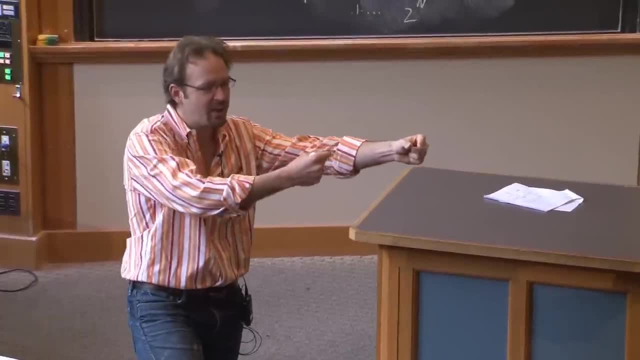 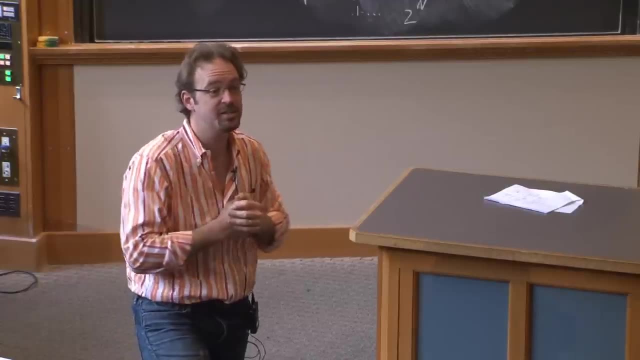 So if I have 10 bits, literally 10 little spin, 1 half objects to accurately specify the quantum configuration system, I need 2 to the 10 complex numbers And that's for 10 spins. How many spins make up this piece of chalk? 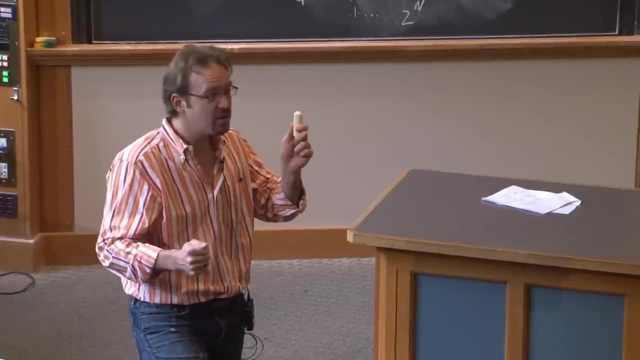 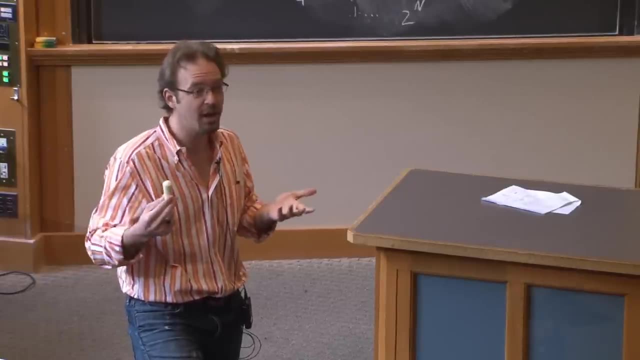 Right. So could you ever in an honest way simulate on a computer- on a classical computer like sits on my desktop- a quantum mechanical system the size of this chalk? Absolutely not. It's completely and utterly intractable. You have to come up with some sort of approximation scheme. 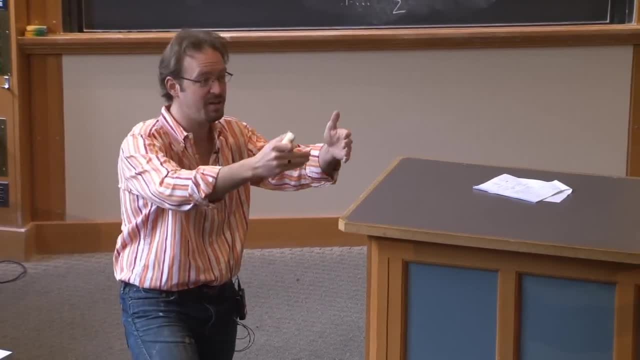 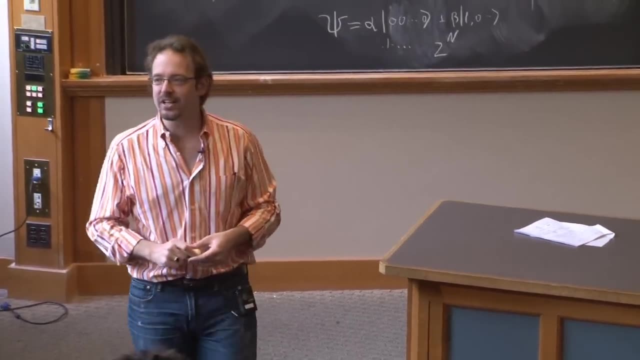 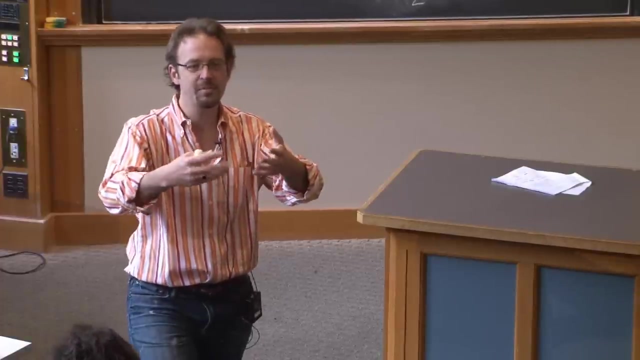 So simulating quantum systems directly by just taking it, taking the spins and representing them with a wave function is wildly inefficient, incredibly difficult. Interestingly, the converse is almost certainly not so difficult. It's almost certainly possible for a quantum system to simulate classical evolution quite easily. 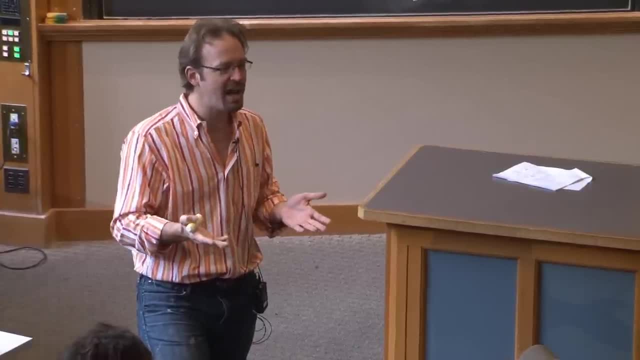 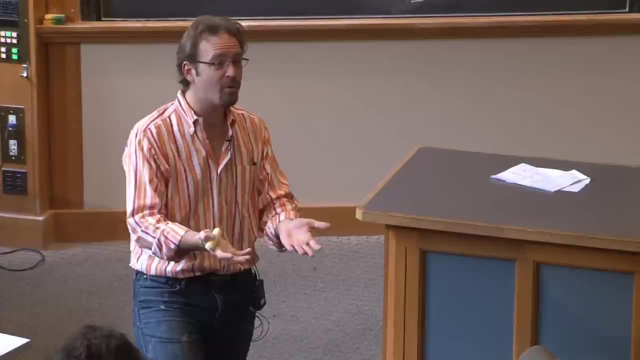 And how do you know that? Yeah, here we are exactly. Nature apparently has no trouble simulating classical mechanics with underlying quantum mechanics. Quantum mechanics is the operating system and classical mechanics is the system that's operating. It's the simulation, it's running in a very useful sense. 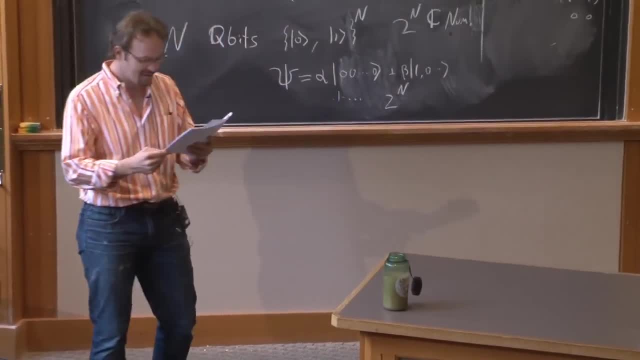 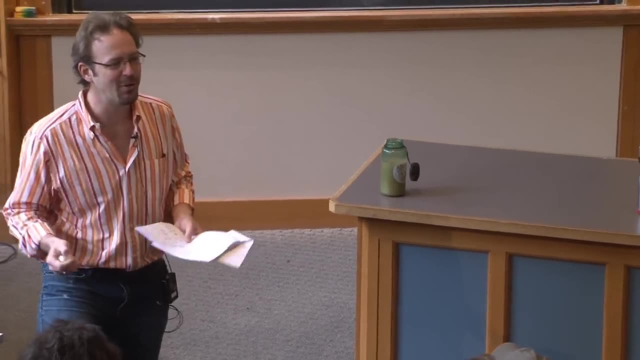 very real sense. So at this point Feynman, I think, was the first person who really pointed this out, But I don't know the details of the history. but the lore is that this was really Feynman's observation. 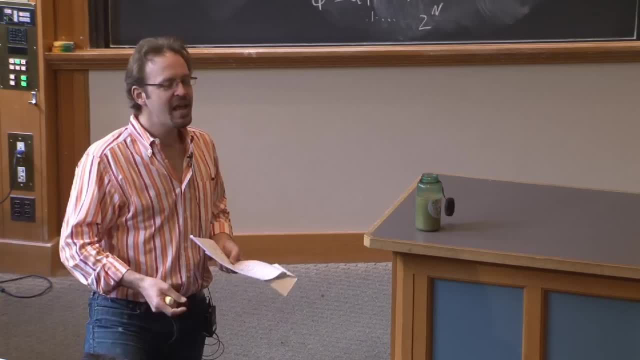 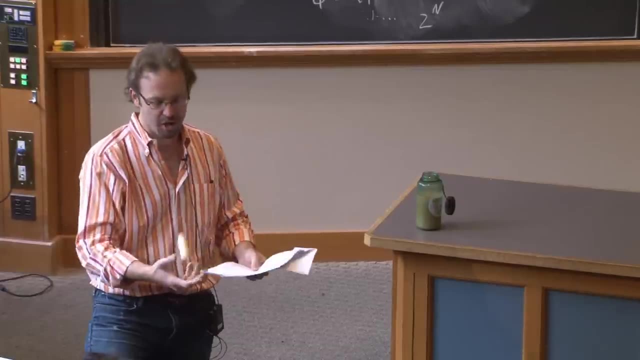 Look, if that's true, this opens up a real possibility for computation. If things like spins hard problems like calculating how spins evolve or even the motion of chalk And the motion of chalk in the room, can be done pretty efficiently by nature. 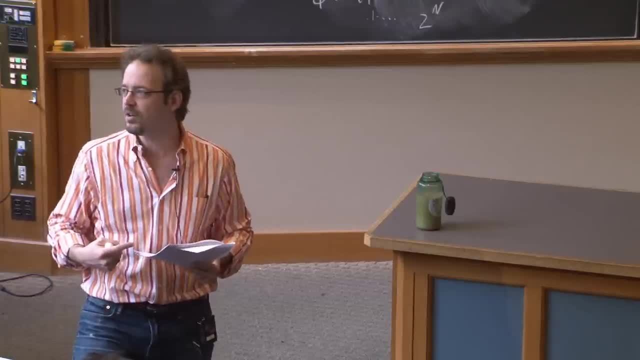 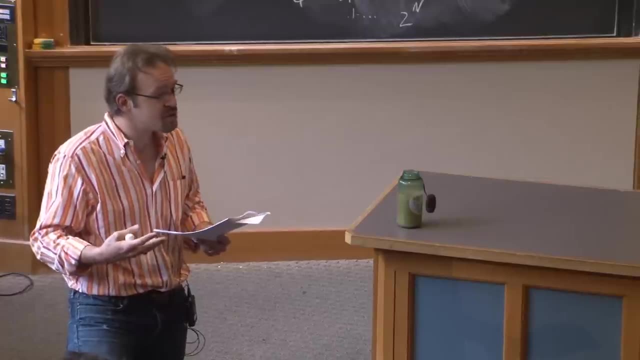 if we could build a computer that used quantum mechanical bits, whose variables were quantum mechanical and involved all the superpositions and interference effects of quantum mechanics, perhaps we could build computers that run exponentially faster and with exponentially less memory and less resources than a classical computer would. 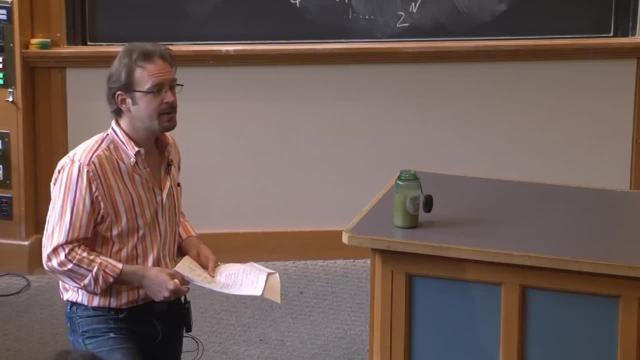 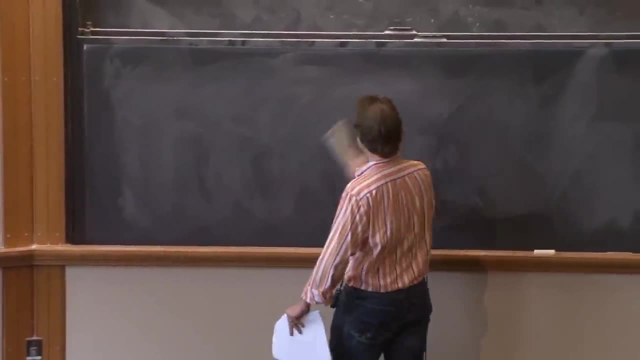 Because apparently it works right, Because we're here as was before he said. So this is the question of quantum computing. Can you use quantum mechanics? Can you use, in particular, the quantum evolution? Can you use the quantum evolution of a system? 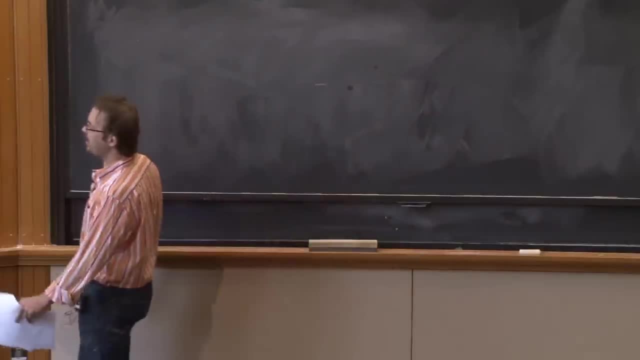 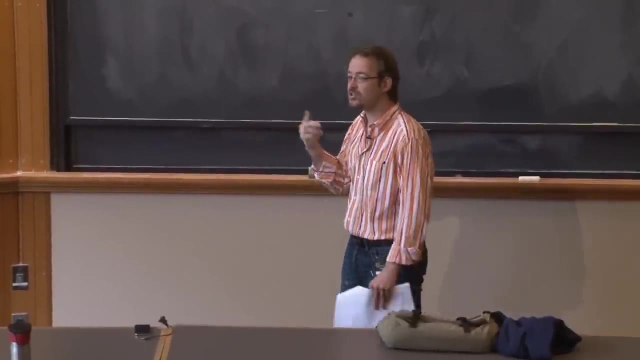 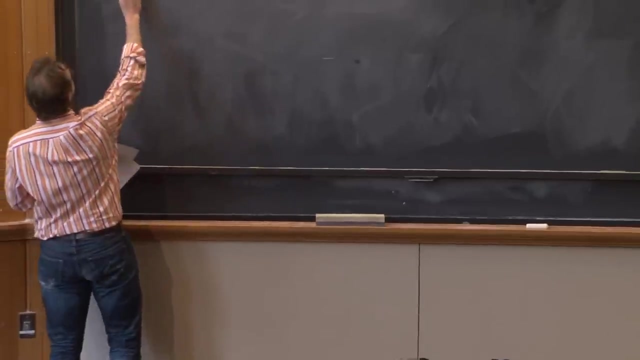 to perform calculations that you'd care about rather than classical computation, And if you do so, do you gain anything? Do you get any sort of speed ups? Is there an enhancement? Is anything better? So here's the basic gig. The basic gig is that we're going to take our system. 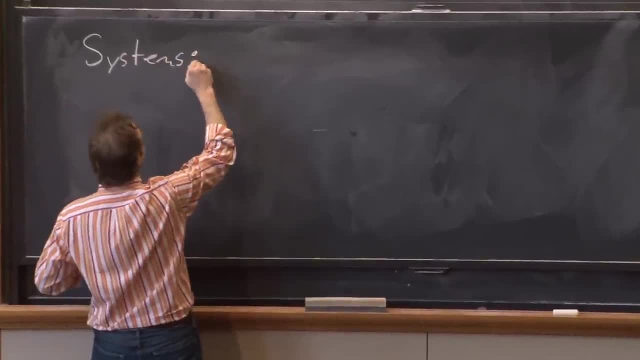 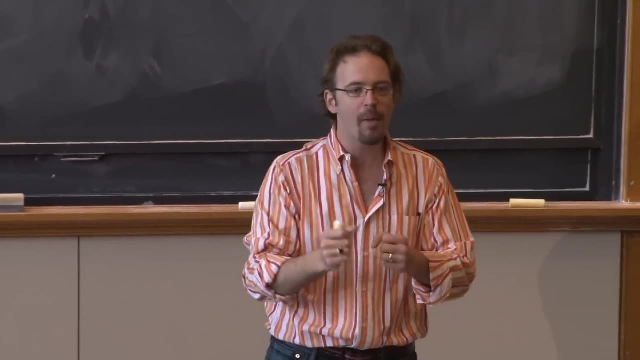 Consider the following kinds of quantum systems. Our systems are going to be n qubits or n spins, But because I want to emphasize that the substrate doesn't matter, The underlying material doesn't matter, I'm going to refer to them purely. 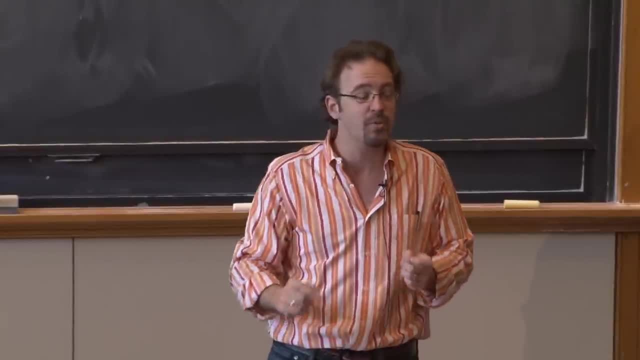 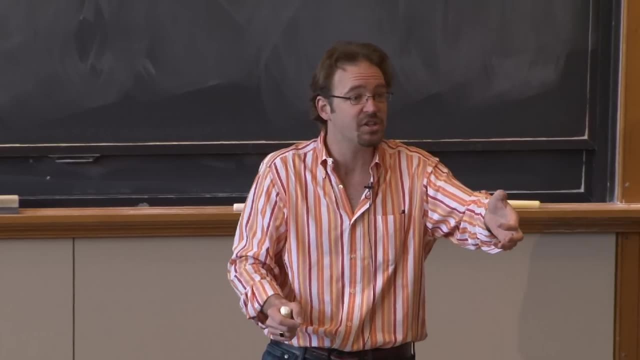 and this is totally typical in the field- as qubits rather than spin systems, And the reason is it might work to use little isolated spinning particles with intrinsic spin That might turn out to be technologically infeasible. It shouldn't matter at the end of the day. 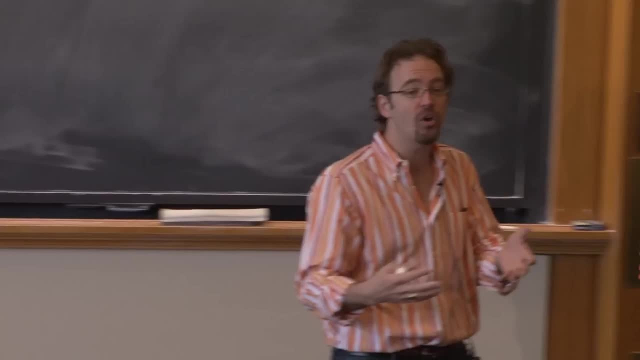 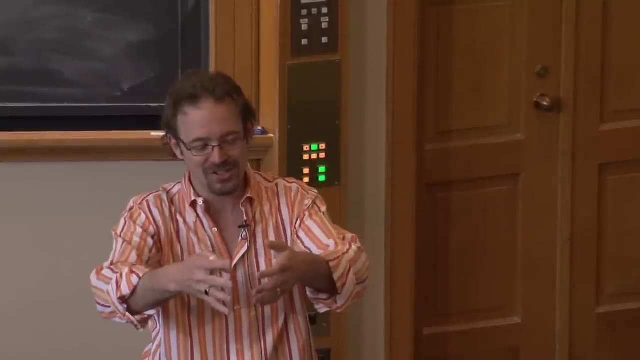 In the same way that if I ask you how does your computer work, Or if I ask you to write a code, you write some code in C or Python or whatever- with the hip kids are using these, So you write some little scheme code. 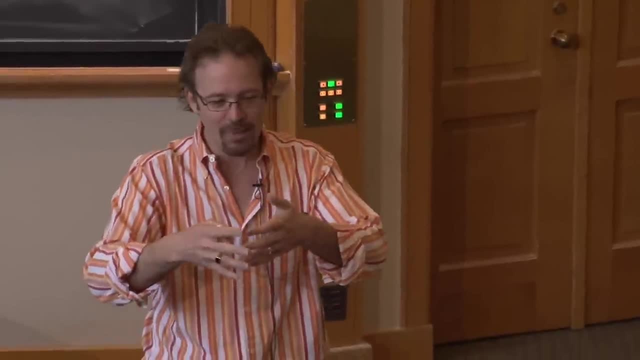 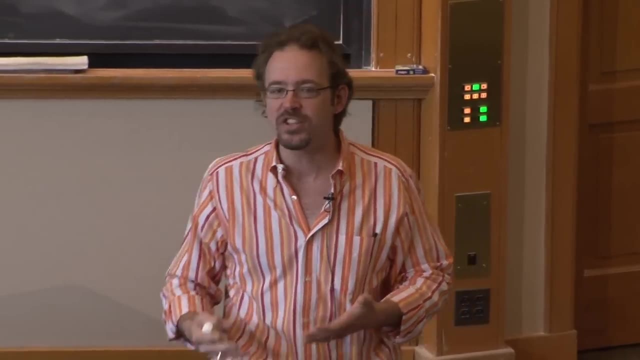 I still love scheme. You write some little scheme code and it performs some calculation. that's defined in just logic, in lambda calculus, in abstract logic. Do you need to know the substrate? Do you need to know whether your transistors are built out? 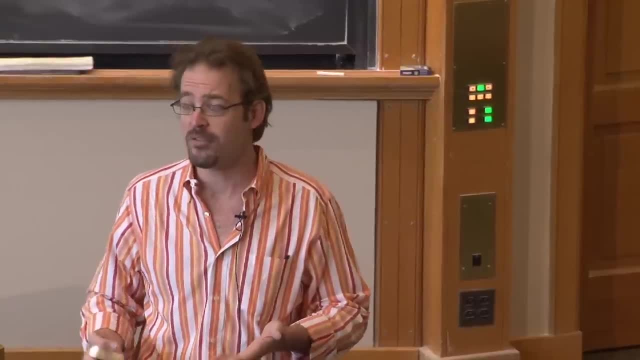 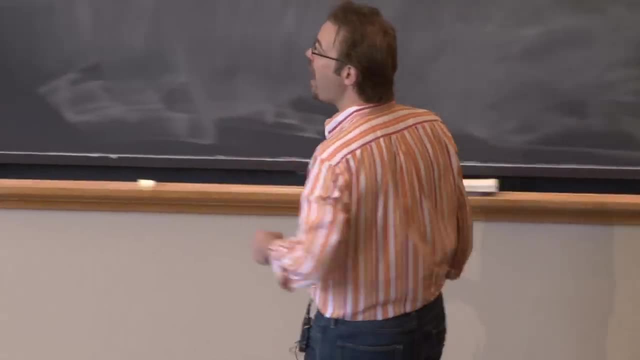 of silicon or germanium, or indeed whether it's running on vacuum tubes. No, that's the whole point of abstracting away computation, that the substrate doesn't matter, So we can use spin 1: half and that's going to be useful for us at various moments. 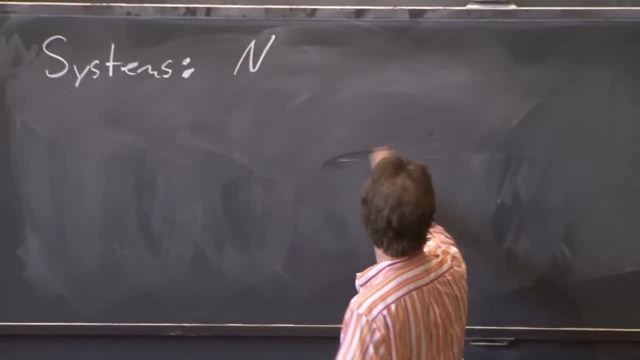 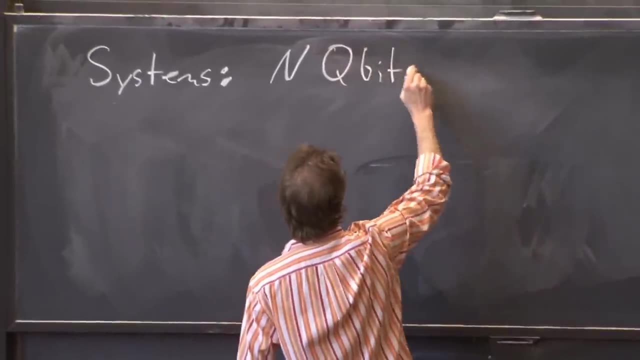 But I want to emphasize that the important thing is the actual logic of the process, not the underlying substrate. So here's what I need. My systems are going to be n copies or n qubits, where each bit is specified by either 1, represented by up. 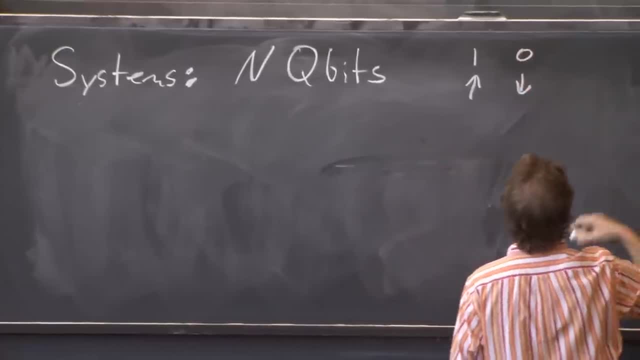 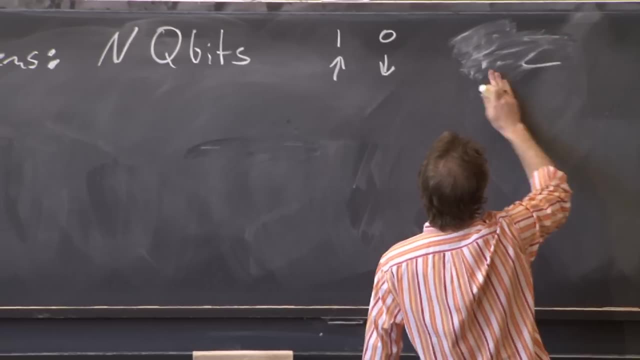 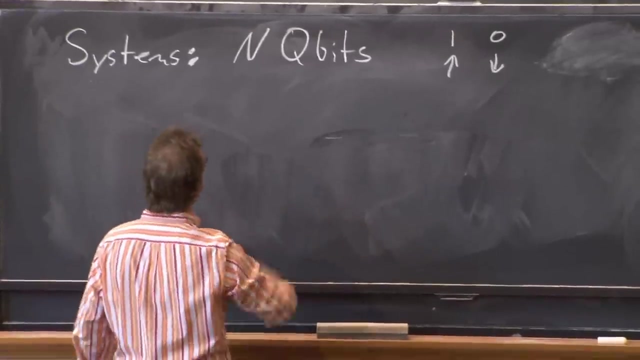 or 0, represented by down. I'll use these interchangeably So that the full system, psi, is a superposition of some overall possible. sorry, I won't even write that. So this is my system. It's going to evolve according to some energy operation. 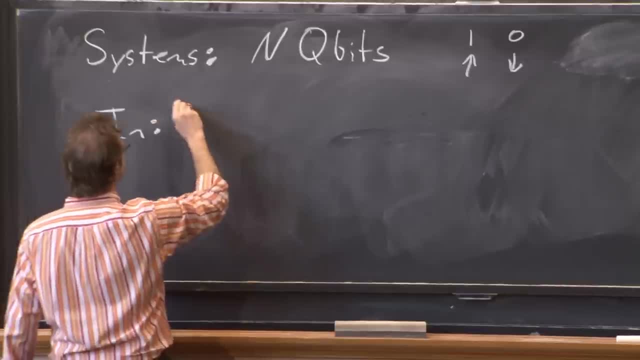 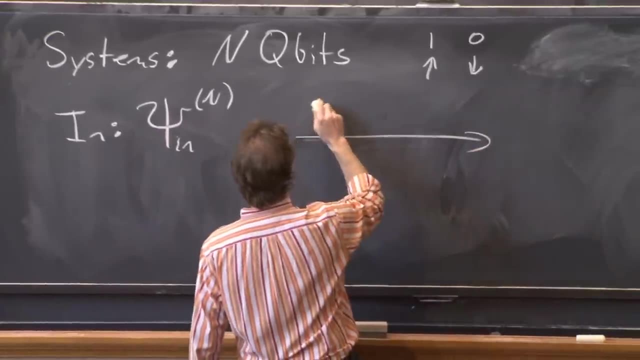 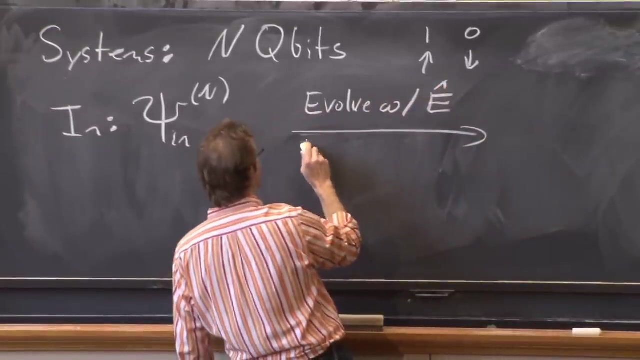 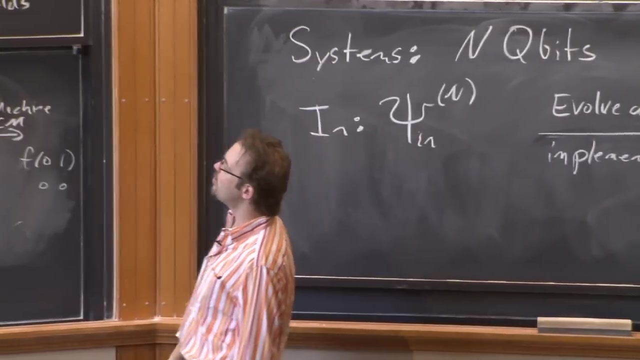 And so my input is going to be Some wave function, psi n for these n qubits. Computation is going to evolve with some energy operator which I've chosen to implement, an algorithm, in the same way that the precise series of magnetic fields. 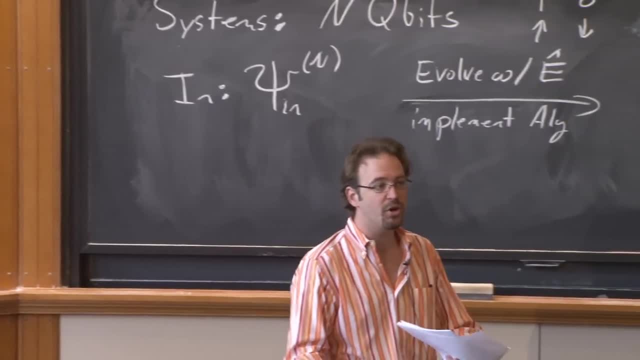 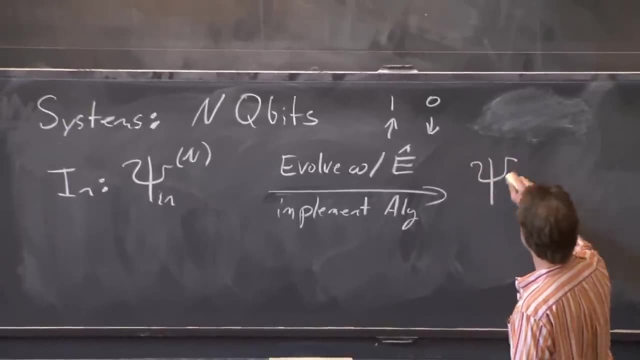 that we turn on in the classical computer, or currents that we allow to flow in a classical computer, implement the algorithm we want to effect. We evolve with some energy operator implementing our algorithm. We get some output, wave function, psi again. 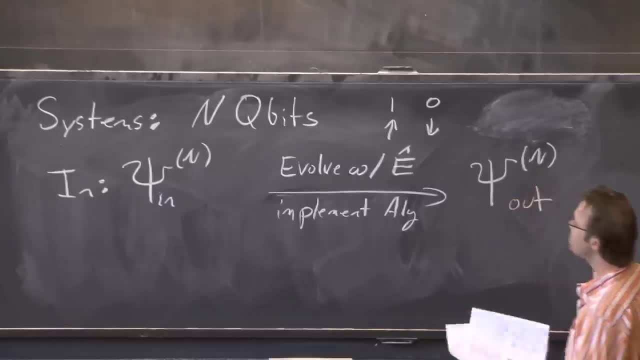 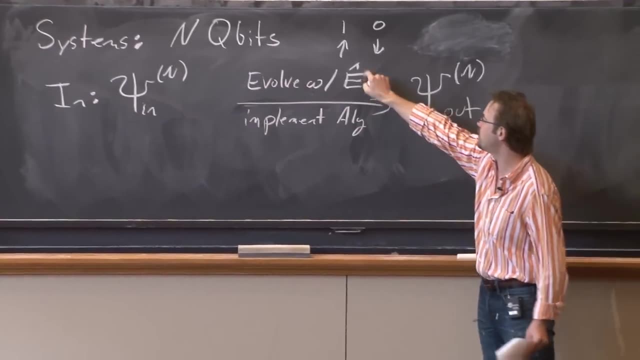 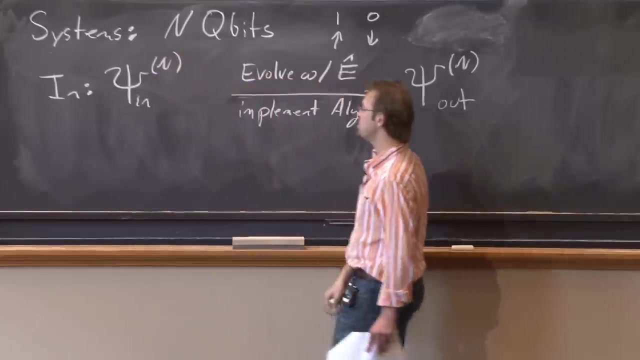 for our n bits and quantum bits out. So this is a basic gig with a quantum computation. We're just replacing strings of binary numbers and functions- evolution according to classical mechanics in Maxwell- to other strings of numbers with superpositions of states, superpositions of strings, as it were. 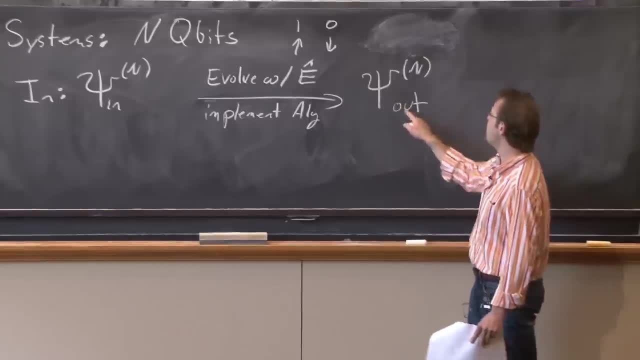 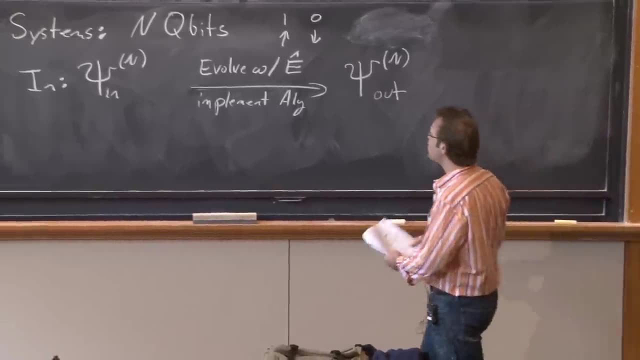 evolving according to the Schrodinger equation into again general superpositions. So how does this differ? What are the key differences from classical computer? So the key things are, first off, the input and output are not definite values. They could in general be superpositions. 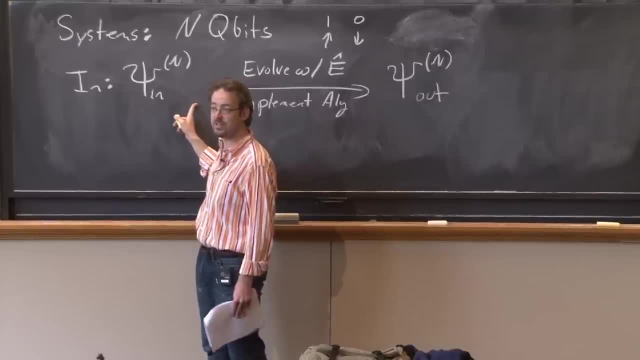 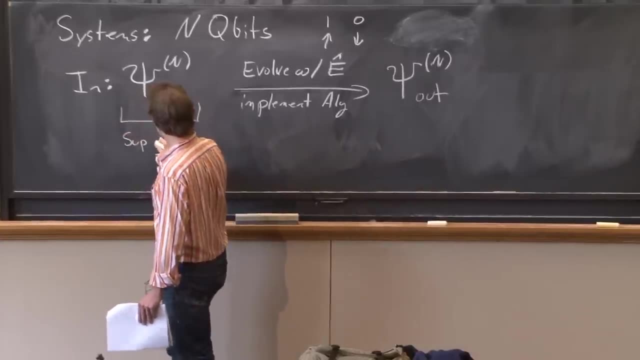 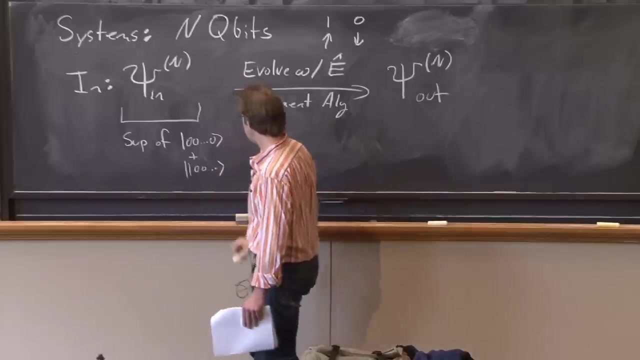 They do not have to correspond to a definite state in the 1, 0 basis. These in general are superpositions of 0, 0, 0, 1, 0, 0.. So the input and output are: 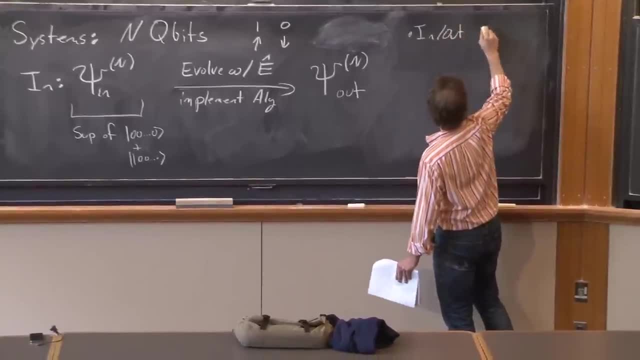 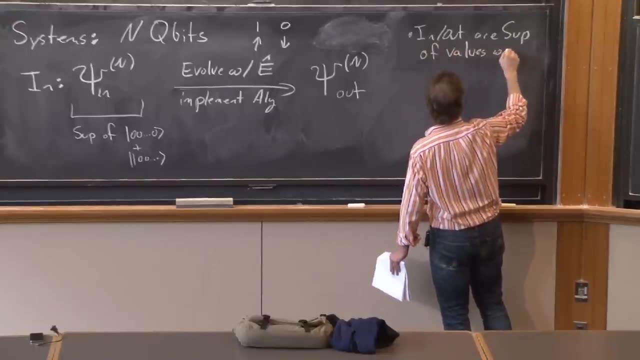 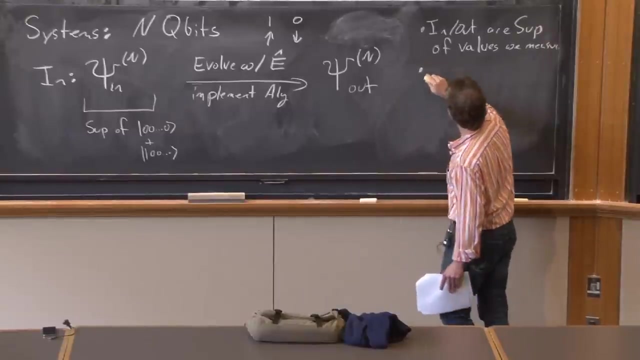 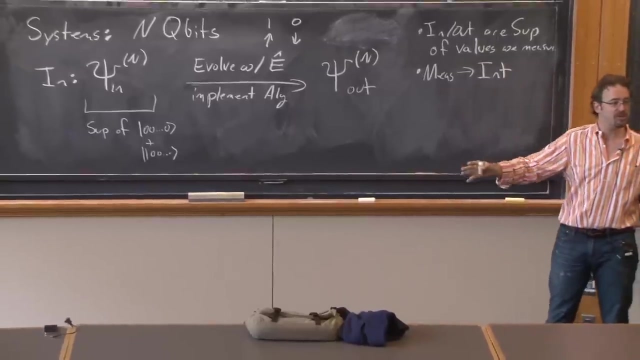 Superpositions are superpositions of the values we'll measure. Second, when we do measure, at the end of the day, the output, we get interference from the various different terms in the superposition. The different terms in the superposition will lead to interference effects. 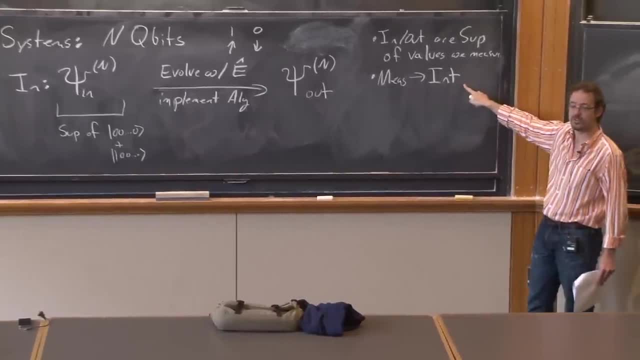 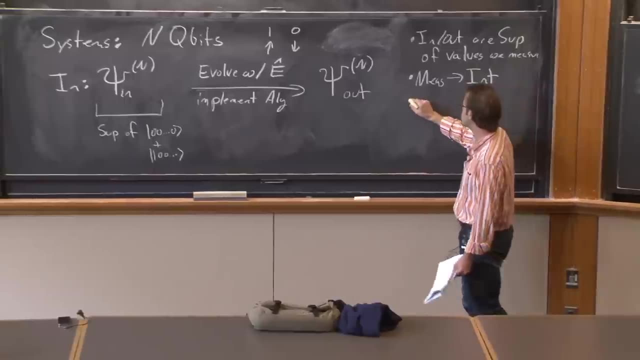 And so our output will be sensitive to that interference between the different terms. It may be that we're in some pure state, but it may be, more generally, we'll be in some superposition of the states we want to measure. So we're going to get interference. 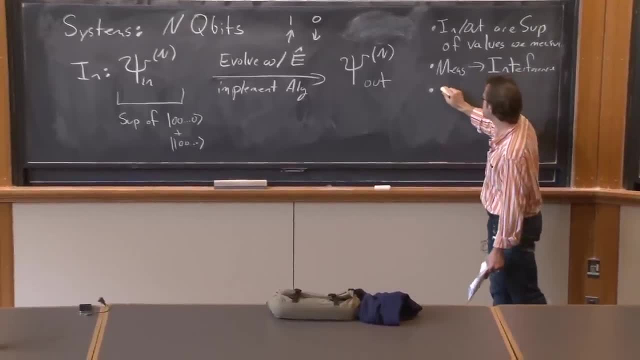 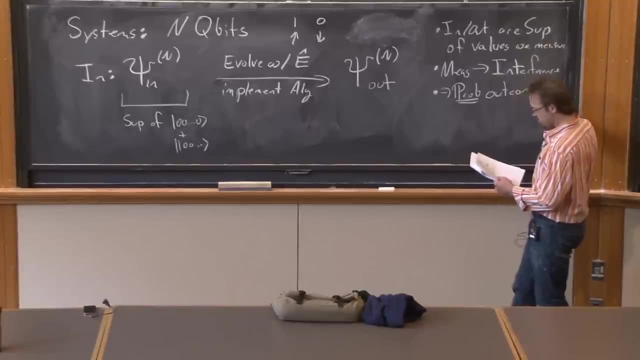 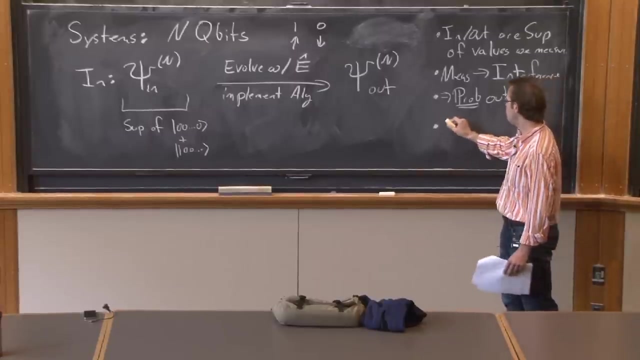 So, naively, this is a disaster because this means we get probabilistic outcomes. That sounds bad. And so this leads to the key difference in quantum or the key move in quantum computation. given that we're going to have interference and given that those interference effects are, 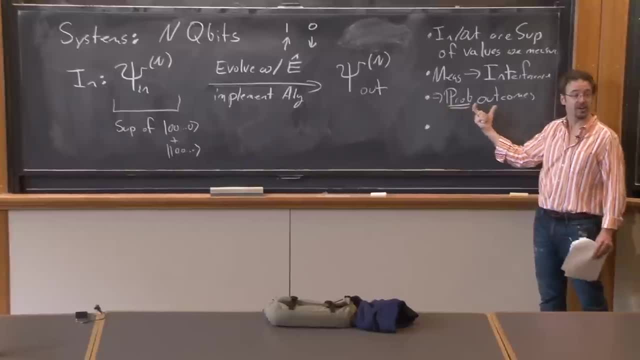 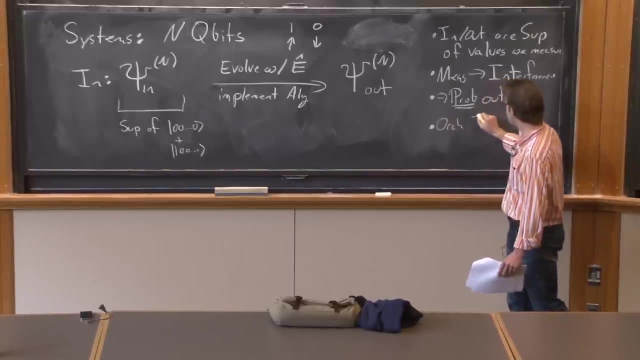 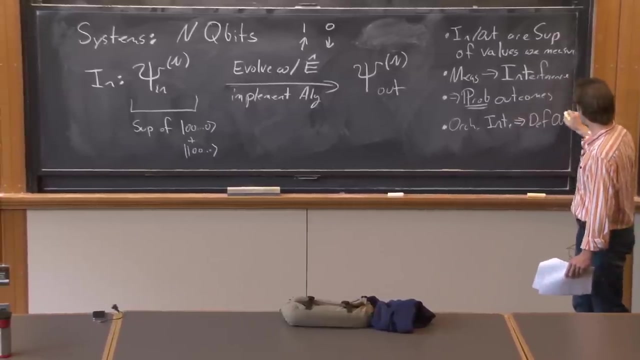 going to affect the probabilities of various outcomes. what we're going to want is to tune or orchestrate the interference to get a definite outcome. We want to get the correct answer out rather than just probably the correct answer out. Now there's a slight variation of this. 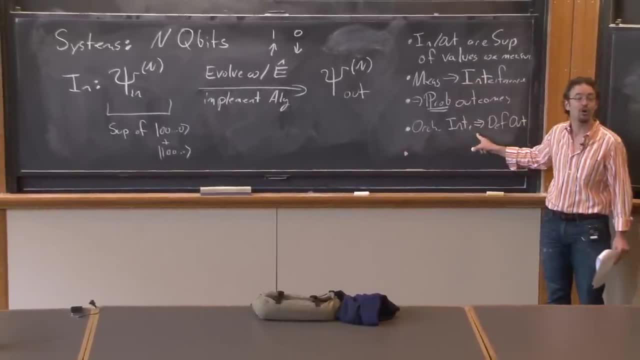 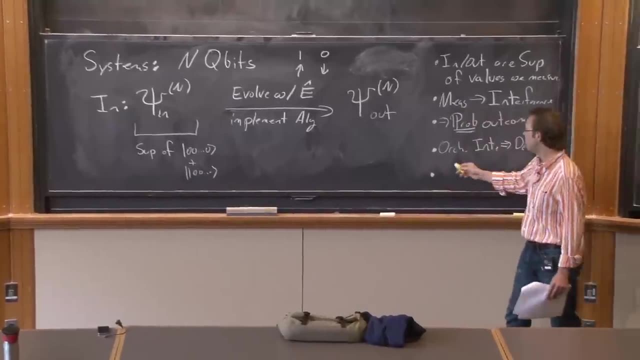 It's not obvious at the beginning how to do that. It's not even clear that you can. So I'm going to show you that you can. I'm going to show you an explicit algorithm that realizes this, But that's obviously going to be tricky. 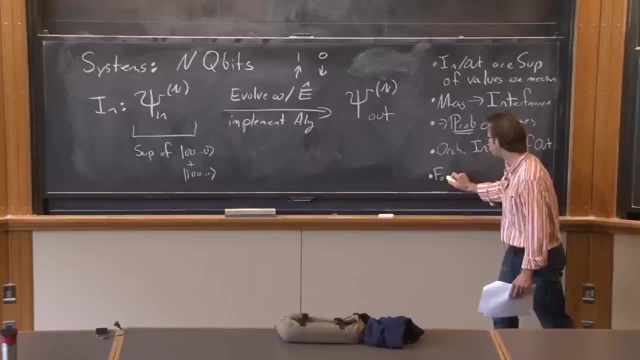 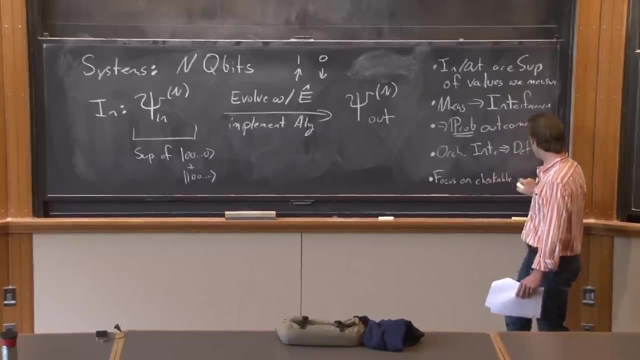 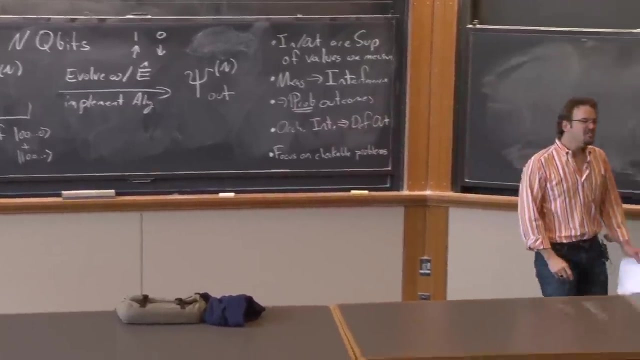 Here's something else you can do. You can also focus on special problems, focus on checkable problems, And what I mean by this. imagine we have some algorithm that gives us an output and that output is probably the right answer, But we're not sure. 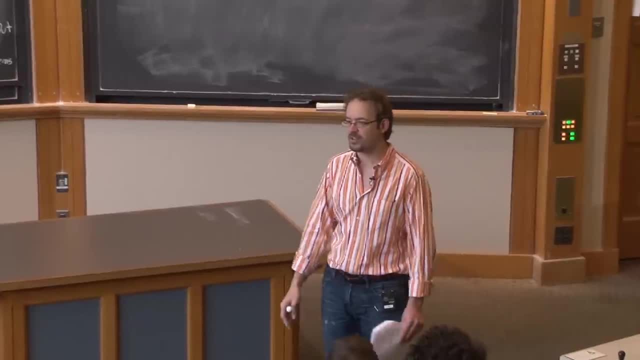 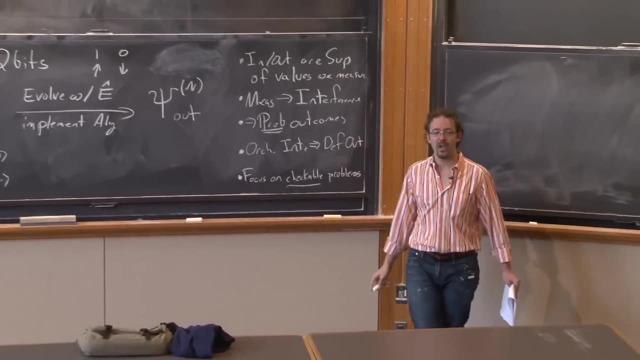 There's some quantum mechanical probability that this is the correct answer to our computation. There's some probability that it's not So. if the calculation was difficult but it's easy to check whether you have the right answer, then that's great. Imagine it's 10%, you get the right answer. 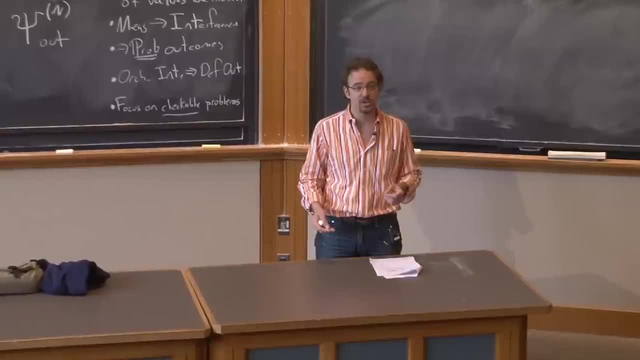 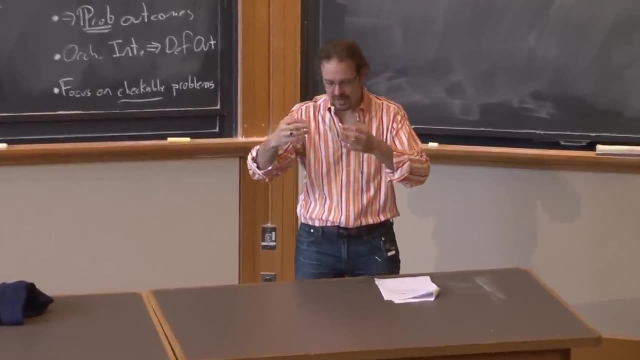 but it's trivial to check. So, for example, factoring numbers: If you multiply the numbers, that's easy. You can check to see whether you got the right thing. So for example, imagine I build a computer that is supposed to factor numbers. 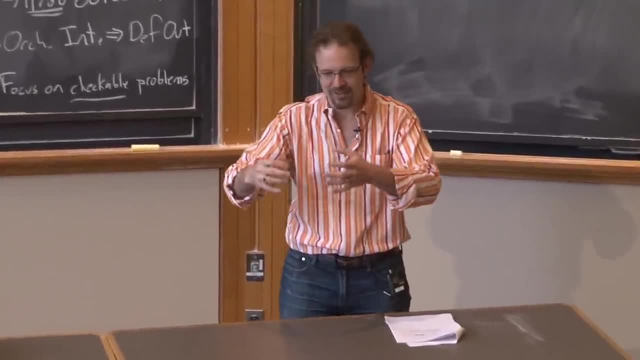 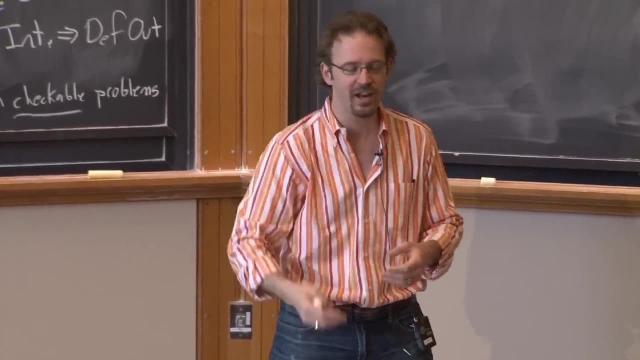 I almost said factor prime numbers. That would be boring. So imagine it: I build a machine that factors numbers, And so imagine its output is probabilistic. So you say 15, and I say 3 times 5.. You say 15,, I say 5 times 3.. 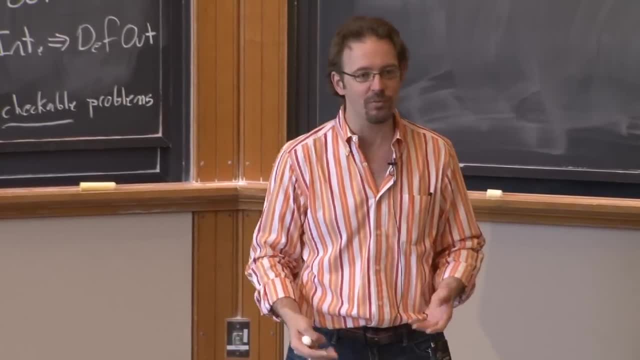 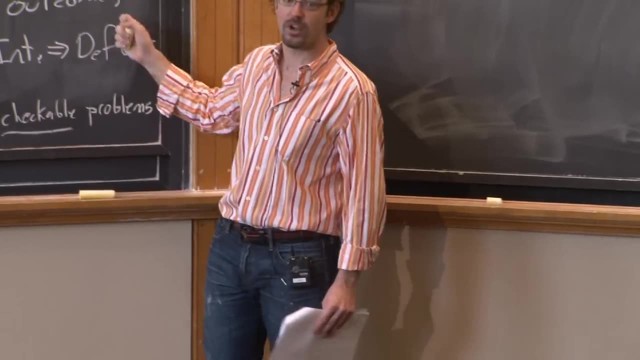 You say 15, I say 7 times 2. At that point you're like: well, which one is right? Well, you can check by multiplying. So if you have a problem which is easy to check but hard to do, then probabilistic is already OK. 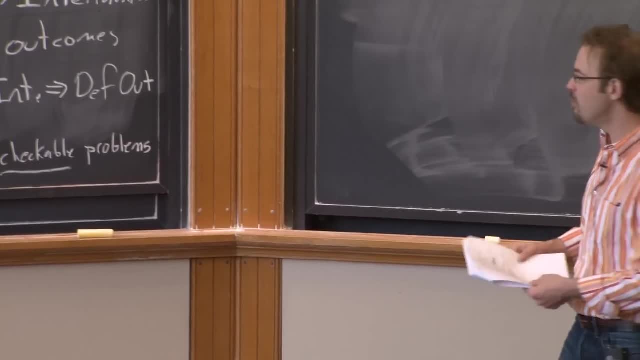 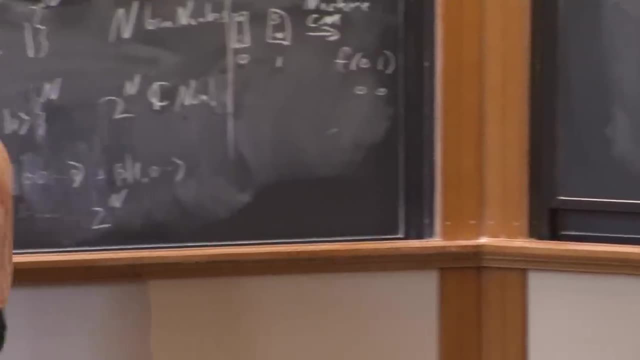 And that's just as true classically as it is quantum mechanically. Those are basic moves, And so the key thing for us is that when we have n quantum bits, we have these interference effects And, in particular, as discussed as we started talking about. 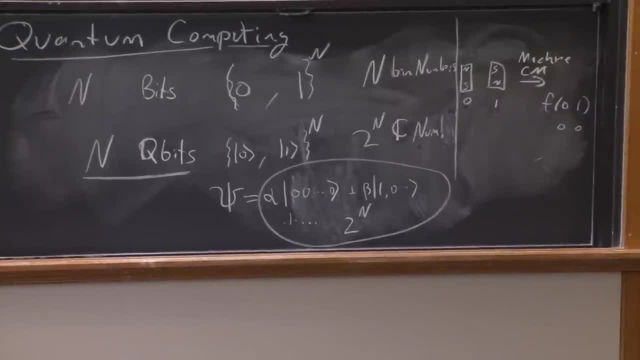 last time we get entanglement effects And what we're going to discover is that the key to making a good quantum algorithm is going to be to attune the entanglement appropriately. So I'm going to have to define that for you in just a minute. 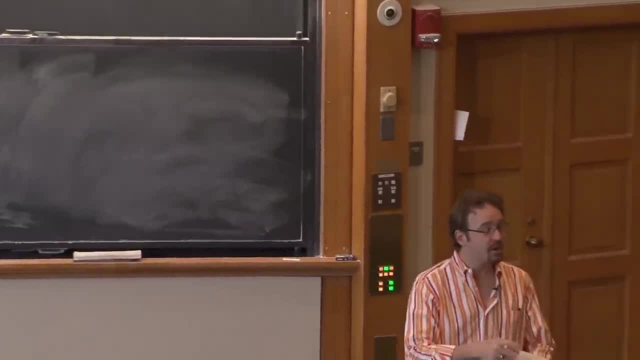 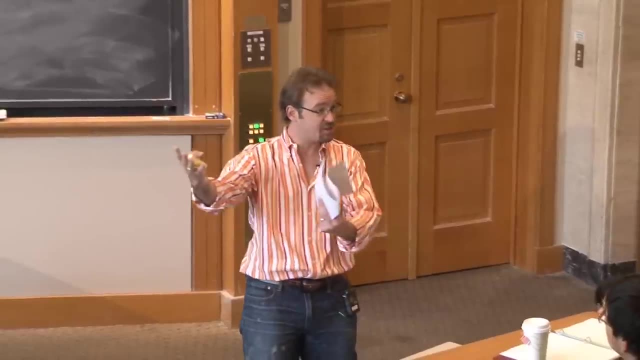 Yeah, But what about the fact that the checking is also probabilistic? Sorry, The checking process is also probabilistic, right? It may or may not be. So the check, for example, could be like. for example, imagine the process I just gave you. 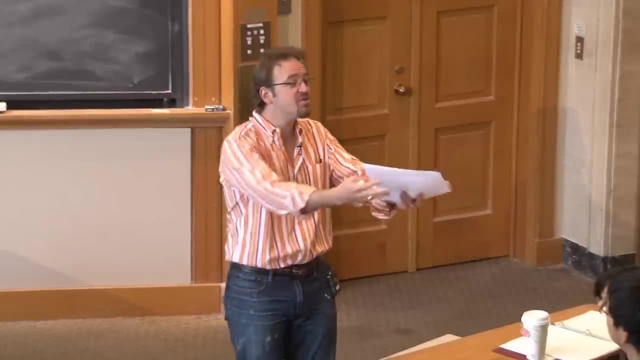 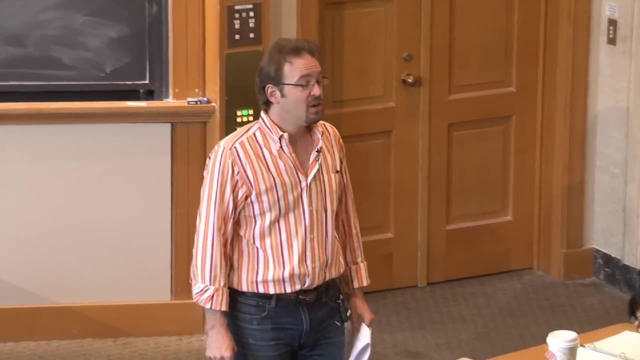 So the question is: what do you do if the checking process is probabilistic? But you can use a classical computer to check if you have an easy checking algorithm, For example multiplying numbers together. So it doesn't meet the point of using a classical computer. 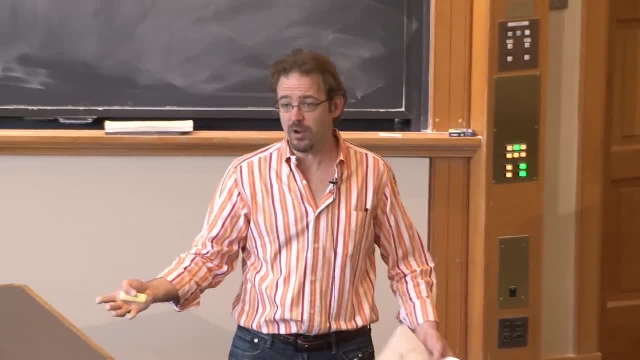 No, because good. And so the question then becomes: it doesn't have to be the point of using a quantum computer if you're using a classical computer to check. And so here's the thing: If I ask you to factor a gigantic number, 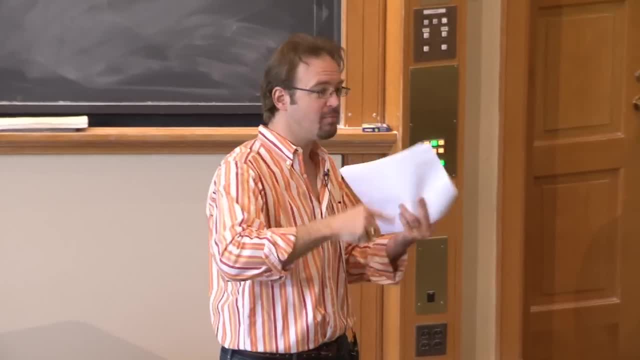 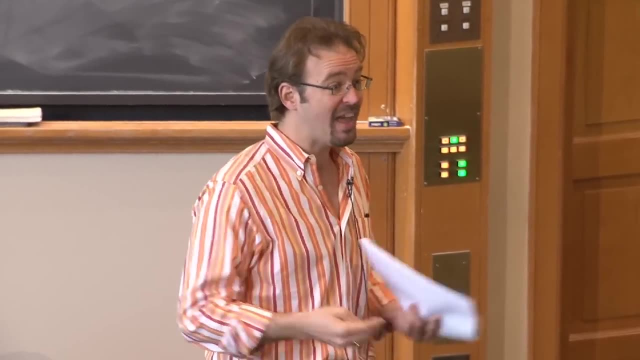 what do you have to do? Well, you have to take all numbers up to its square root And you have to multiply them together. And that takes forever, right? But if I tell you, do these two numbers, multiply to give you a third number. 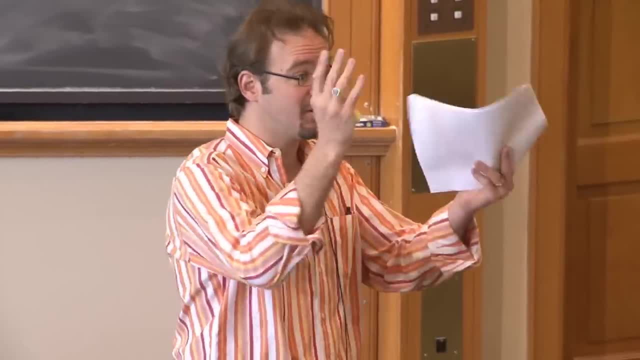 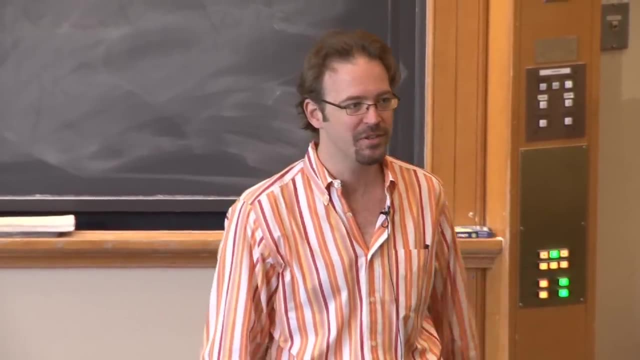 That's easy, right. So I use the quantum computer for the hard part And the classical computer for the forward part, for the checking, And that's a special class of problems which are checkable. These all have fancy names in information theory. 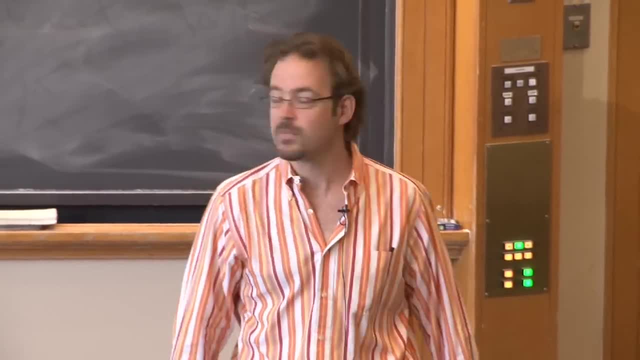 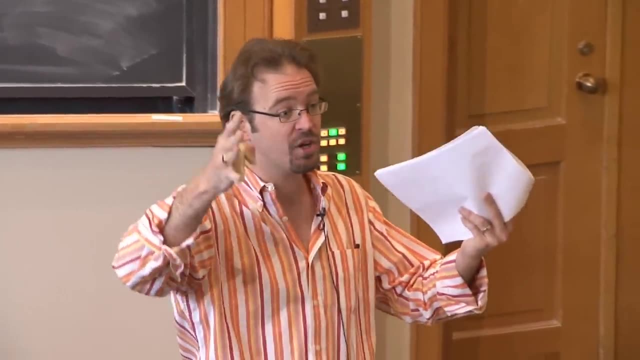 I'm not going to use the fancy names. Yeah, By using theories do you mean the relaxation of the wave function? Yeah, exactly, I mean that when we compute, suppose I give you some output, And let's say the output is 0, 0 plus 1, 1.. 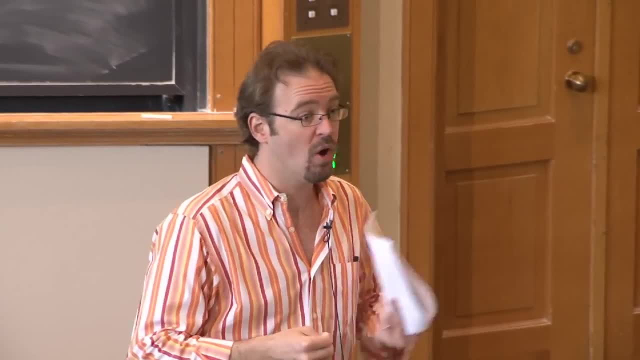 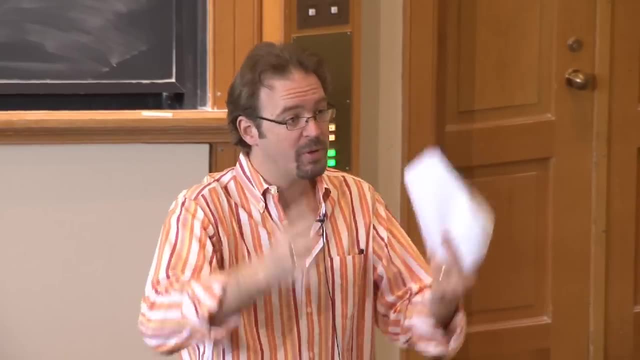 What are you going to get if you measure the first bit? Well, you're either going to get 0 or 1, with one probability or another. When we compute the probabilities in general, when we have many terms in our superposition, 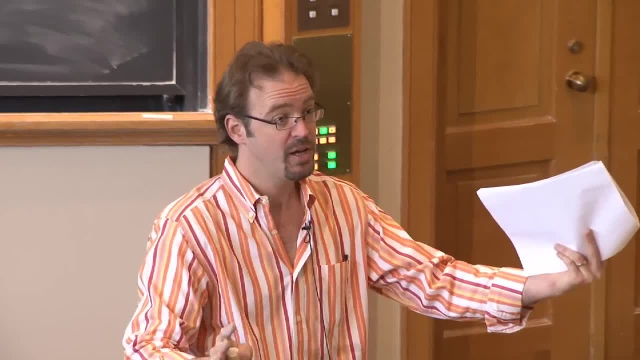 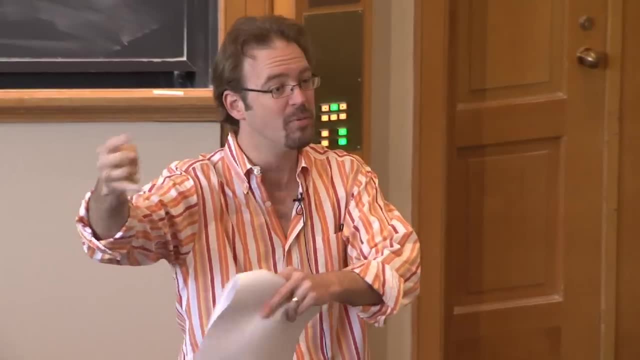 we're going to get interference effects from different terms in the superposition And those interference terms will tune the probability, so that not just the naive probability of that one thing, but that you get these quantum interference terms, The norm squared of 1, norm squared of 2,. 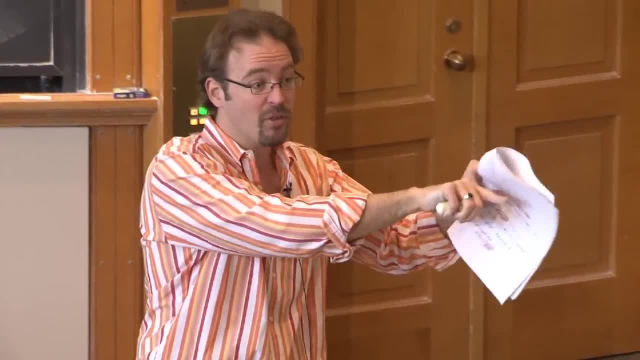 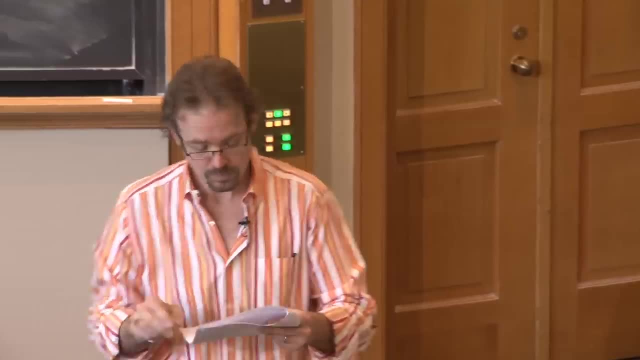 and then the real part, twice the real part of the cross term. And that twice the real part of the cross term didn't exist classically, But quantum mechanically it's important And it can change the final probability. That's what I mean by the interference effects. 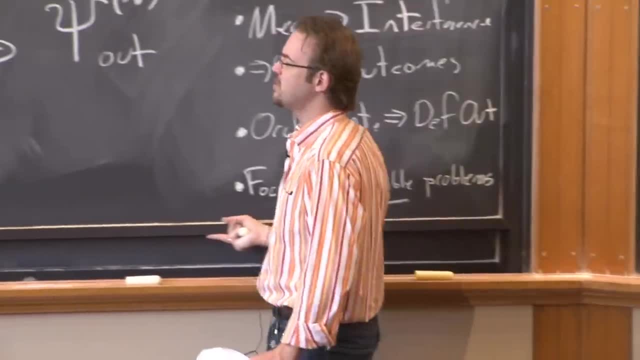 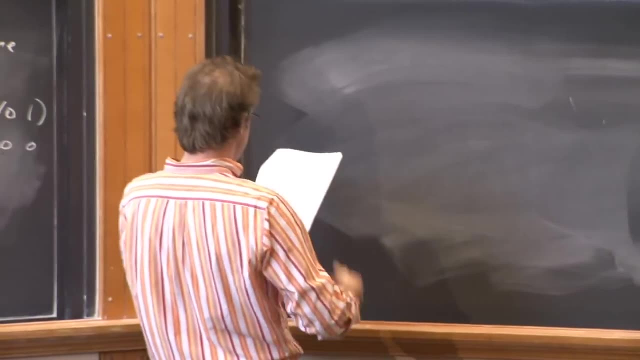 OK. So let's make all this much more explicit. So so far I'm just giving you philosophy, And you should be deeply suspicious of philosophy in a physics classroom. So again to be explicit, a quantum bit or qubit. 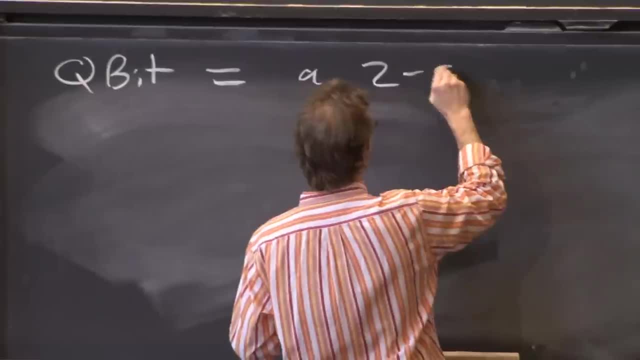 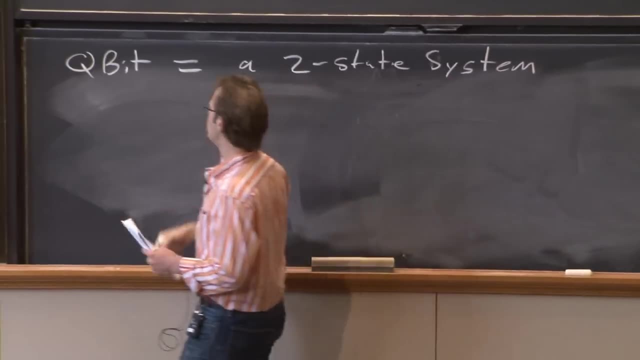 is equal to a two-state system, And again the substrate doesn't matter. I could be talking about spin 1 half systems, Or I could be talking about ropes on a cylinder with winding mod 2. I could be talking about all sorts of things. 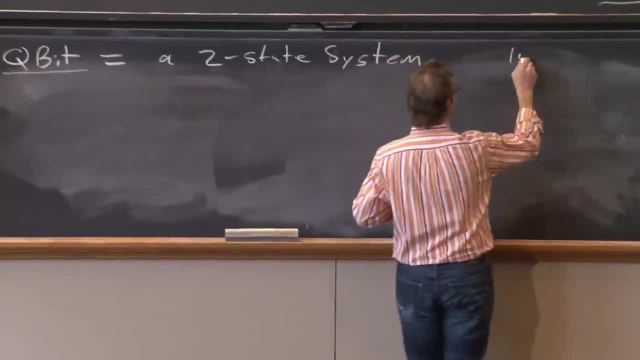 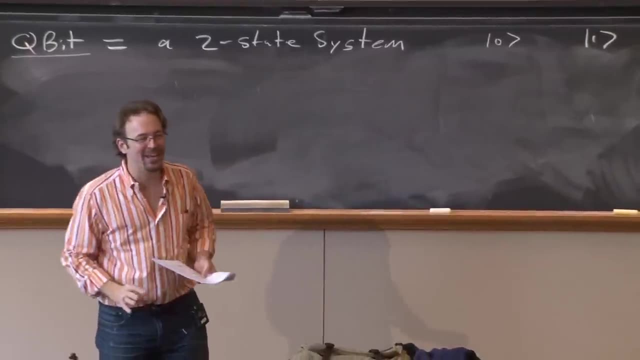 But it's some system with two quantum states, 0 and 1.. I want to emphasize: this is not going to be on the final, So this is for your moral well-being, OK. So a quantum bit is a two-state system. 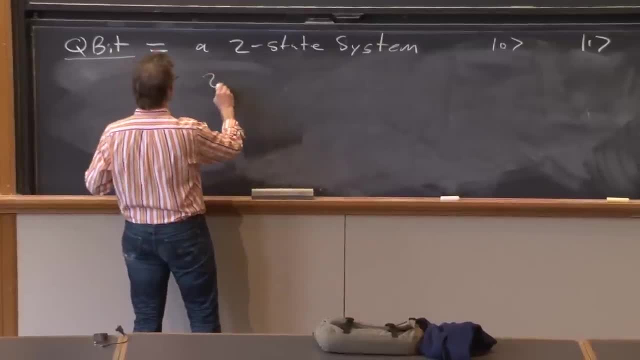 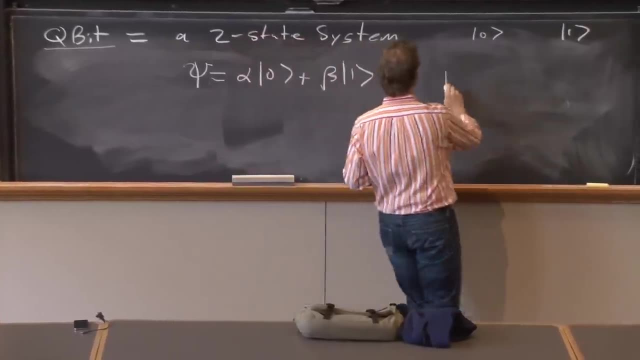 We have these two states, which I'll call 0 and 1.. And a general state. a general wave function is: psi is equal to alpha 0 plus beta 1.. OK, And the probability? what this means is the probability that I measure, 0.. 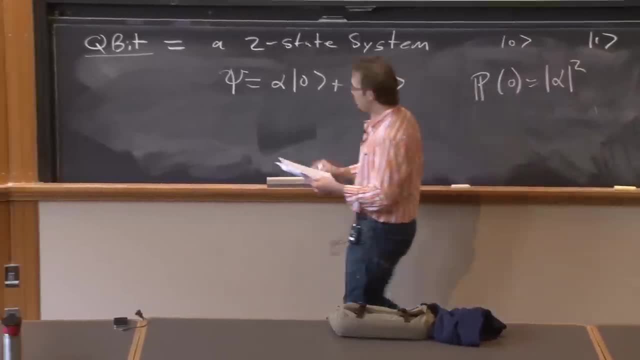 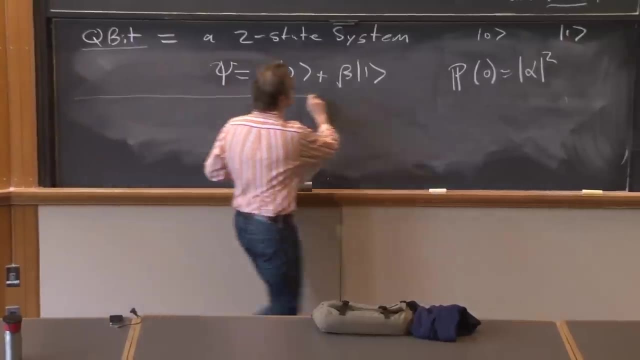 It's equal to norm, alpha squared, et cetera. Now again, many systems can be used, many different substrates. This is what I'm going to mean by a qubit. So that's one qubit. The much more interesting system is two qubits. 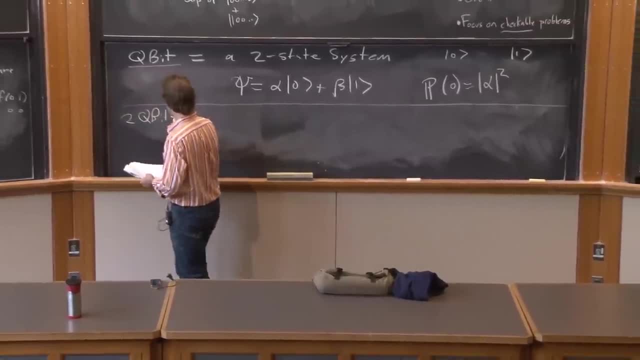 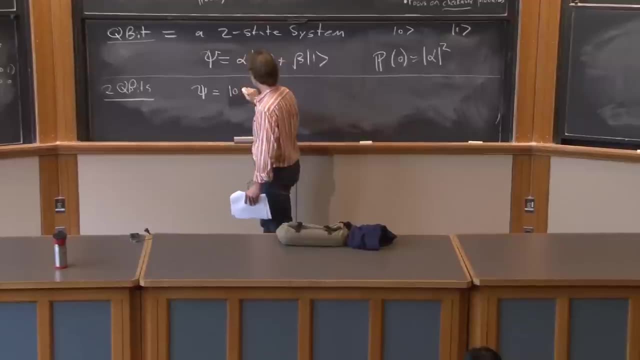 So let's study two qubits. So, in the case of two qubits, what's a general state? Well, a general state is going to be. well, the first particle could be 0, and the second particle could also be 0.. 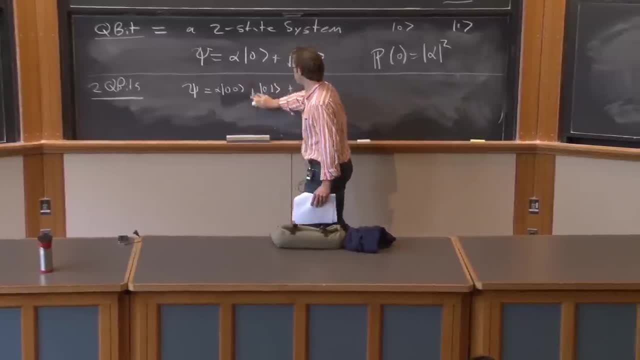 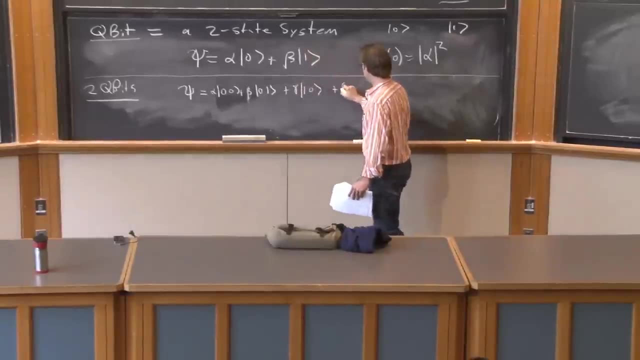 Or we could have the first particle 0 and the second particle 1.. With some coefficient, plus beta, plus gamma 1, 0,, plus delta 0, 1.. OK, So this is just a general superstition. Now you might worry at this point. look, 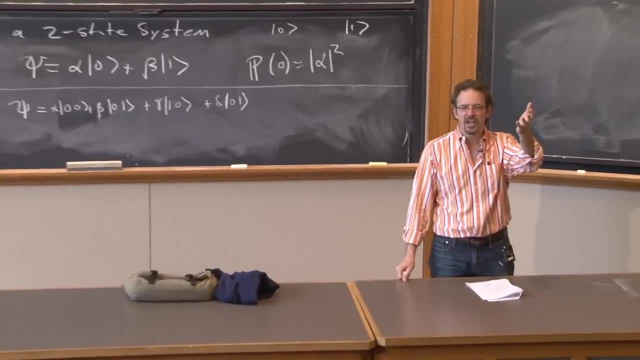 are these identical or are these non-identical spins? But here's the thing: I've got a spin here, It's in a box. I've got another spin here, It's in a box. I've got another qubit over here. 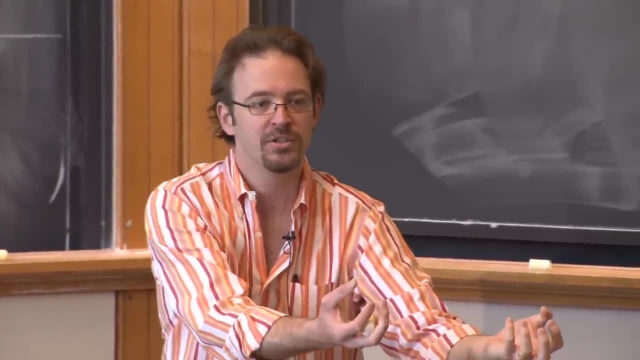 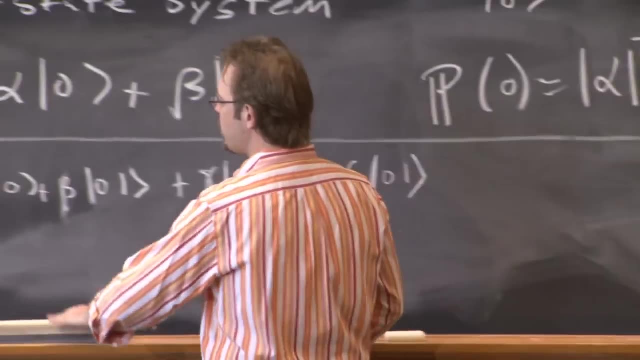 It's in a box, So they're distinguishable because they're in different places in my laboratory. So these are distinguishable particles, The particle in this box. The box is either up or down, OK, So these are distinguishable. I don't have to worry about symmetrization. 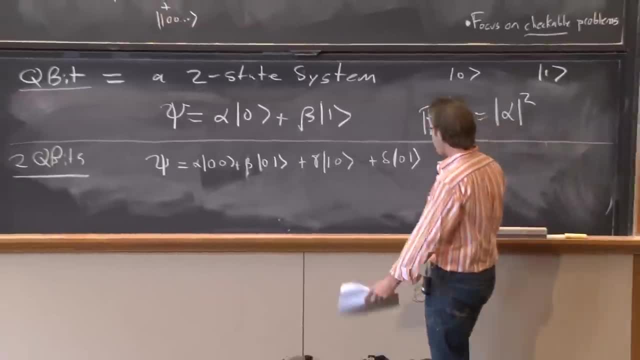 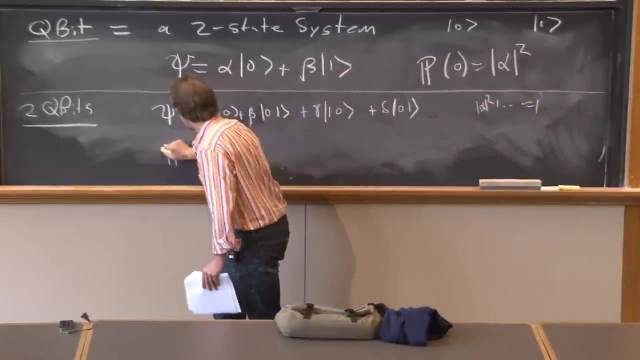 bosonic or fermionic statistics or any of that. They're distinguishable And we need normalization. So norm alpha squared plus dot dot, dot is equal to 1.. And what does this mean? Well, what this means is that, for example, 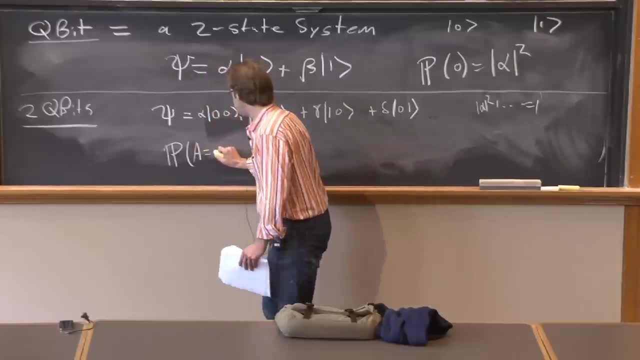 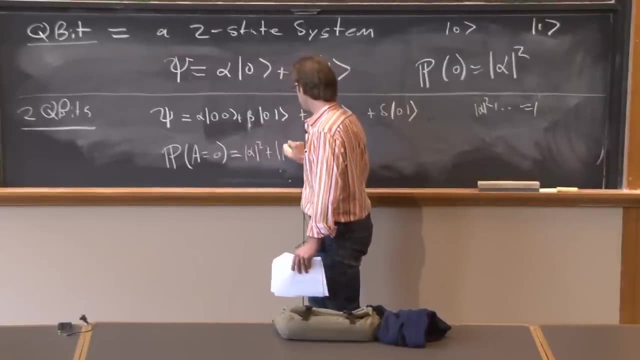 the probability that the first particle, which I'll call A, is equal to 0 is equal to well, some of all the possible ways we could do that. We have norm alpha squared plus norm beta squared. But these guys are whoops. 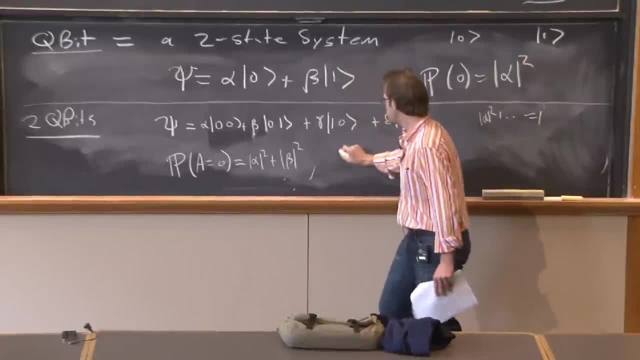 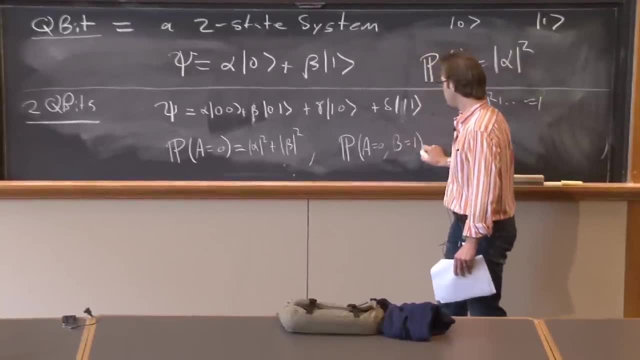 This was 1, 1.. Thank you. And if we're more specific, the probability that the first qubit is 0 and the second qubit is 1 is equal to well, I need 0, 1.. That's, this guy is norm beta squared. 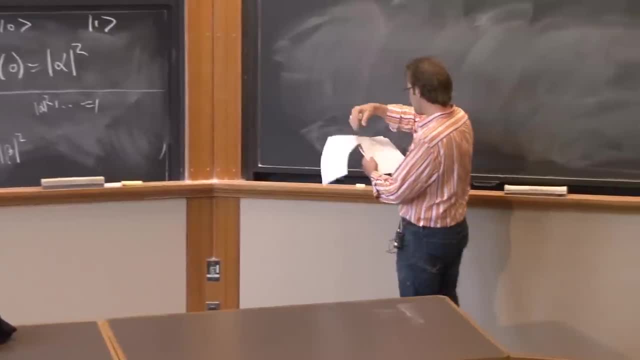 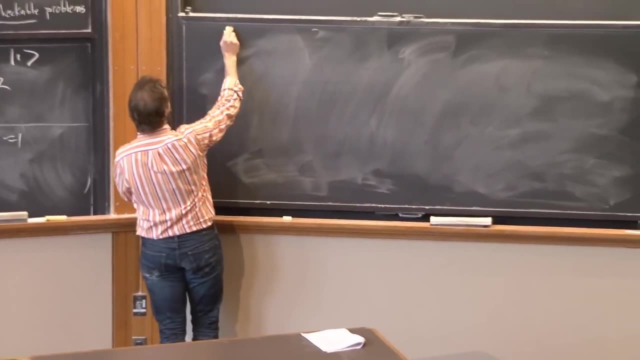 OK, What do I mean by two qubits? But this immediately leads to a funny thing. There are two kinds of states that a pair of qubits could be in: A very special set of states which are called separable states, And these are special. 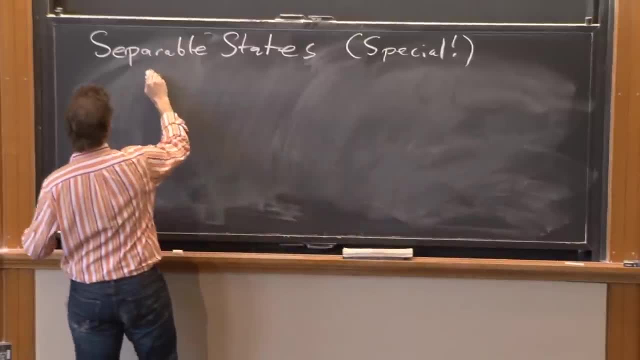 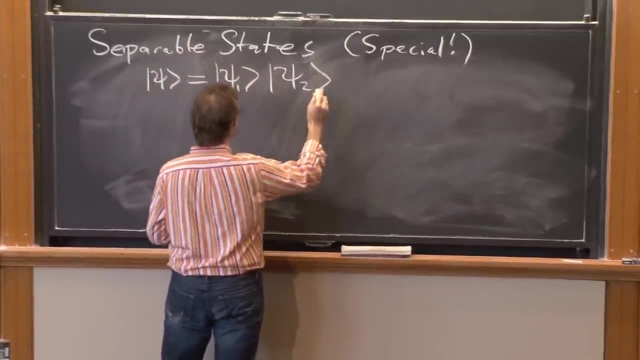 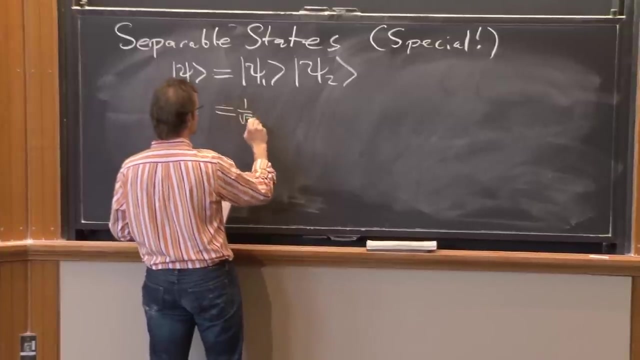 And these states corresponds to the full system being in the state, where the first particle is in one state and the second particle is in the second state. OK, So for example, this could be: eg the state 1 over root 2. 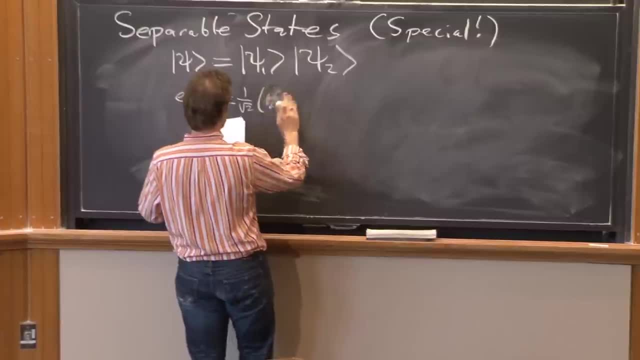 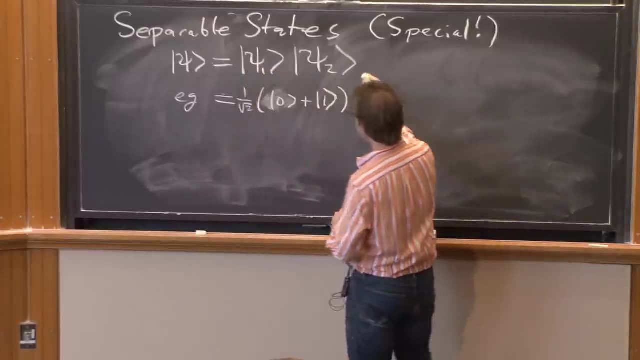 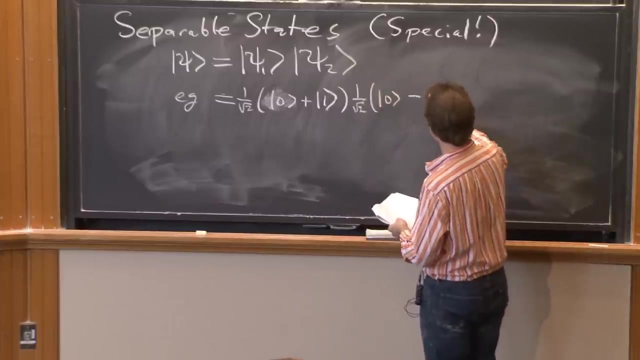 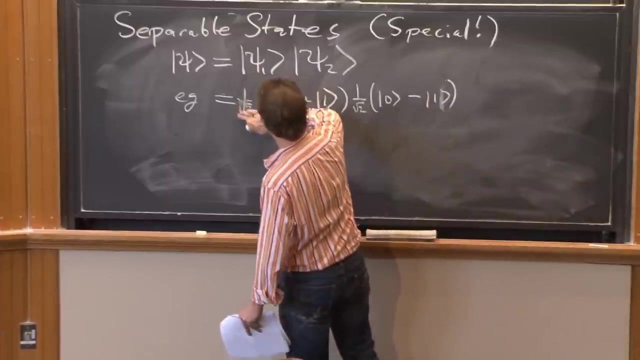 up plus sorry, yeah, 0 plus 1 for the first particle And the second particle would be in the state 1 over root, 2, 0 minus 1.. Oops, Is that the example I wanted to make? Oh, let's just call these general coefficients. 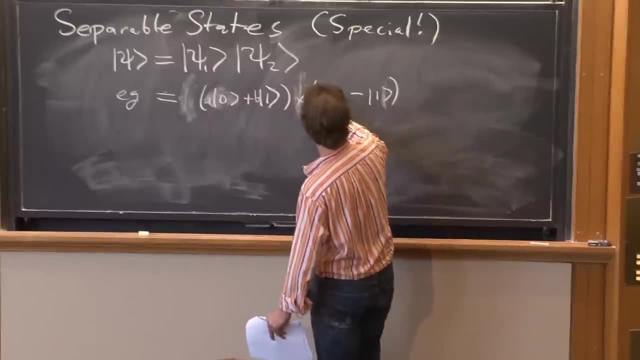 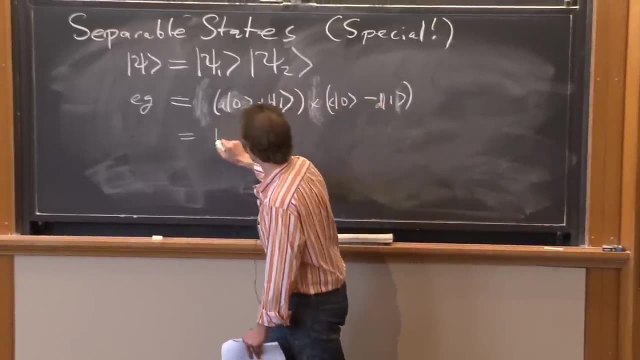 a plus b and times c plus d. OK, So what is this equal to? Well, this is of the form. Well, there's going to be a term that's 0, 0. And that's ac plus a term that's 0, 1.. 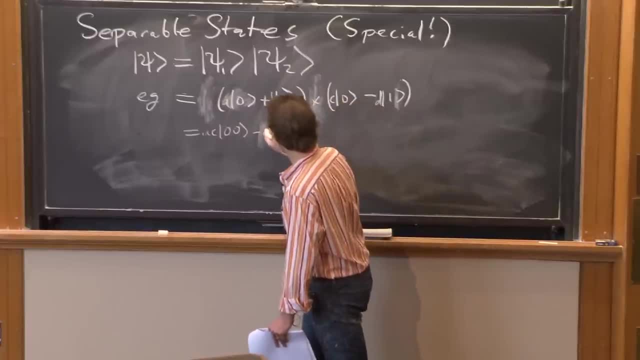 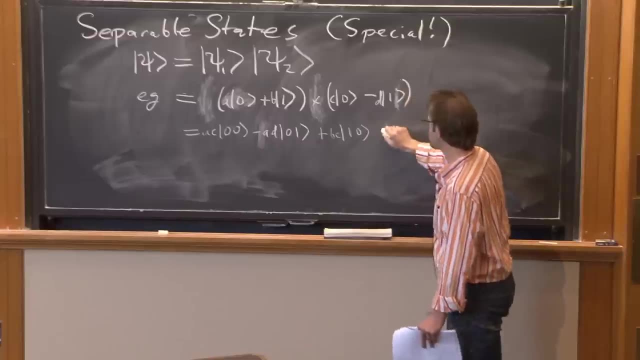 And that's ad with a minus, Minus ad plus a term, that's 1, 0.. And that's bc plus a term, oops, minus a term, that's 1, 1.. And that's bd, OK. 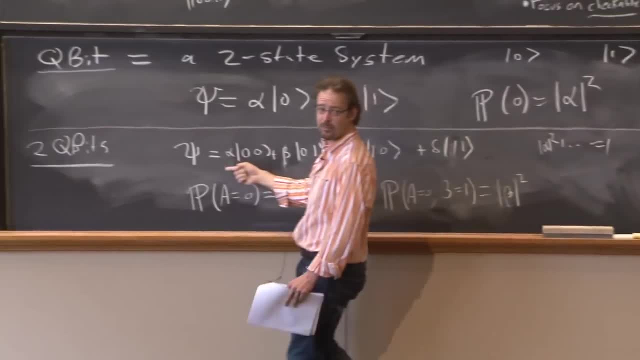 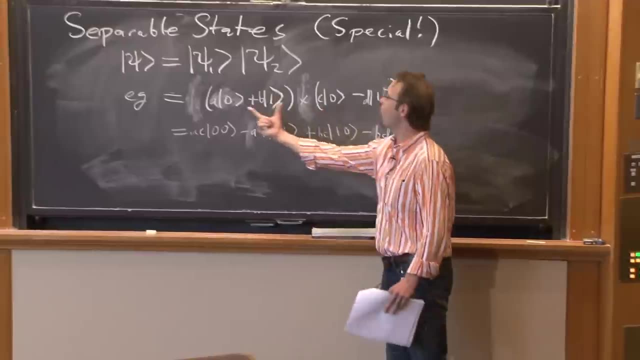 And this is clearly not generic because it implies relationships amongst the alpha, beta, delta and gamma, apart from just normalizability. Everyone see that. So it's a pretty non-trivial thing that you can write a thing as the first particle is in one state. 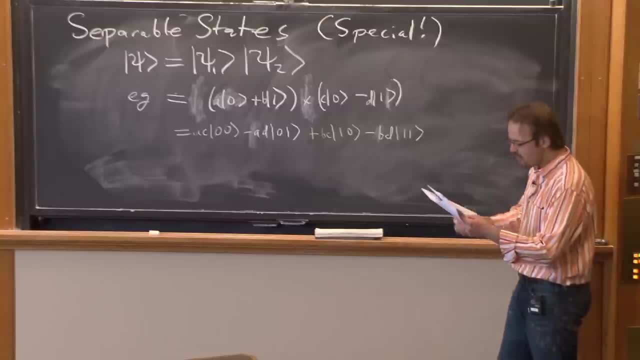 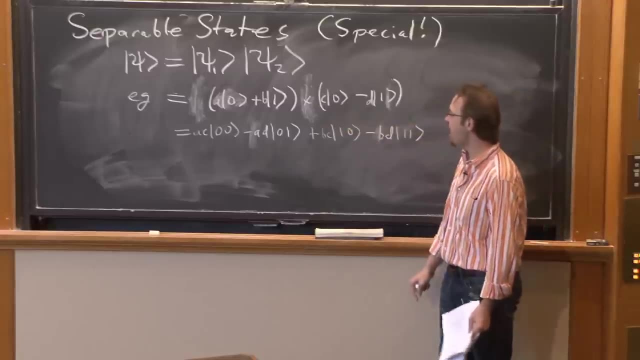 and the second particle is in the second state. And here's physically what that means. Physically, what that means is that if you're in a state like this and I ask you, what's the probability that I measure the first particle to be 0,? 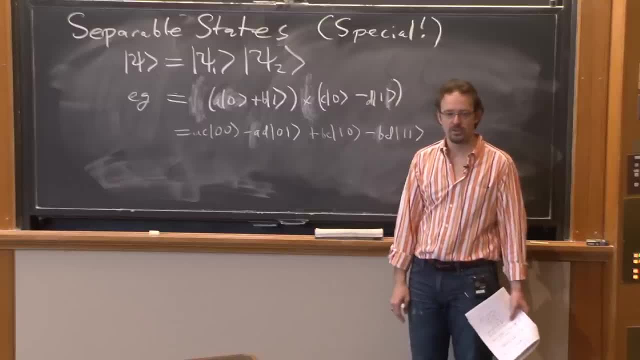 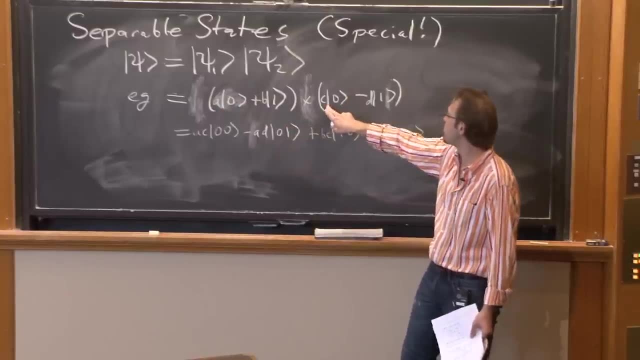 do I need to know anything about the state of b? No, The relative. if I want to know what the probability is, the first particle is 0, I just take norm a squared, Because I'm going to get plus norm c squared plus norm d squared. 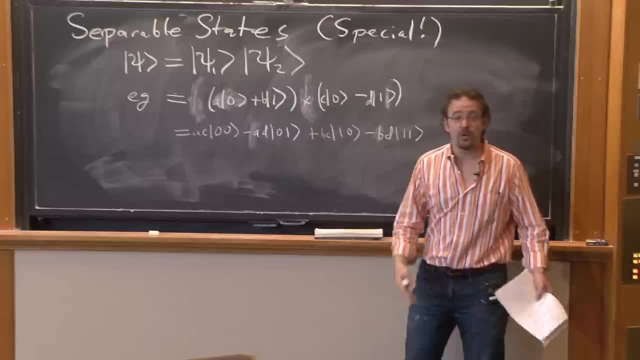 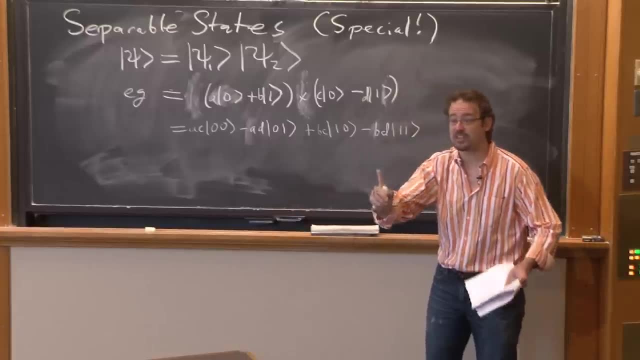 And if I want to know whether the first particle is going to be b? OK, So, that's fine. So imagine, so the probability of the first particle being up or down is independent of any information about the second particle, right? But there's another thing that's important. 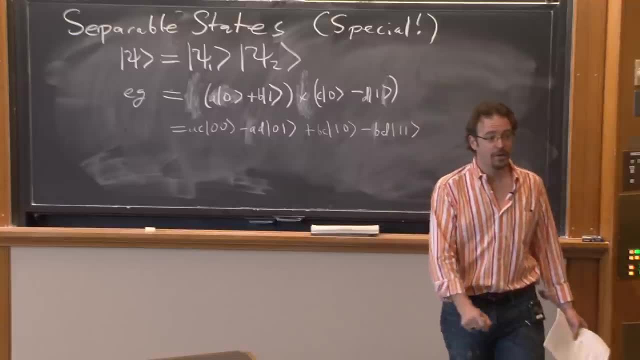 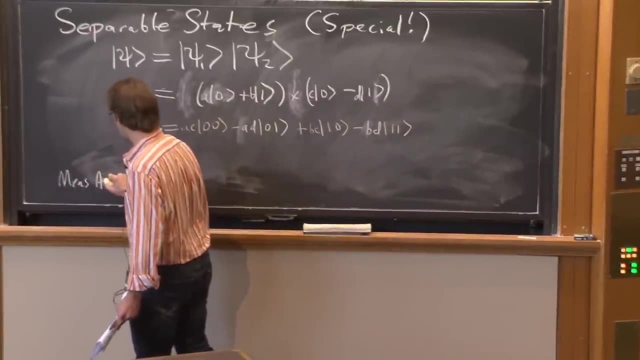 Suppose I tell you: aha, I've measured and the first particle is in the state 0. OK, Cool, What is the state subsequent to that measurement? So if we measure a is equal to 0, what does that mean? 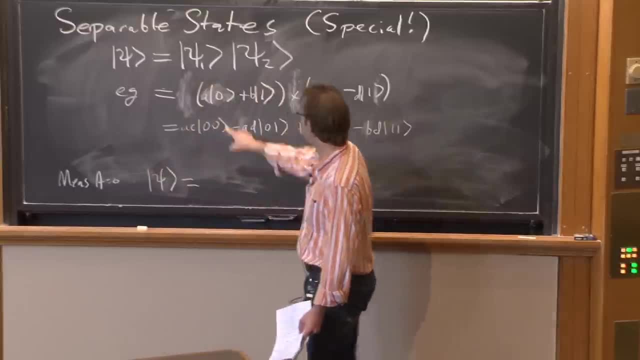 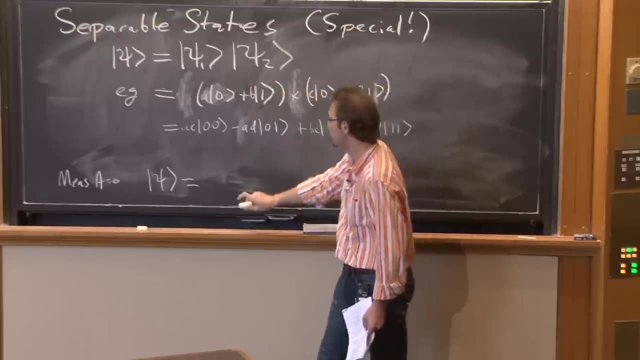 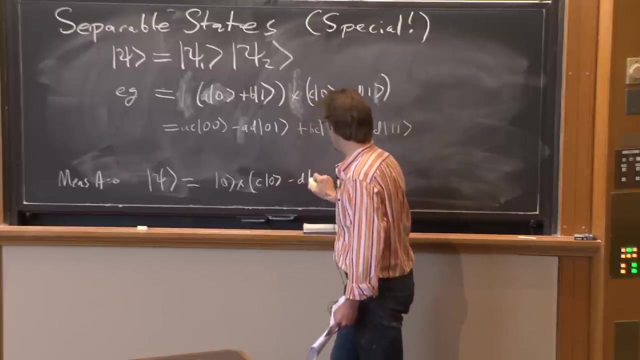 What is the state? subsequent Psi is equal to well, that's 0, and we know we've lost this. So this particle is now this particular subsystem, this particular qubit has been collapsed to the state 0. So we have 0 times c0 minus d1 for the second particle. 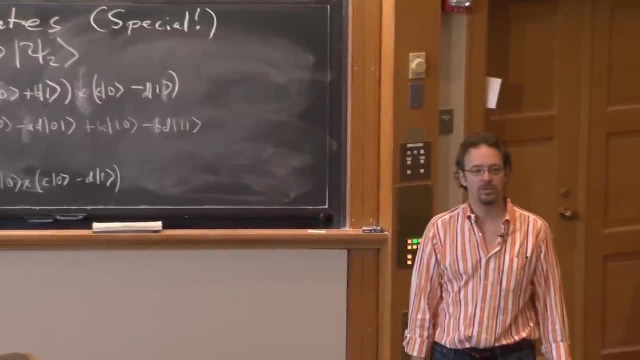 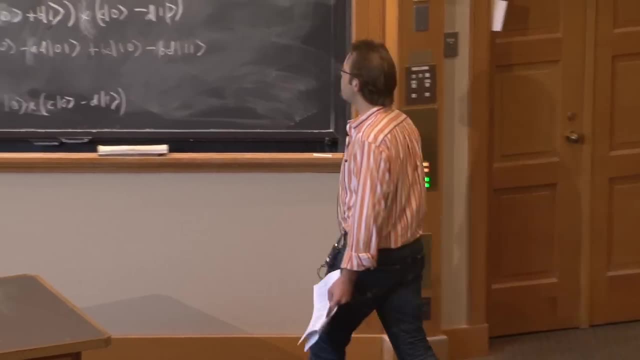 Have we learned anything about the state of the second particle? Have we learned anything about the state of the second particle? Absolutely not. right Beforehand. what was the probability that the second particle was 0? Norm c squared And the second particle 1?? 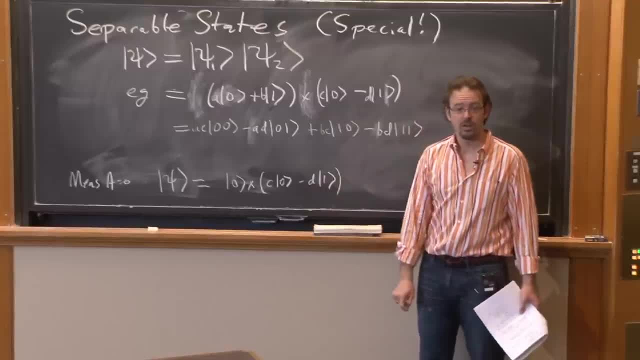 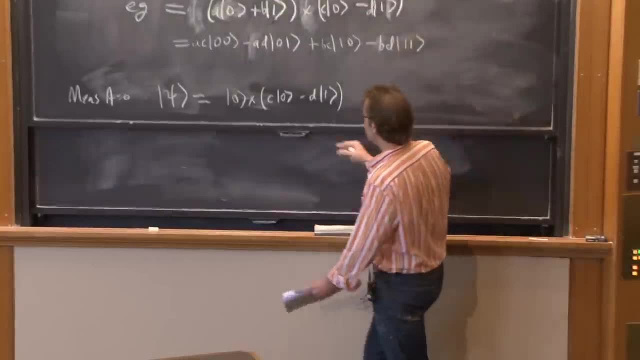 Norm d squared. Now what's the problem? Same norm c squared, norm d squared. So when you have a separable system, measuring one qubit tells you nothing about the other qubit- cool. On the other hand, consider a state which is not separable. 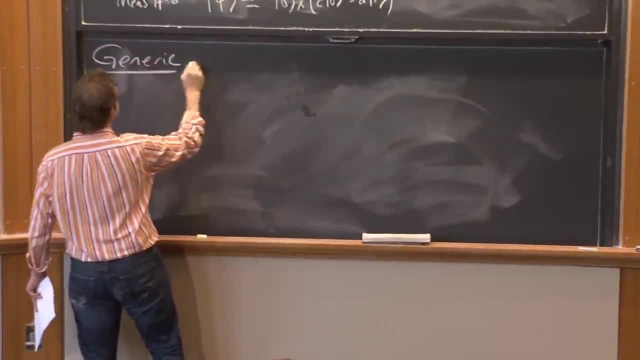 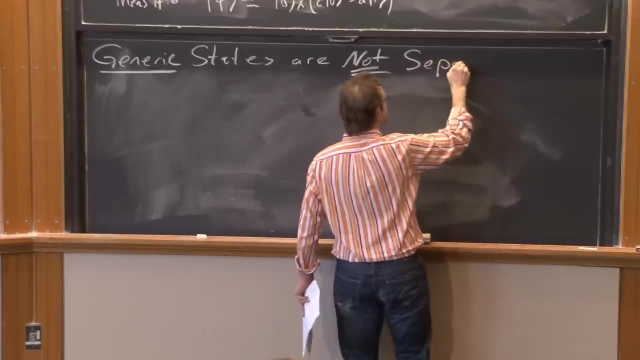 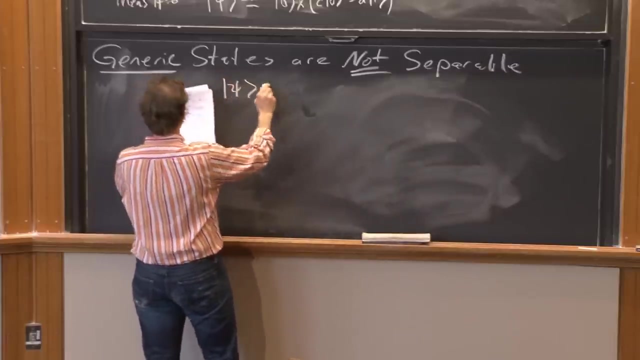 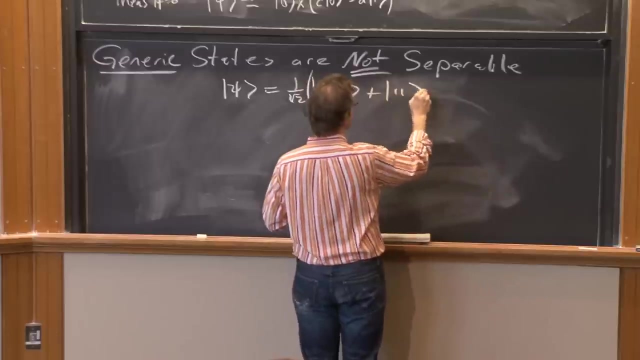 So the generic state? generic states are not Not separable. And let me give you an example of a state which is not separable. Which one do I want to pick? Yeah, what the hell. Psi is 1 over root, 2, 0, 0, plus 1, 1.. 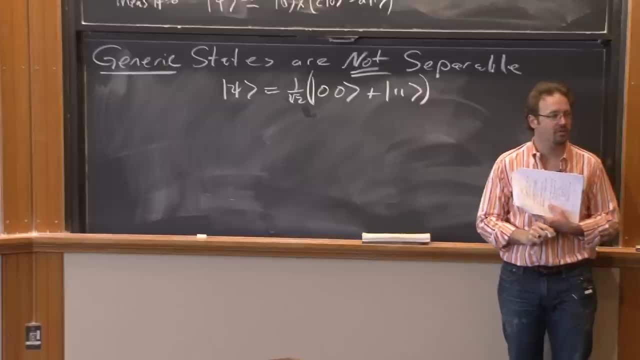 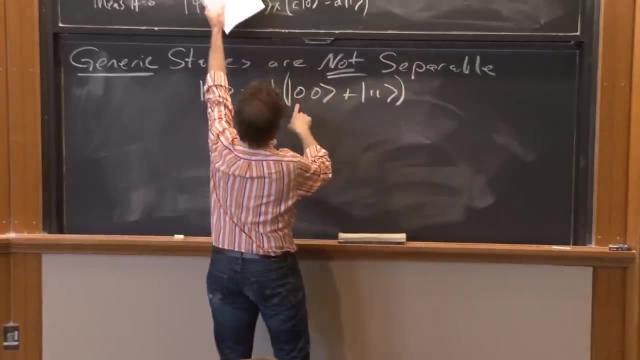 Can this be written as the product of the first particle in one state, the second particle in the other? No, because there would have to be cross terms which don't exist here. Just compare this to that form. So we have that. the coefficient of 0, 0 is ac, both so a and c. 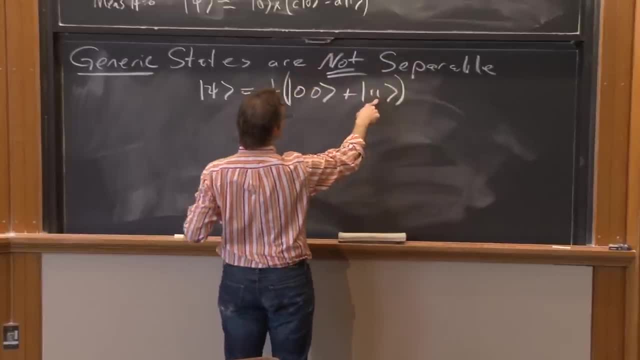 must be equal. Both must be non-zero And the coefficient of 1, 1 is bd, So the coefficient bd must be both of those must be non-zero. So ac and bd are all non-zero. That means these terms have to exist in order. 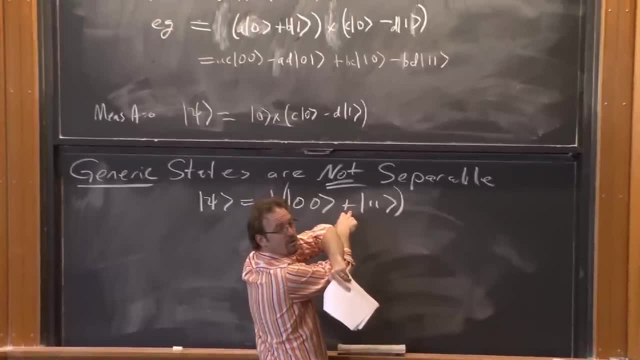 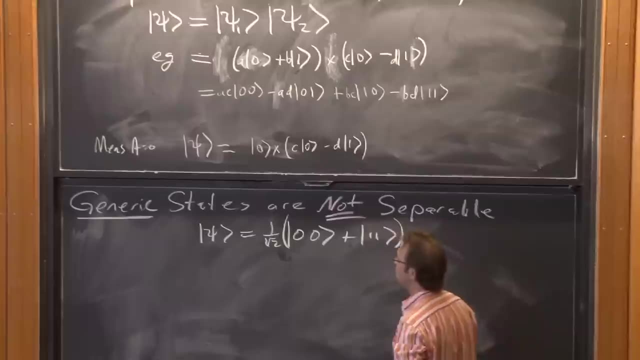 for it to be separable. Yeah, Because a and d can't vanish and b and c can't vanish, and these are orthogonal states. They're independent. So this is not a separable state. We call these states entangled. 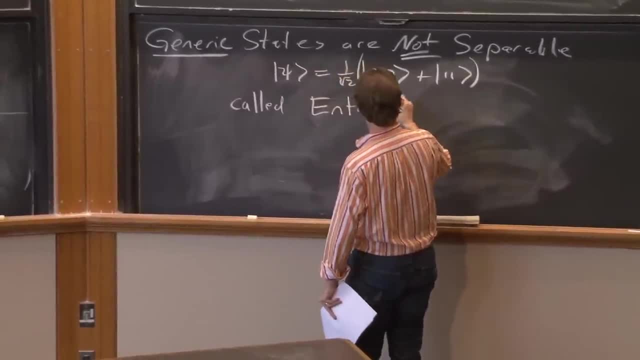 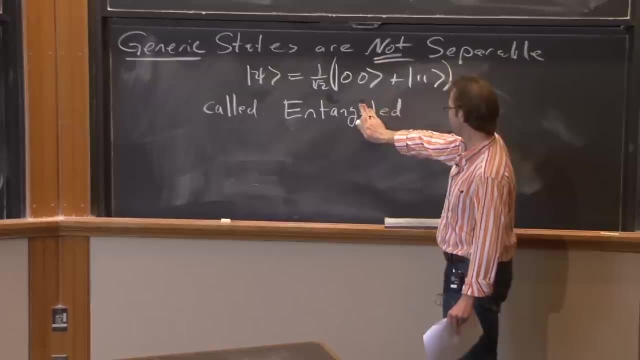 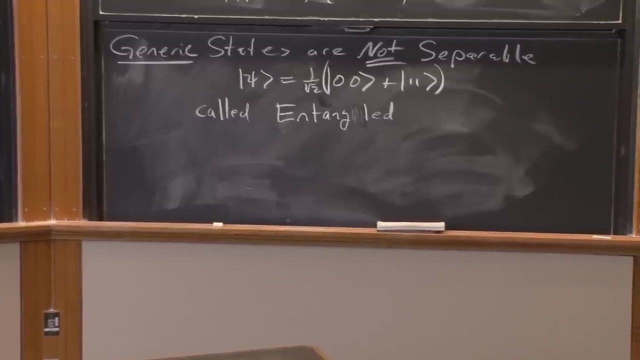 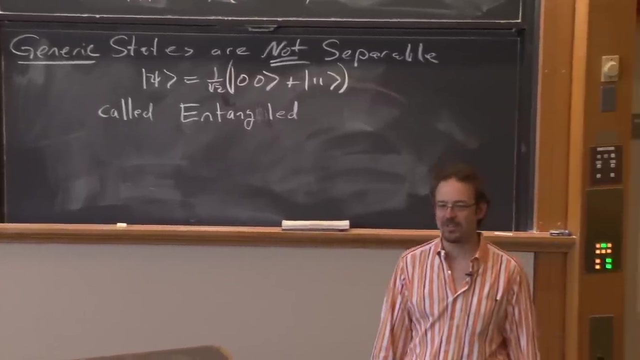 And it's funny because entangled, I think there's an e in there. OK, that's better. Look, I'm not a professor of spelling, So we call these states. It's a little bit funny to give these a special name. 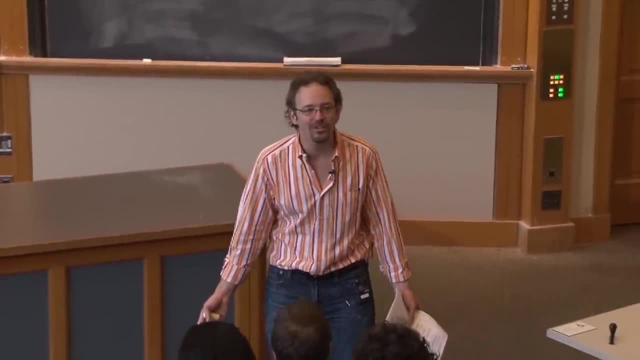 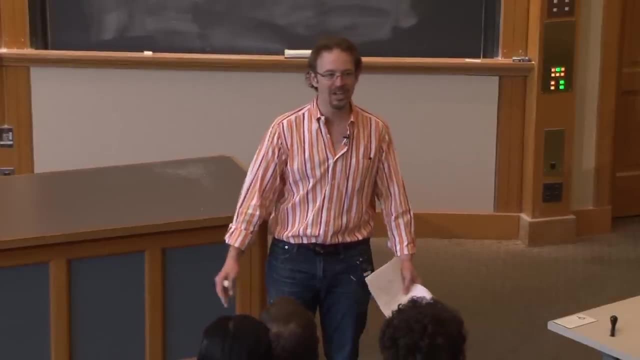 and call them entangled, because the generic state is entangled. It's sort of like calling mice mice and calling all the other mammals non-mice, Right, Oh, look, Well, that was a bad example. A look at mice ran across the room. 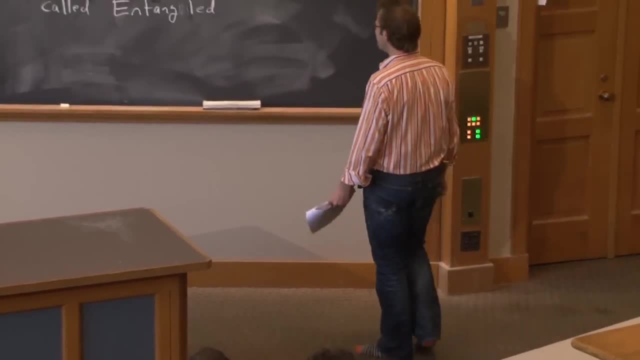 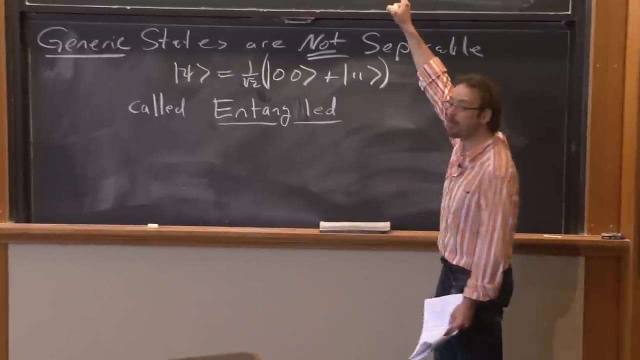 So hearkening back to an earlier lecture, But in any case, we give these a special name And the reason we give them a special name is that these separable states do more or less what you expect classically. There are no strange correlations. 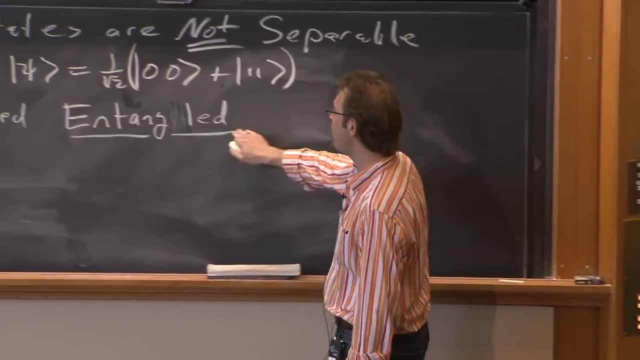 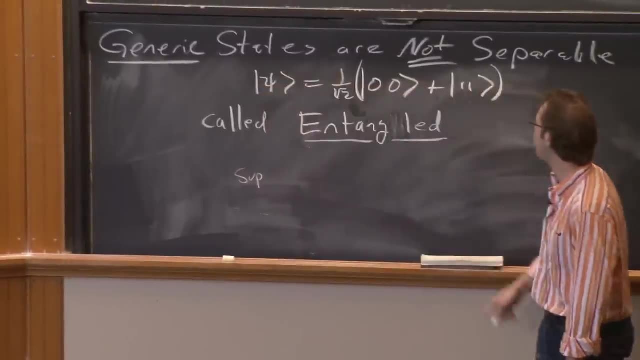 between the state of one and the state of the other. They are independent quantities, But when you have a generic state, something funny happens: They're entangled. And here's the funny thing that happens. Suppose, given this state, what's the probability? 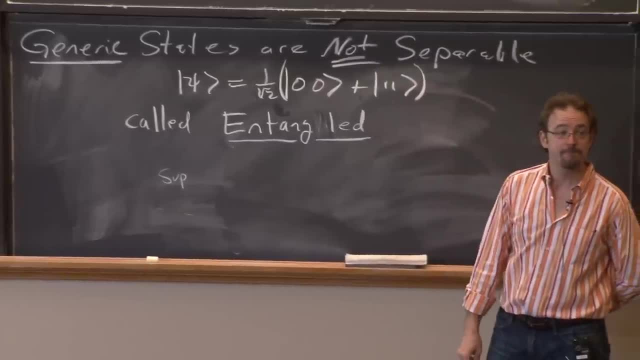 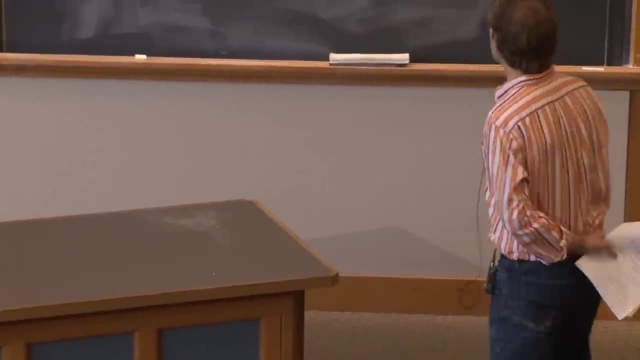 that I measure the first particle to be up or to be 0? 1 1⁄2.. What's the probability that I measure the first particle to be 1? 1 1⁄2.. So, before doing any measurements, 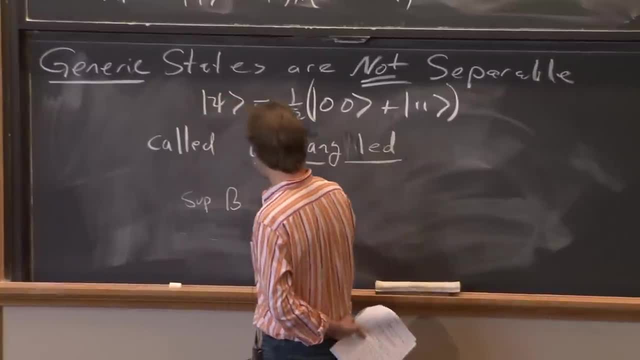 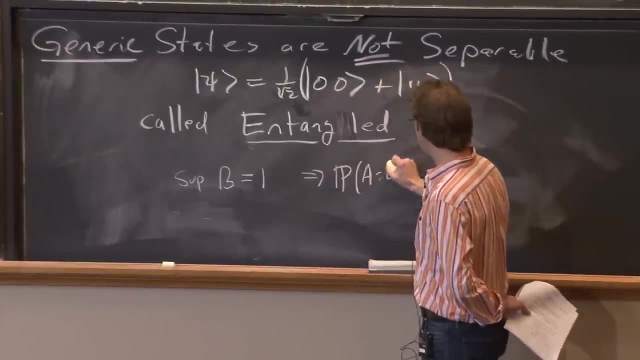 the first particle is equally likely to be either 0 or 1.. But suppose I measure the second particle to be up, Then the probability that I measure the first particle is 0 is equal to 0.. And the probability that the first particle is 1. 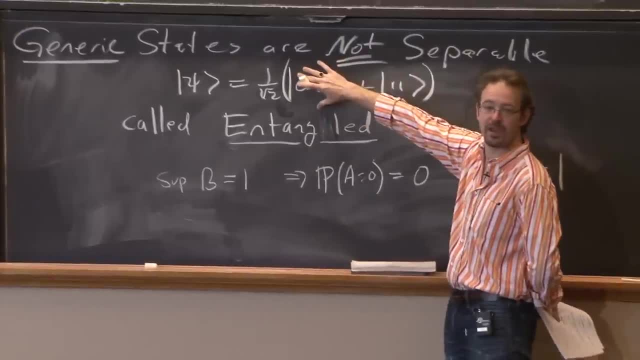 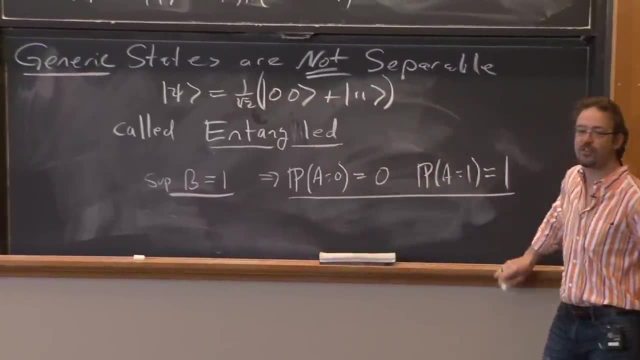 is equal to 1. 1. 1. 1. Because I've collapsed onto this term in the wave function. So measuring the second qubit alters the probability distribution for the first qubit. These guys aren't independent, They are correlated in a way that you. 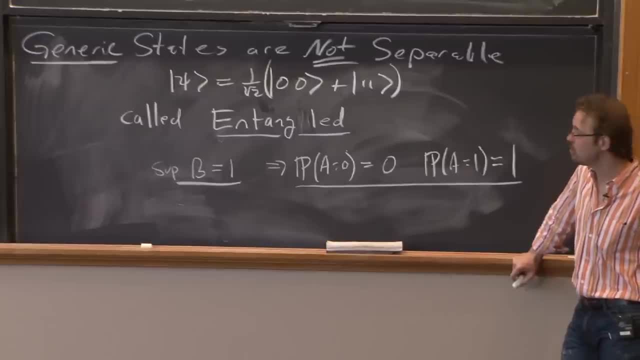 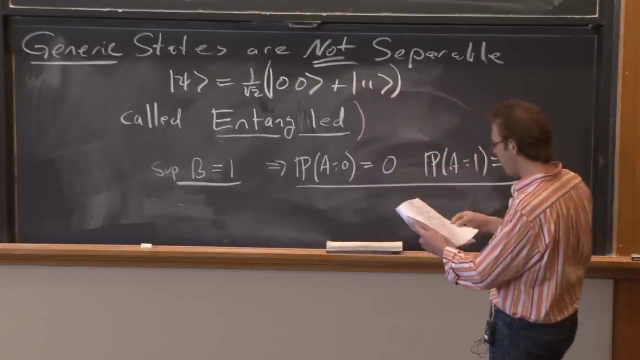 studied on the problem side. They are correlated, They're in a correlated state. We call this correlation entanglement. And here's the thing that's most spooky about this, And we'll come back to this in a few minutes. But I didn't tell you anything about the geometry. 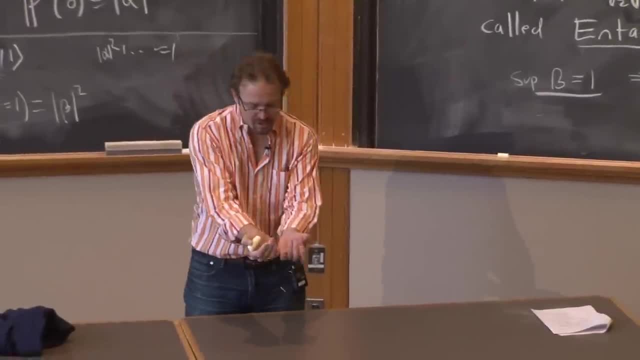 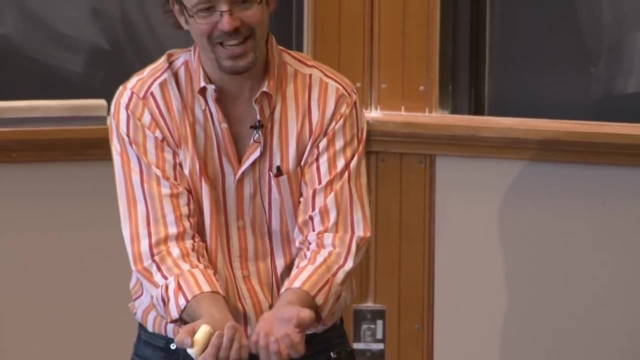 of this setup. But in fact, when I was thinking of that measurement, I built the two little qubits in my lab And then I took one and I sent it to France, And I took the other one And I sent it to the planet Zorg. 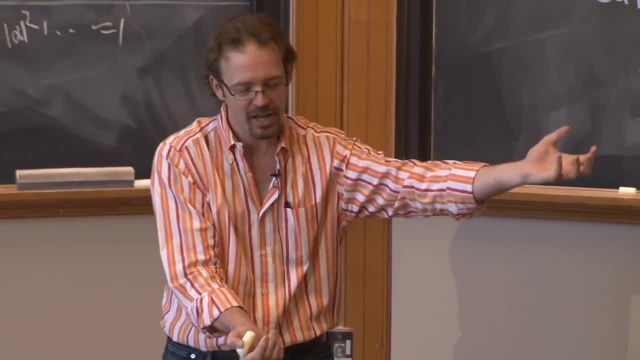 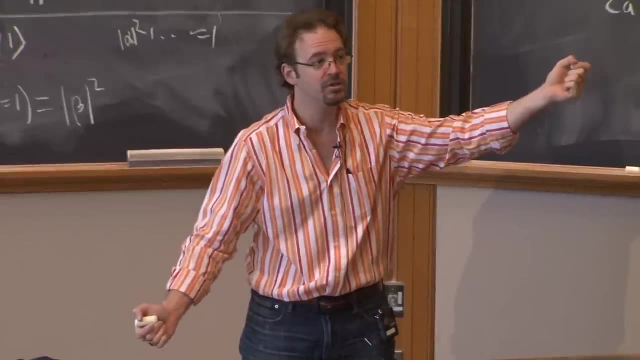 And so off on the planet. Zorg is some poor experimentalist huddling in the cold And our French experimentalist makes a measurement altering the probability distribution instantaneously on Zorg. That should make you a little worried. That sounds a little crazy. 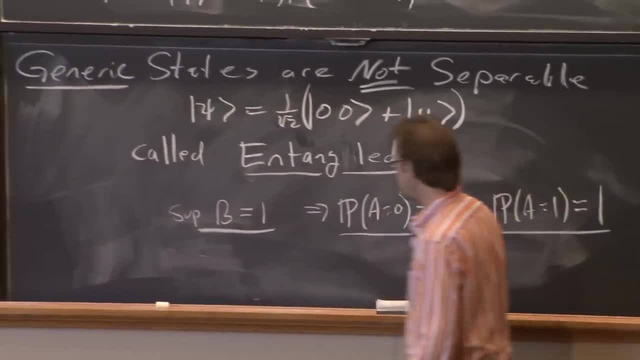 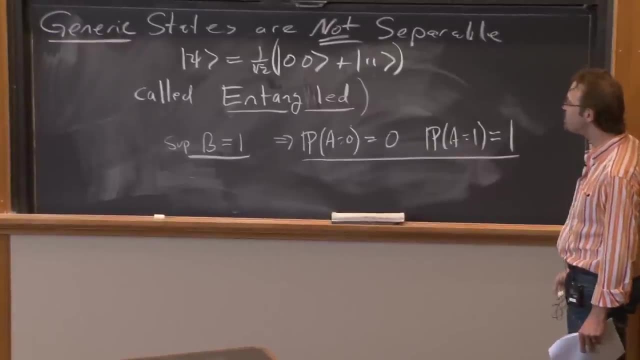 We'll come back to why that is or isn't crazy And the EPR analysis, which sort of puts flesh on it, sounds crazy in a little bit. But for the moment let me just emphasize that while the generic state is entangled, 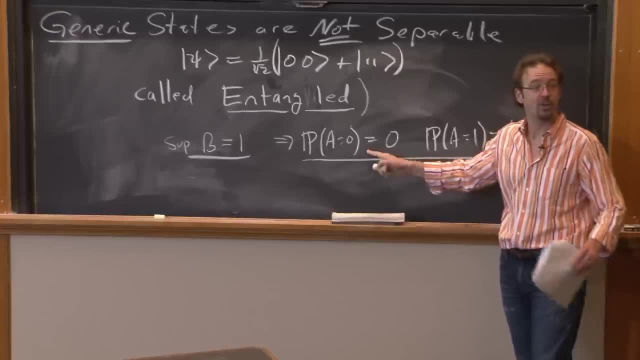 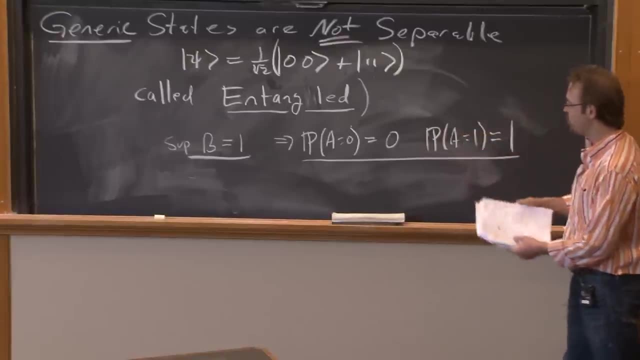 the generic state is also different than what your classical intuition would expect. There are correlations between the particles, So this is something that happens with quantum mechanical particles, that doesn't happen with classical particles, And that means it's something that can be used in a quantum. 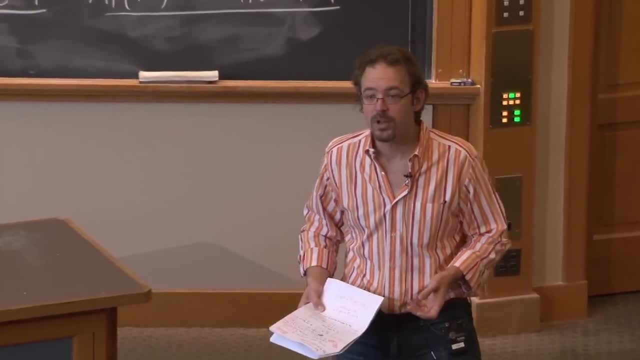 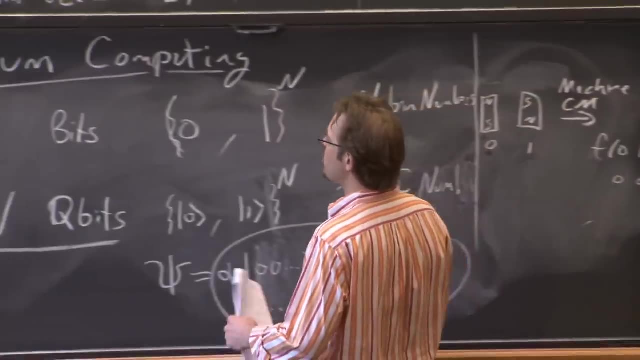 computer that can't be used in a classical computer. So let's see. So let's see what using entanglement gives us for computation. So let's come back to the quantum computing problem. And how do we compute with qubits? So how to compute. 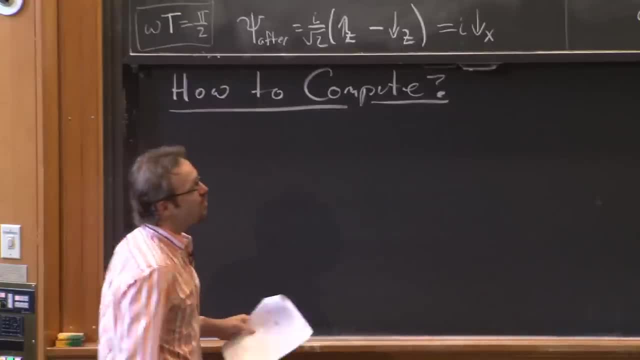 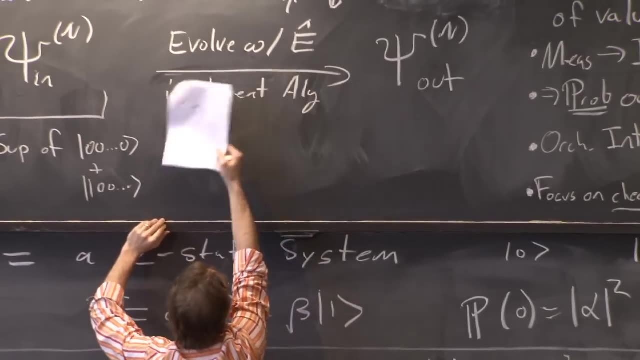 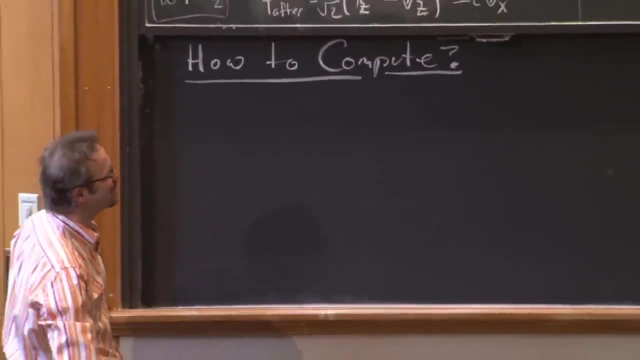 So again, as usual, the way we take our input to our output is we build a machine that implements an algorithm of our choice by arranging the physical evolution of the system under time. So that means picking an electric field, Or, sorry, an energy operator. an electric field, good lord. 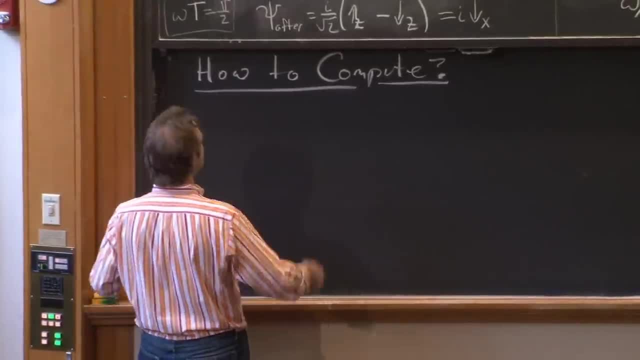 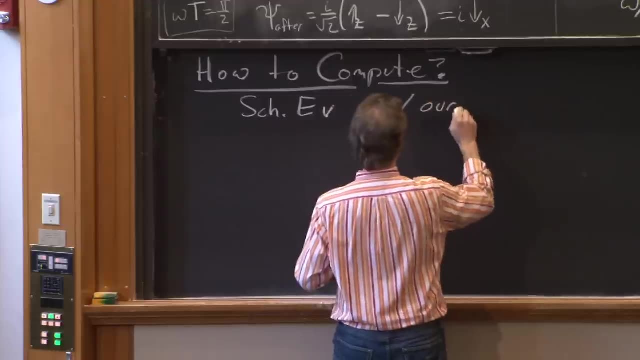 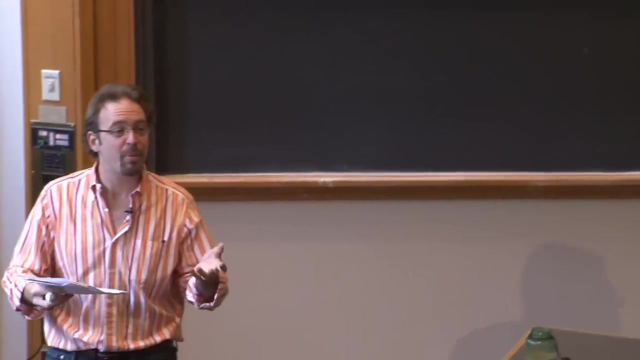 So it means picking an energy operator. So computing is Schrodinger evolution with our chosen or our tuned energy operator. So, for example, I want to build for you now a couple of basic circuit elements that you might want to use in a quantum computer. 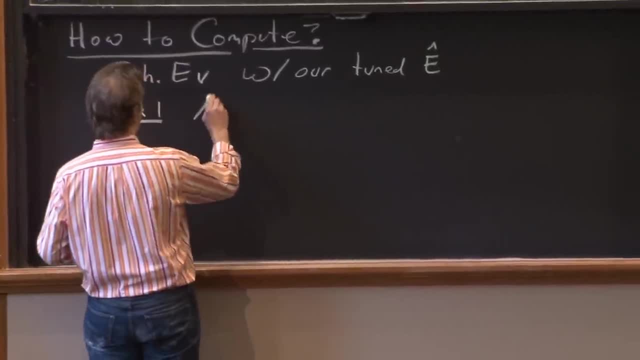 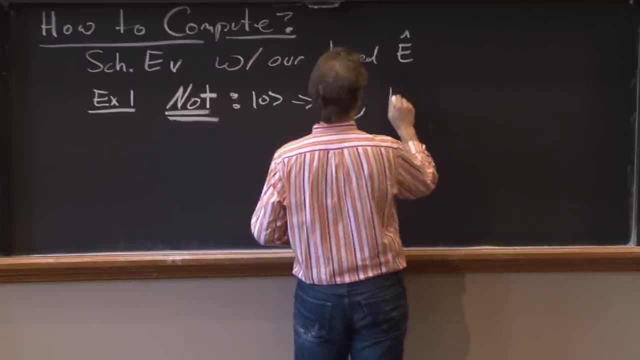 So example one, First example, is: I want to build a NOT gate, And what NOT means is it takes the state 0 and gives me 1.. And it takes the state 1 and it gives me 0. This is what NOT does. 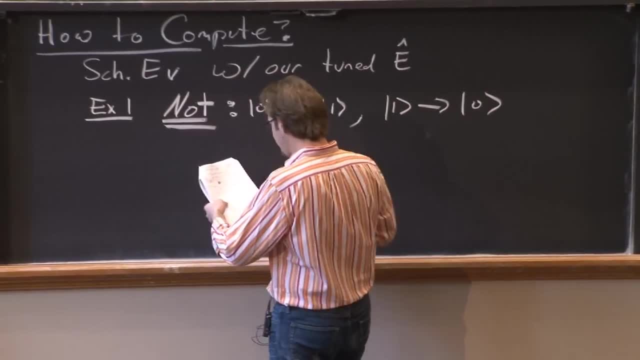 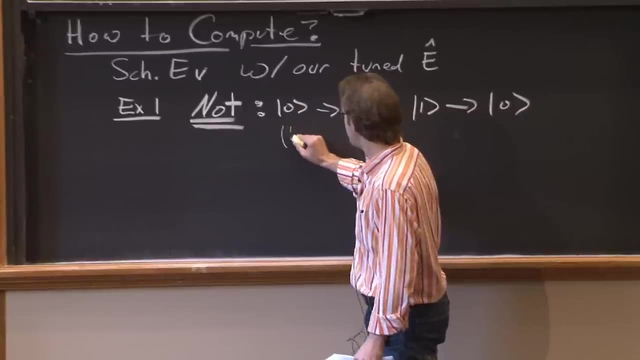 So how do I build a NOT gate? Well, I can realize this in a nice way. Do I want to say it that way? Yeah, good. So if I realize 0 as 1, 0 and 1 as 0, 1 from last lecture, 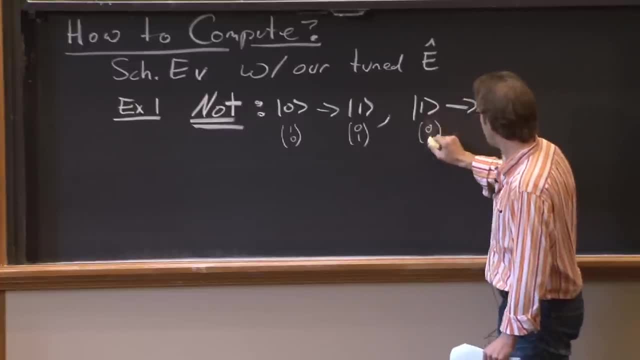 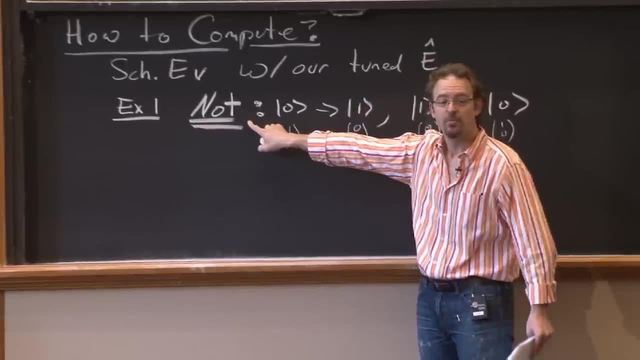 then 1, 0. Oh sorry, 0, 1.. 0, 1, 2, 1, 0.. So we need an operator, We need time evolution, to effect multiplication by an operator that takes this vector to this vector. 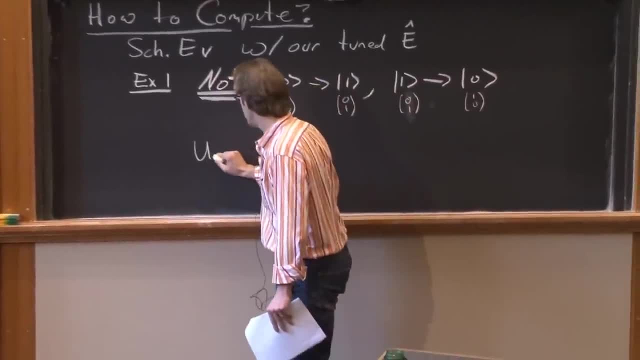 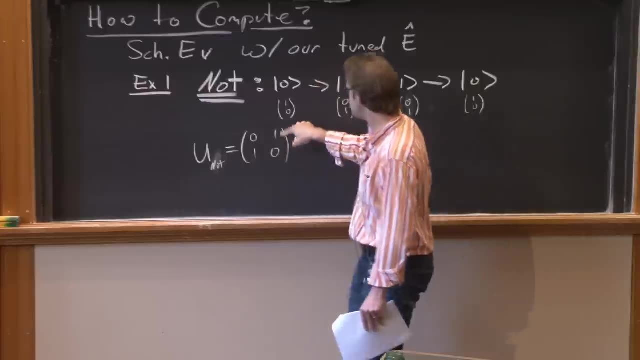 and this vector to this vector. But we know what that unitary operation is. That unitary operation, which I'll call NOT, must be equal to 0, 1, 1, 0. And this operation takes this guy to this guy. 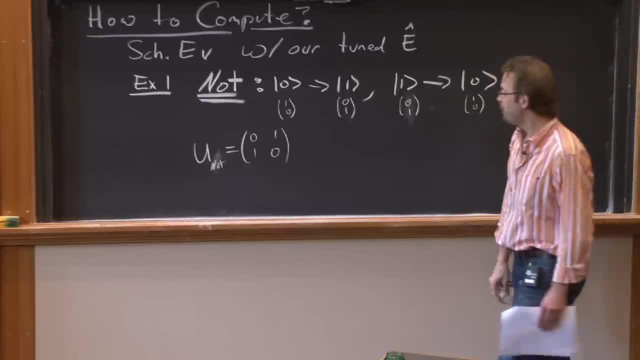 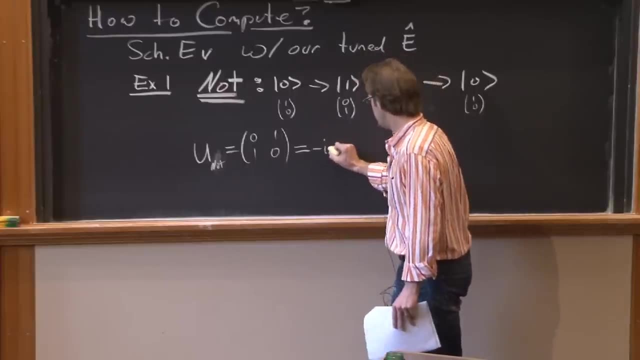 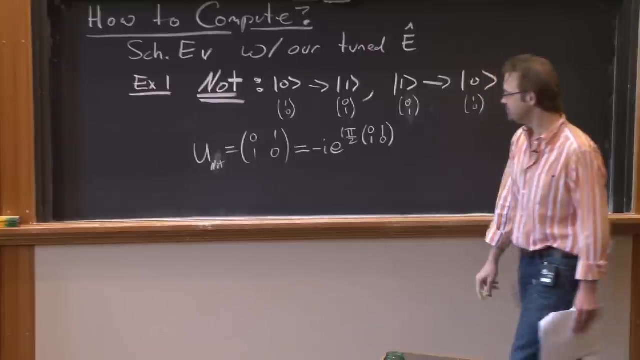 and it takes this guy to this guy. Yeah, But I can write this. I like this. I can write this as shoot. there's a phase minus i e to the i pi over 2, 0, 1, 1, 0.. 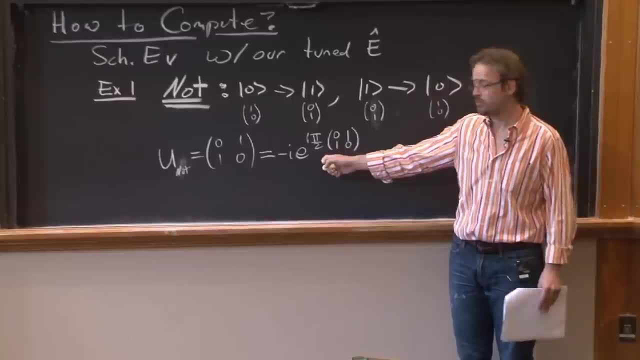 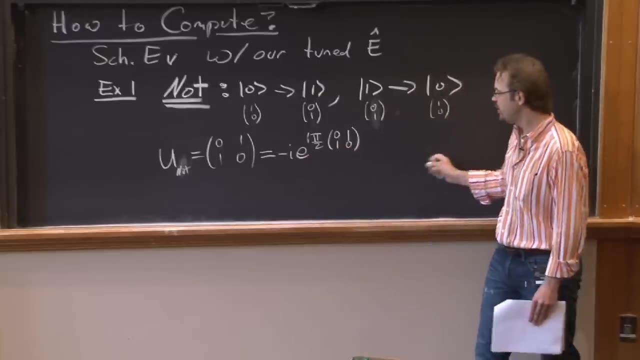 I mean you can't stop me. So this expanded out as we've done before. expanding this out gives me, with the exponential 1 plus the thing and then all the other terms, This becomes minus i times cosine of pi over 2.. 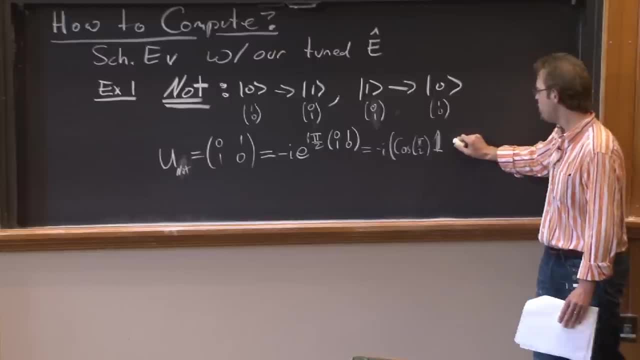 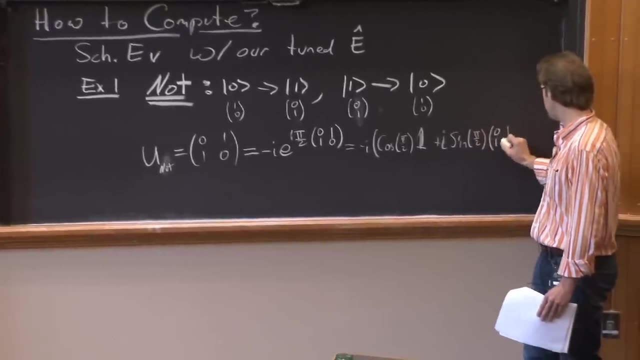 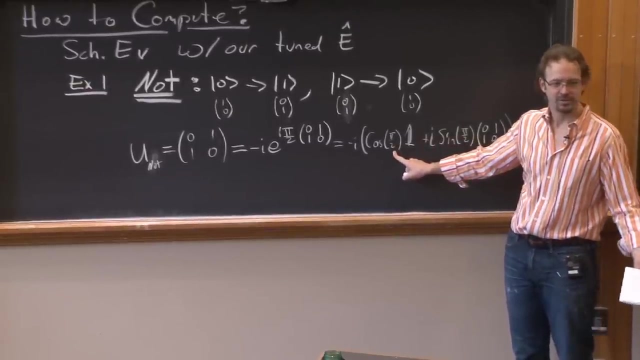 1 times the identity, the 2 by 2 identity plus i sine of pi over 2 times 0, 1, 1, 0.. But what's cosine of pi upon 2? 0. Yeah, 0.. 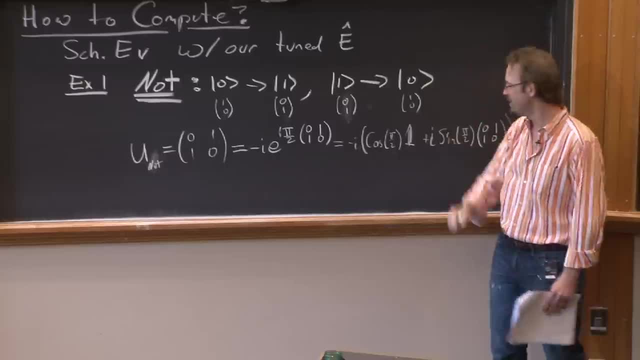 Come on, Because I've been that tired. So cosine pi over 2 is 0.. Sine of pi upon 2 is 1.. That gives us i times minus i, That's 1 times 0, 1, 1, 0.. 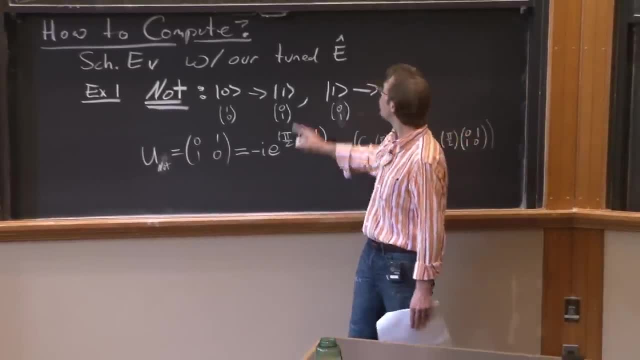 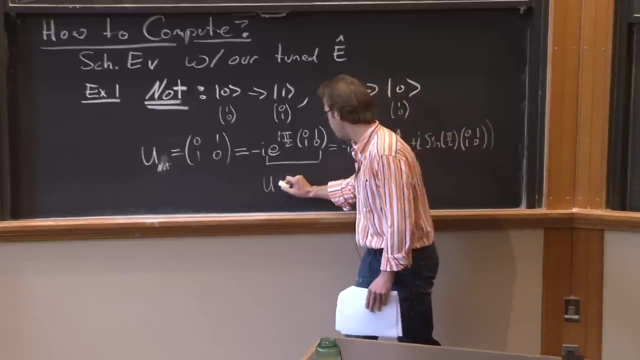 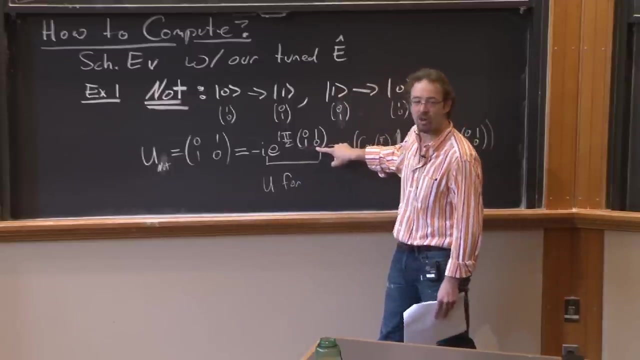 Pretty solid. But what is this? Well, this is Schrodinger evolution with a magnetic field, and this is just the unitary transformation for a magnetic field. Well, OK, we can say this: This is the x-poly matrix from last time. 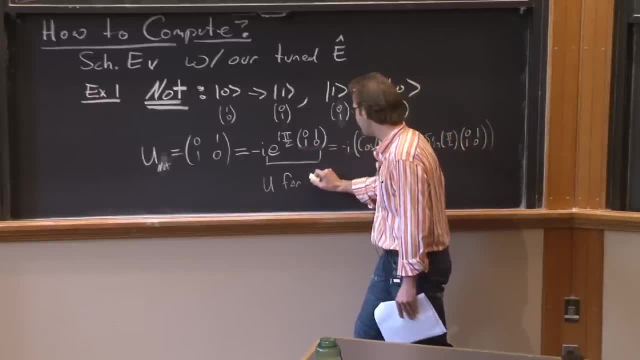 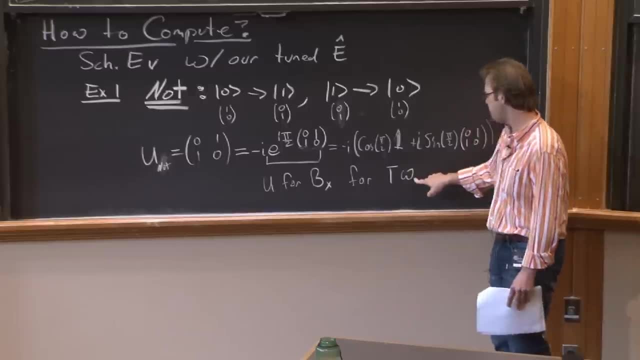 So this is like Sx Unitary transformation for a magnetic field in the x direction for some time, t for a time. t times the frequency omega which is given by mu b upon 2.. It is equal to pi upon 2.. 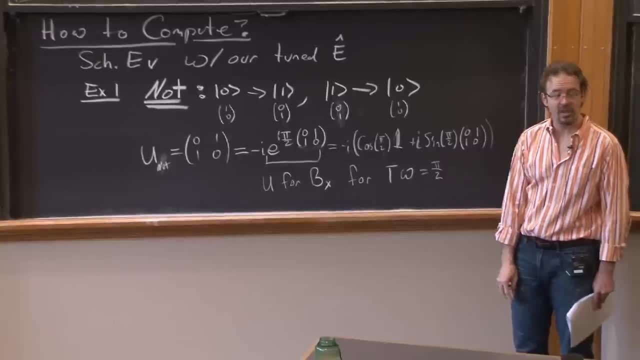 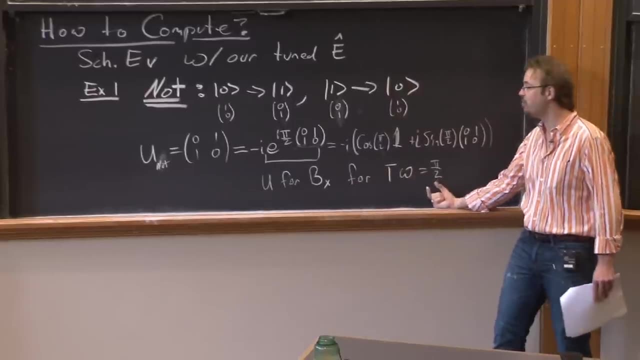 Just like before, but for a slightly different one, Slightly different magnetic field. So my point here is that we can pick a magnetic field that does this. We turn on a magnetic field with a known amplitude, with a known amount of time. Details here don't matter so much. 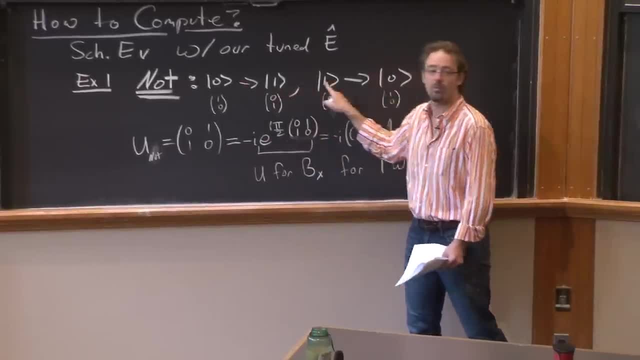 The point is we can do it. We turn on a magnetic field in the x direction and it takes 0 to 1 and 1 to 0.. Everyone cool with that? So here is a substrate, an actual physical system that affects this particular evolution. 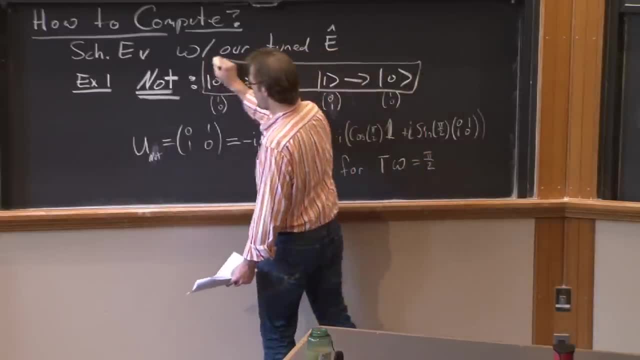 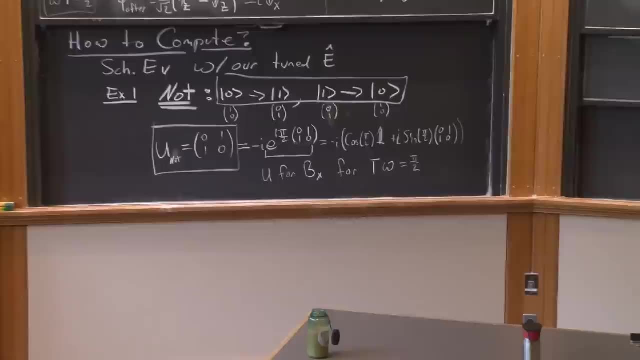 I can build a knot. The crucial thing is: I can build a knot, I can build a knot gate And I'll represent that knot with some unitary transformation: u sub knot. So that's a useful one, but it's not the most useful gate. 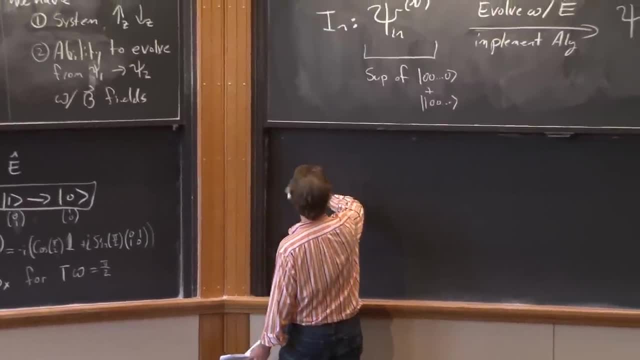 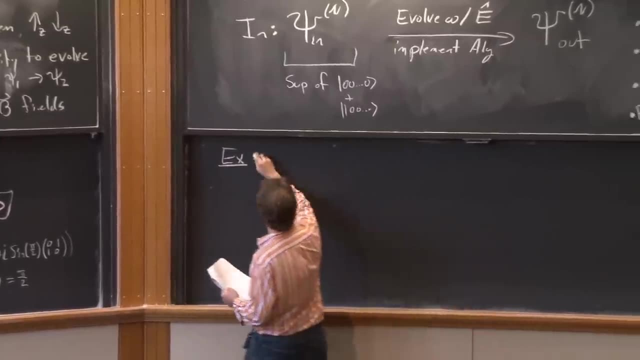 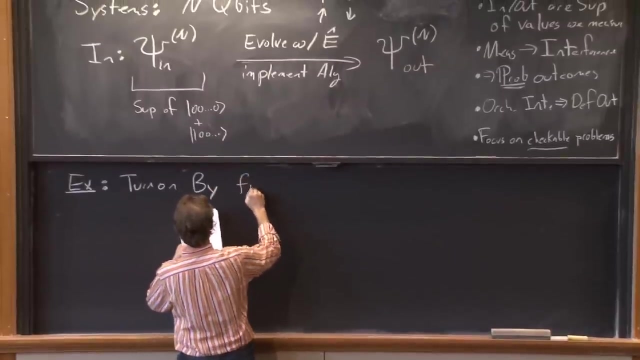 If you only ever impose logical knots, you just get everyone angry, But you don't actually get anything done. So second example: let that be a lesson to you, Congress. So the second example: if we turn on the magnetic field in the y direction for a time t 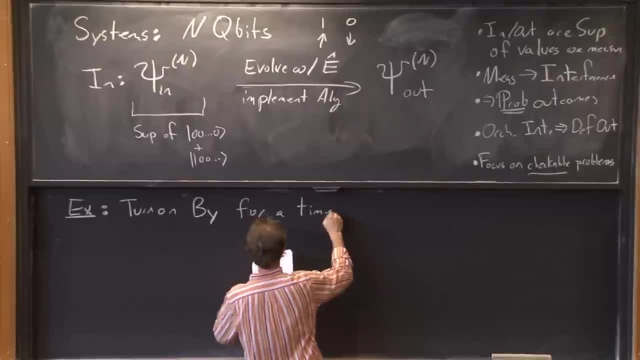 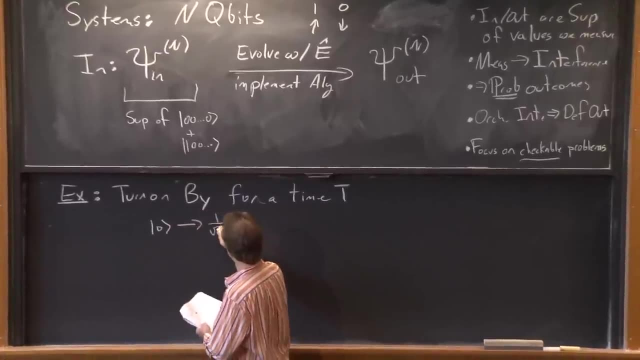 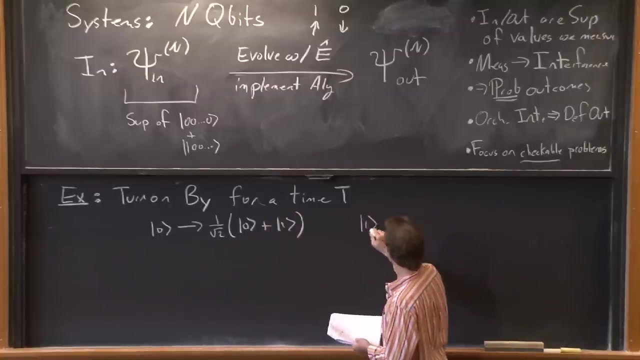 For a particular time, t. what we find is that 0 goes to 1 over root 2, 0 plus 1.. And 1 goes to 1 over root 2, 0 minus 1.. And this should be familiar. 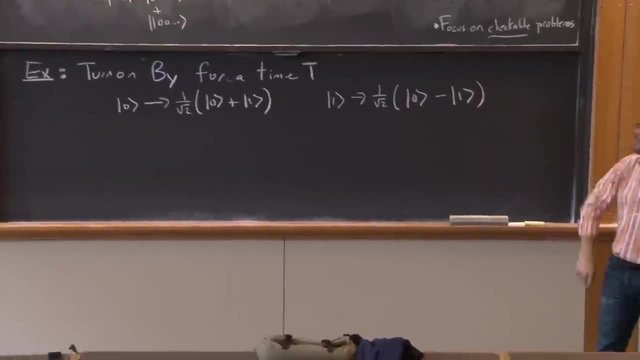 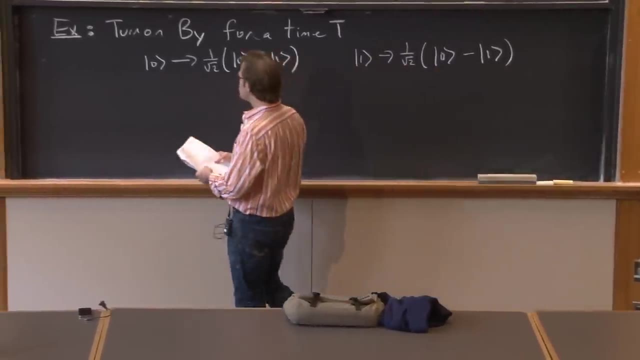 This is the up x state and this is the down x state, just as we talked about before. So we turn on some b field and we get this. So this operation has a name because it's going to turn out to be very useful for us. 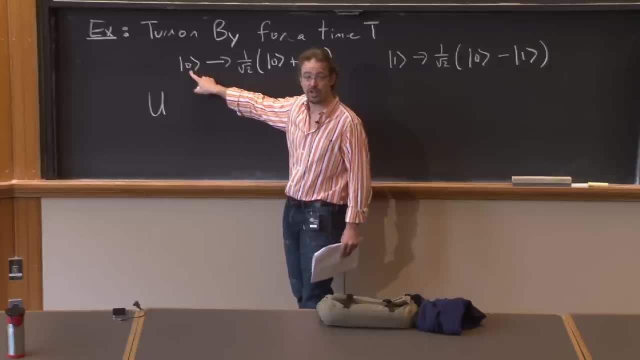 It's taking a system that's definitely in the state 0, for sure, and it puts us in a superposition of 0, 1.. It's a definite superposition, so it's not like we don't know what happened. 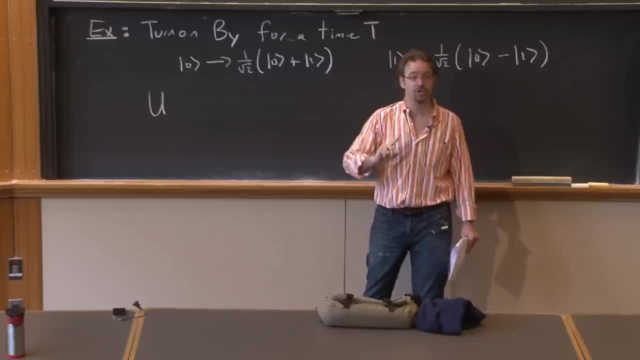 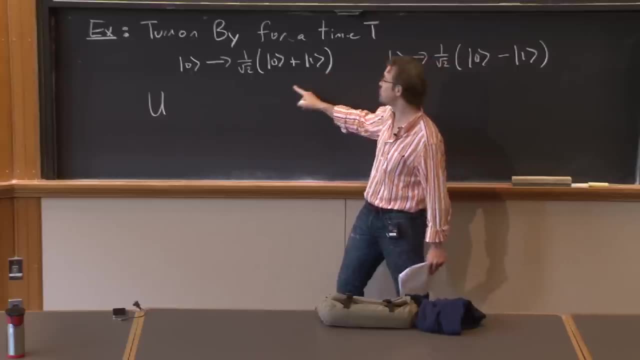 But it's a superposition and you've lost certainty that you'll measure up in the z direction. You've gained certainty that you'll measure up in the x direction, But if we do all our measurements in z, we've just taken ourselves from definite to superposition. 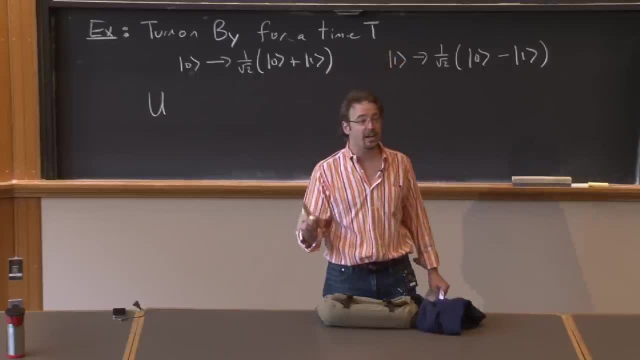 Cool. So that's useful because we know that something a quantum computer can do that a classical computer can't do. something a quantum computer can take advantage of that a classical computer can't take advantage of, is this process of putting things in superpositions. 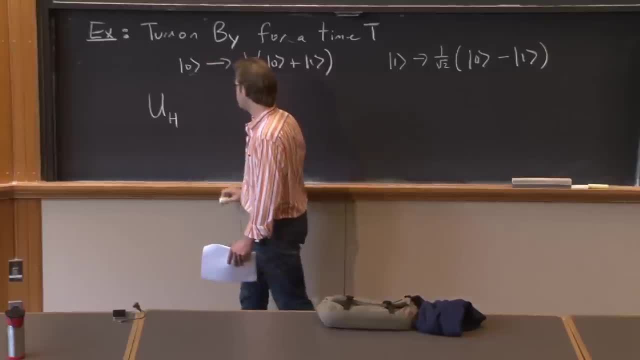 So here we've got an operation that puts things in superpositions And I'll call this Hadamard, And I don't know the history of why that's called Hadamard, but presumably there's some guy with the last name Hadamard. 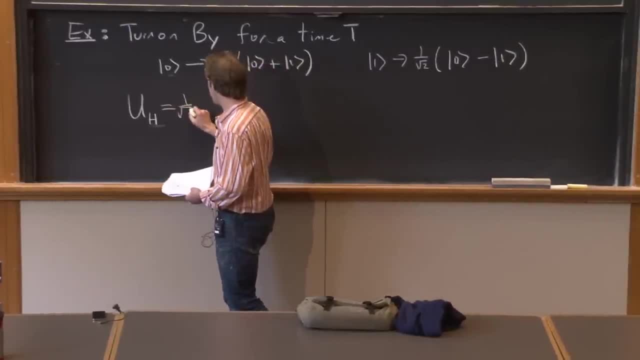 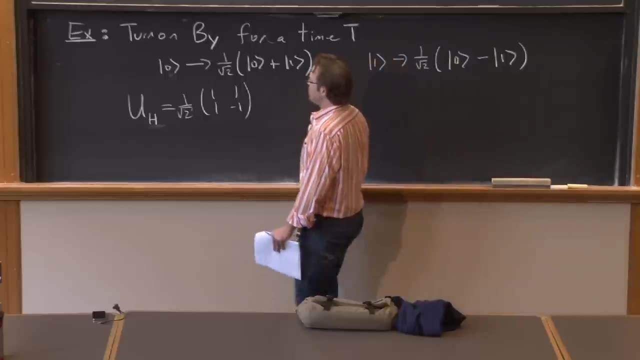 Anyway, the? u Hadamard does this And as a matrix it's represented as 1 over root 2, times 1 over root 2.. 1, 1, 1, minus 1.. And there's a last one which is going: 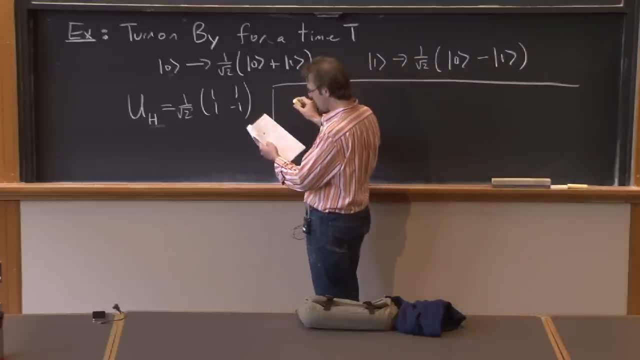 to be useful for me. which is called, which is oh, and this is represented in the following way: Well, we don't worry about that. Another one is called c0, controlled 0.. Controlled 0 does a really cool thing. 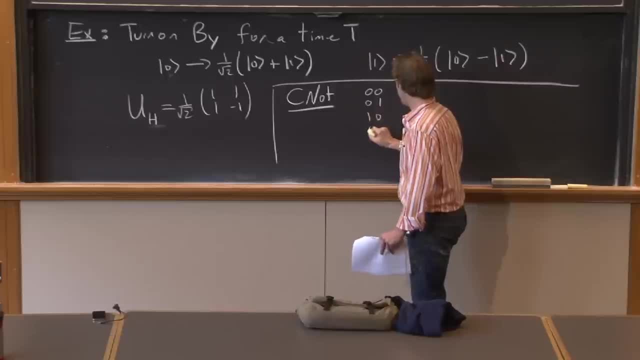 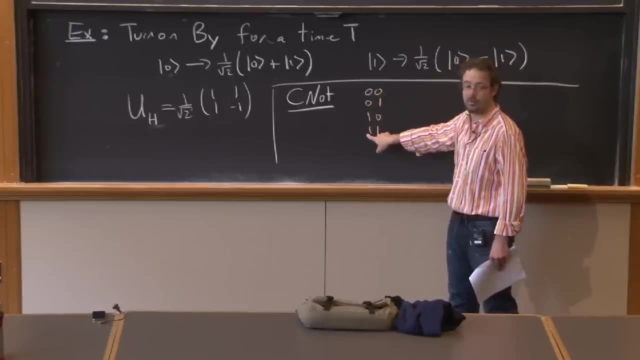 It takes 0, 0, and 0, 1, and 1, 0, and 1, 1.. What it does is it says: I'm going to apply a 0 to the second qubit If, and only if, the first qubit is a 1.. 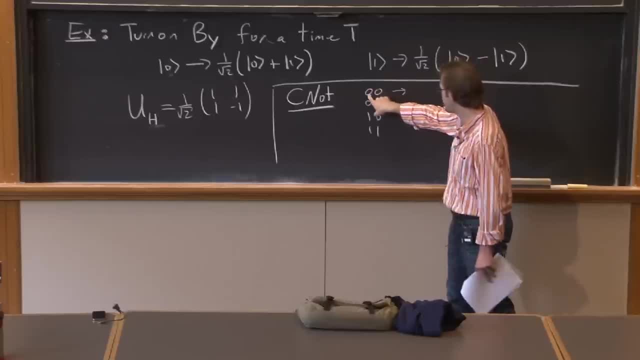 So this takes me to 0, 0 goes to well, do I perform a not on this bit? No, So 0, 0.. Do I perform a not on this bit? No, 0, 1.. Now I do perform a not on 0, so I get 1, 1.. 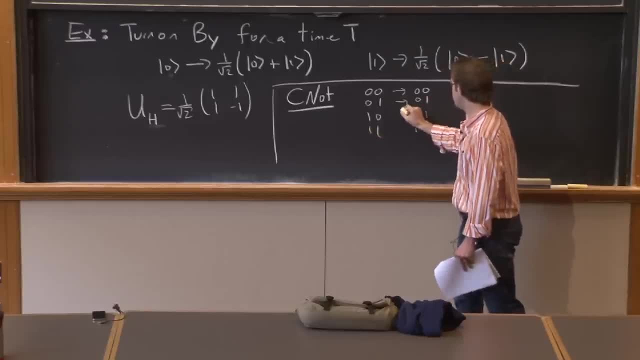 And 1, 1,. I perform a not on this bit, which gives me 1, 0. So this is called a controlled not. It's a very useful thing And I'm going to represent this in the following way. 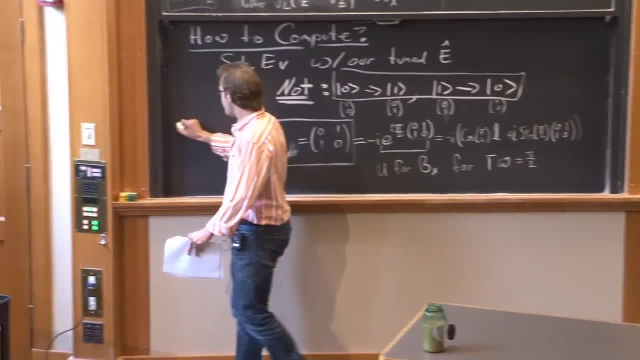 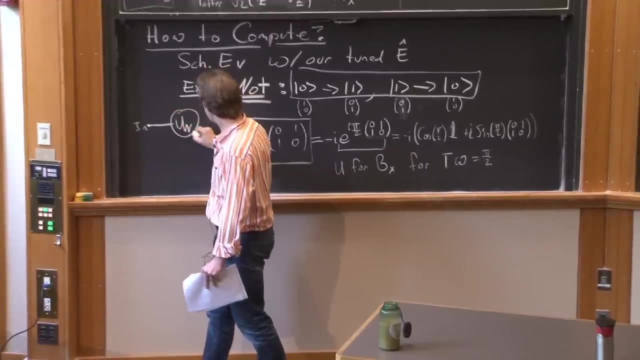 Oh sorry, I should represent this. I'm going to represent all of these, So this not gate. first I take some initial bit and it's in some state, and then I impose u not and it gives me an out state. 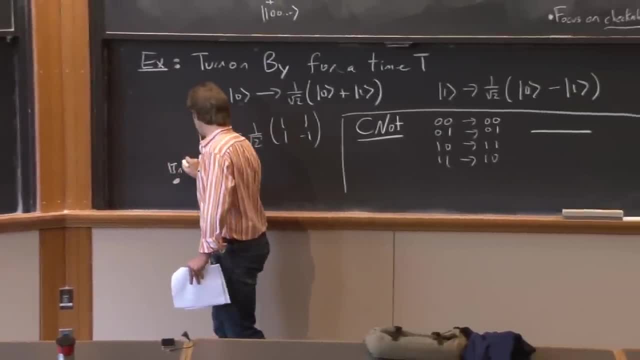 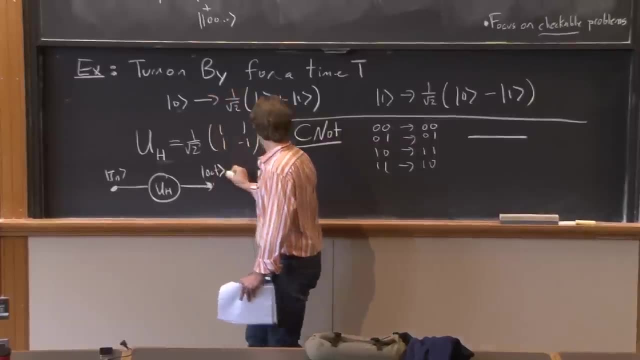 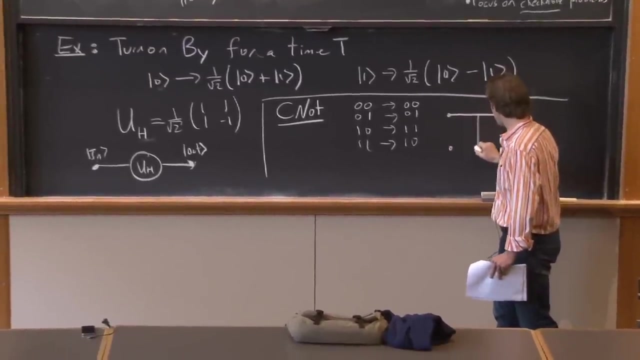 Similarly with the Hadamard. I take an initial state in and I apply u Hadamard and I get u out And for a controlled not. I now have two qubits And I take the two qubits and I do a controlled not which? 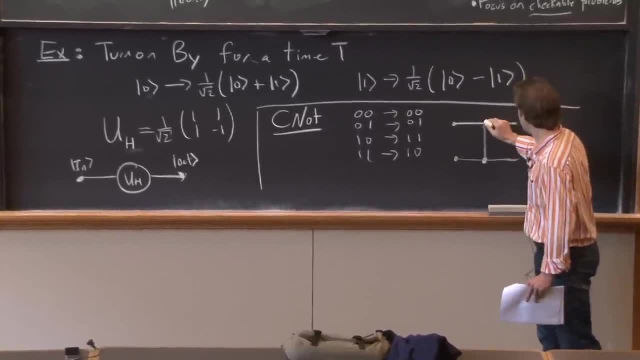 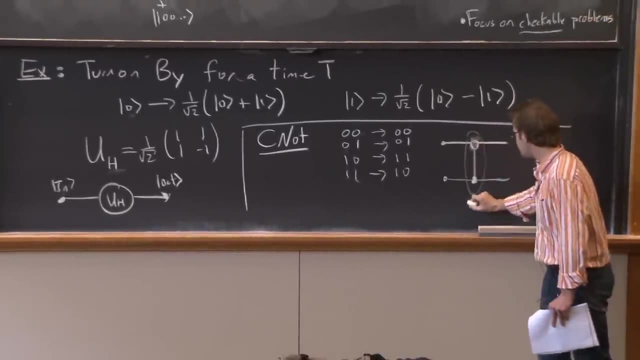 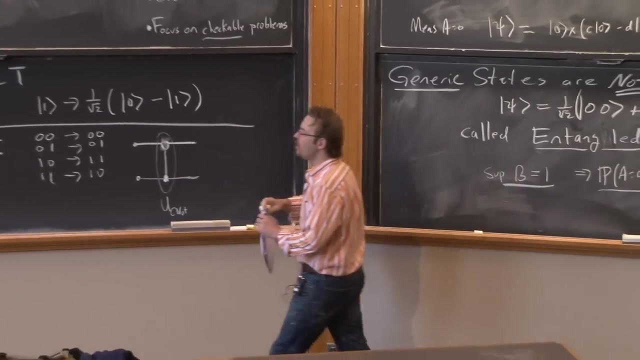 is represented in this form, which says: do a not on this guy controlled by this first bit, And so this acts as u c not. And the key thing here is that, while it's always possible to find a physical representation of some particular unitary transformation, 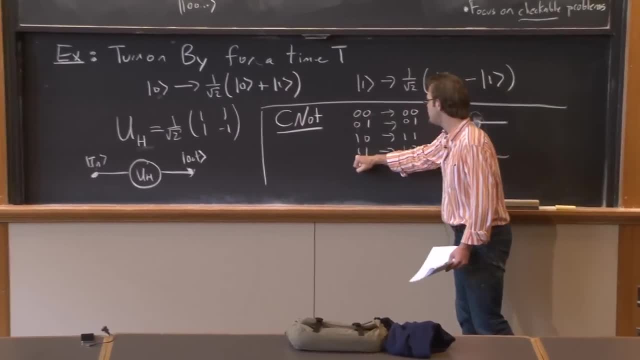 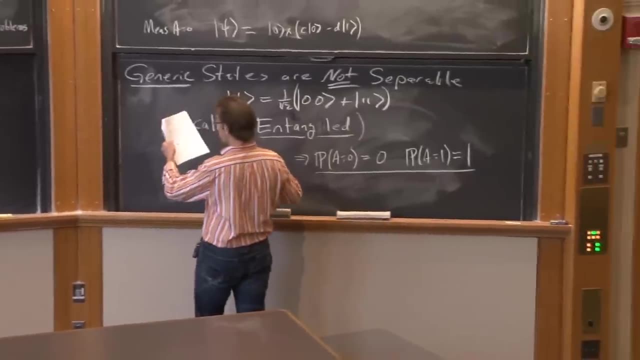 at the end of the day, all we're going to need is some truth table. At the end of the day, all we need is the logic that's being affected, And so the details of the substrate can be abstracted away, OK. 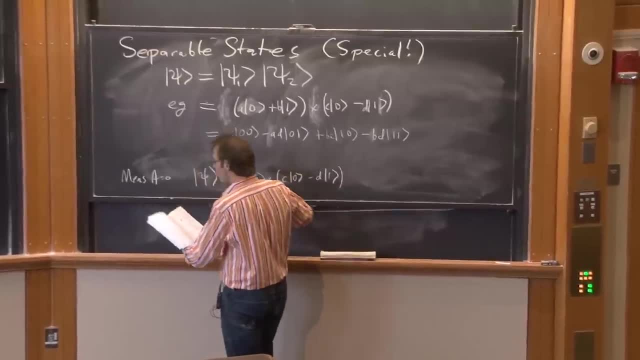 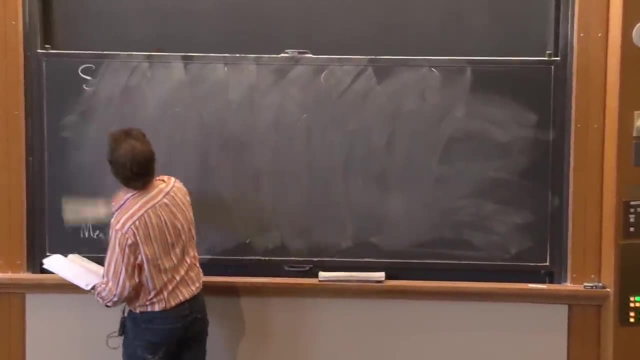 So what can we do with this? So what can we do? Before we actually talk about what we can do with it, let's briefly talk about what you can't do with it. So what are things you can't do with these sorts of operations? 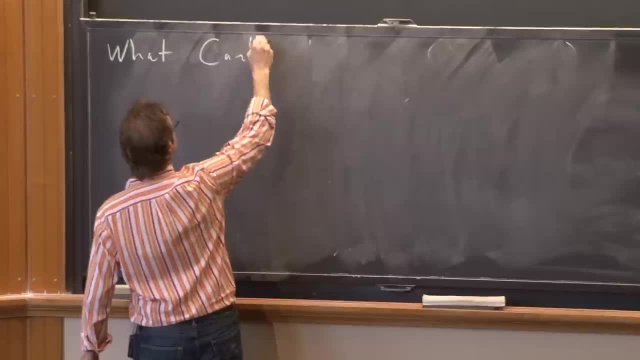 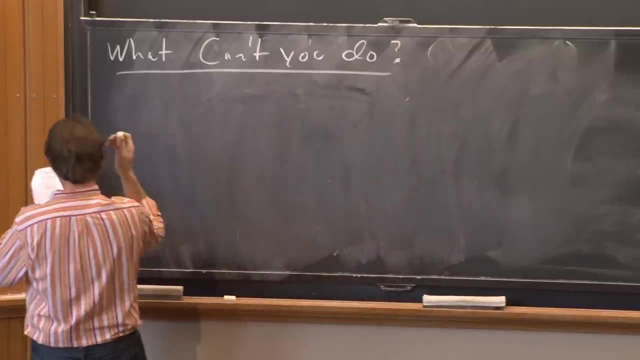 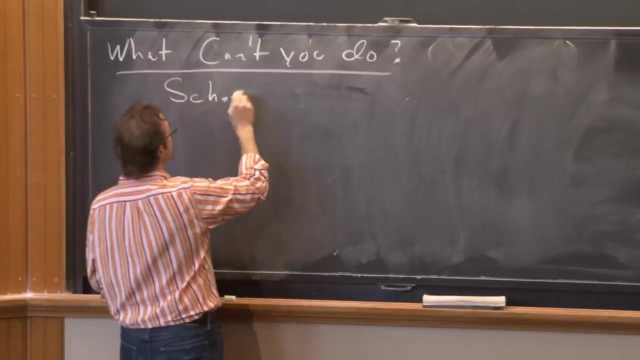 What can't you do? And to me this is among the more surprising things. So here's a really surprising thing. Remember that what we're doing here is going to be evolving a system forward with Schrodinger's evolution, And Schrodinger's evolution is linear. 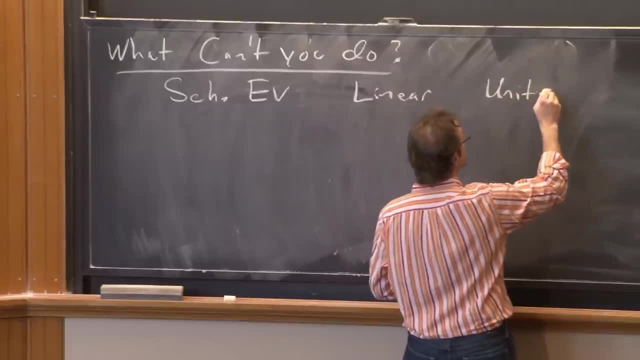 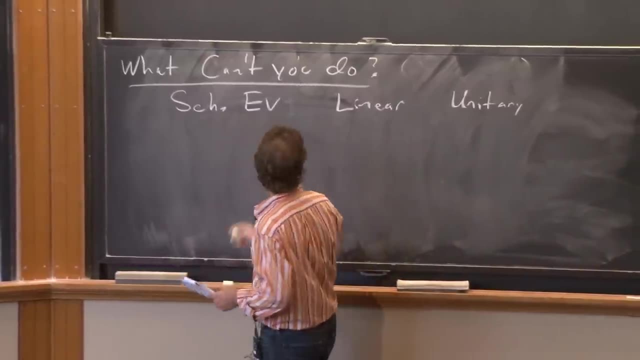 It respects superpositions, It's unitary, It preserves probability And it's well, let's just focus on that. It's linear unitary. It has lots of other properties: time reversal, invariant, unless you turn a magnetic field, which we do. 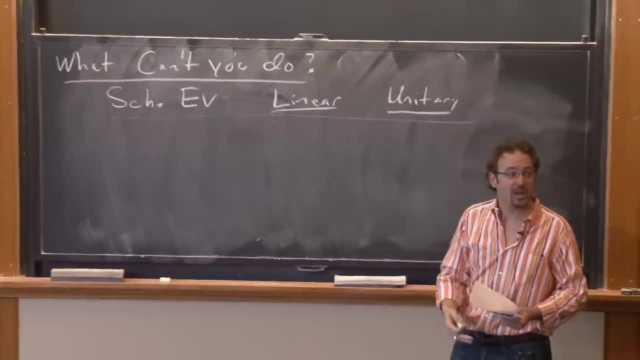 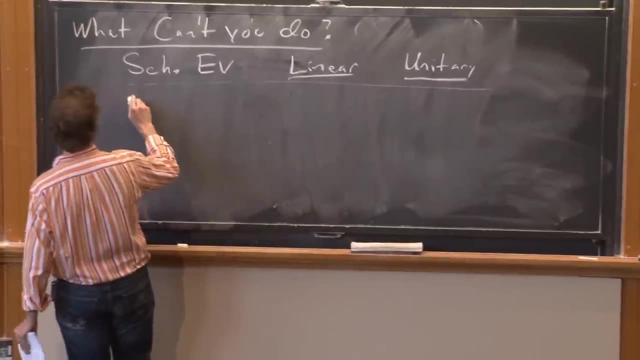 But in particular it's linear and unitary And those facts are going to constrain powerfully the kinds of operations We can effect on a quantum system. So in particular, when we look at just two qubits, there's a beautiful theorem that says there's no cloning. 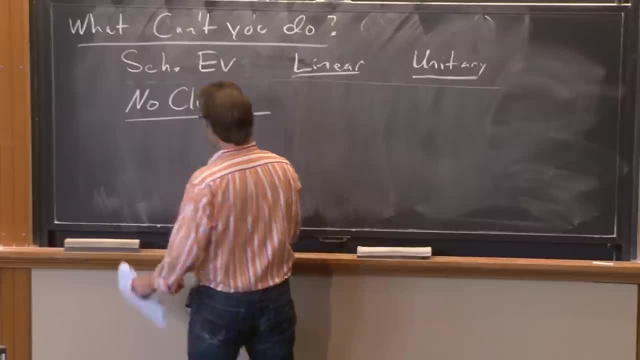 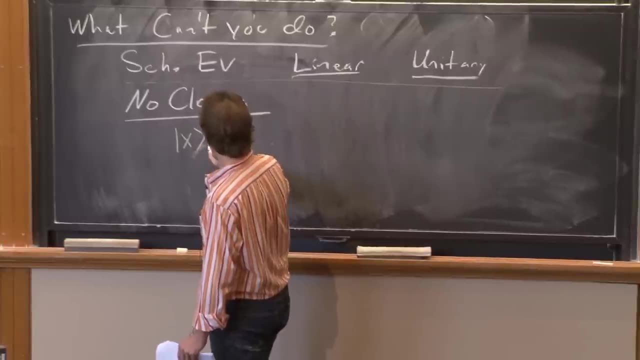 And here's what that means. No cloning theorem, which is pretty highfalutin for what it really is, says the following: Suppose we have a system which is input x, y And I want to build a machine that says: look, 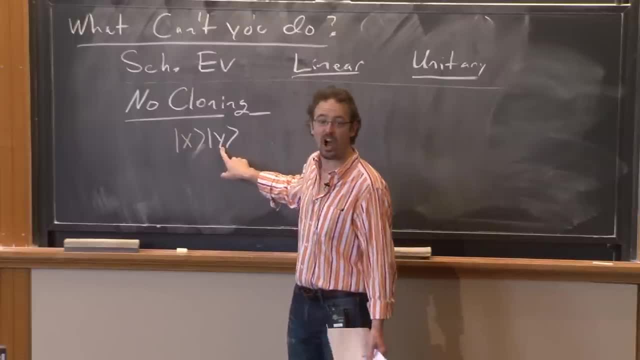 I've got this first qubit in the state x And what I want to do is I want to make a copy. I want to make another quantum system that's in exactly the same state as whatever x is. So you hand me a system where the first bit's 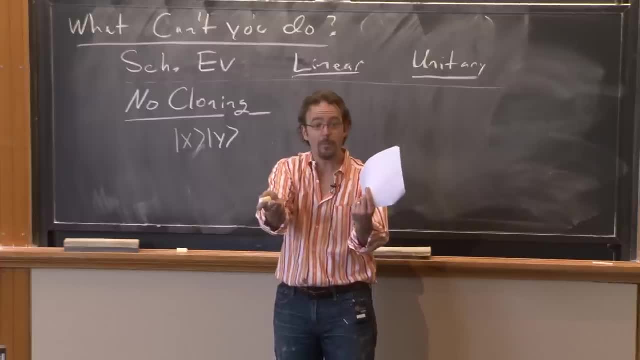 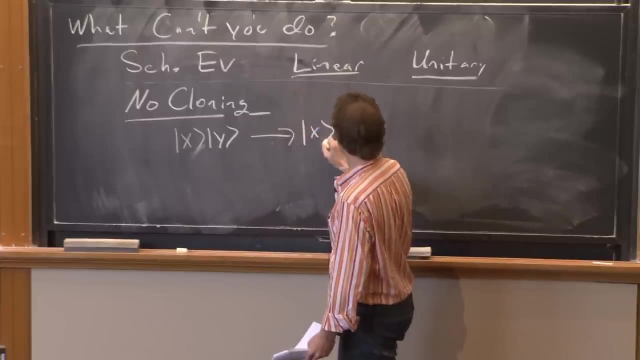 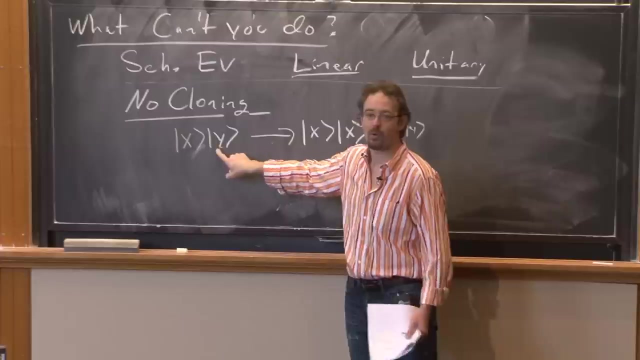 in state x, the second qubit's in state y And I want to make a copy of x And y is just the who cares what's in it. So I want this to go to x, x for all, y. So regardless of what data was in here, 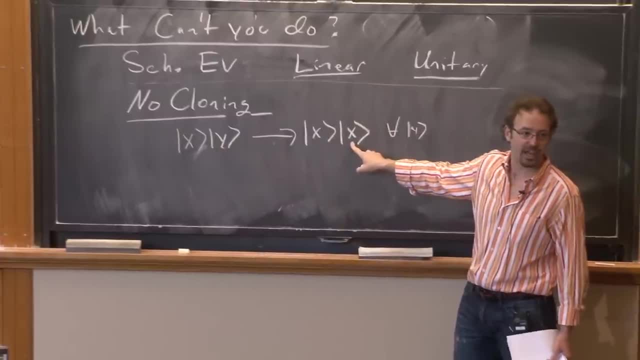 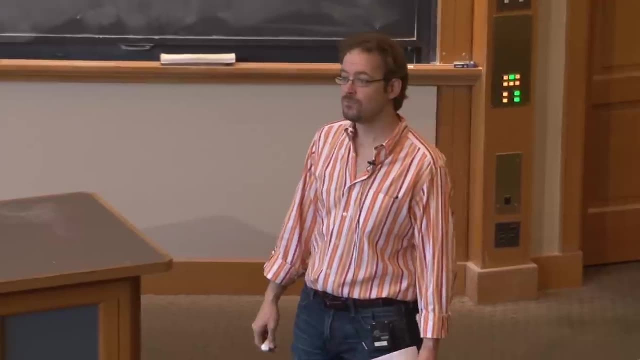 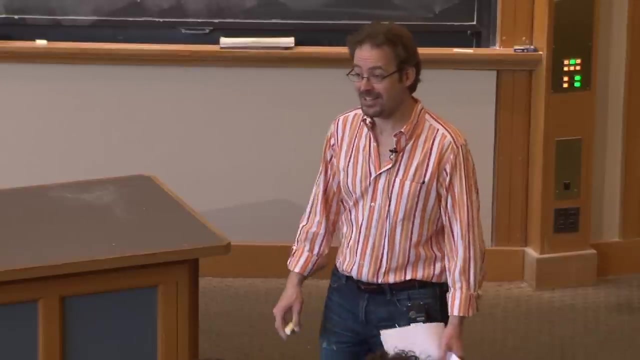 I want to overwrite that data and rewrite it, or that datum and rewrite it with x. Can you do this? No Right. Why? Because it would violate linearity. Excellent, It would violate linearity and also unitarity indeed. 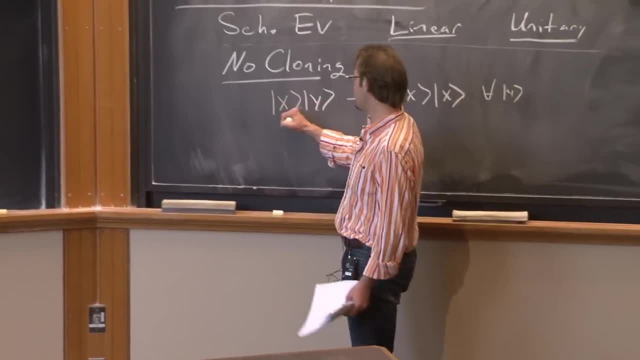 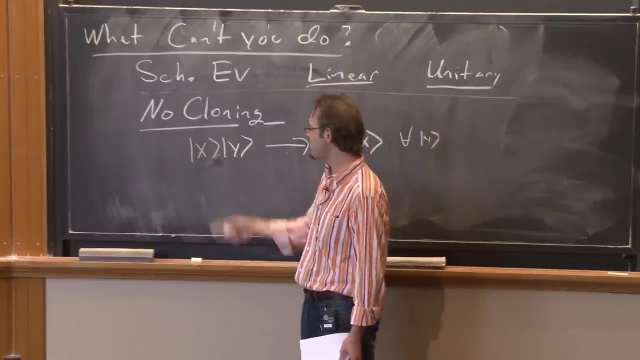 So to see that quickly, so it's easiest to see the unitary, I think, Well, it violates them both. But for unitarity, why don't you take a linear combination of these guys where the two states y are orthogonal? 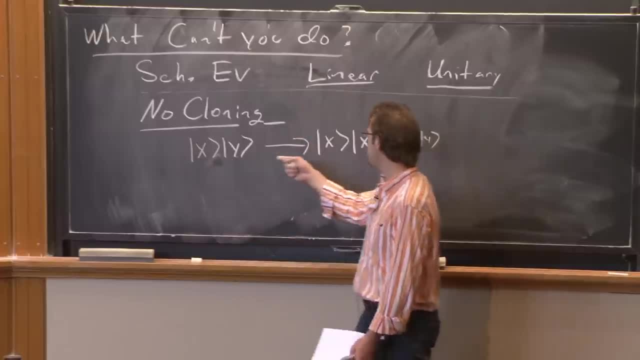 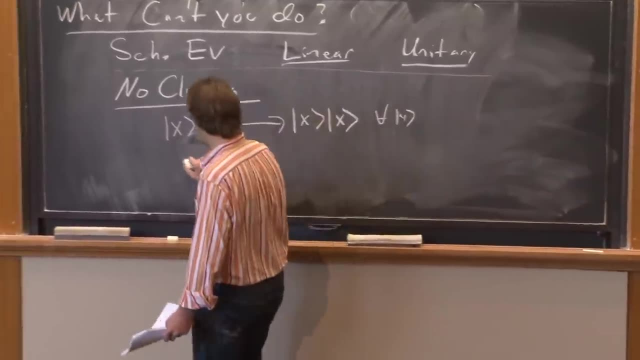 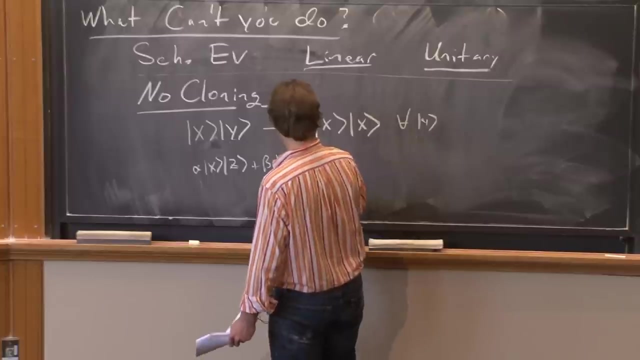 You take the norm squared, so you normalize it to 1. That linear combination, each one goes to x, x, where the coefficient is the sum of those two terms. So we have, for example, x, z, Alpha, x, z plus beta x. y goes to alpha plus beta x, x. 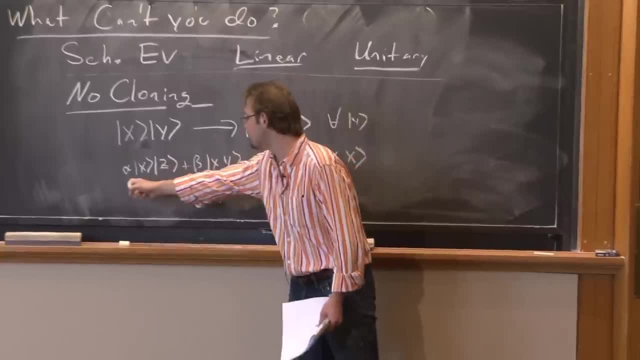 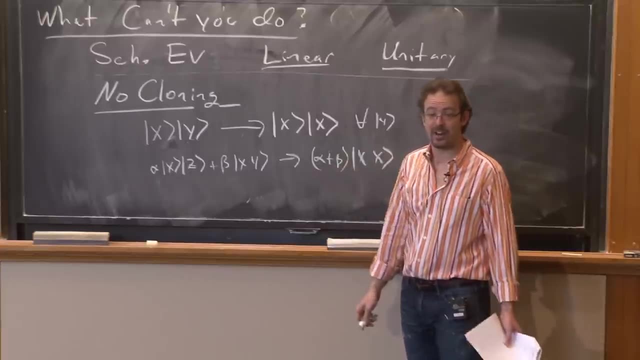 And that's really bad, Because if z and y are orthogonal, then normalization is alpha squared plus beta squared is 1.. But x, x, the normalization is alpha plus beta quantity squared is 1.. And in general that's not true. 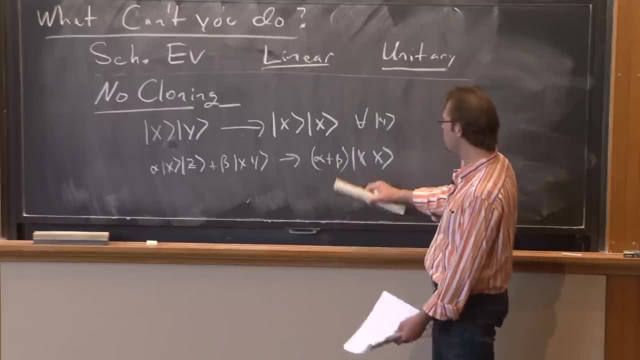 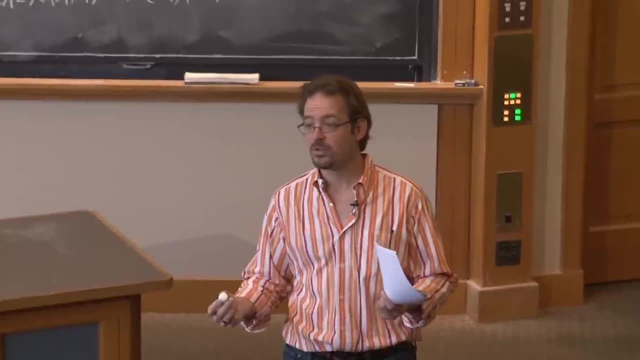 In fact this could be 0. So this violates linearity and unitarity rather badly. So you can't clone. This is really disturbing. That means if you have a quantum and you want to make a copy of it, you can't. 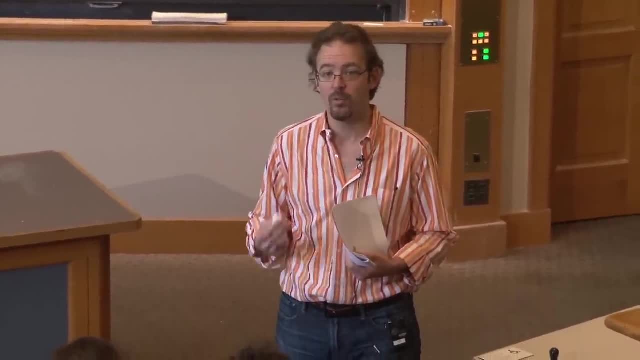 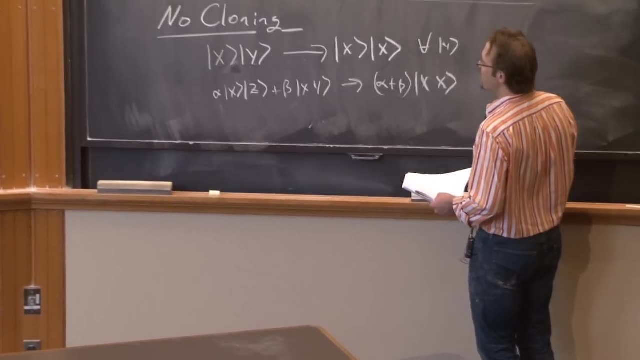 You can't ever make a copy of your quantum system. One copy, one chance, that's it. No cut and paste. So, as you can imagine, that pretty powerfully constrains things you can do. So a related thing here is that there's no forgetting. 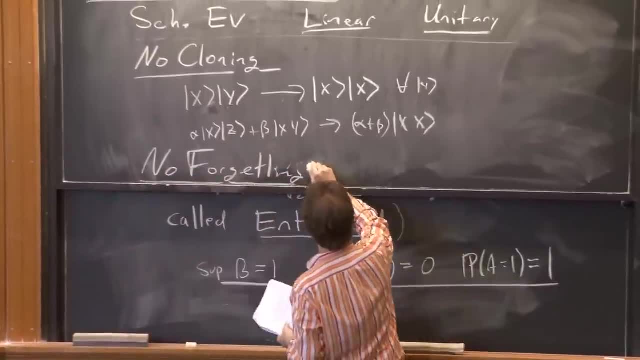 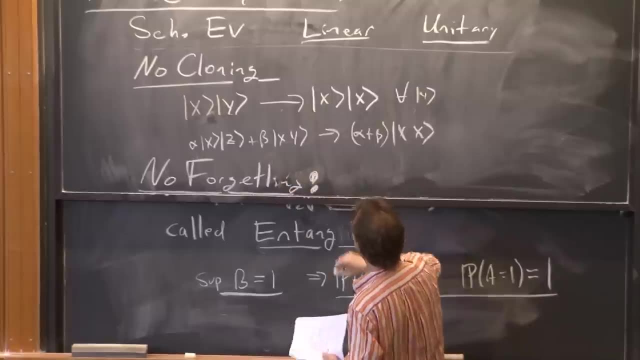 Quantum evolution is unlike an elephant. It is highly. it has a very well. it's like an elephant because it remembers very well. It never forgets anything And you can see that from this. This would be an example of forgetting. 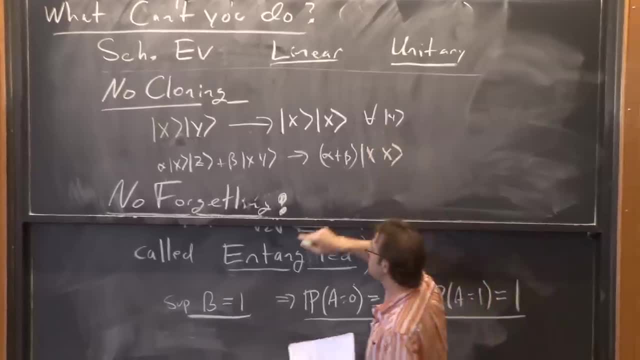 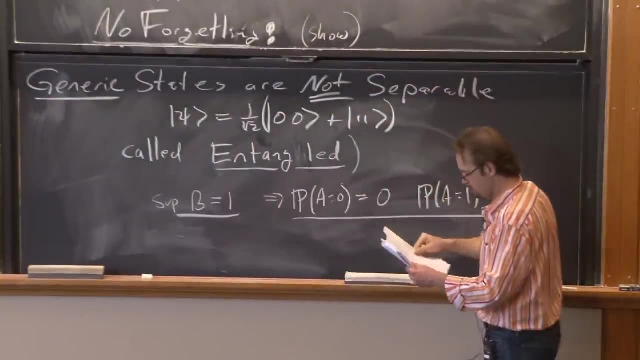 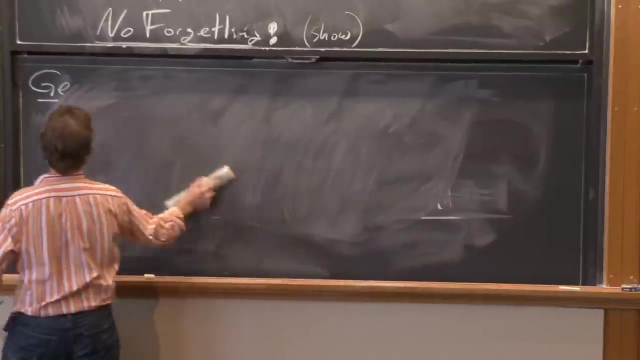 You forgot what was in the state y. You can't ever do that, So I leave this as a challenge to you to prove this show. It's a simple extension of the same logic. So what can you do? What you can do is you can entangle two qubits. 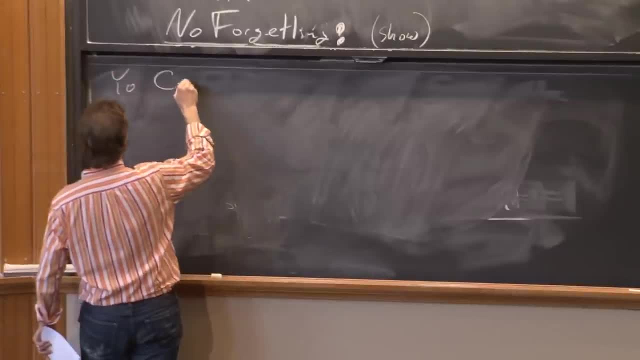 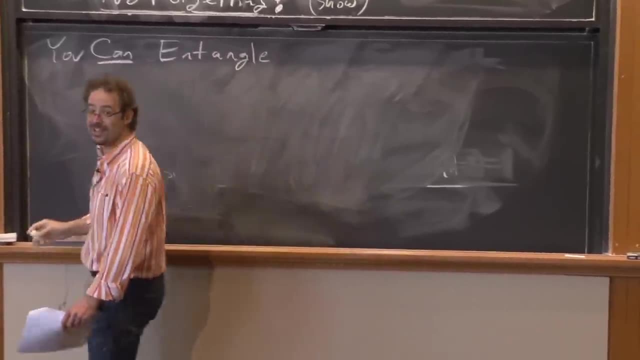 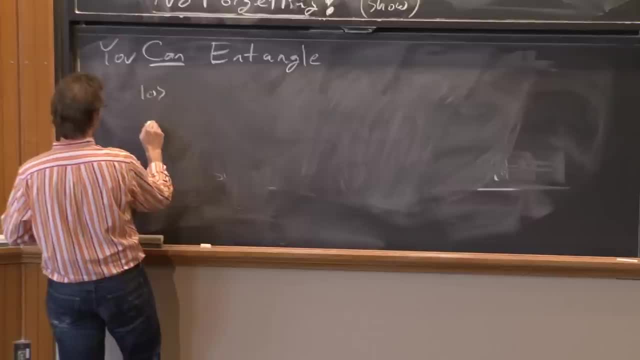 So you can entangle, And here's how you do it. Let's take the state 0, 0.. So we have two qubits, The first one's in the state 0, and the second one's in the state 0.. 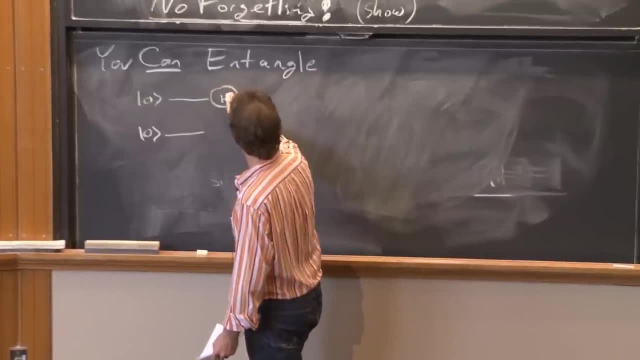 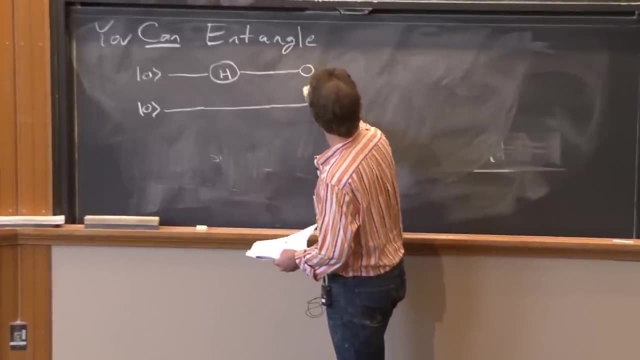 And now I'm going to do the following set of operations to it. I'm first going to impose a Hadamard operation on the first qubit and nothing on the second, And then I'm going to apply a controlled knot And I'm going to see what I get out. 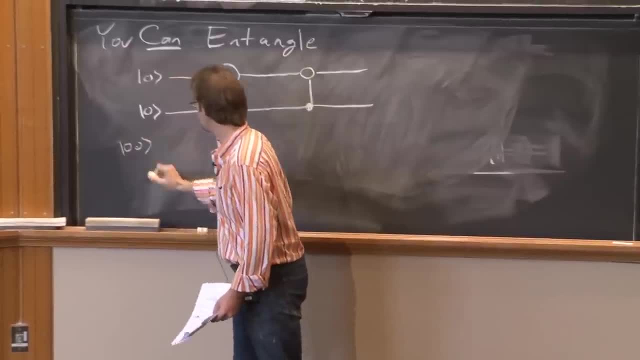 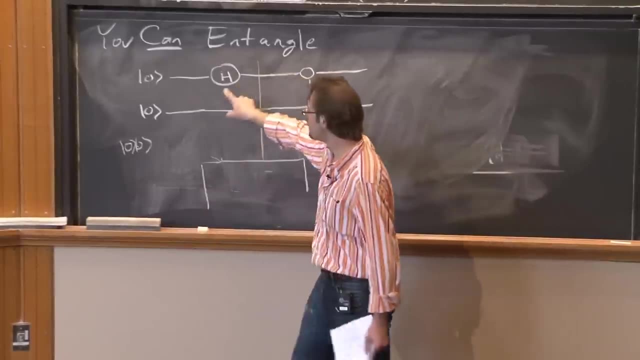 So the initial state is 0, 0.. I'll write this as 0, 0.. After I Hadamard, the state is well, the first bit is no longer in 0.. Hadamard on 0 gives me 0 plus 1.. 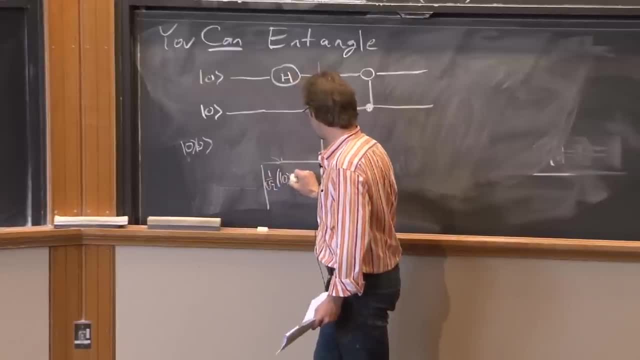 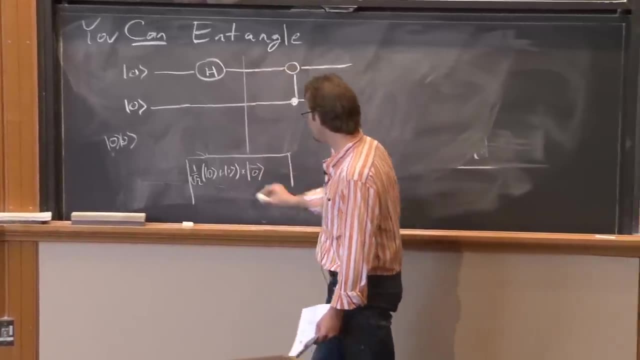 So this is now the state: 1 upon root 2, 0 plus 1 times 1.. Sorry, times 0.. OK, OK, OK, OK, OK, Also known as 1 over root, 2, 0, 0 plus 1, 0.. 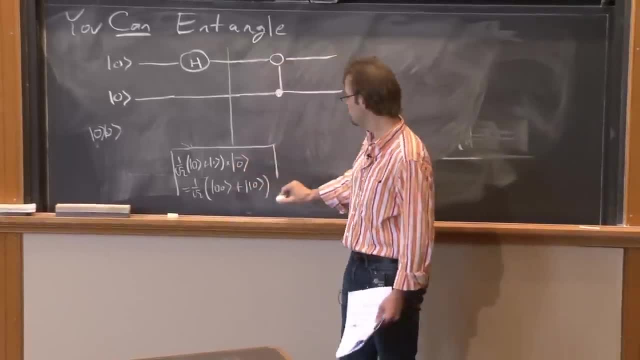 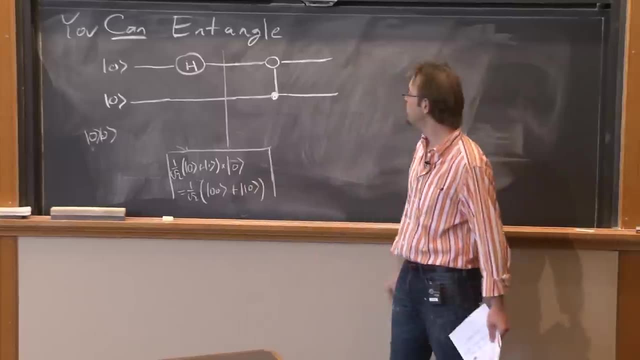 Now, is this a separable state? Yes, There, it is separated. And now I'm going to perform a controlled knot. And what the controlled knot does is it switches the second bit if the first bit is a 1.. So what is the state after we've done this? 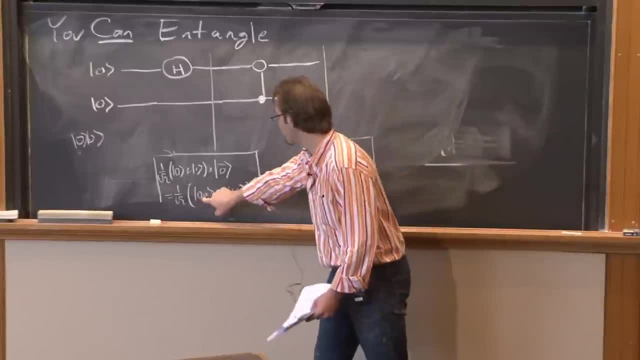 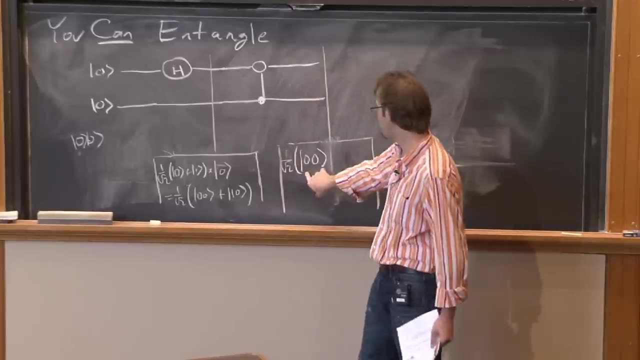 The state after we've done this is well, from the first term, 1 upon root 2, from the first term, 0, 0, what happens to that? when we control knot, Well, we knot this if this is 1.. 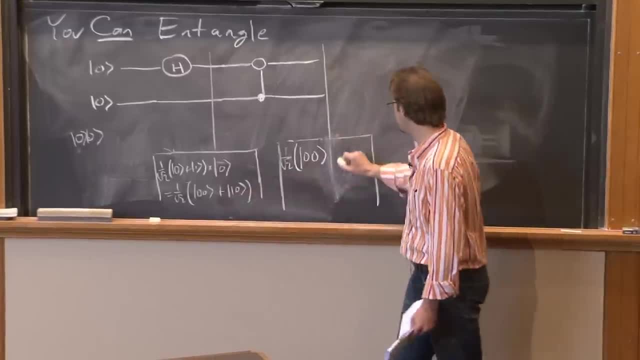 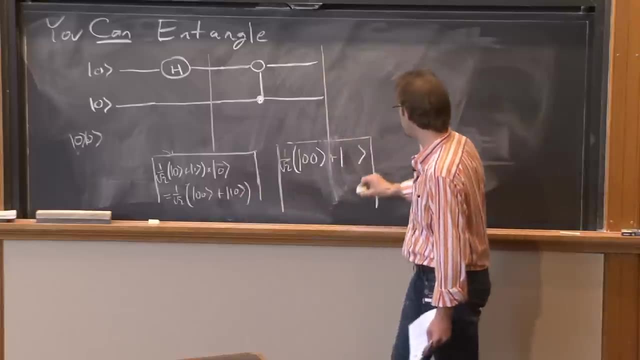 This is not 1, so we leave it alone. And the second term: 1, 0 plus. well, we flip this if this is 1 and knot if it's not. This is 1.. We flip it, We get 1, 1.. 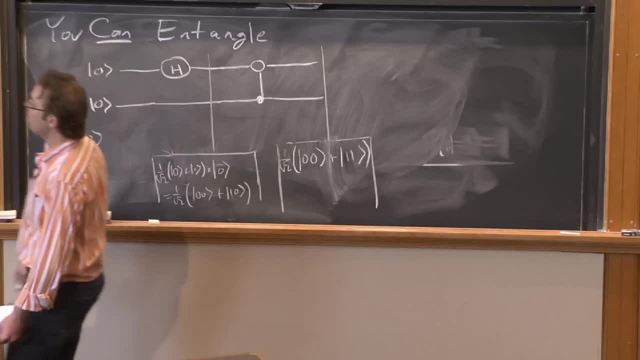 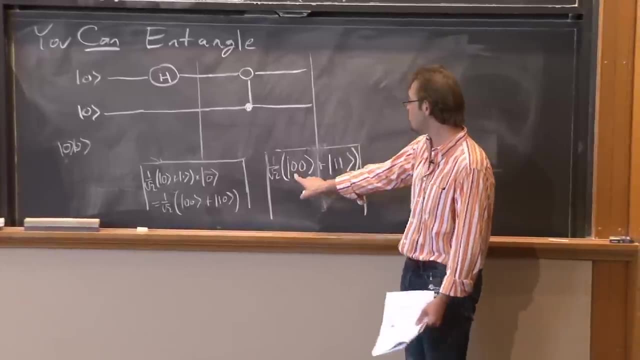 And now this is the prototypical entangled state that I think I just erased. But this is our entangled state. It's not separable. If I measure the first one, I know what the state of the second one is, which is to say it's entangled. 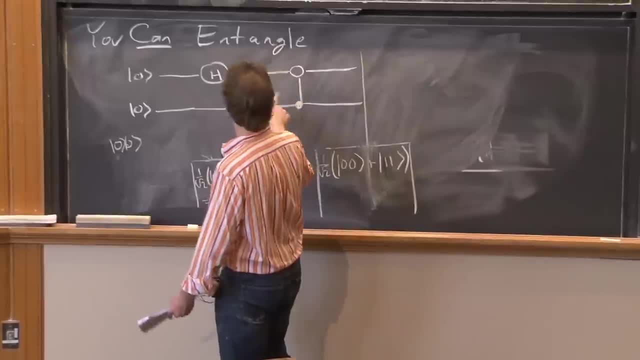 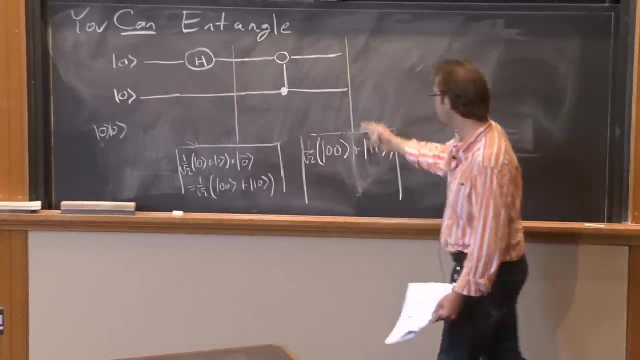 Cool. So by performing this series of operations, which is nothing other than a series of magnetic fields which I'm going to impose to the system, I've taken a state with initial condition 0, 0 and put it into an entangled state: 0, 0 plus 1, 1.. 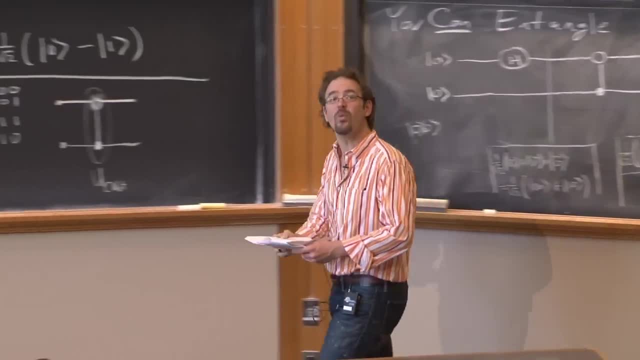 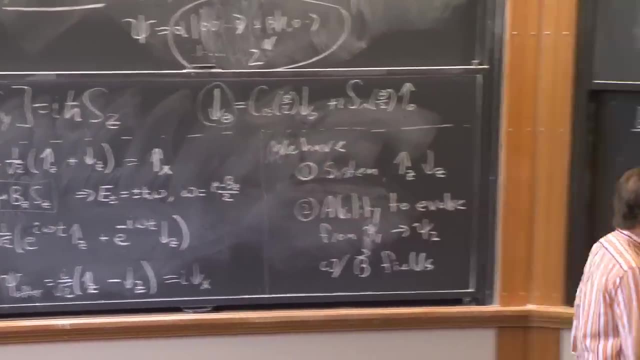 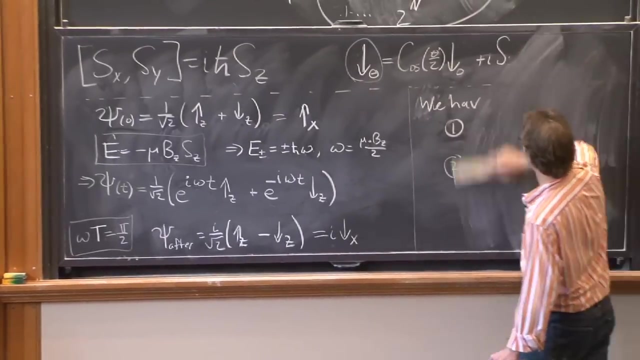 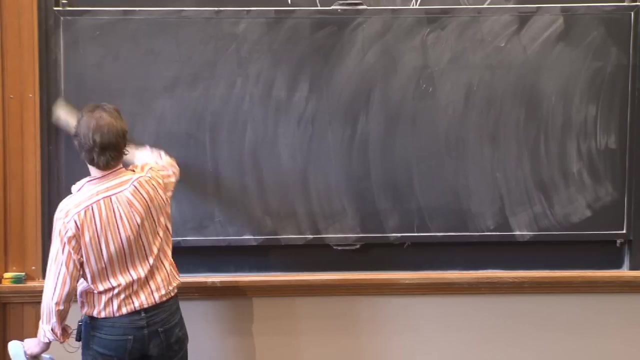 Cool And that's all we need for the first basic algorithm of quantum computation. So this idea that quantum computers might be able to do things faster than classical computers floated around for a while. It took a while for people to make that sharp And David Deutsch, who is a very entertaining and bombastic 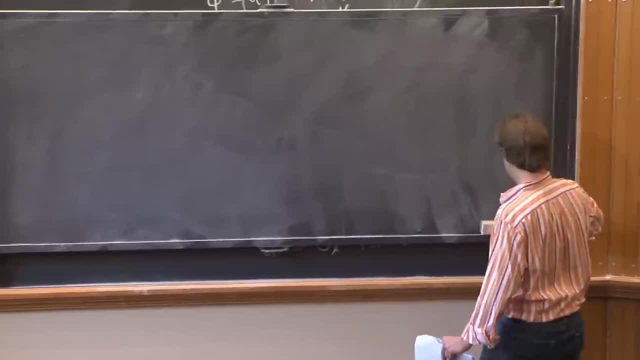 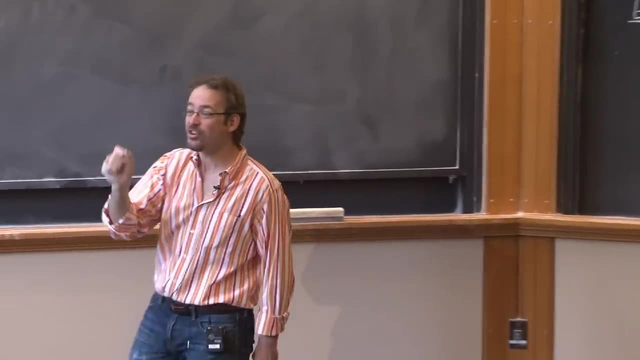 speaker and he wrote, I guess, several now pretty entertaining books on the topic And he sounds crazy. You listen to the guy talk and he sounds nuts. He sounds like he's just way out there. The thing he sees, just gah. 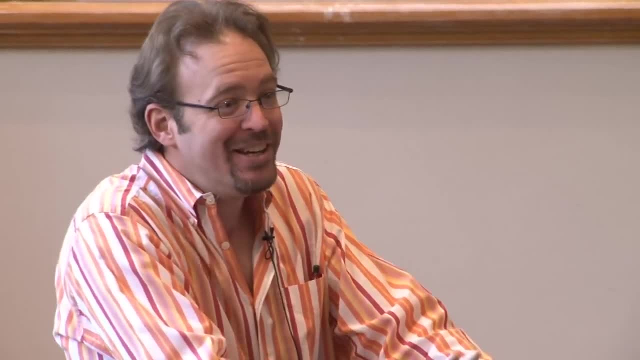 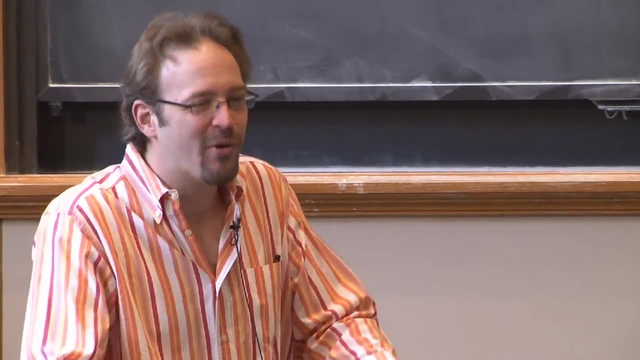 As a theorist. you listen to him and you're like go Just slow down there, buddy Right. And so for a long time I thought the guy, because I only knew his sort of public persona. I thought, yeah, he's a little bit crazy. 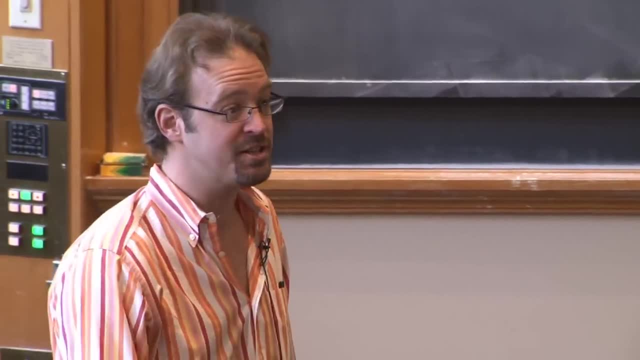 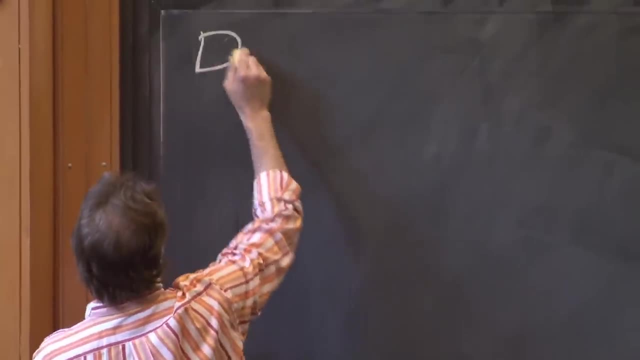 I'm not exactly sure, And this is why everyone thinks he's such a damn genius, Because this is beautiful. So here's: I don't know how he came up with this, but he's clever. So here is what's now called the Deutsch. 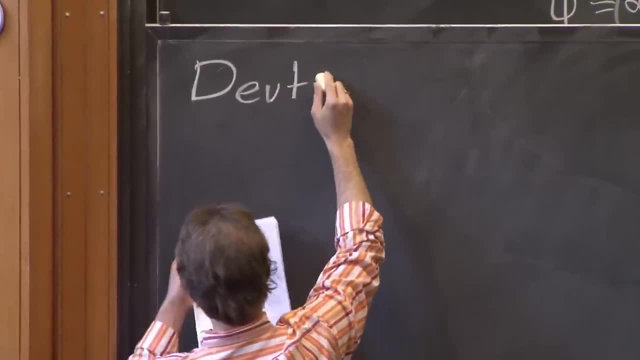 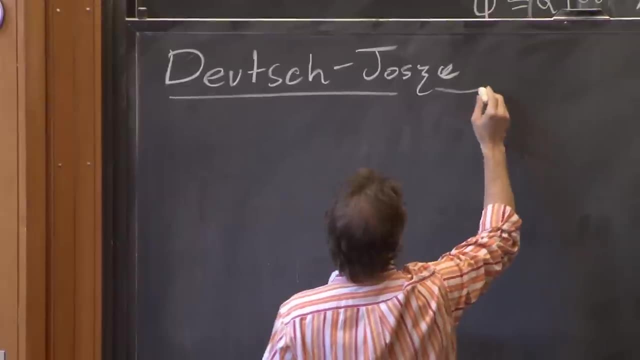 and it's really the one-bit version of the Deutsch D-U-T-S-C-H JOSA algorithm. So there was first an algorithm by Deutsch. It didn't quite do it. It was supposed to do it. Then it was improved together with JOSA. 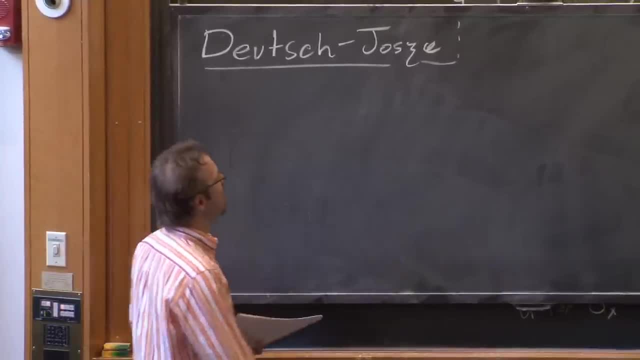 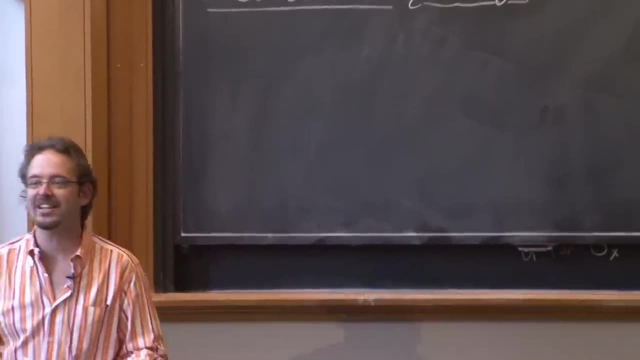 and they made an n-particle version and then everything was awesome. But here's the Deutsch-JOSA algorithm And what it is: it's a series of rules for how to make a quantum mechanical system evolve so as to affect the calculation you wanted to calculate. 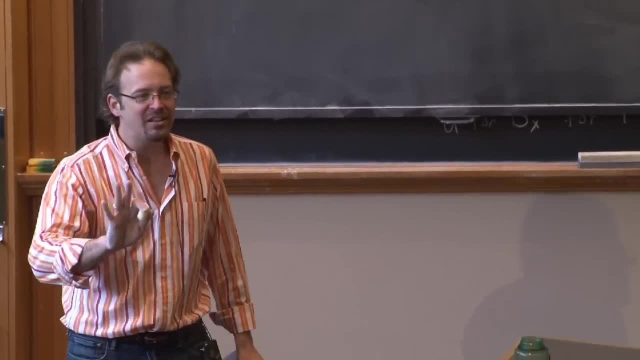 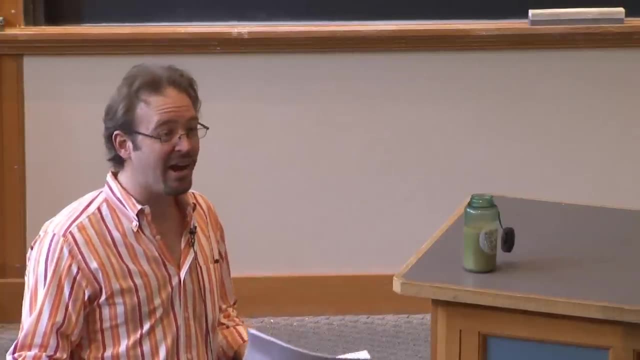 So you have to grant to begin, you have to. let me pose a problem to solve that can be solved in this fashion, And this problem is going to sound a little contrived And in fact it's going to sound a little contrived. 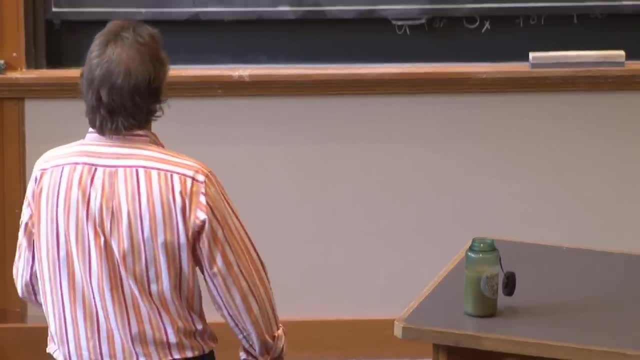 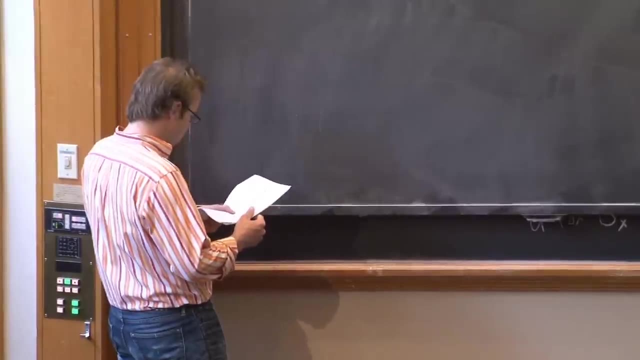 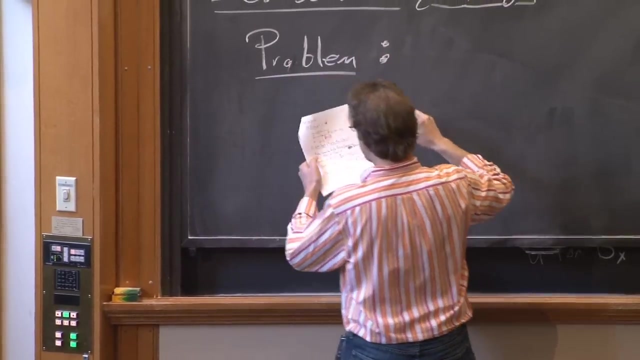 In fact it's wildly contrived. It was contrived so it could be solved in this fashion, But it's one that pre-exists- the algorithm itself- so it's not quite as ridiculous. So here's the problem. So the statement of the problem is that someone 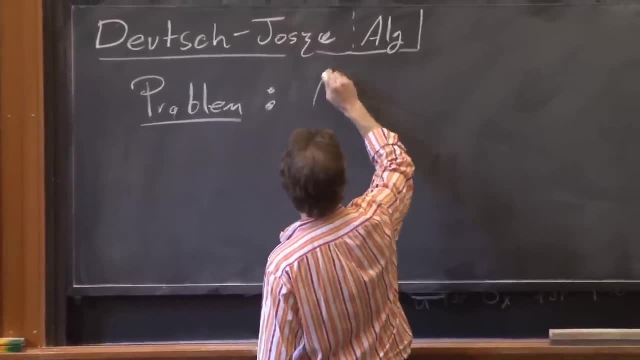 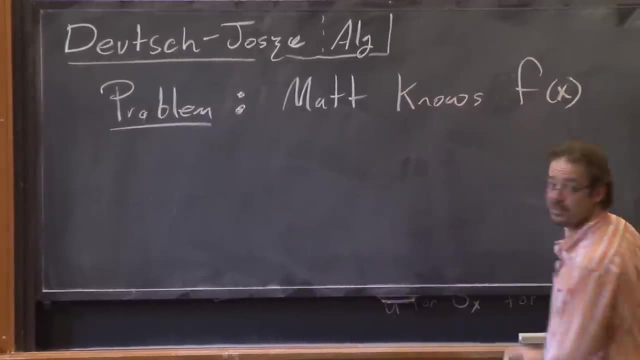 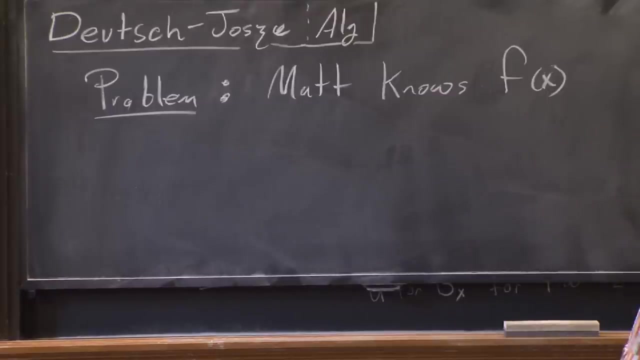 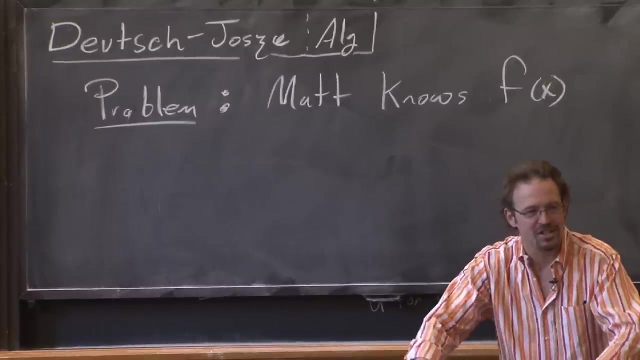 has a function f of x. So let's say Matt knows a function f of x. Now the thing is, it's extremely expensive to evaluate this function f of x. So the way you evaluate it involves putting 20 kilo mirrors in superposition states with each other. 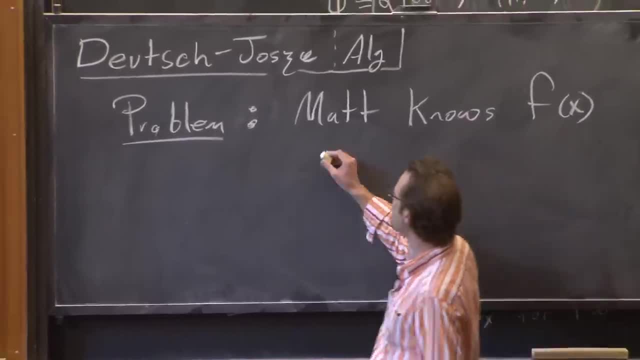 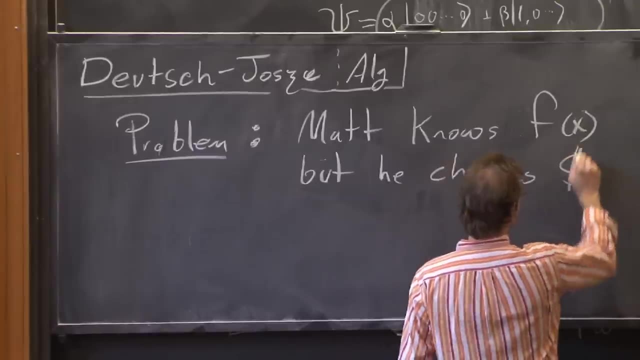 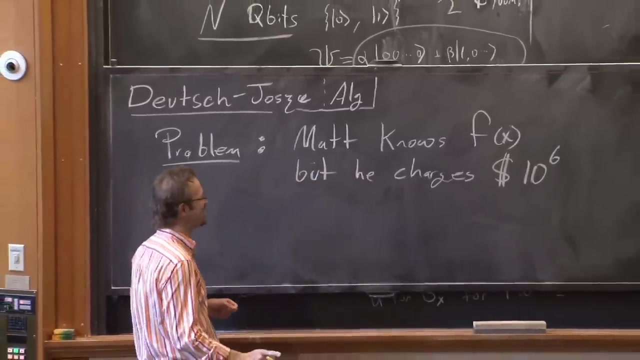 You have to run a whole experiment And it costs a lot of money to run. So he charges $1 million in order to solve this. Thank you, You guys are not quite old enough. So he knows a function f of x and he charges $1 million. 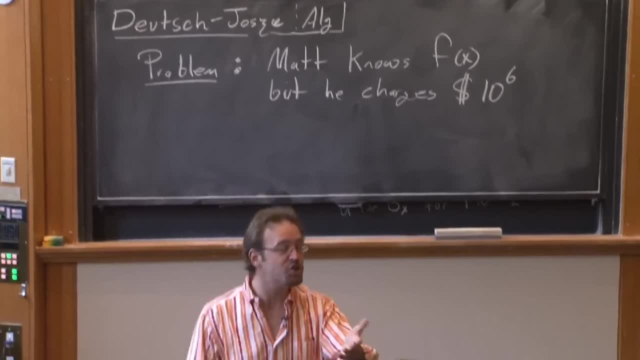 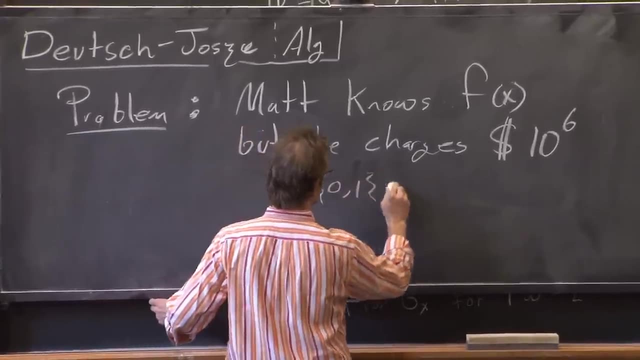 in order to evaluate the function. You say: hey, Matt. well, look, I know this is a function. I should tell you: f is a function that takes a single bit- 0 or 1, to another single bit- 0 or 1.. 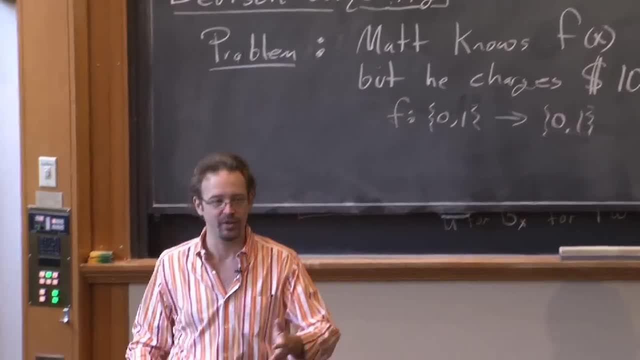 So it sounds like how hard could this possibly be? But in fact it's a very hard function to evaluate. So you say, hey, Matt, what's f of 0?? And he's like give me a million bucks. 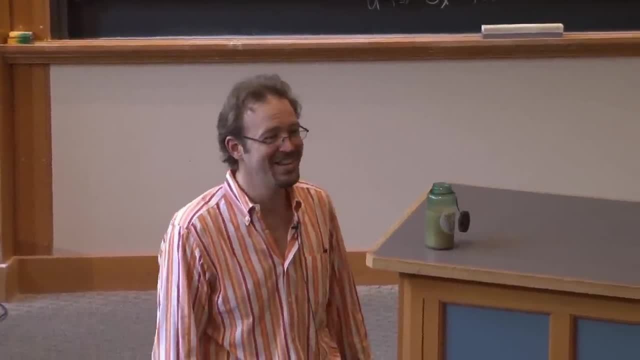 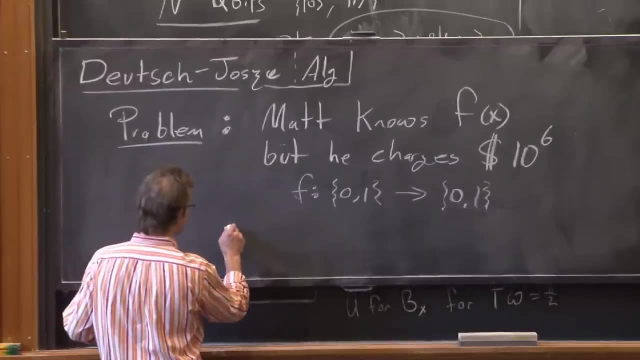 And you give him a million bucks And he's like 1. You're like, damn, that costs a lot of money. OK, and now here's the question. So this is not yet the problem. The problem is this: 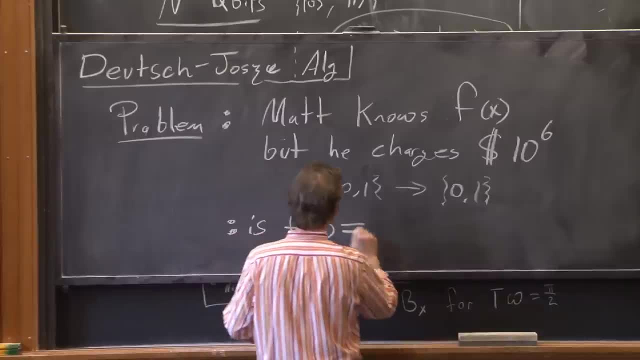 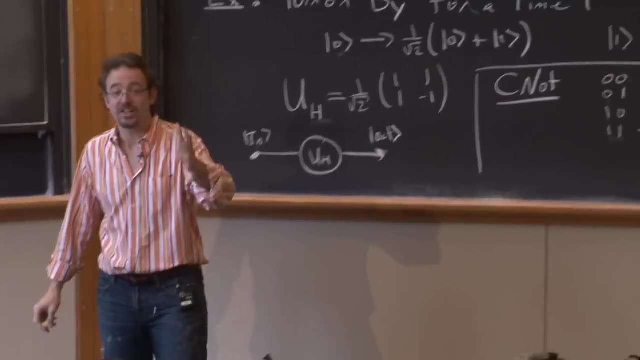 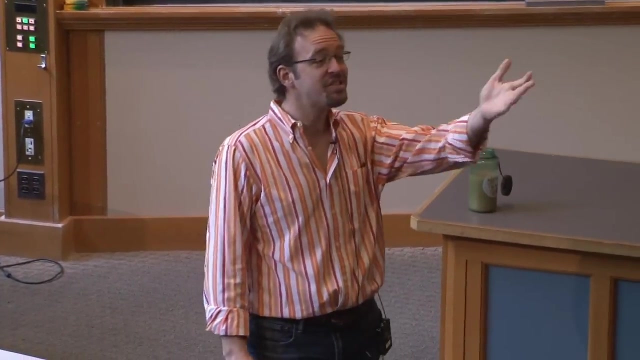 Is f of 0 equal to f of 1 or not? OK, so f of 0 is either 0 or 1.. f of 1 is either 0 or 1.. Are they equal to each other? So this is easy, right. 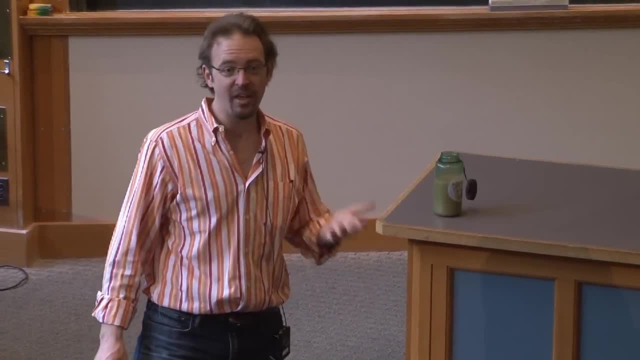 Classically. this is stupid. You've calculated the function f twice. You evaluate f of 0, and you get a number. You evaluate f of 1, you get a number. You look at your piece of paper, You say it's either the same or different. 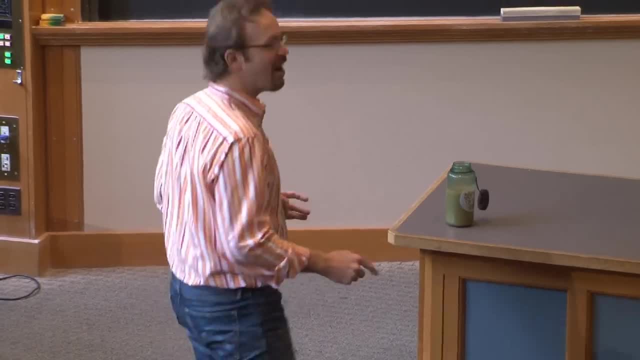 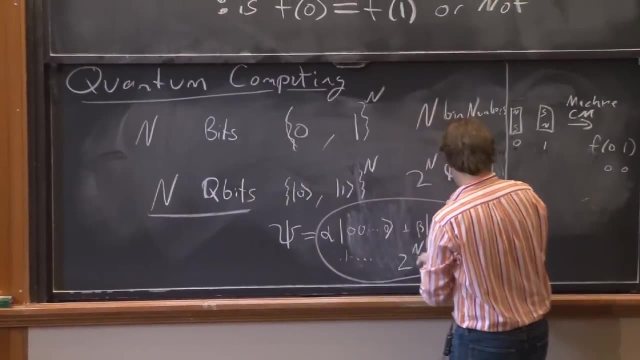 How much does that cost you? Two million bucks. Better have good funding. So this is an expensive. And here's what Deutsch and Josa have to say, And this is really Deutsch. at the beginning It's all really quite spectacular. Deutsch says actually: I tell you what. 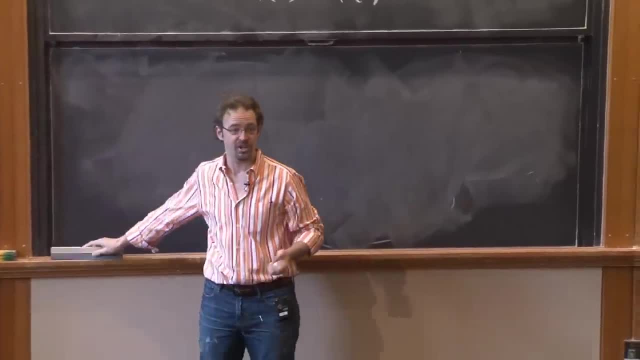 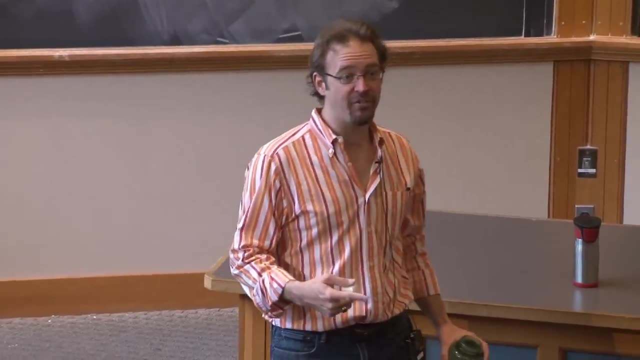 Give me a million and a half and I'll do the computation and give you the answer. At which point you think, like I did previously, the guy's clearly raving. In fact, he's going to make a profit And here's how he's going to do it. 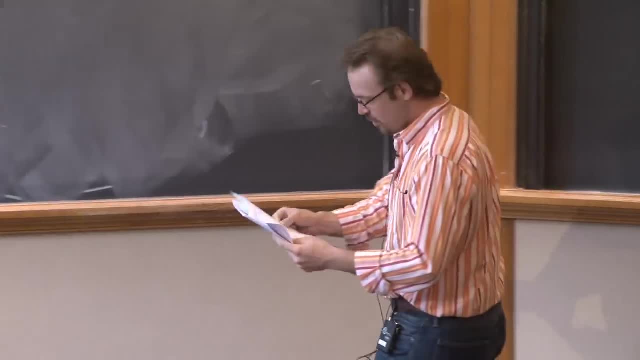 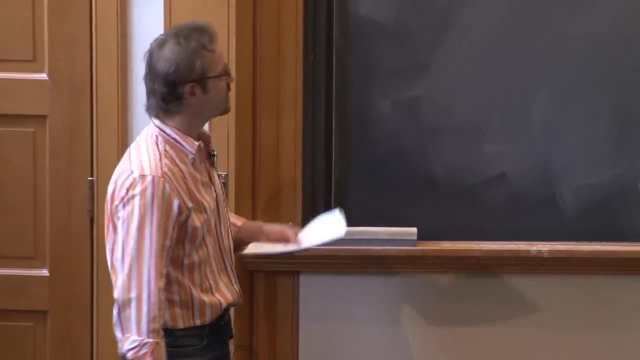 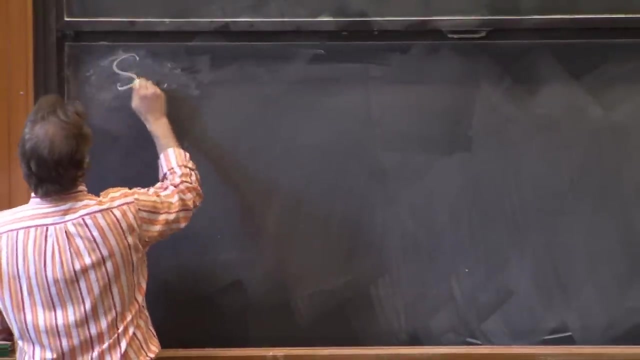 He's going to build not a classical computer but a quantum computer using quantum interference and entanglement to do this calculation with one evaluation. And here's how it's going to work. The first thing we have to do is a preview or, sorry, setup. 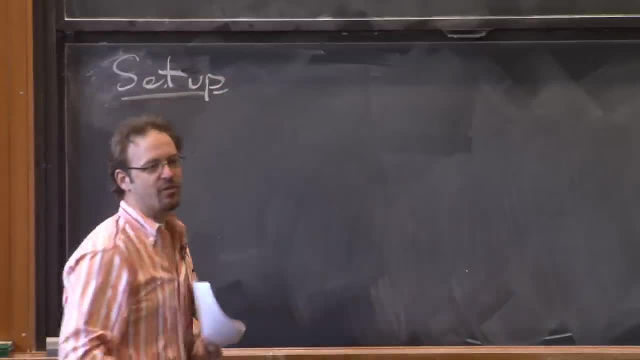 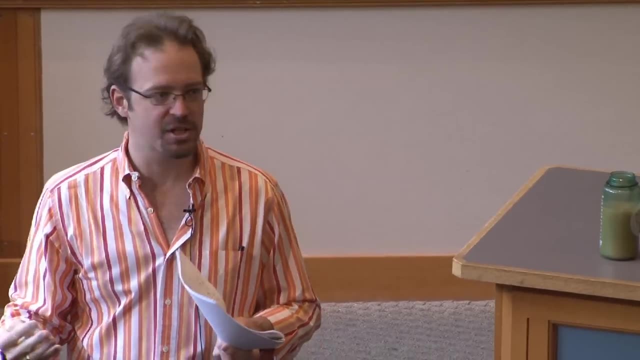 In order to do this calculation, you need two things. First off, you need Matt to be able to evaluate his function In a way that respects quantum mechanics. So, in particular, Matt had better be able to do his experiment if I give him a superposition. 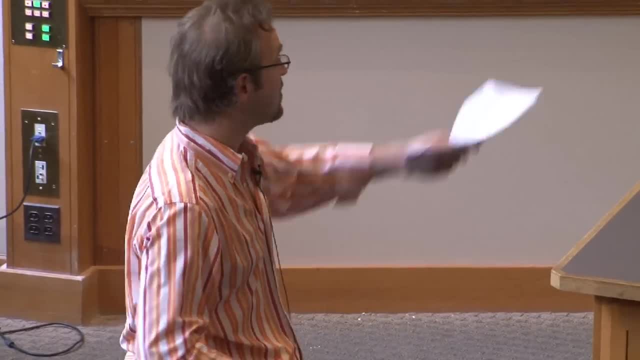 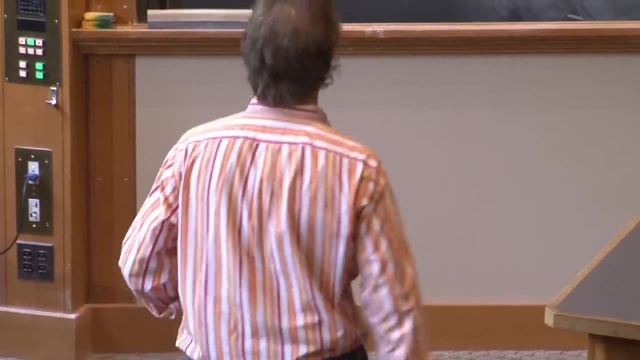 So he'd better be able to effect the calculation in a quantum mechanical way, the same way that we implemented a- not quantum mechanically, or the controlled not quantum mechanically, or the Hadamard with some set of magnetic fields. He must be able to implement it quantum mechanically. 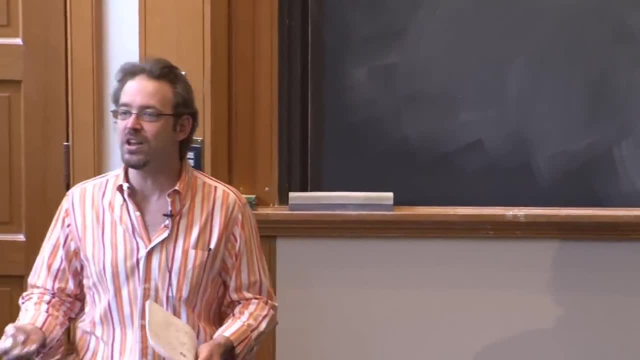 Otherwise it's not an interesting function. And let me just point out that any function you can think of can be implemented quantum mechanically. because you are quantum mechanics. You're just not elegant. implementation, no offense, You're just not elegant. You're just not elegant. 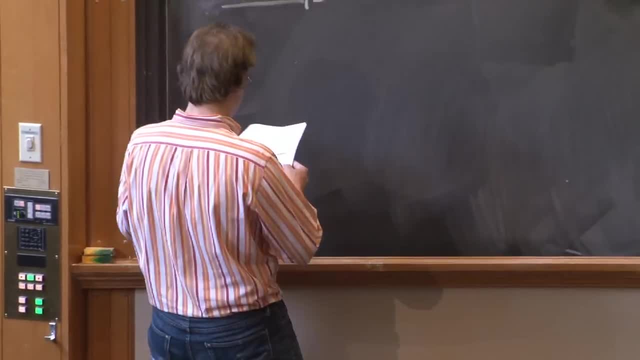 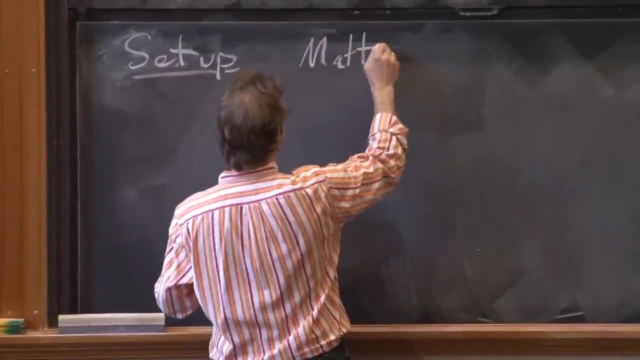 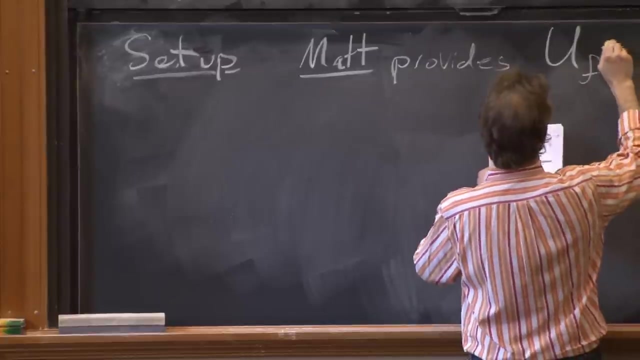 You're just not elegant. You're just not an elegant implementation of the quantum mechanical computation. So what I want so setup is Matt needs to be able to give me Matt provides a unitary transformation, unitary operation, u sub f that takes two qubits, x and y. 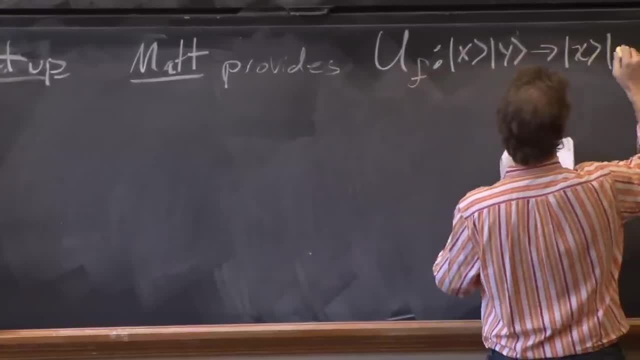 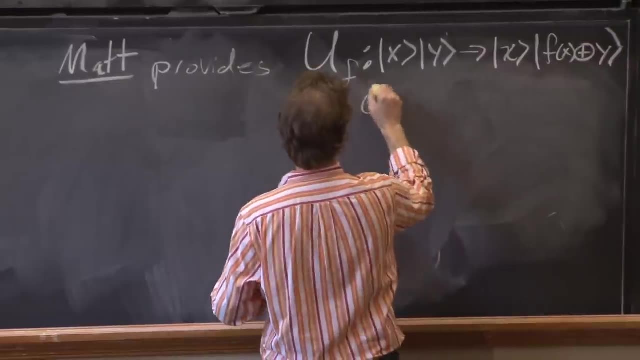 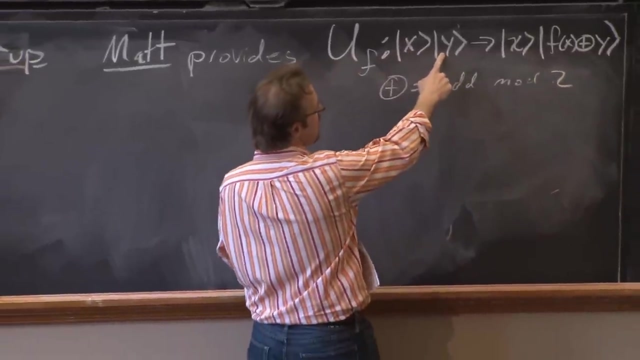 to x and f of x plus y, Where what this means- f of x plus y, f of x plus y is plus- is addition mod 2. So what this says is: if y is 0, then this gives me f of x plus 0.. 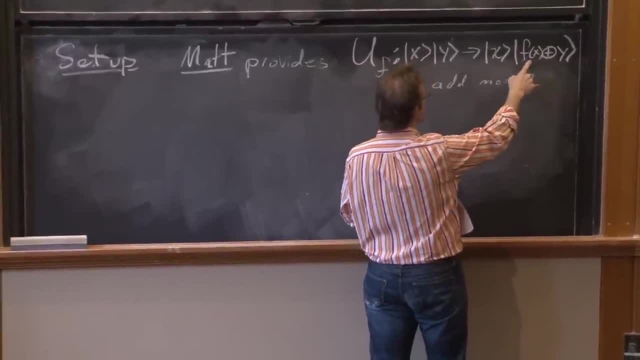 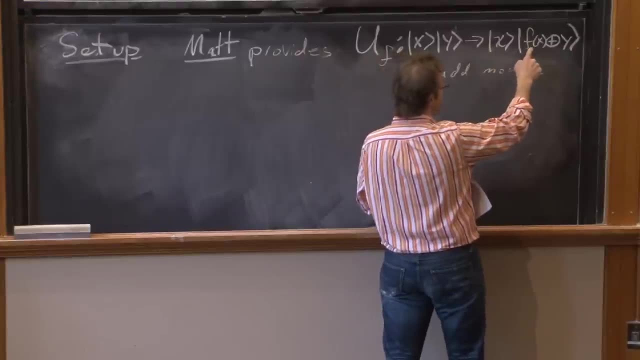 If f of x is 0, that's 0 plus 0, so that gives me 0.. If f of x is 1, this gives me 1 plus 0, that's 1.. On the other hand, if y is 1,, then this gives me. 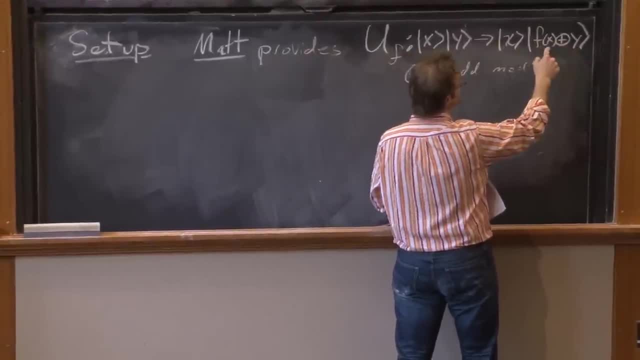 if f of x is 0,, this gives me 1 plus 1, which is 0.. And if f of x is 0,, this gives me 0 plus 1, which is 1.. Everyone cool with that OK? 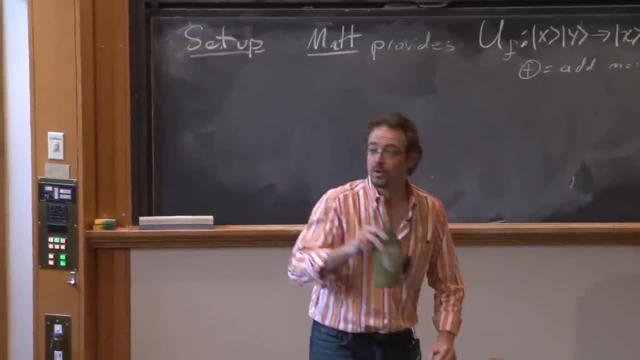 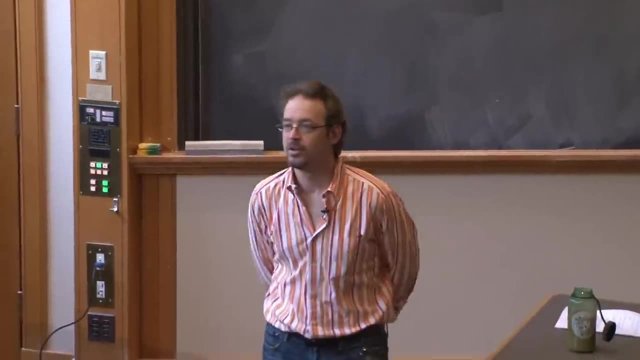 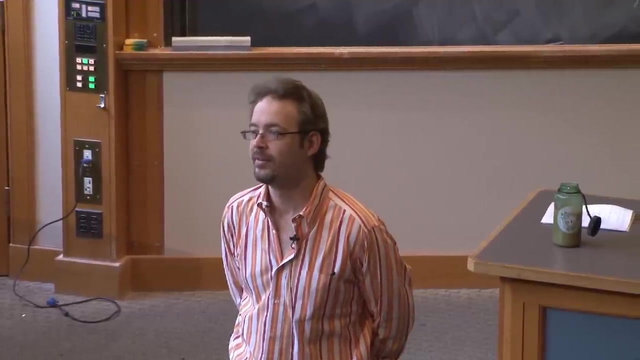 Yeah, It's not really a question, but how do we know that nature can actually play a part? How can we know that nature's actually proof that quantum mechanics can basically solve any problem? I mean, what if? what? nature is just an approximation? 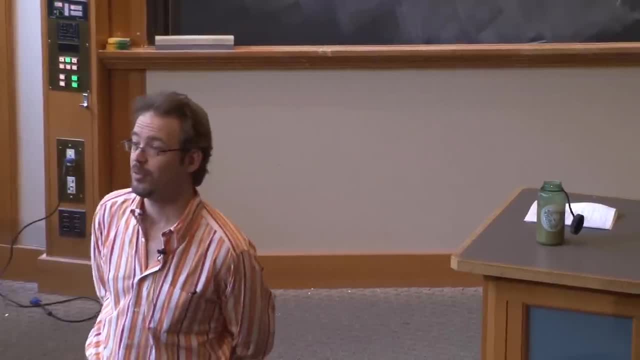 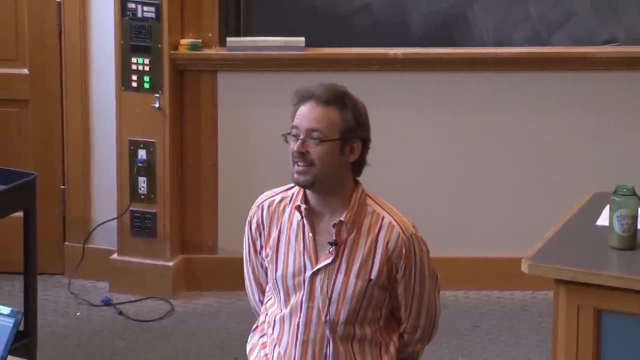 You mean? what if quantum mechanics is only an approximate description of the? No, I'm sorry, No, sorry, Like what if quantum mechanics like in elements irrepressible? Yeah, It's just an approximation of quantum mechanics. 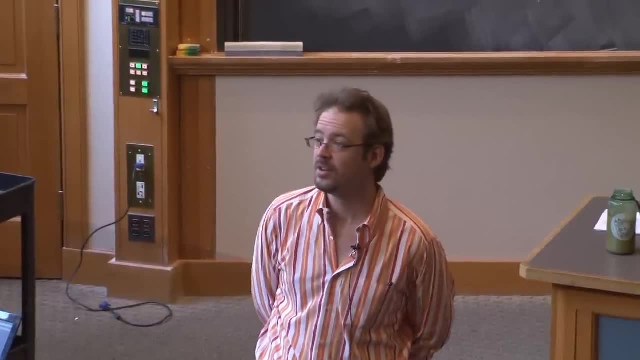 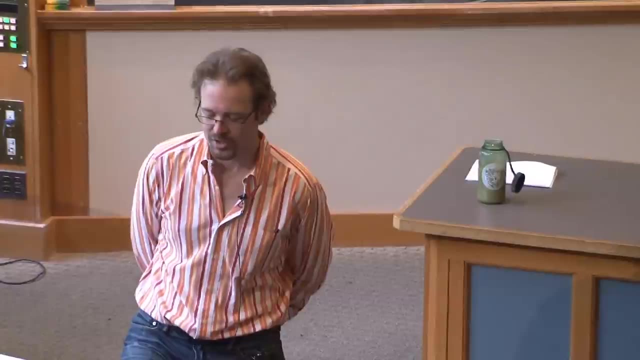 It's inescapable. It's just an approximation of the problem. It's just a really really good problem. Yeah, this is an interesting question, So it's tempting to think that this is a philosophical question, but it turns out not to be in a way that will be made. 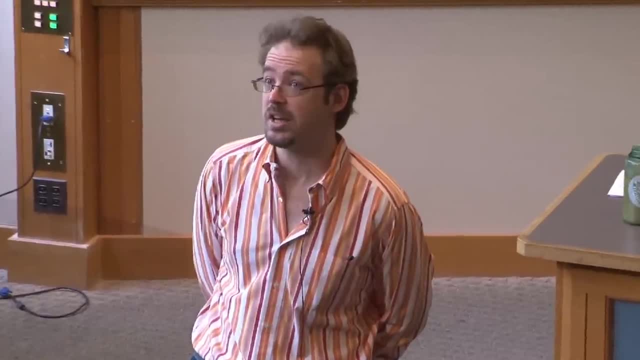 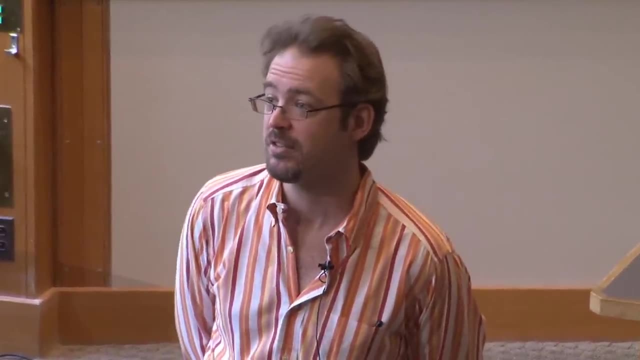 sharp in about 10 minutes with Bell's inequality. But a good answer. a complete answer to that question remains open, and I think it probably always will. But let me rephrase the question slightly and tell me if this is an accurate statement. 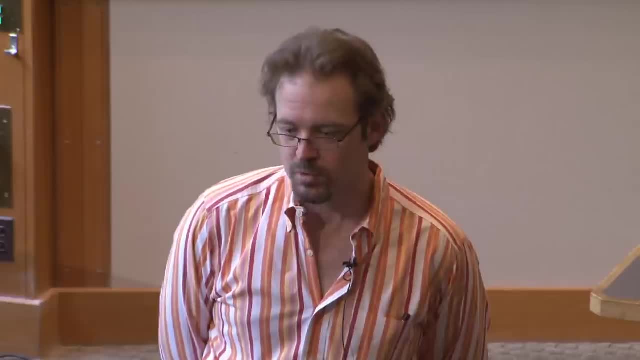 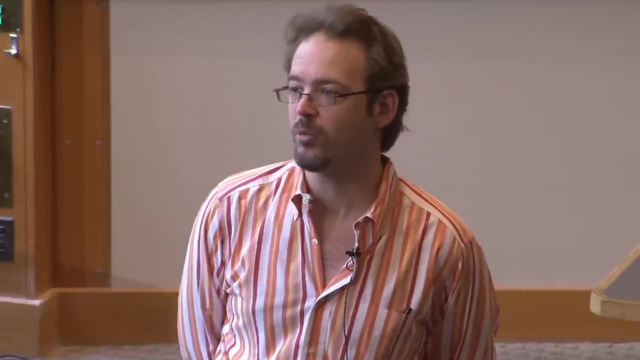 Look, At the end of the day, what we're doing is we're going to develop a model where quantum mechanical calculation does something in particular, And that may or may not be a good model of the real world And, in particular, whatever the actual thing, the actual system, 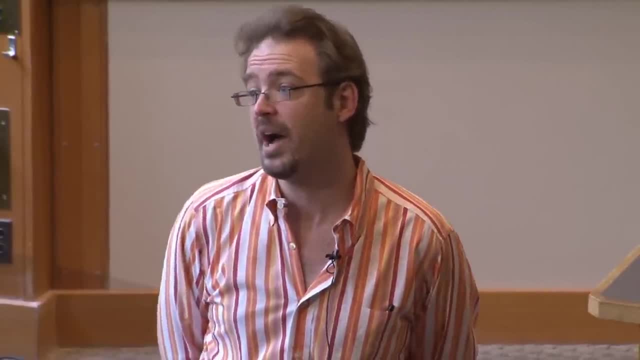 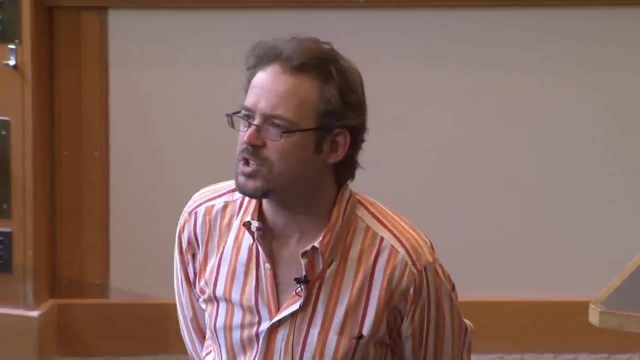 that we're studying does may or may not be well described by that quantum mechanical model. So can we check whether or not it is? And is that more or less the question? Yeah, it's a hard thing to make, So the problem is: 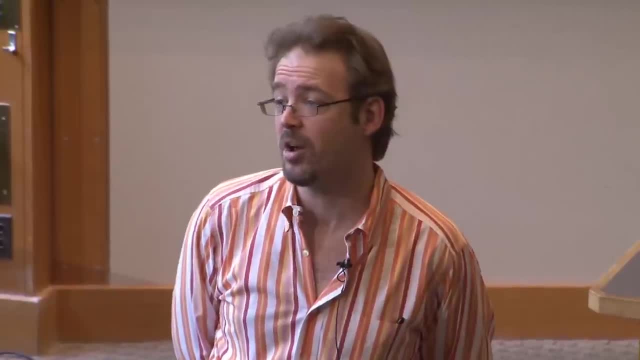 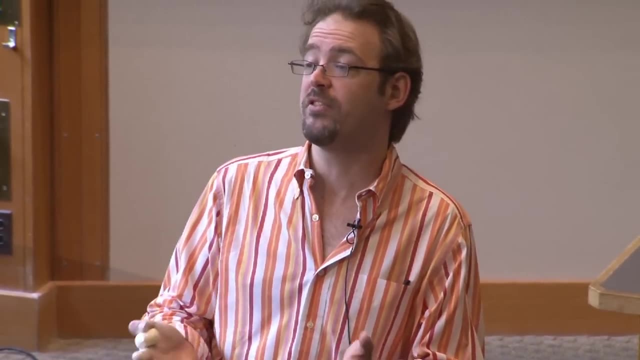 All we can ever do is say that our model is a good model or a bad model. On the other hand, we can do the following, And this is the really neat thing, You might say: look, underlying quantum mechanics is going to be something more fundamental, that's. 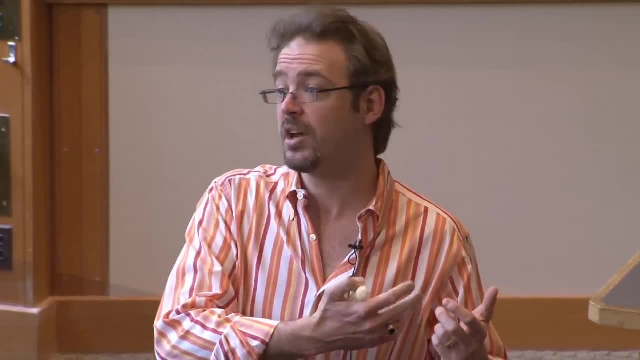 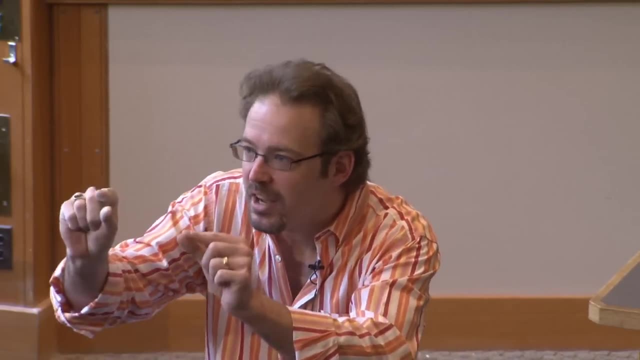 going to lead to slightly different results, in exactly the sort of situations where we're going to care about quantum computation with large numbers of bits And if you tell me just a little tiny bit about what properties that underlying description will have, that becomes an empirical question. 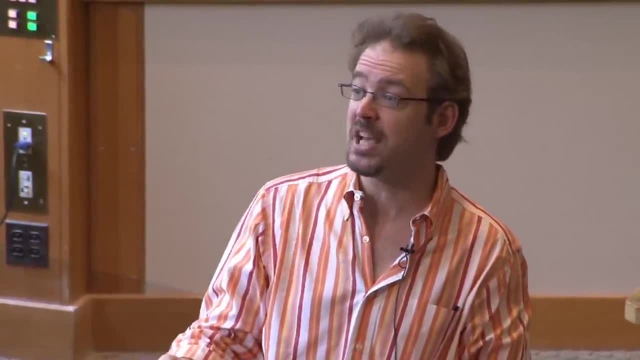 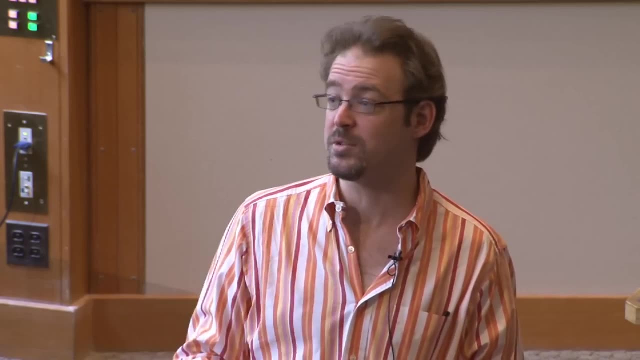 So, for example, if you say: look, I suspect that underlying the quantum mechanical probabilities is some classical probability distribution over a hidden variable that you have not actually measured, And what we're going to find out is that we can rule that out experimentally, 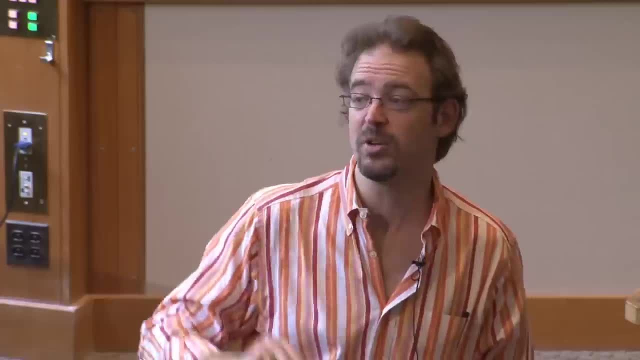 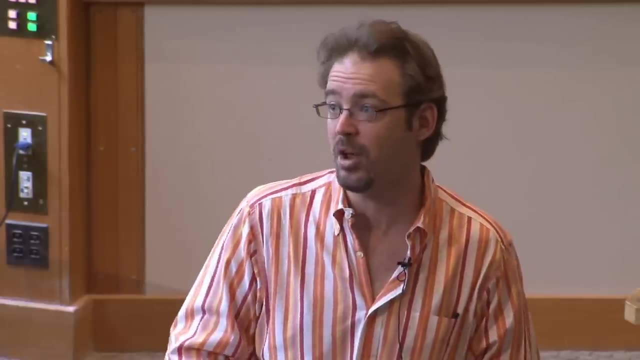 Just that extra little assumption that there's an underlying hidden variable, a secret probability distribution on some variable that we just haven't observed yet. That is enough information about the system to rule out that model amazingly. So I think we'll never have a full answer to your question. 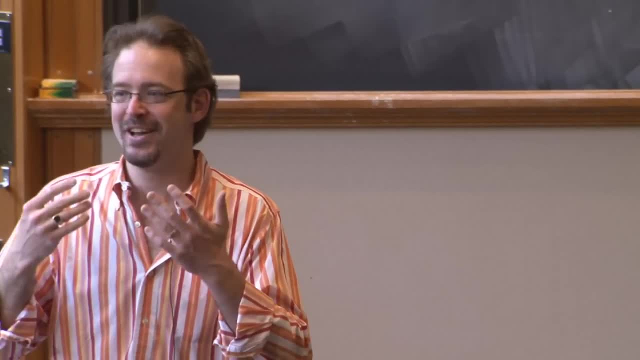 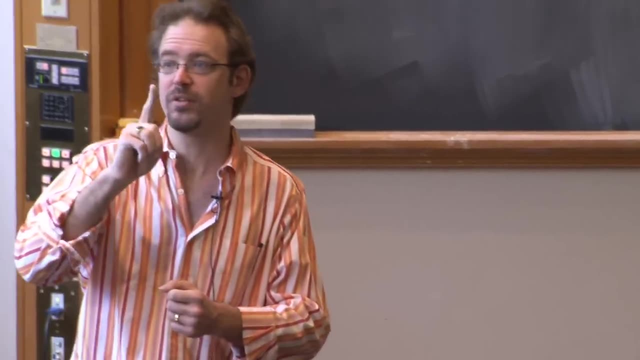 But all we can do is work and see how well our model fits And so far nothing has ever disagreed with the quantum mechanical description. Let me hold off on questions just now because I want to, But it's a good and interesting question. that's a hard one. 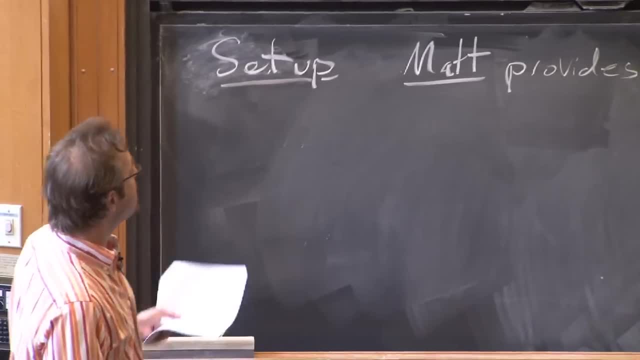 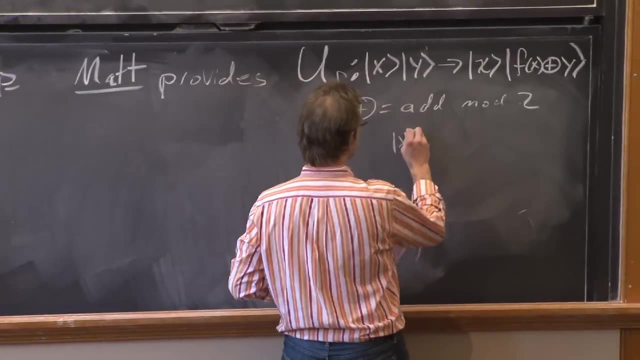 to deal with, by which I mean it's an open question. So Matt provides for us an operator that allows us to calculate f of x. Now, remember, you might have said: well, look, why not just take x and why not have? 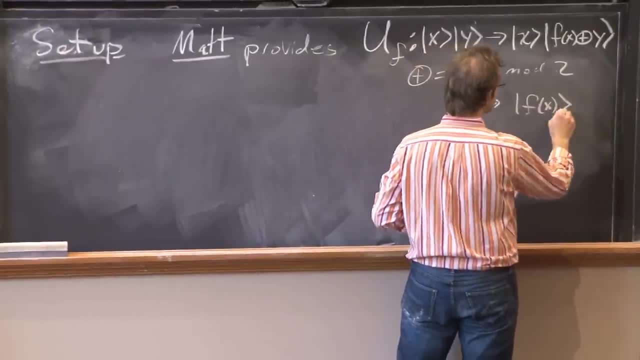 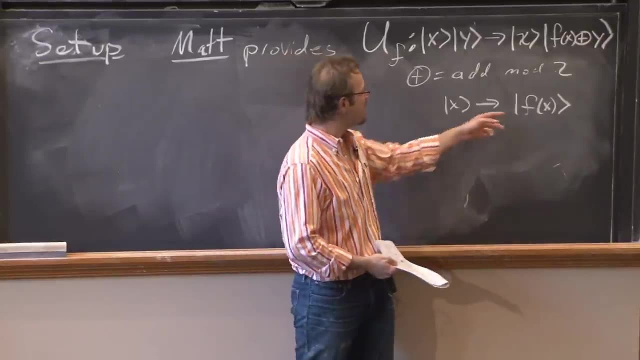 Matt, build a machine that takes x and gives you f of x. Could you have done that? Is there no cloning? Well, it's not exactly no cloning, But let me leave this to you as a fun thing to think about. Why do we need this carrier bit as well? 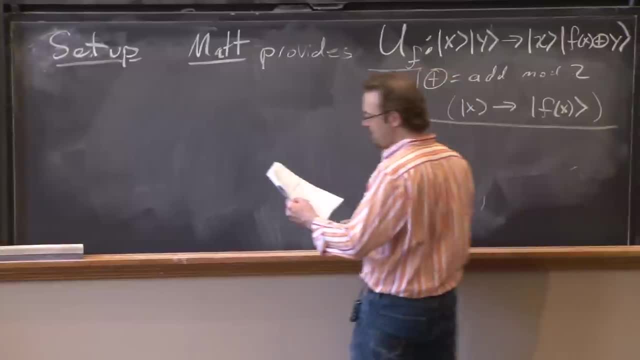 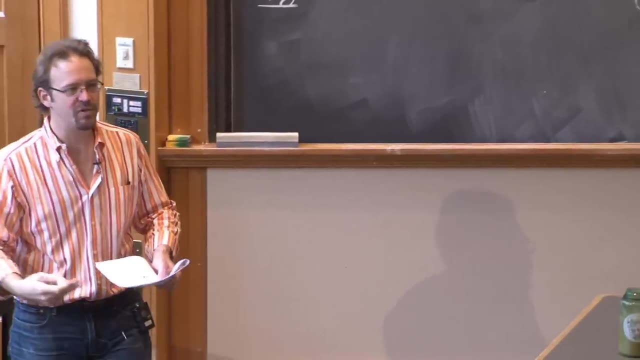 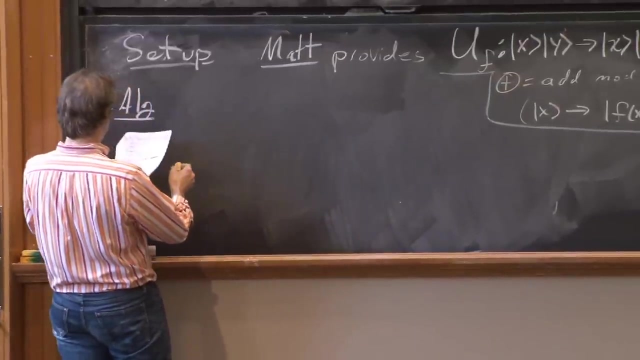 So there's our setup. Matt provides this function for us. u And here's the algorithm. So the algorithm, And it's a series of steps, One by one, we do them. We perform these operations on our qubit. So here's what Deutsch says. 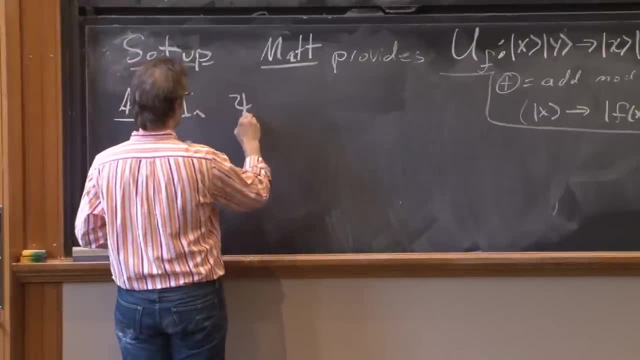 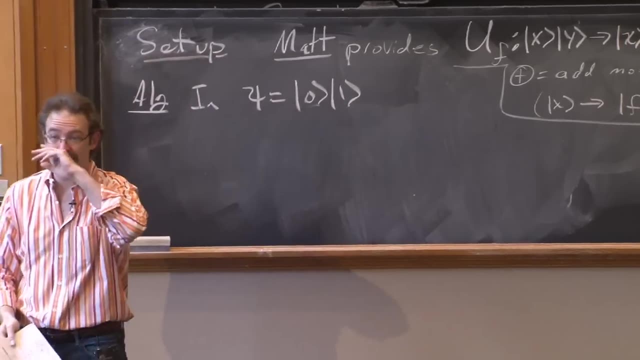 Deutsch says start input. a state psi is equal to 0, 1.. First qubit is 0 in the state 0. The second qubit is in the state 1. for sure We implement that with our boxes, or however we want to implement it. 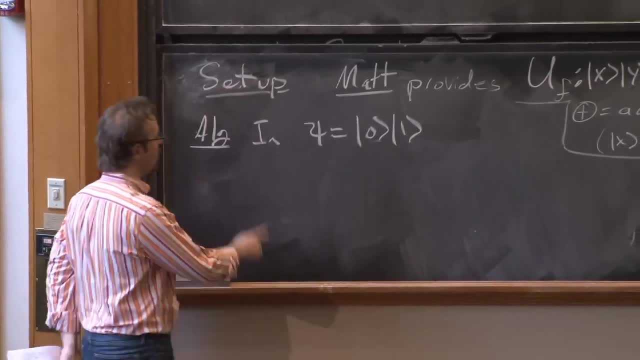 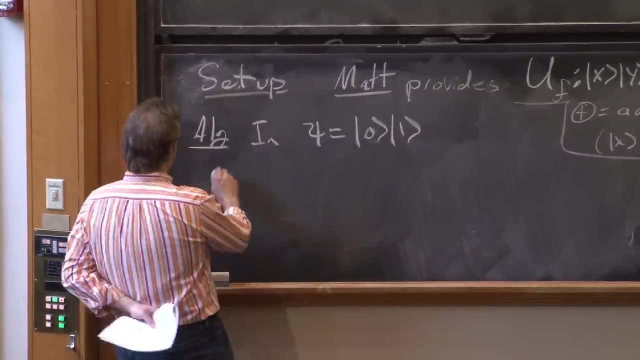 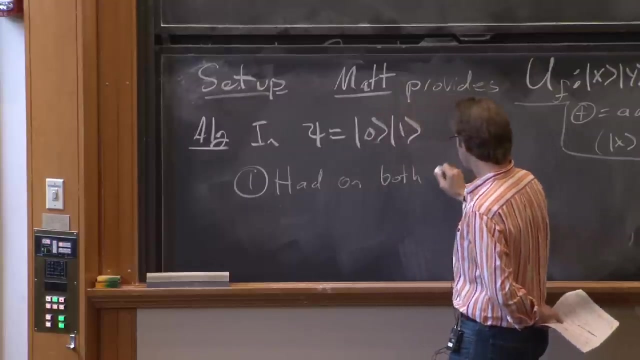 So we find ourselves in a definite state: Hard, soft. We take a hard box and we take a soft box and we pull out the hard one and the soft one. 1. Hadamard, each Hadamard on both bits, both qubits. 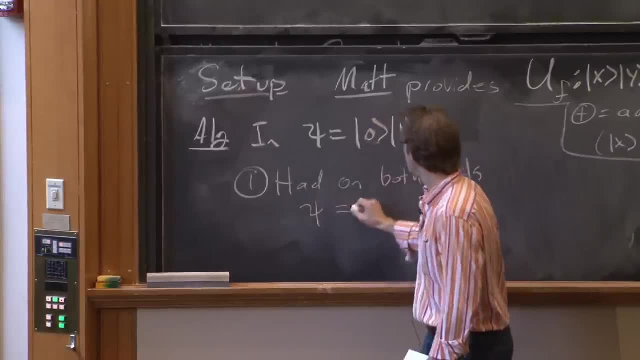 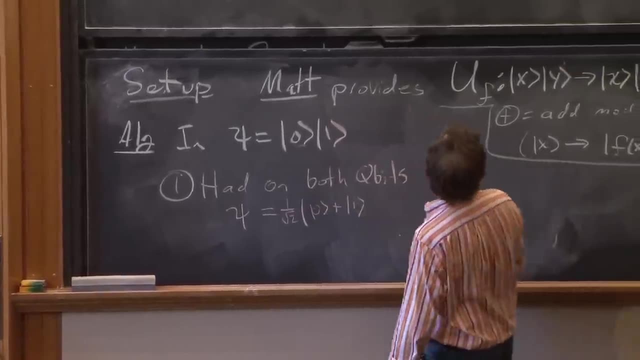 So what does this take us to? It takes us to: psi is equal to well. the 0 goes to 1 over root, 2 times 0 plus 1.. Did I erase Hadamard? No Good, There's Hadamard. 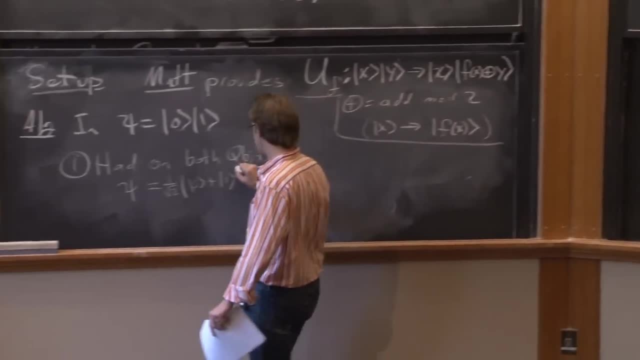 So it does this. it does this. So it takes the first one to 0 plus 1, and it takes the second one to 1 over root 2. 0. 0. 0. 0. 0.. 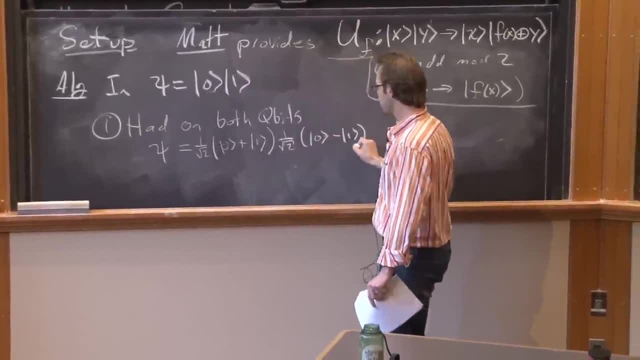 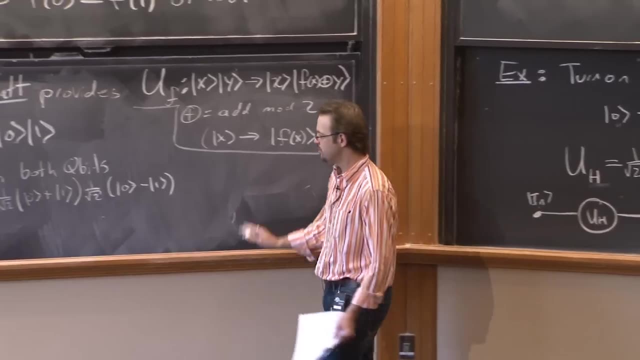 0 minus 1.. Cool. So at this point, this is very interesting. All we've done is we've taken it from one superposition to a different superposition, And it doesn't seem to have anything to do with f. In fact, we haven't measured f. 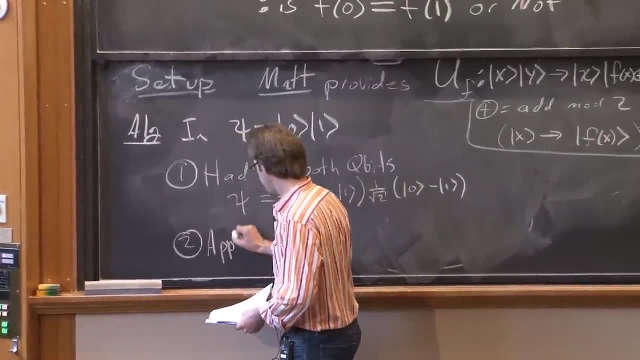 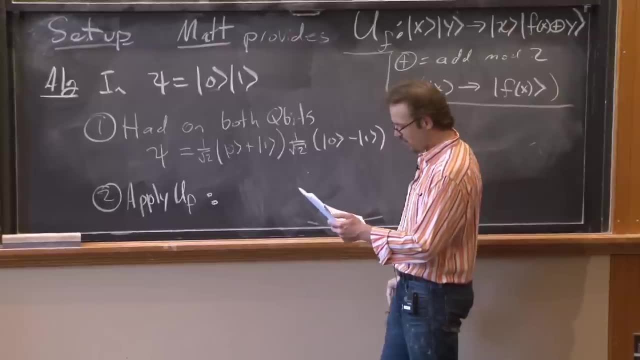 2. Apply f. So we apply our operation u sub f, And this takes us to: ah well, this is a sort of entertaining one If we take this 1 over root 2, so I'm going to rewrite this. 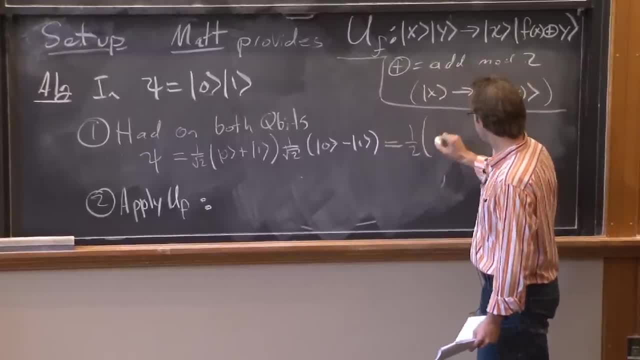 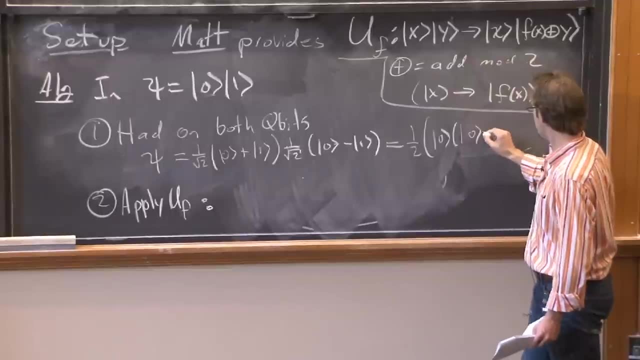 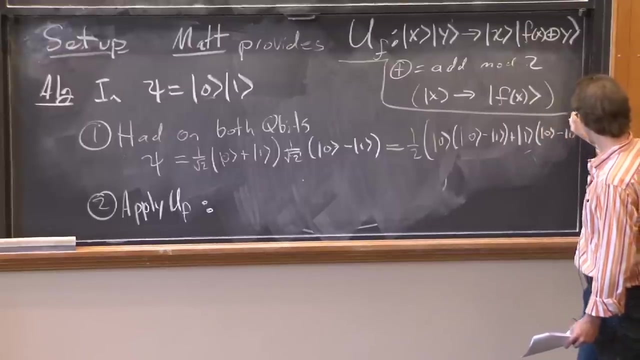 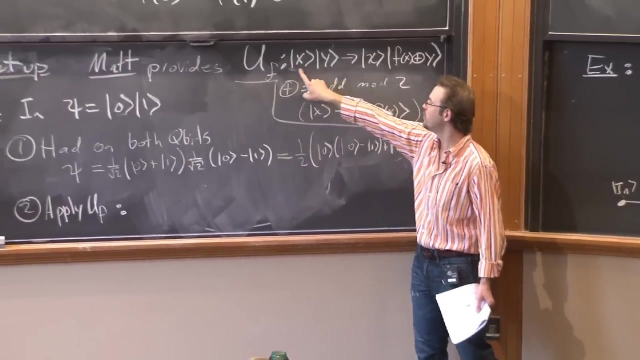 In a slightly simpler form, this is 1 half 0 times 0 minus 1 plus 1 times 0 minus 1.. And the reason I'm doing that is we're going to apply uf And uf. our function f uses that first bit. 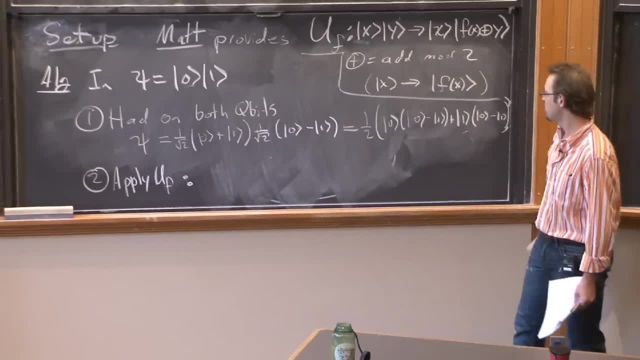 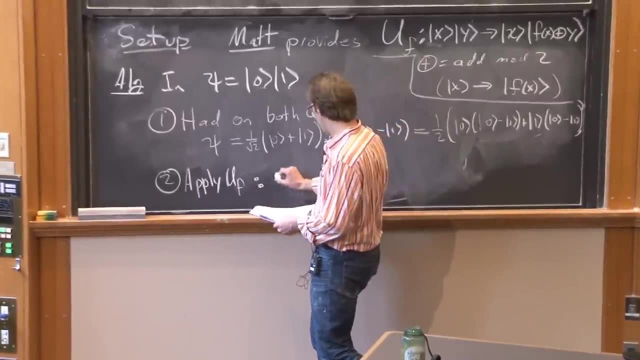 as a control bit for the second. So here's the control bit for the second. So we apply uf And this gives us 1 half. I'm going to actually do this on the next board because it's going to be gigantic. 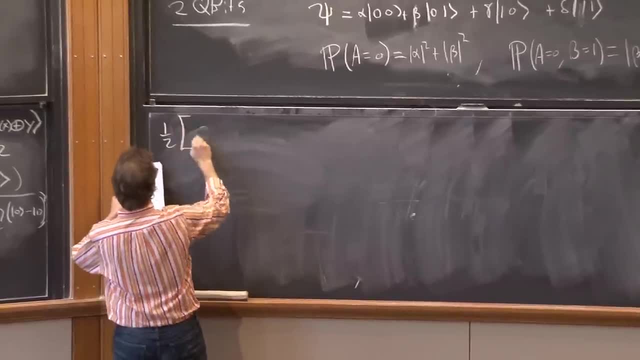 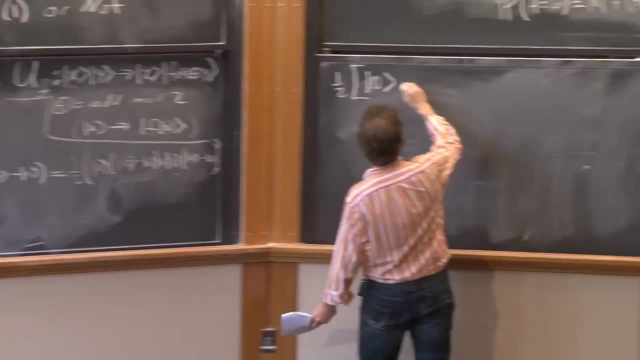 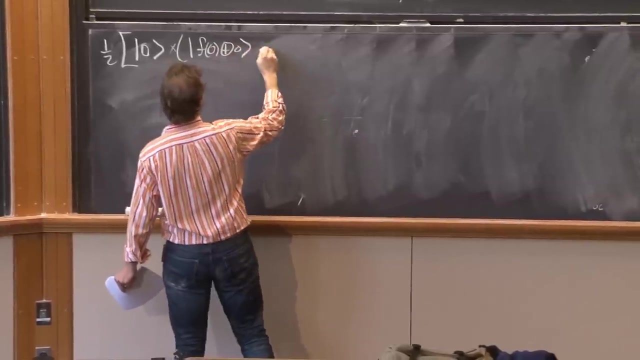 So this gives us 1 half. So that first one, this is going to take this and give it 0 plus f of 0 and 1 plus f of 0. So times f of 0 plus 0 minus f of 0 plus 1.. 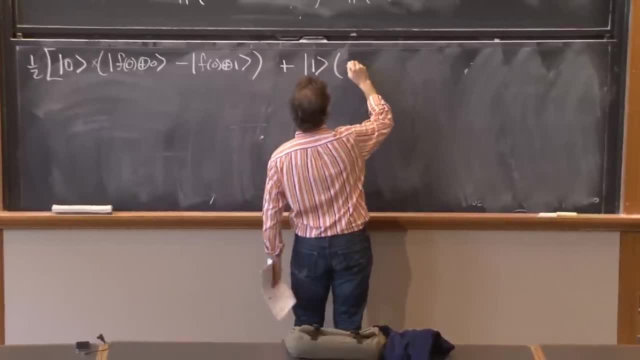 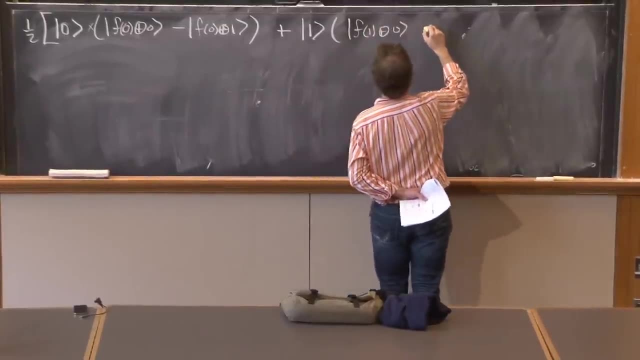 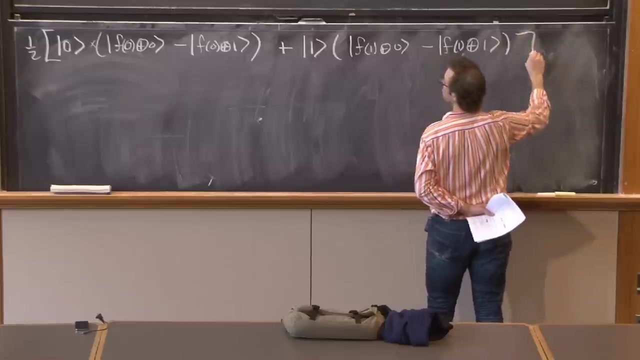 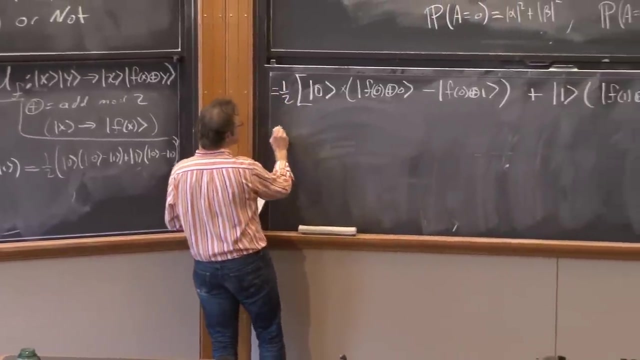 Plus for the 1, this is going to be times f of 1 now plus 0, minus f of 1, plus 1.. Now here's a crucial step. This is equal to, and I want to note the following: 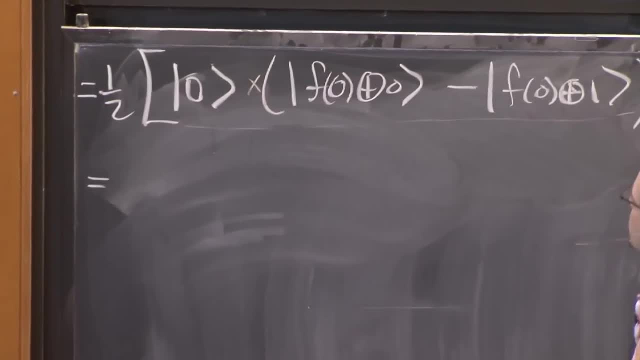 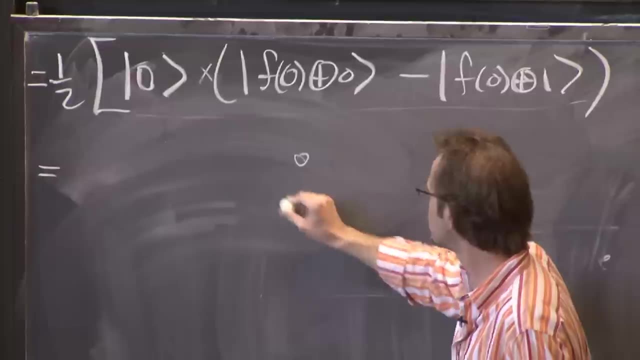 Look at this particular guy. So for that particular guy, suppose f of 0 is 0.. If f of 0 is 0, then this is 0 plus 0, which is 0.. So f, If f of 0 is equal to 0, then this gives me 0. 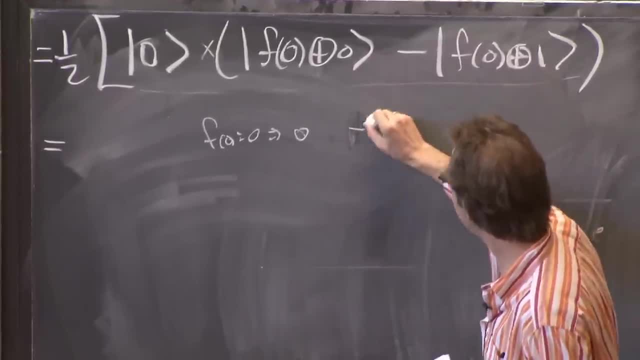 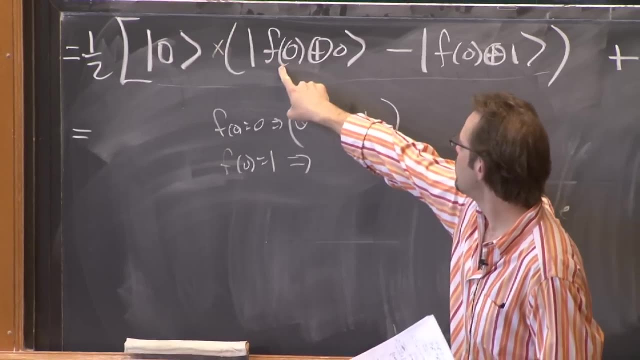 And this gives me 0 plus 1,, which is 1, 0 minus 1.. On the other hand, if f of 0 is equal to 1,, then we get 1 plus 0,, which is 1.. 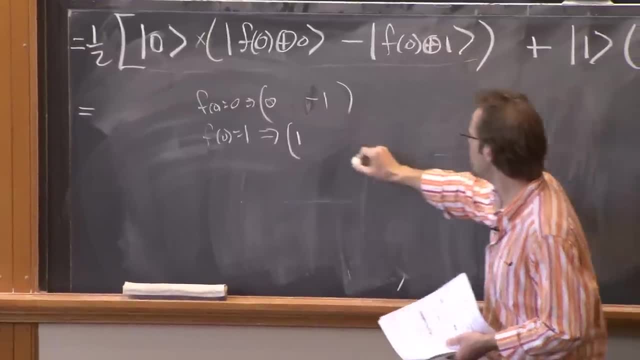 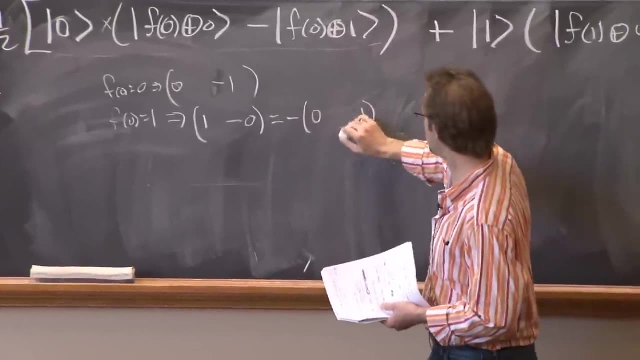 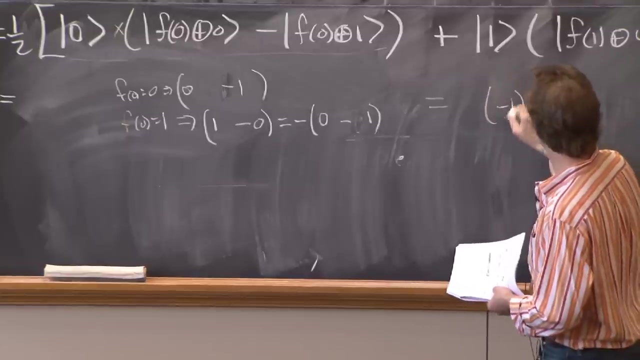 And here we get 1 plus 1,, which is 0 minus 0,, which is equal to minus 0 minus 1.. Yeah, Cool, then, So I can write this as minus 1 to the f of 0 times 0 minus 1.. 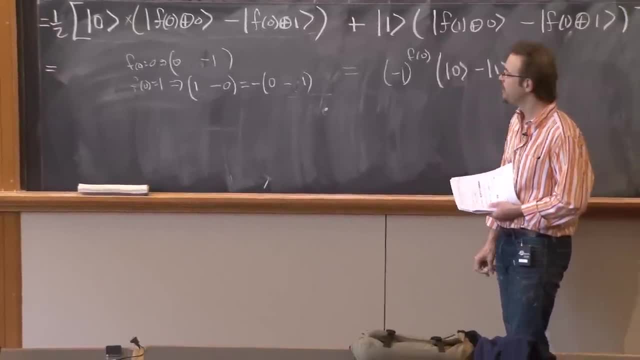 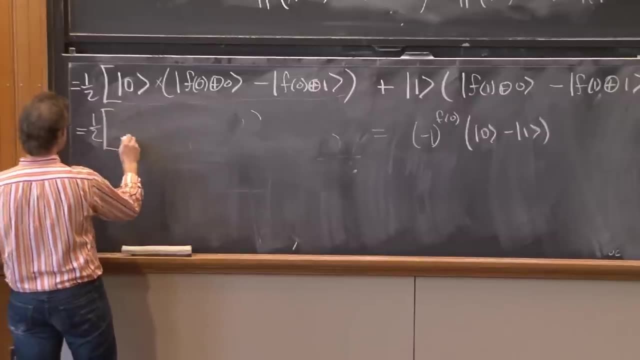 Very cool then. This is just a little exercise in binary arithmetic, So I can write this first term. This is 1 half minus 1 to the f of 0. 0. 0. 0. 0. 0.. 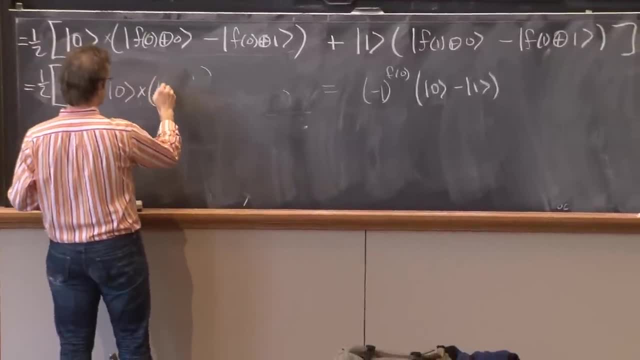 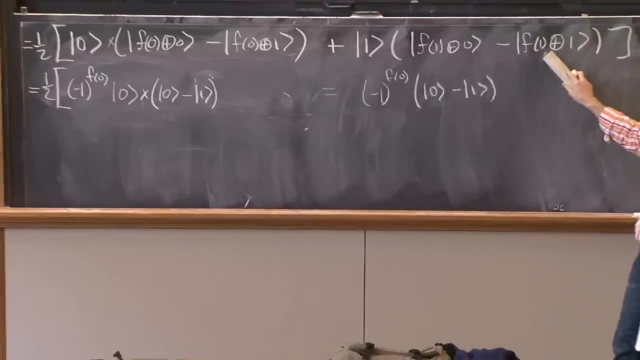 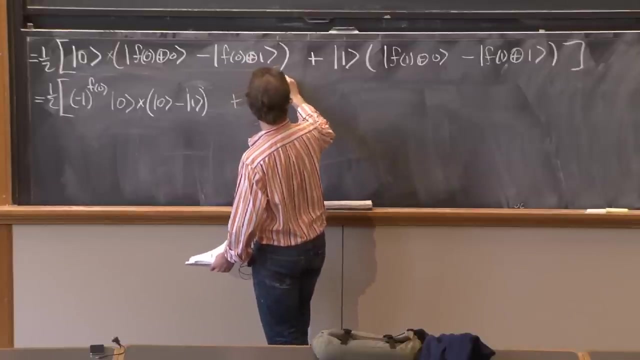 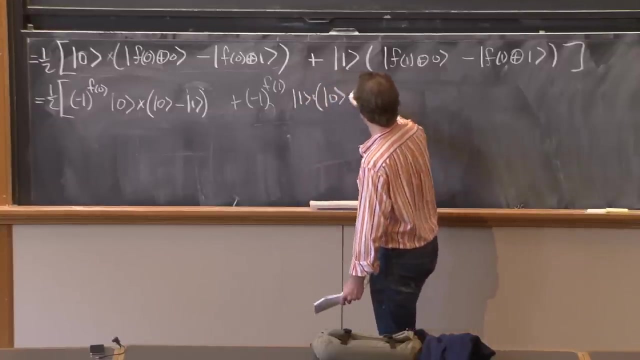 0 times 0 minus 1.. So that's from the first one And exactly the same logic is going to apply to the second, but now f of 1 instead of f of 0. Plus minus 1 to the f of 1 times 1 times 0 minus 1.. 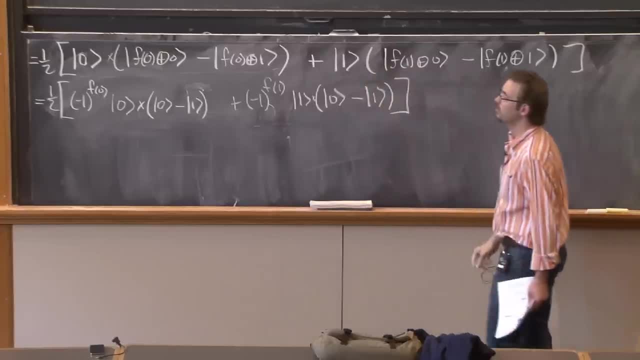 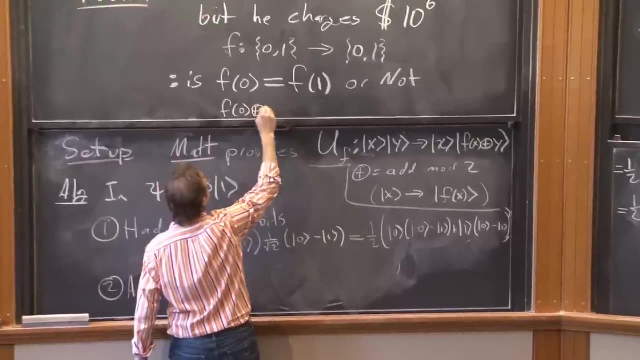 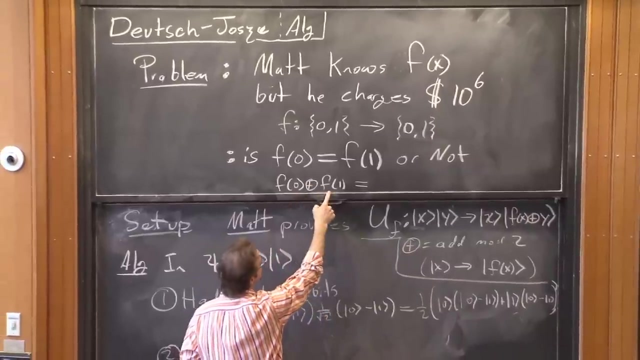 Now I want to point something out to you. If f of 0 is equal to f of 1, then what's true of f of 0 plus f of 1?? Well, if they're the same exactly, then either it's 0 plus 0, in which case we get 0,. 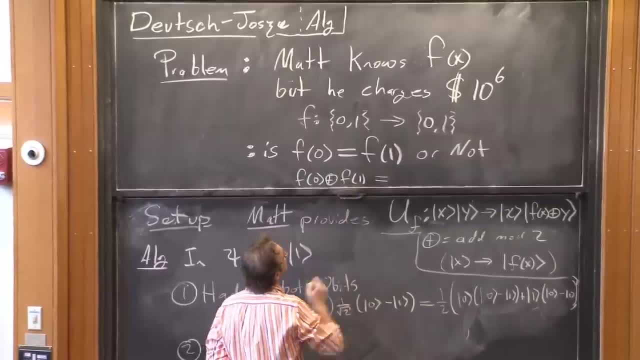 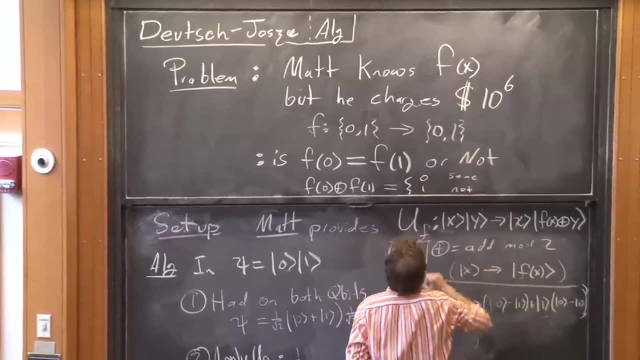 or it's 1 plus 1, in which case we get 0. So this is 0 if it's the same and 1 if it's not. So we could either Know them both or we could measure f of 0 plus f of 1.. 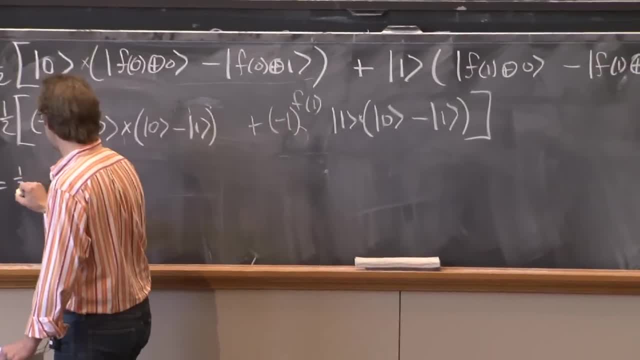 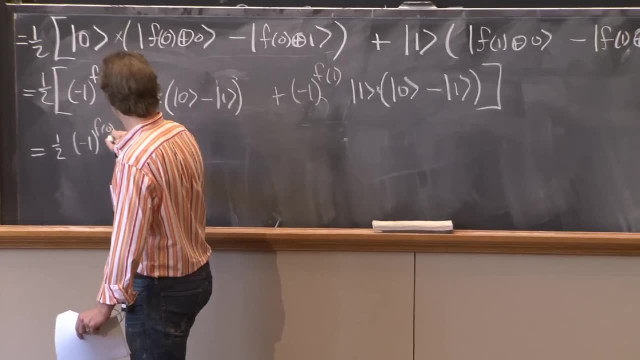 So notice what happens here. This is equal to 1 half, And now I'm just going to pull out a factor of f of 0. Minus 1 to the f of 0 times. Well, both of these terms have a 0 minus 1. on the second bit, 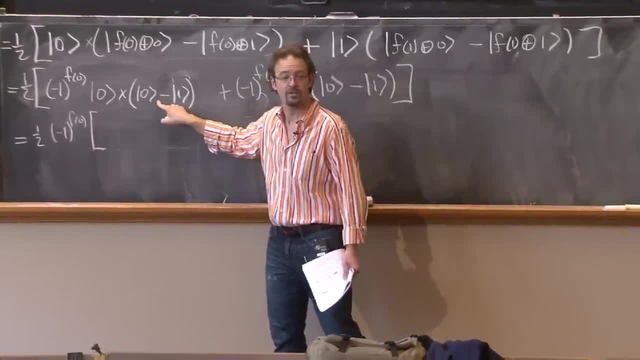 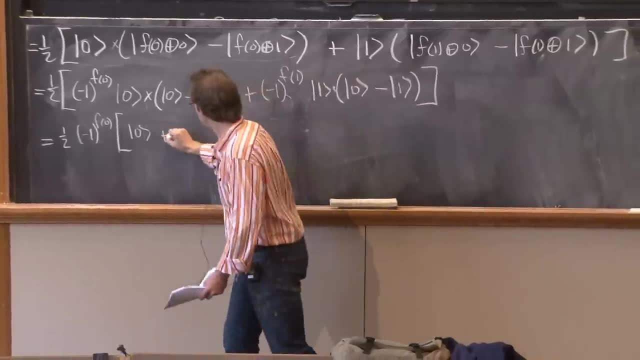 So the second qubit is in the state 0 minus 1.. Right, Everyone cool with that. So this is equal to, for the first qubit, 0 plus 1 times minus 1 to the f of 0.. I've pulled out to square it. 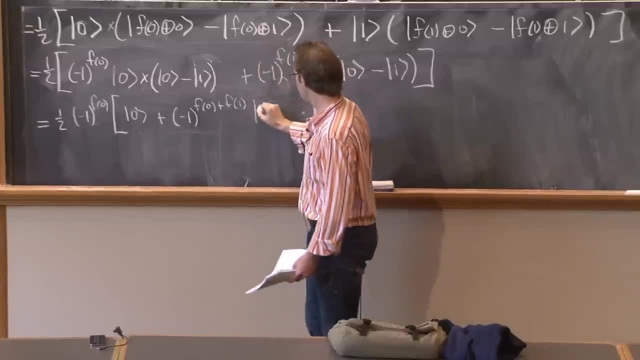 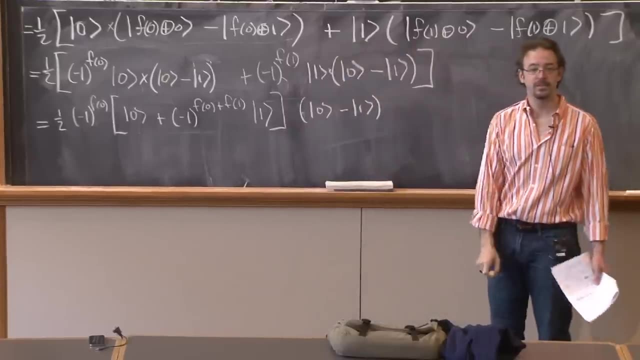 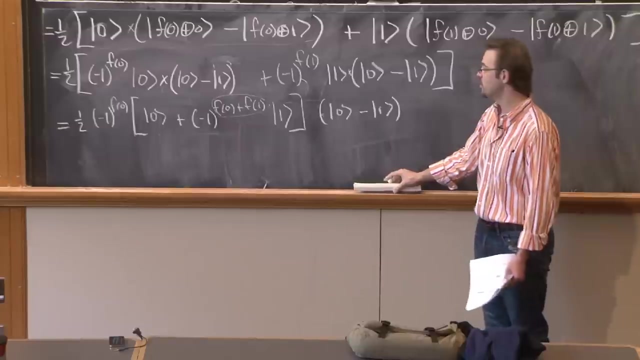 Plus f of 1 times 0 minus 1.. And here's the quantity we wanted to measure. If this is 0, then they're even, Then they're the same, And if it's 1,, then they're not the same. 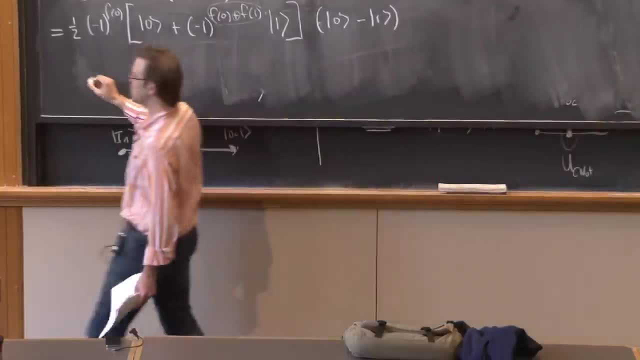 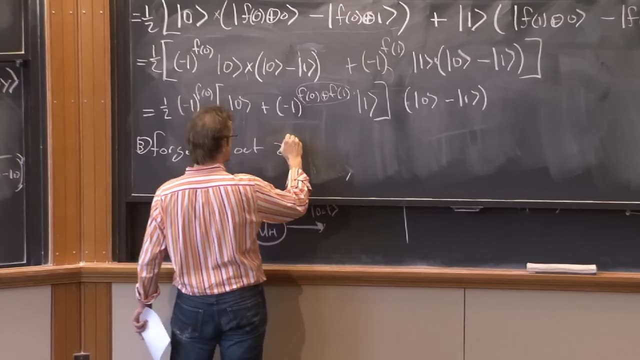 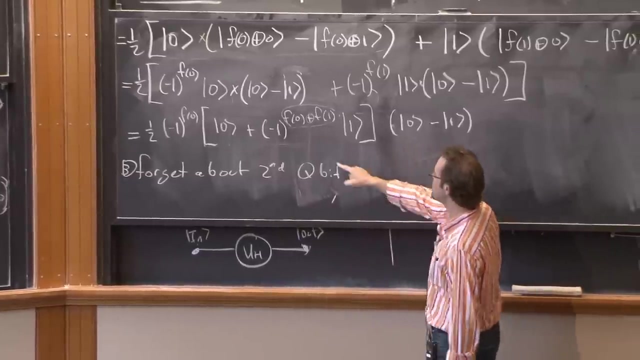 So now, at this point, we just forget. 3. Forget about the second qubit, Oh lord. Forget about the second qubit And we get the state. So forget about the second qubit. just does this. Just focus on this guy. 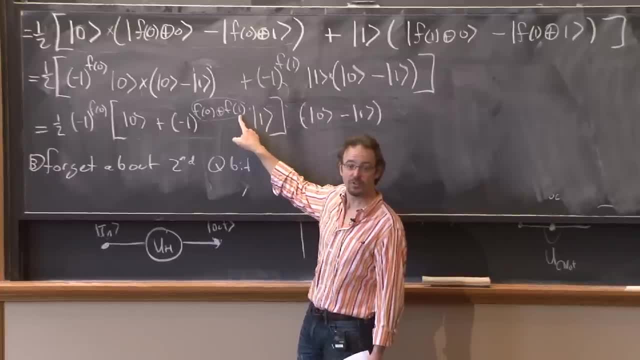 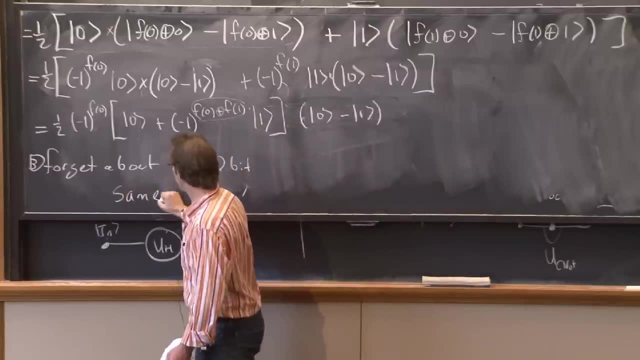 And now, if f is 0 plus f of 1 is 0, so that they're the same, This is 0. Minus 1 to the 0 is 0. So we get 0 plus 1.. So same. 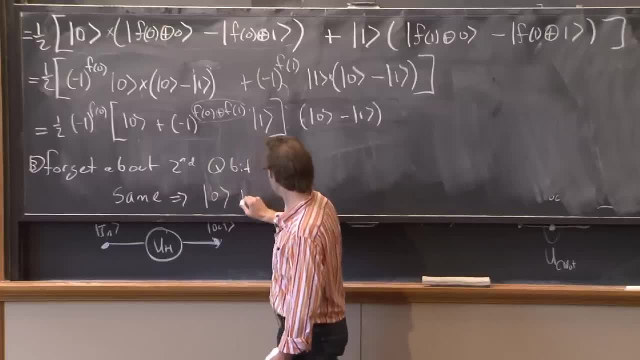 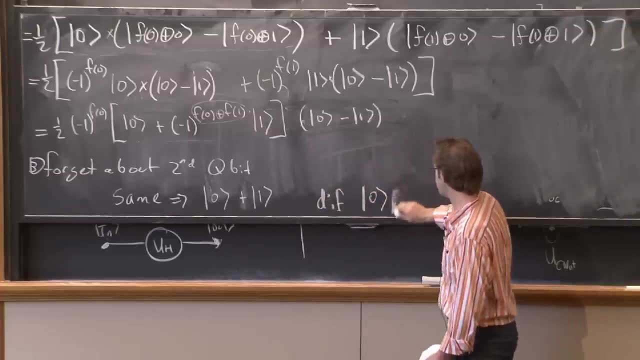 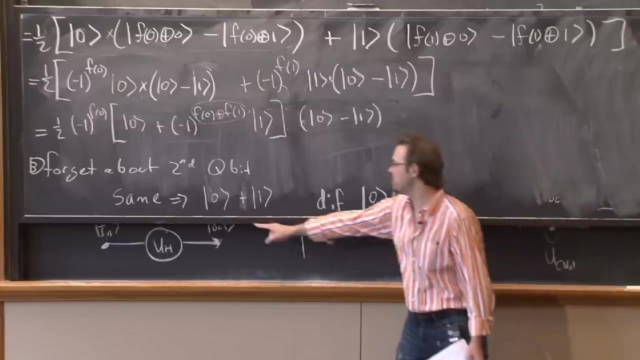 Then our state is 0 plus 1.. And if they're different, then we get the state 0 minus 1.. Everyone agree with that. So if they're the same, we get 0 plus 1.. If they're different, we get 0 minus 1.. 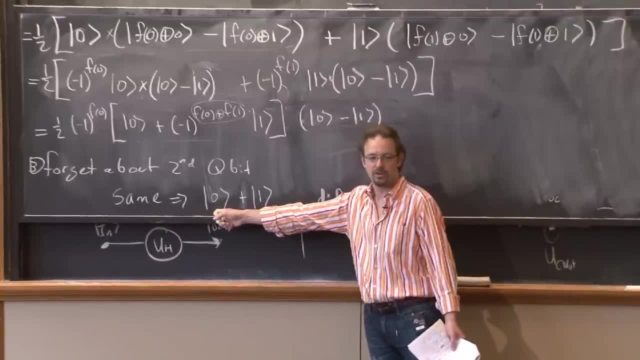 Still doesn't work for us because if we measure what's the probability we get 0, here 1 half. The probability we get 1 is 1 half. It's similar if we measure here, it was 0, 1 half, 1, 1 half. 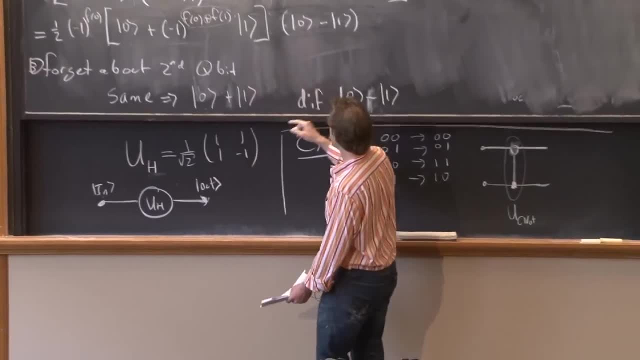 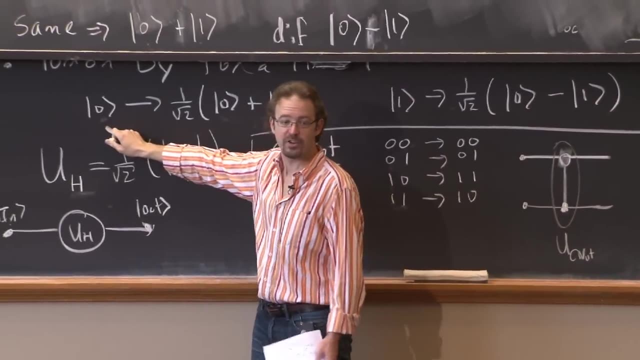 On the other hand, these states are familiar to us because they're what you get by Hadamarding. So why don't we take these from these states to these, by doing the inverse of the Hadamard which it turns out is Hadamard itself? 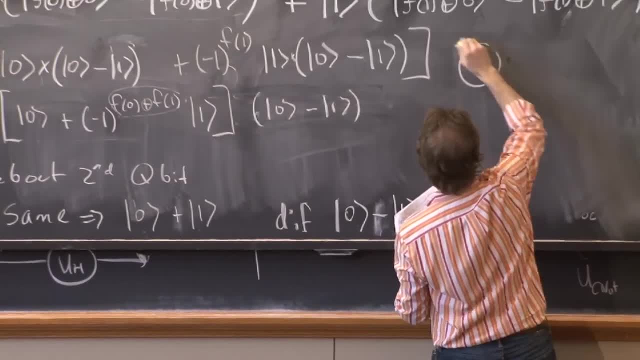 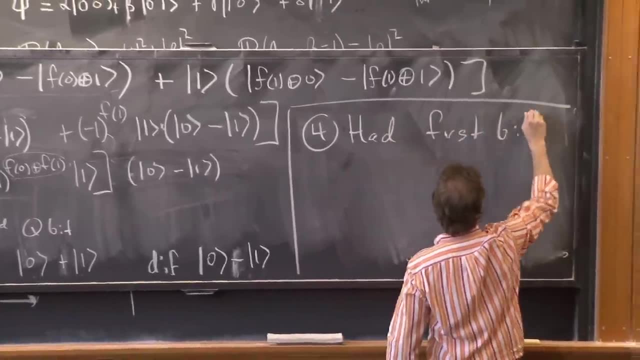 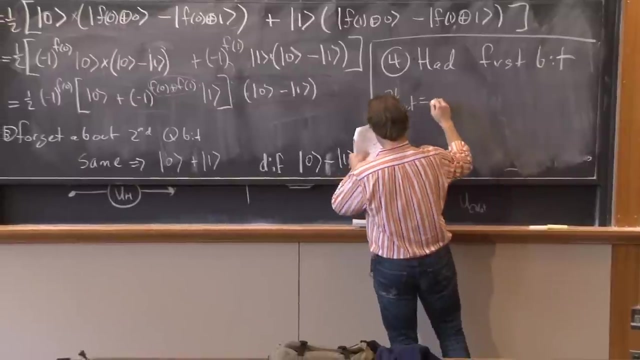 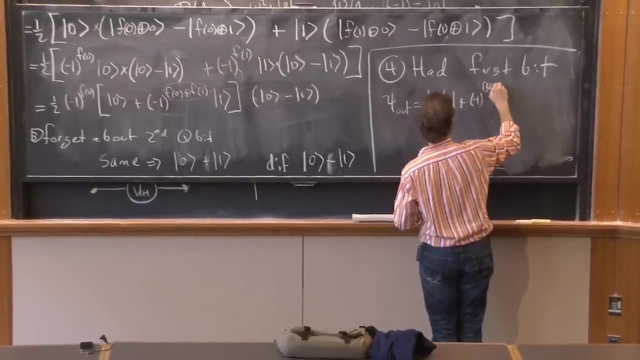 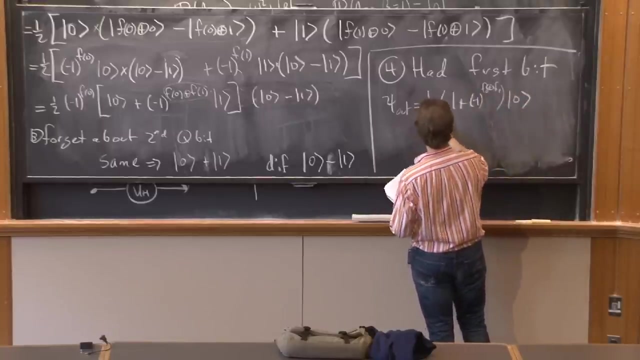 So for Hadamard the first bit had the first bit and we get The output is: the state psi out is equal to 1 half 1 plus minus 1 to the f0 plus f1: 0 plus 1 half 1 minus minus 1 to the f0 plus. 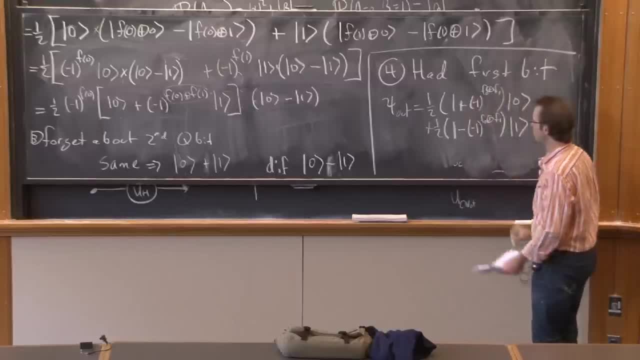 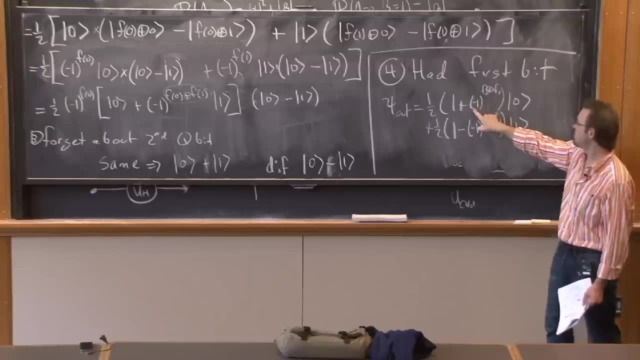 f1- 1.. And now, if f0 and f1 are the same, this is a 0.. We get 1 plus 1.. We get just 0, and this is 0.. Because this is 1, this is 1, we subtract, we get 0. 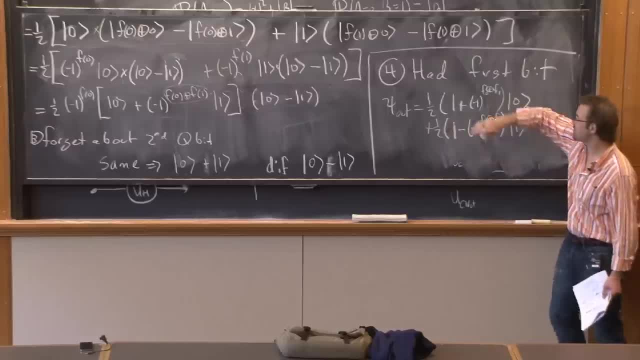 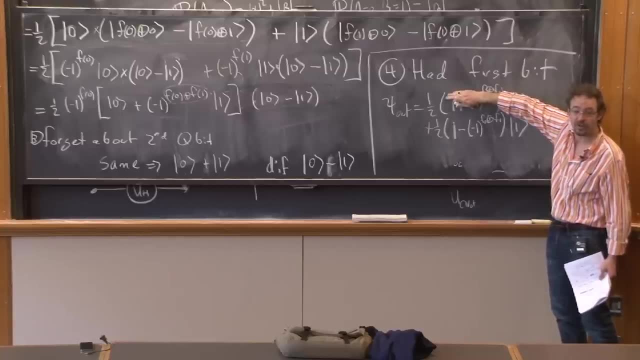 They're the same, you get this state 0, properly normalized. If they're not the same, you get this state 1, properly normalized. Now, if we measure 0, we know they're the same, And if we measure 1,, we know they're different. 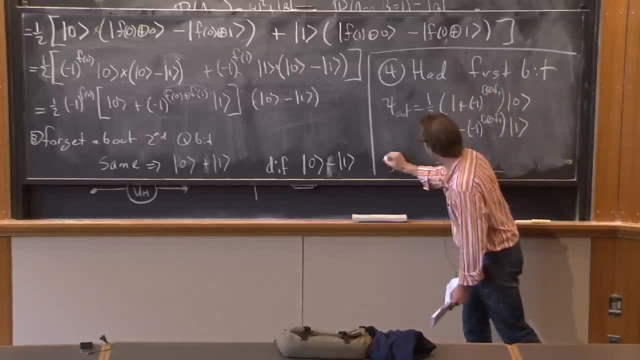 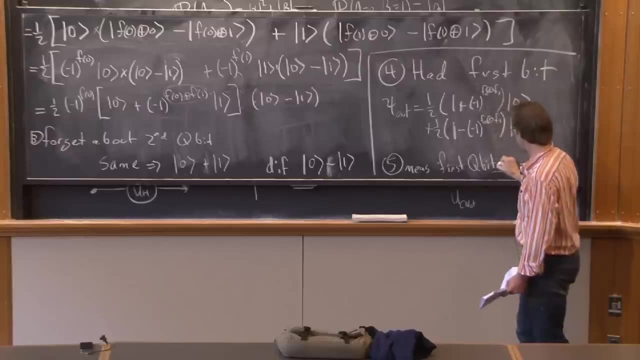 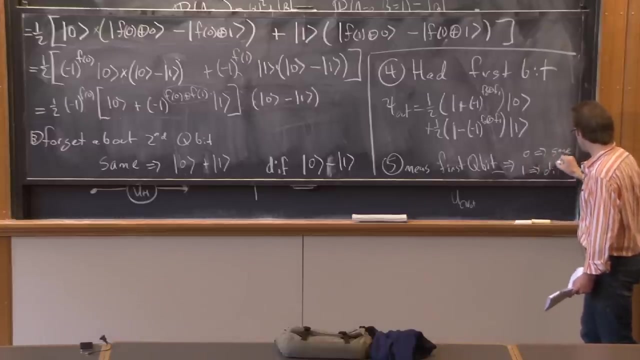 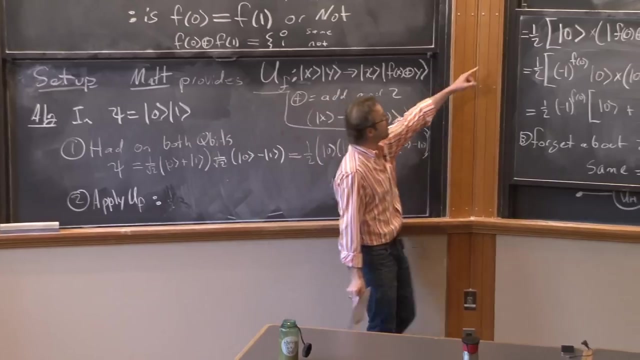 And so, with absolute certainty now 5, measure the first qubit And we get: 0 implies the same and 1 implies different. And we did all of this with a single evaluation of our function f right here. This is where we applied our function evaluation. 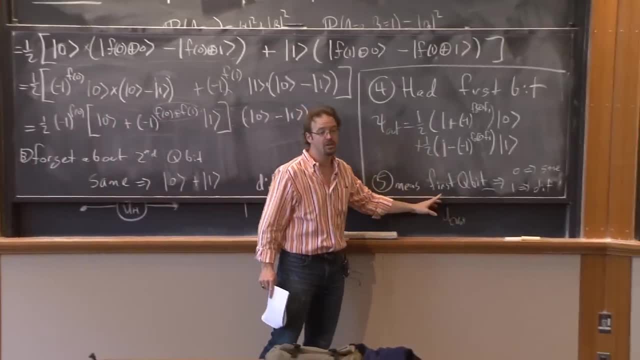 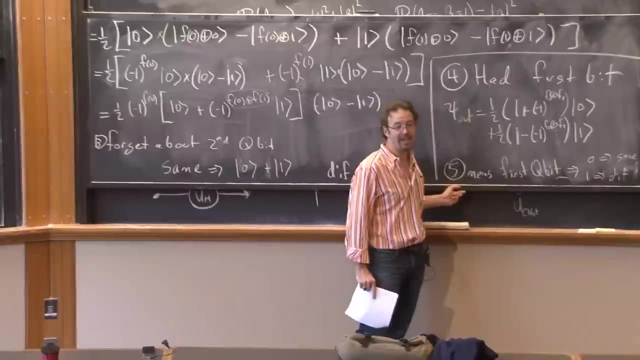 We've applied the function evaluation once and we deterministically get the result whether they're the same or different. So with one call to Matt to my oracle, with one call to Matt which cost me $1 million, we get the answer to whether it's the same or different. 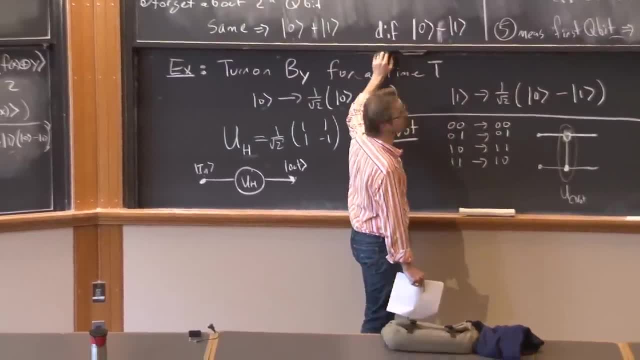 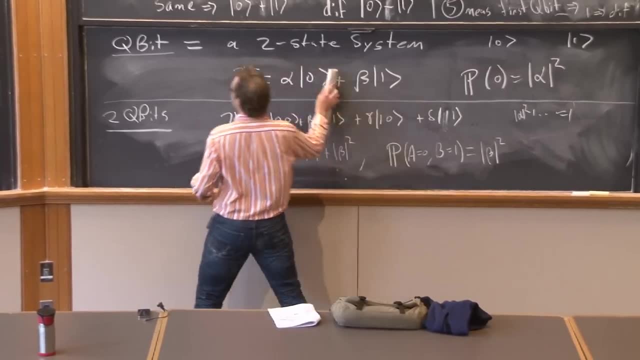 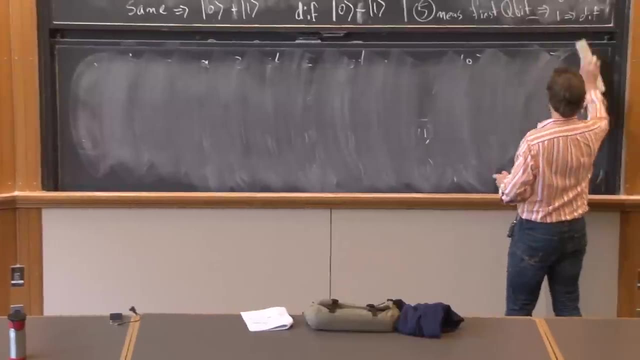 And that's a factor of 2 faster than the best classical algorithm, But that's not so satisfying. This was supposed to be exponentially better, And so that's where Joza comes in, And together with Deutsch, Deutsch and Joza show the following: that there's an exactly analogous problem. 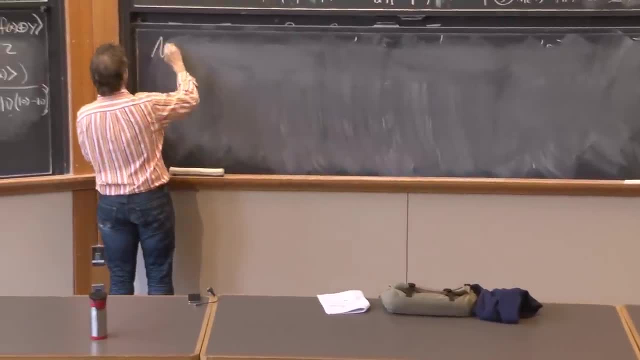 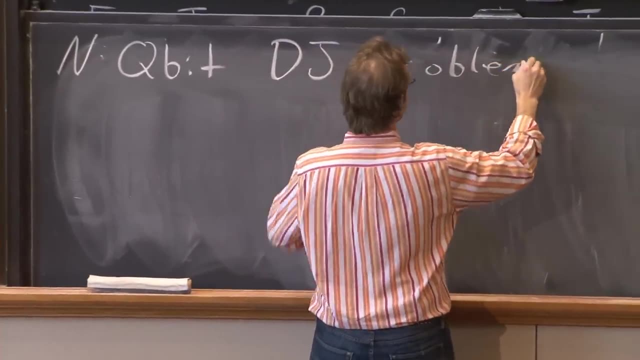 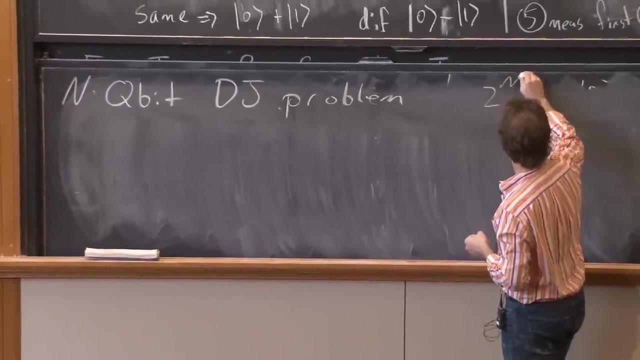 for n qubits. Wow, There's an exactly analogous problem for n qubits- Deutsch Joza problem. And now, how many different strings of integers could you put in? There are now 2 to the n possible states, And if you want to know whether f is the same for all of them, 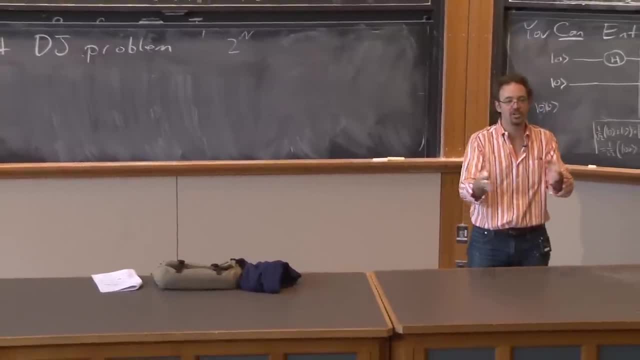 the worst case scenario is you evaluate f on the first possible combination- 0, 0, 0, 0. And you get some number Measure f on 0, 0, 0, 0, 0, 1.. 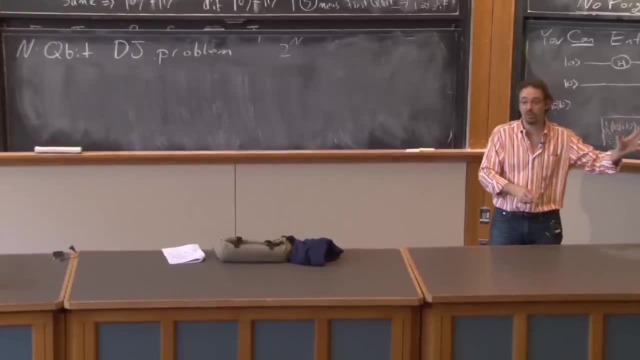 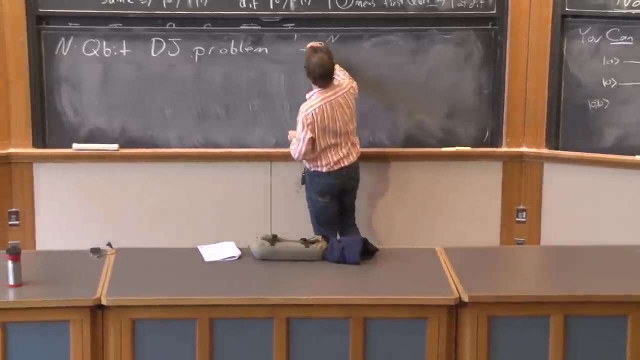 And you get the same number And you just keep doing that forever And you still don't know if they're all the same until you get to the very last one. So it's 2 to the n. It's order. 2 to the n is the worst case scenario. 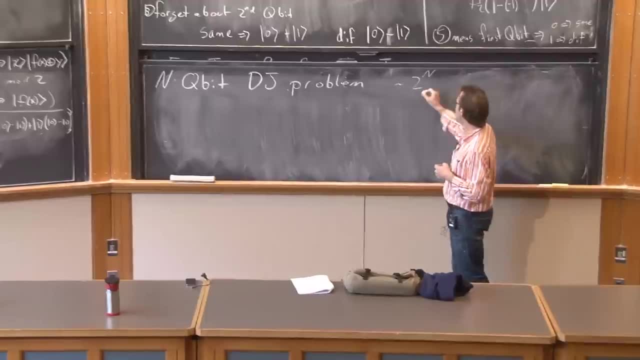 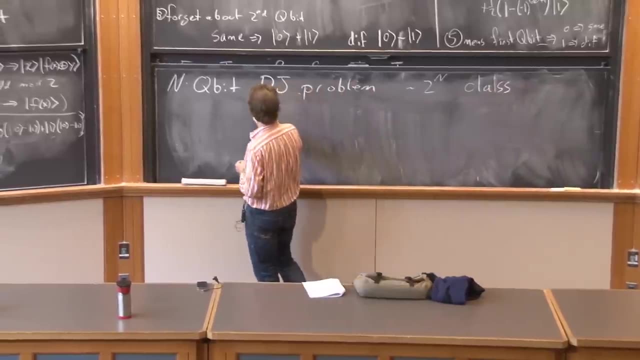 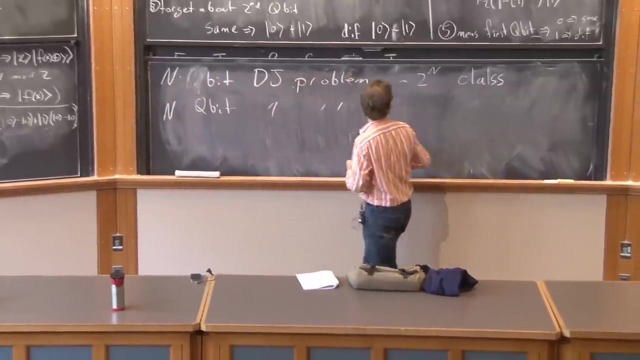 But typical scales are of order 2 to the n, So classically it takes an enormous number of observations. But the quantum of Deutsch Joza algorithm- Sorry, that was n bit Deutsch Joza And now the n qubit Deutsch Joza problem. 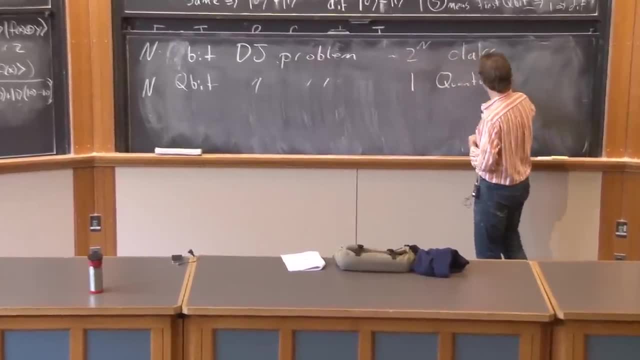 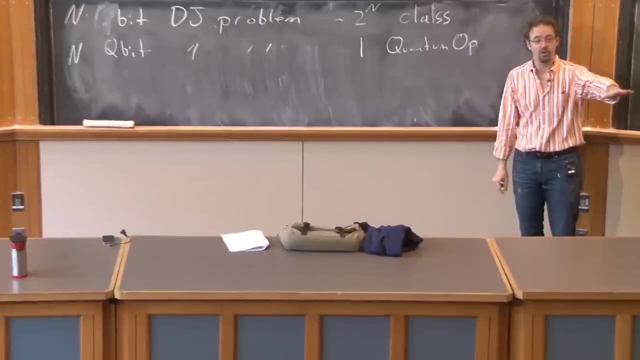 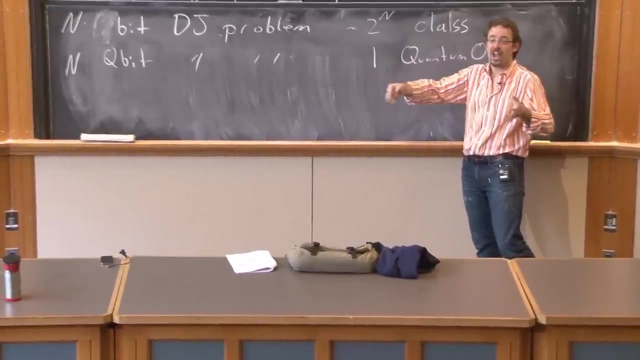 One quantum operation And you get a deterministic result And all of this 1,. you evaluate it once and you know you've solved the problem. So instead of 2 to the n operations, it takes a single 1.. And now for a large number n of bits, 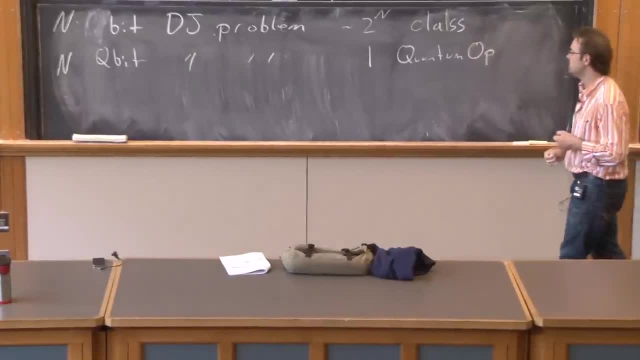 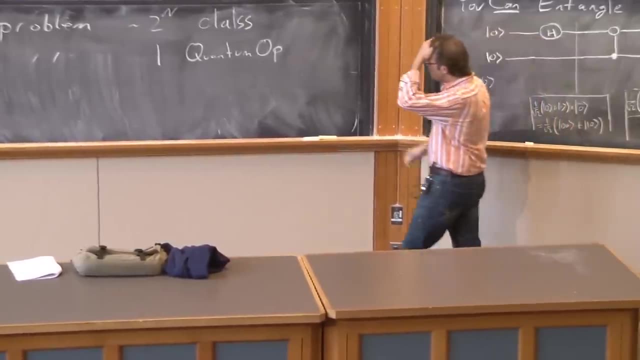 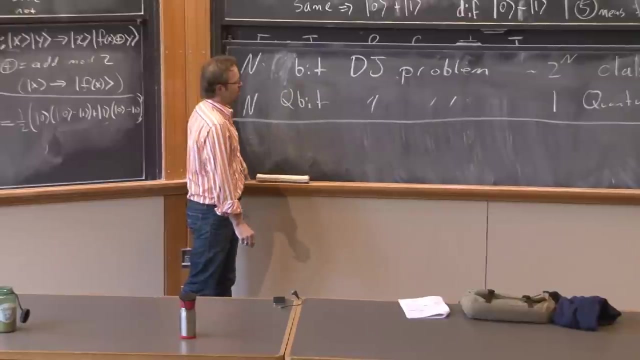 for example, for large integers dealing with very large numbers, this is dramatically, exponentially more efficient than the classical algorithm. So this is the basic. At this point people start really seriously thinking about quantum computation, whether you could get it to work And how much juice you could get out of actually building. 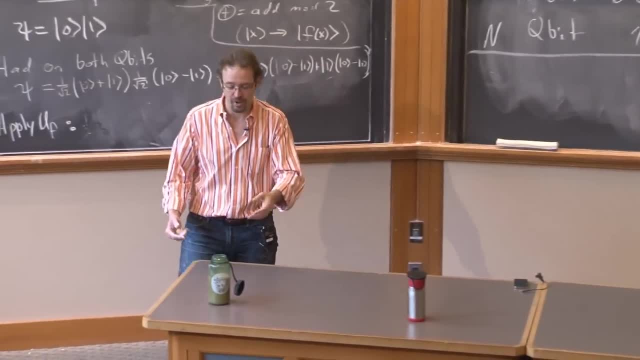 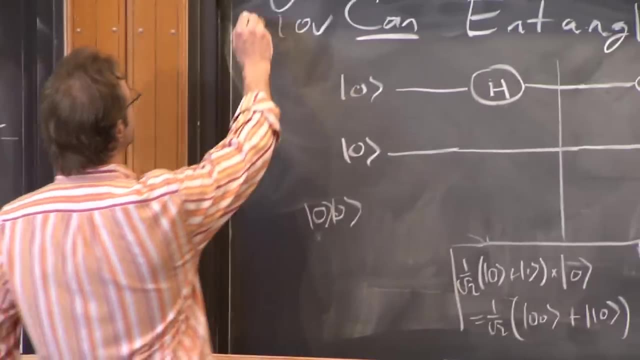 such a quantum computer And this is developed into a whole field of the theory of computation. The thing I want to emphasize is that the crucial move is observing that in quantum mechanics you can entangle degrees of freedom. The crucial move is observing that you 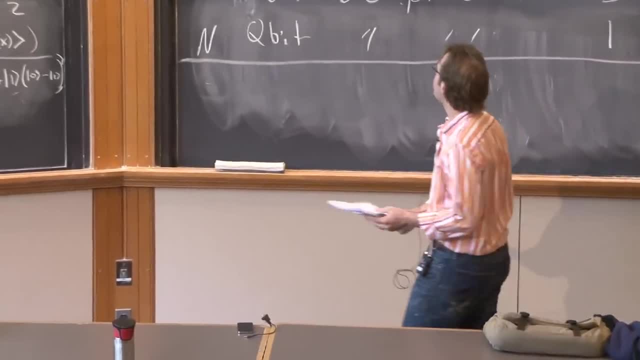 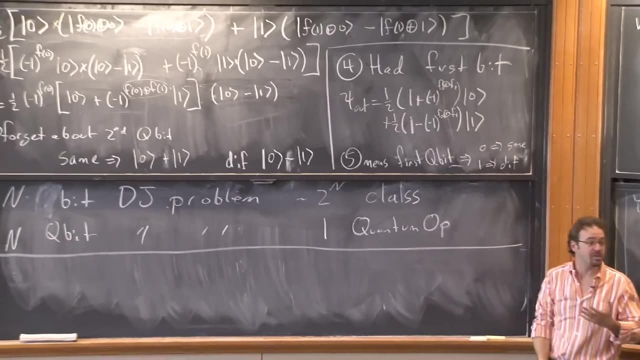 can entangle degrees of freedom quantum mechanically, And that's what gave us all of the nice effects We have: these interference effects. And these interference effects lead to the deterministic outcome being correlated With the result of the computation. The interference is crucial. 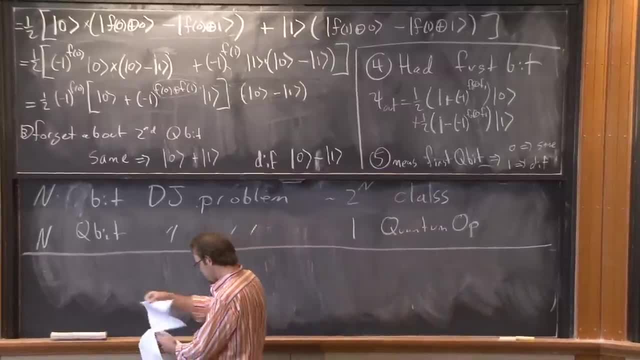 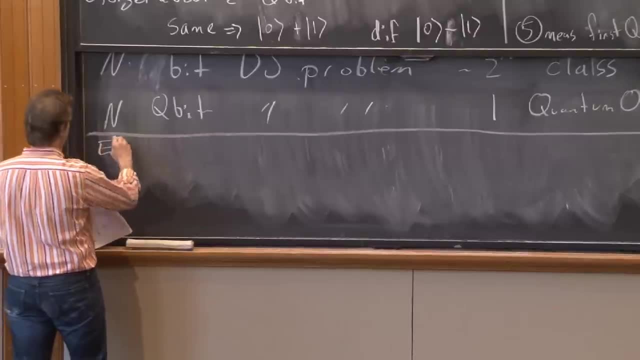 And this brings us to the last point, which is exactly what's so troubling about entanglement. And so here is where EVR came in, And Einstein, Podolsky and Rosen say the following. They say: look, there are two things. 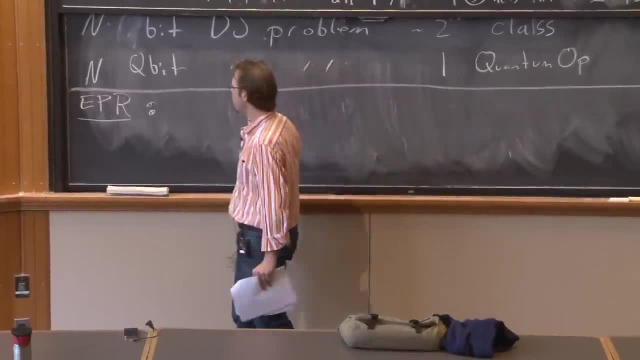 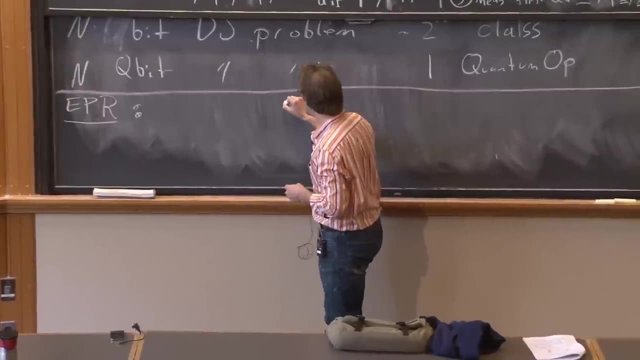 that are deeply upsetting about this entanglement story. The first: let me just give you a precise experiment, they say. They say: let me give you a precise experiment. that embodies all the weirdness of this. Suppose they take two, I take two of these qubits and I put the two qubits 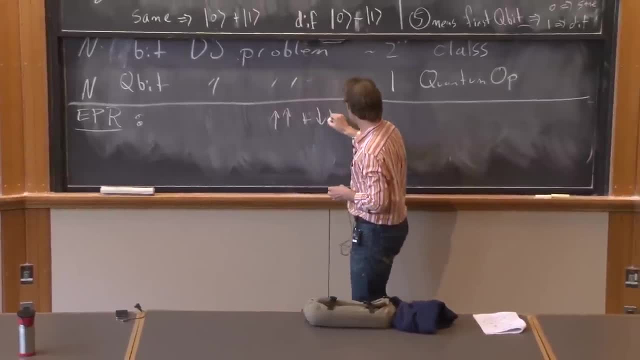 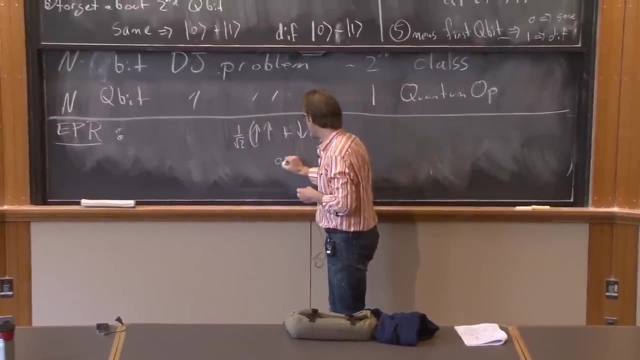 in an entangled state, up up plus down down, And let's normalize this with 1 upon root 2.. So there's our state, And then we take the first qubit. So there's our two bits, And we take the first qubit and we send it some far away. 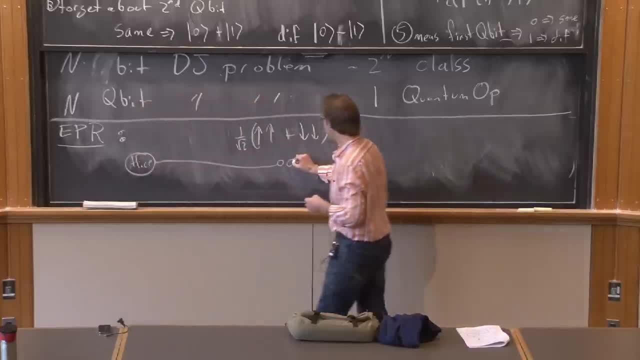 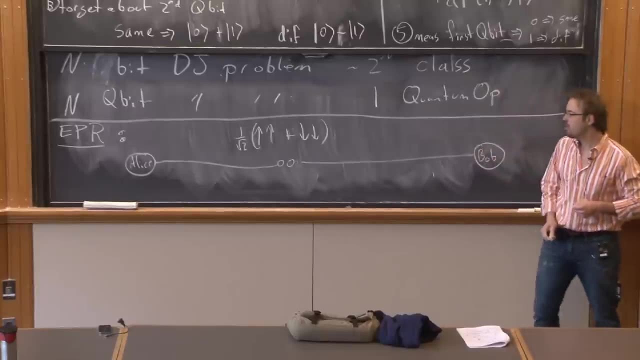 And someone named Alice is sitting here and is holding onto that bit, And we take the second one, and we take it far away And someone named Bob, conventionally, is sitting here and holds the second bit. Now, given this, 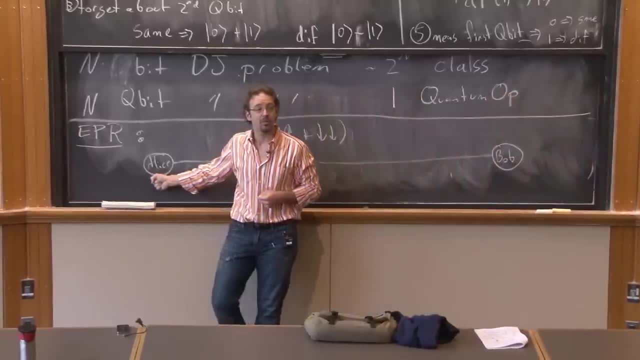 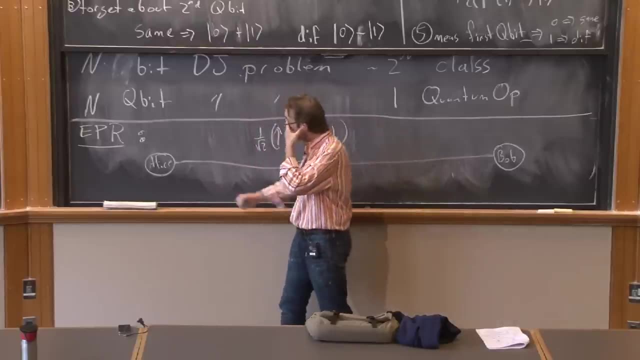 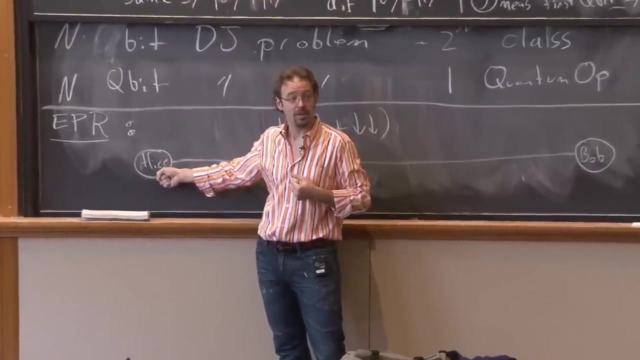 Initial configuration. What is the probability that Alice will measure the spin to be up, Her spin to be half and then half down, Similarly Bob half up and down. Once Alice has measured the state to be up, immediately she knows something about Bob's spin. 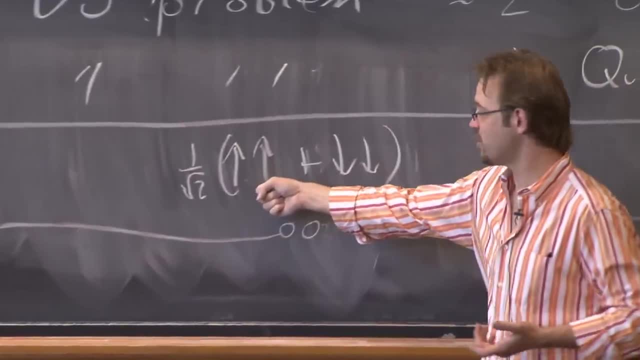 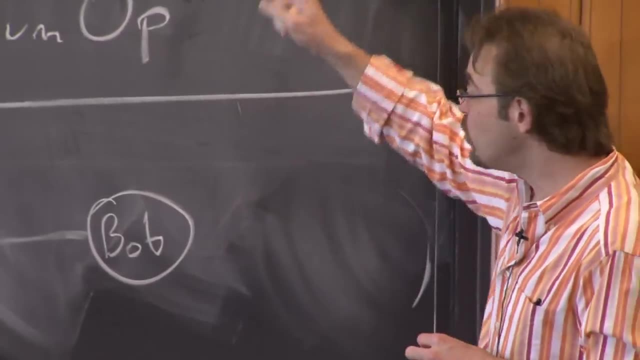 Bob's state will be up Because I chose this one. I could have chosen the other one, which is the more popular EPR pair, So Bob's will also be up Now if you look at the list, if you do this over and over. 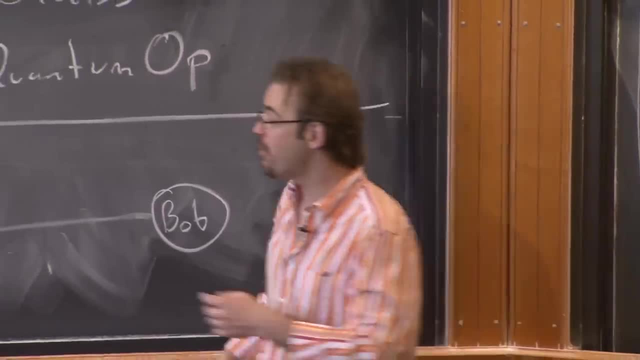 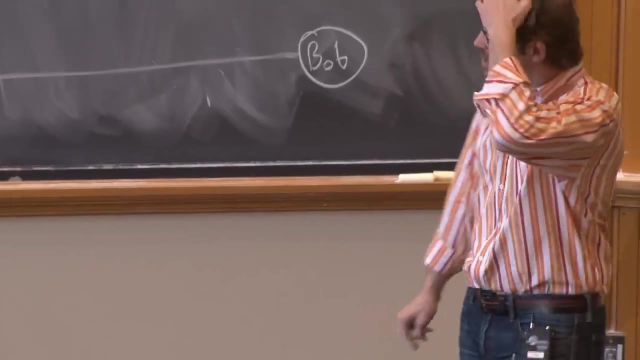 and over again. The list is just some random list of ups and downs, ups and downs, But they're exactly correlated amongst each other. So at this point EPR are really upset Because they say: look, there are two possibilities. Either there was an answer to the question all the way along of whether Alice's was up and Bob's was up, or Alice's was down and Bob's was down, Or there's some deep nonlocality in the universe such that a distant measurement causally disconnected. 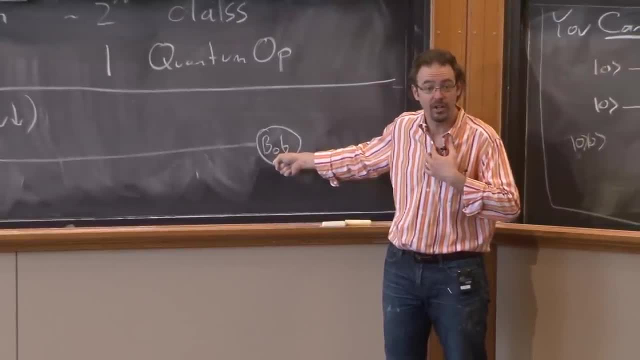 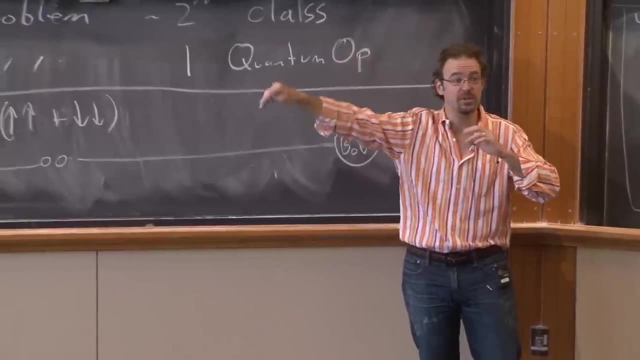 can have an influence on Bob's state such that they're correlated. This may seem random, but it's certainly not random, Because it's correlated with Alice, even though Alice is wildly disconnected, distant, distant, distant observer. Nothing could have traveled across that distance. 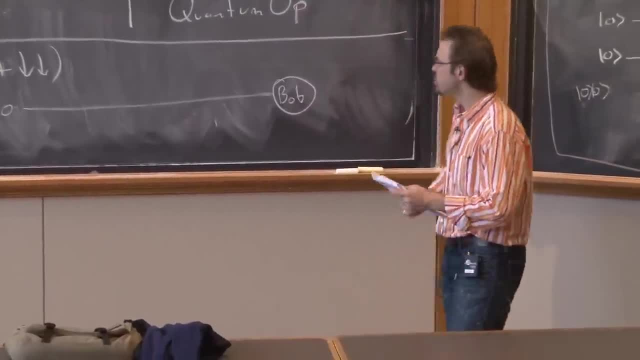 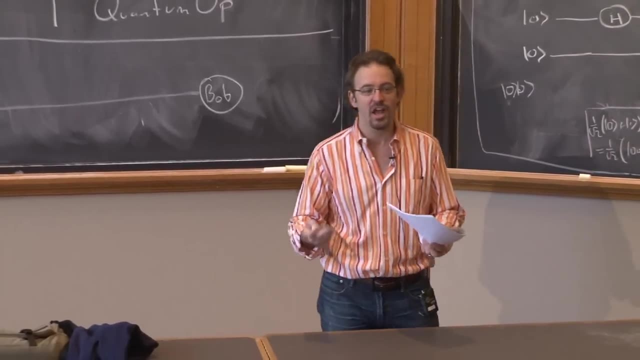 in the time it took to do the measurement. So there are sort of three responses you could take to this. The first response is: look, there isn't a problem here, It's just saying that quantum mechanics is insufficient. Really, secretly, there's a hidden variable, a variable you. 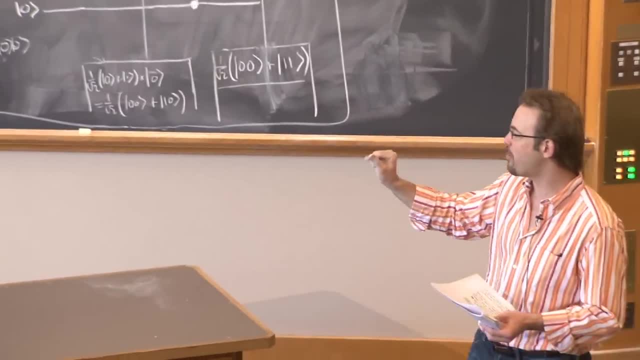 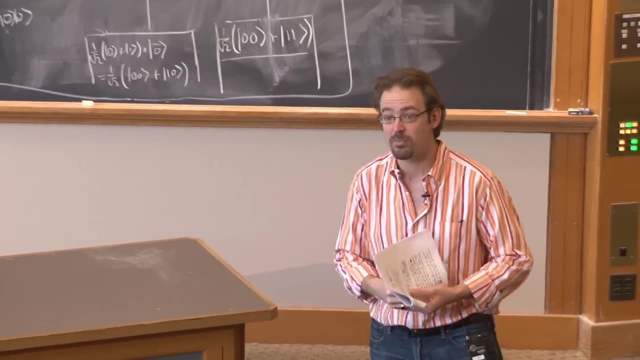 haven't observed yet. It's the property of an electron that determines whether it's going to be up or down early on, And the fact that it looks probabilistic just means that there's some classical dynamics for this hidden variable that, effectively, is probabilistic. 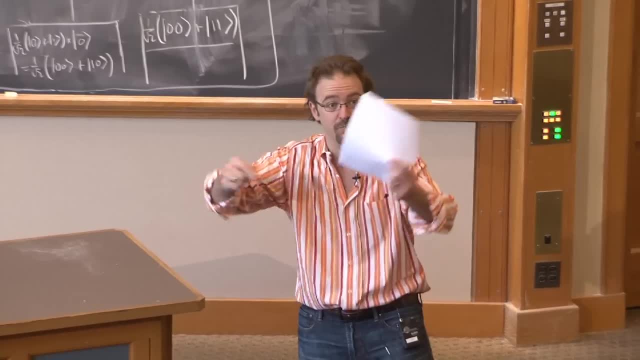 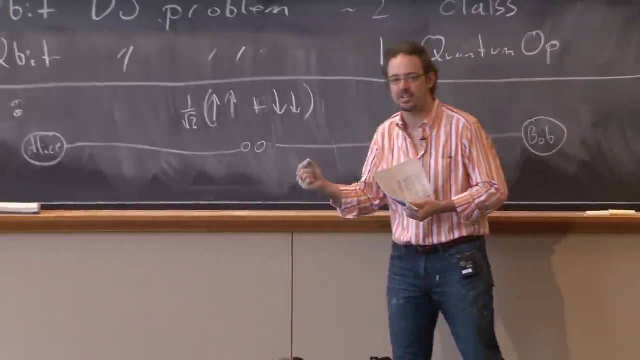 like a particle moving in a fluid, like dust, pollen, grains in a fluid. It just moves around randomly, But it just looks random. It's not actually random And that's because there's an underlying classical mechanism controlling the probability distribution. The second version is a quantum mechanical version. 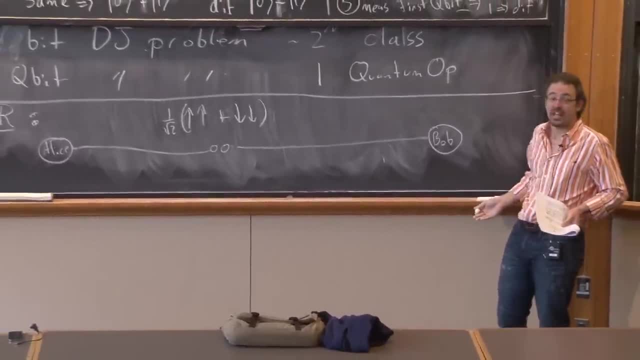 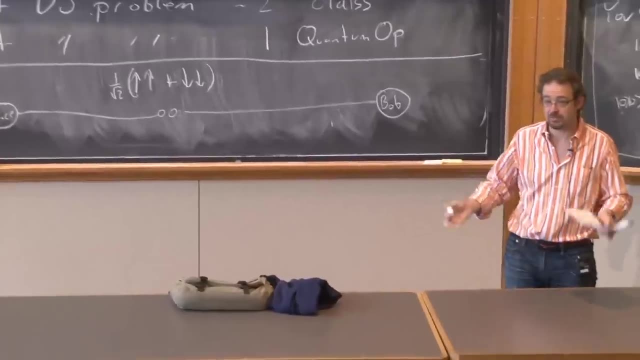 The second interpretation is to say: look, this may look upsetting, And I grant you that it looks upsetting, But I'm a quantum mechanic And quantum mechanics works like a champ And I'm not about to throw it out and say that there's some secret, hidden variables. 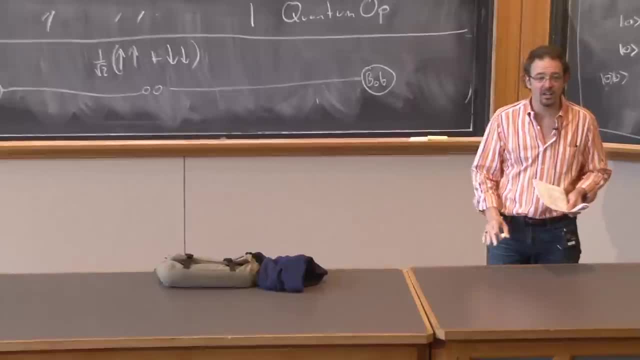 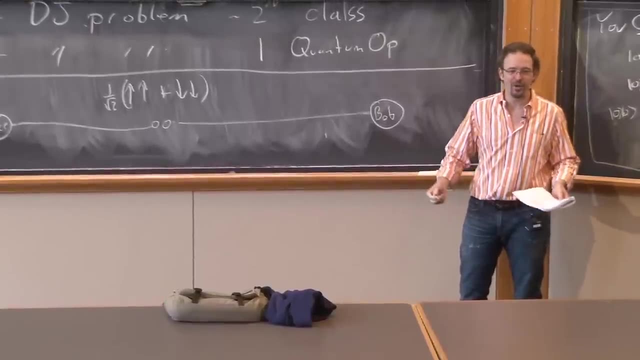 It just works. So just give up on your naive notions of locality. Let it go And just do the quantum mechanical calculation. Practicing physicists look at this and just yawn. If you're a practicing physicist, just forget it. Obviously it works. 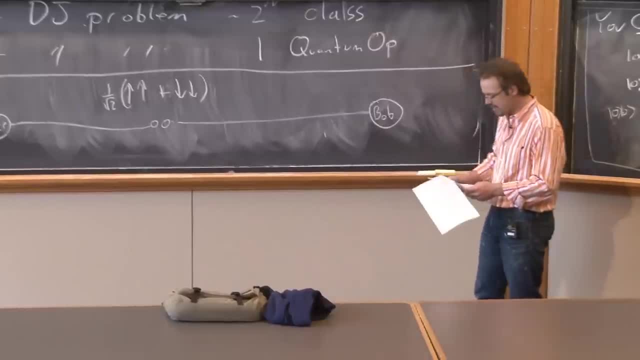 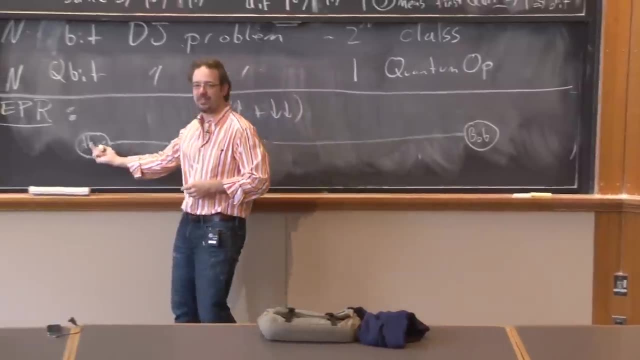 So there's no more conversation to be had. So meanwhile there's a second version of this which is slightly more disturbing. Suppose Alice measures up, And this is all in the z-direction. Suppose Alice measures up in the z-direction, She thus knows that Bob's particle is up. 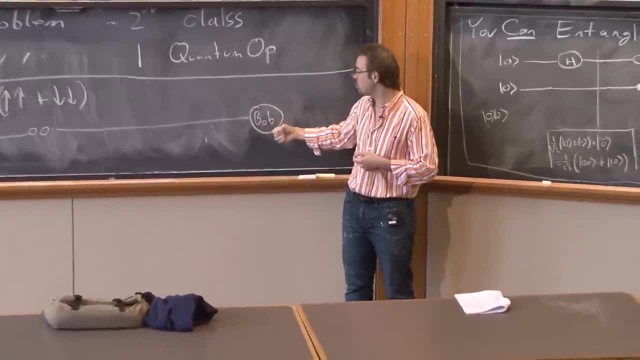 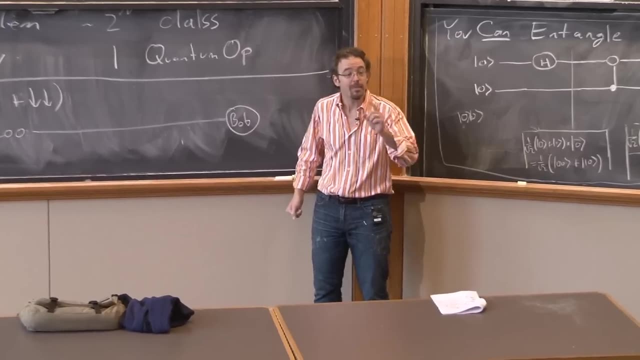 in the z-direction. But simultaneously Bob could measure spin in the x-direction and determine that his spin is up in the x-direction as well. At that point EPR say: look, we've measured empirically, We've measured that the particle is both up in the z-direction. 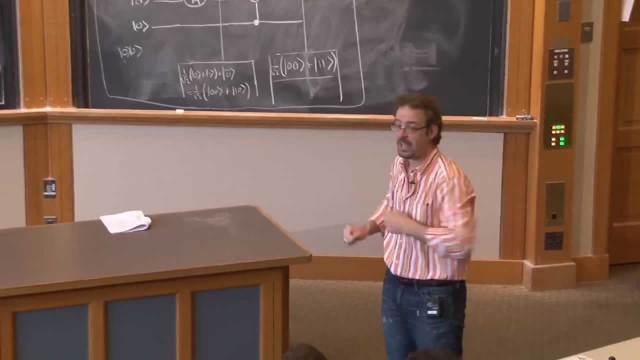 and up in the x-direction. It's just that we did that measurement using entanglement, But at the beginning of the day, at the very beginning- oh shoot, I erased it. Dang, that's not what I wanted. 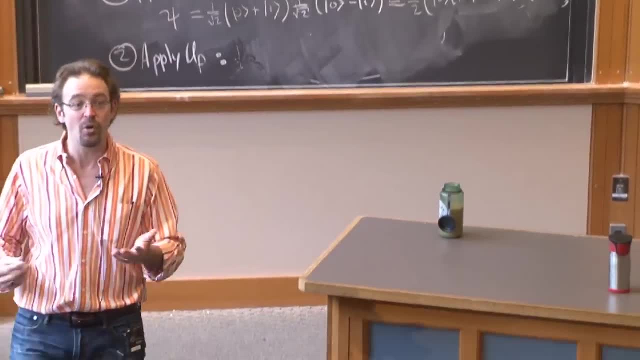 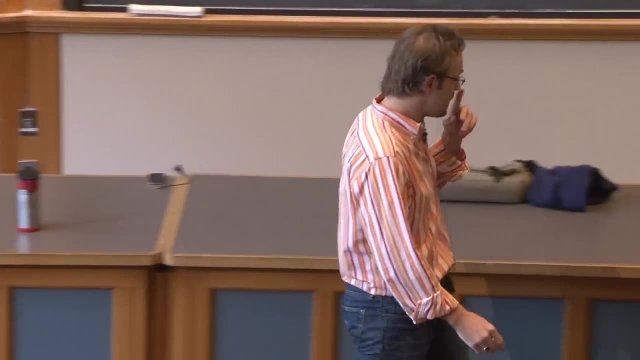 So at the very beginning of the day we had that Sx and Sz don't commute. So you can't have a state with definite Sx and definite Sz. You cannot possibly. It doesn't mean anything to say so Einstein wants to say that this is because quantum mechanics is. 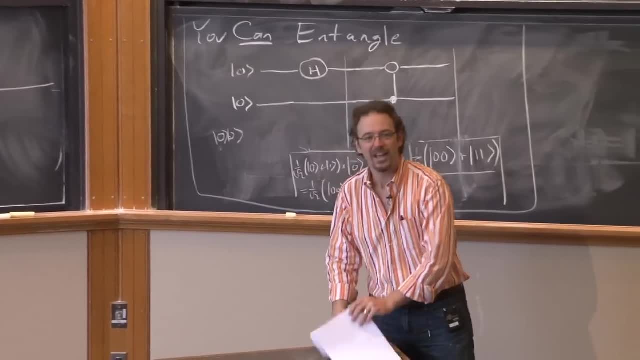 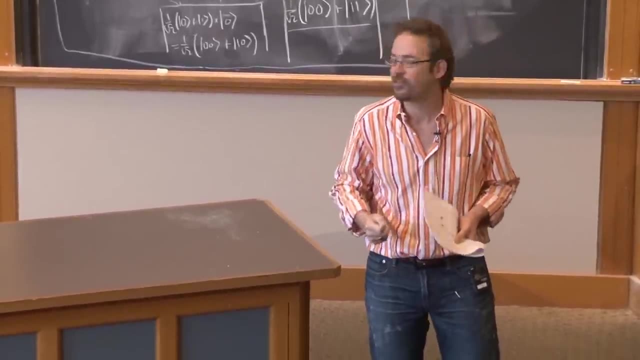 great but incomplete. The rest of us want to say that no, it's not, But that sounds like a philosophical question And that's the way it was treated for a very long time, until you come along to Bell, And Bell made a beautiful observation. 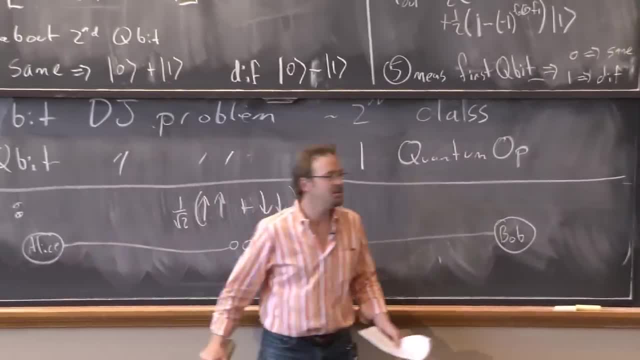 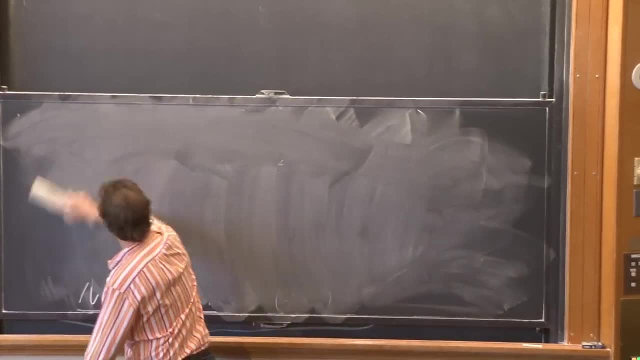 Bell said: look, telling me that there's an underlying classical description, telling me that there's an underlying probabilistic classical description tells me enough to make this an empirical question, Because it's saying that the statistics, the random statistics for Bob and Alice, are correlated. 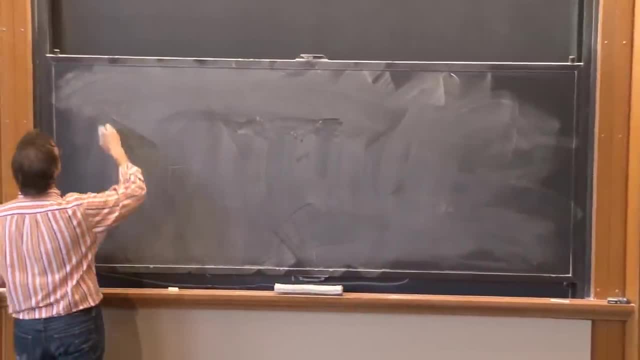 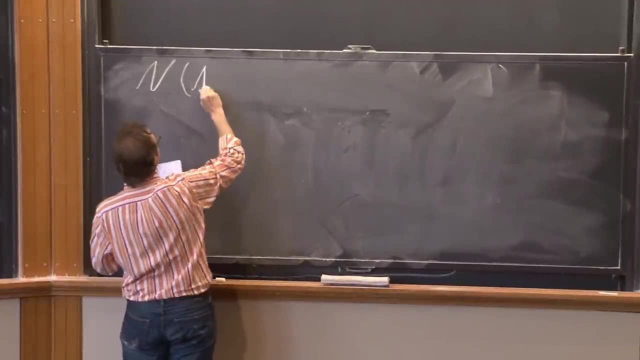 by a classical dynamics rather than independent. So here's Bell's version. So remember, at the very beginning we talked about Bell's experiment. We said: consider three binary properties: A, B and C, The number of that Of some set that are A and not B, plus the number that are B. 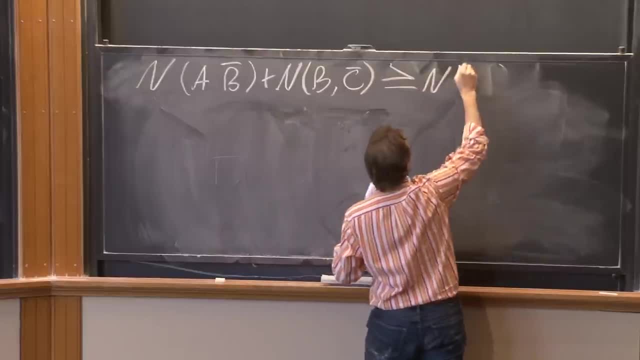 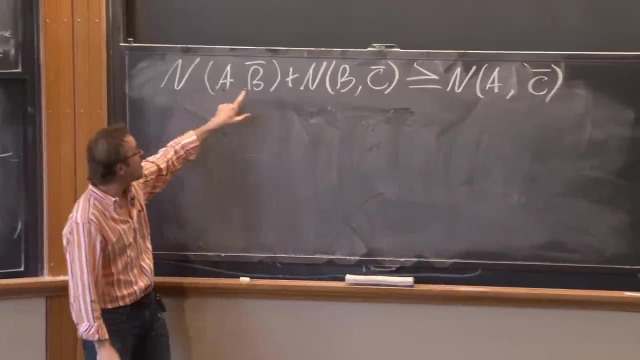 but not C, is always greater than or equal to the number. that are A but not C, And the way we proved this was just by noting that if these are classical deterministic binary properties, then A not B means A not B and C, or A not B and not C. 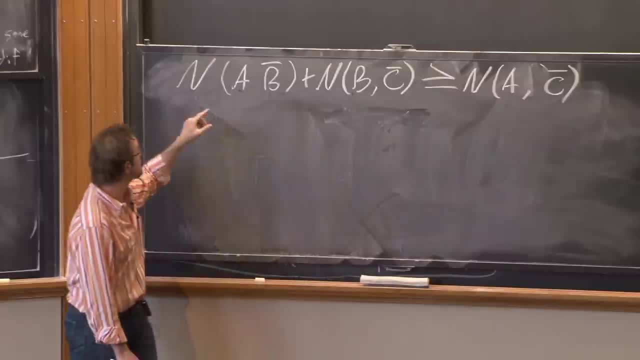 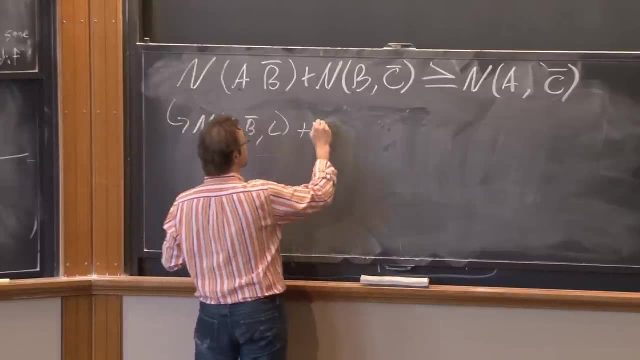 And ditto for each of these other guys, And we ended up with an expression which was number that are A. So using that logic leads you to number that are A, not B and C, plus the number that are not A, B and not C is greater than or equal to 0. 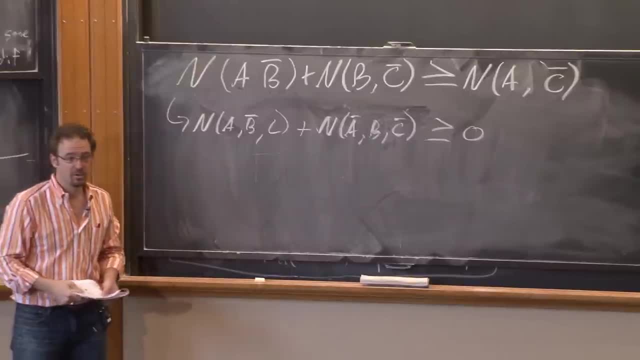 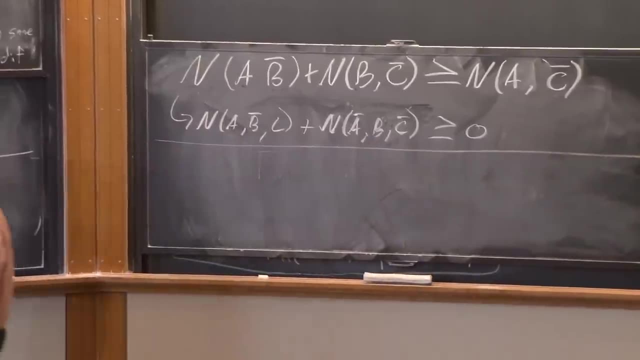 And that's clearly true. You can't have a number of elements be negative, So this is trivially true mechanically. But now here's the experiment I want to do. I want to do actually the EPR experiment, And here's the experiment I want to run. 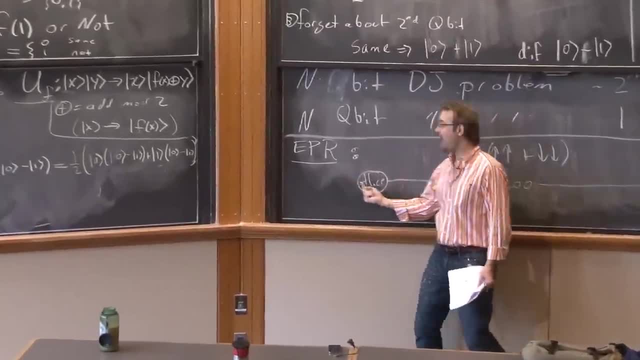 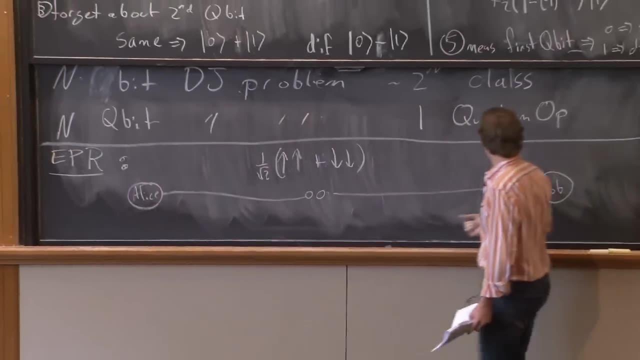 Alice is going to measure up or down at 0. And Bob is going to measure up or down at theta. Alice is then going to measure up and down at theta And Bob is going to measure up and down at 2 theta. And the third experiment is going. 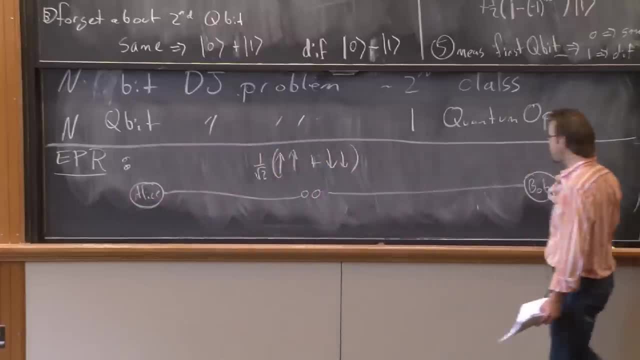 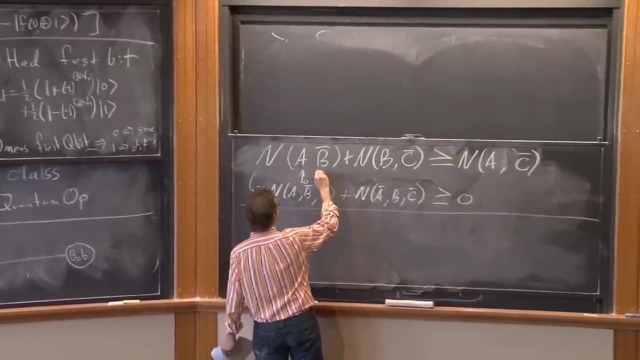 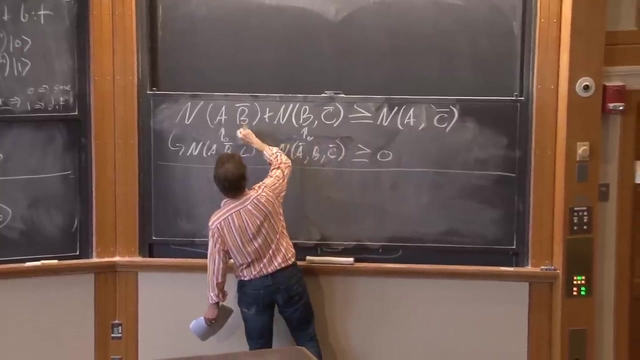 to be. Alice is going to measure up and down at 0. And Bob is going to measure up and down at 2 theta. So A is up or down at 0.. B is up at theta. B is up at theta. Sorry, this is going to be down at theta. 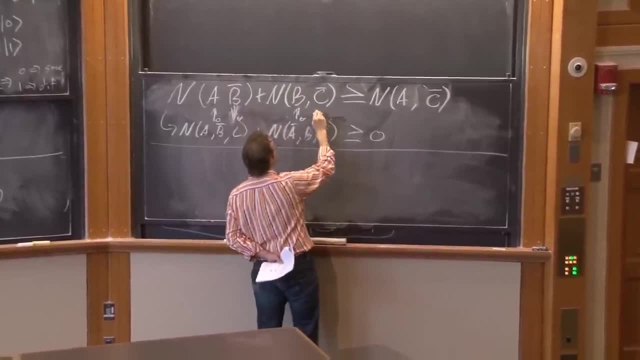 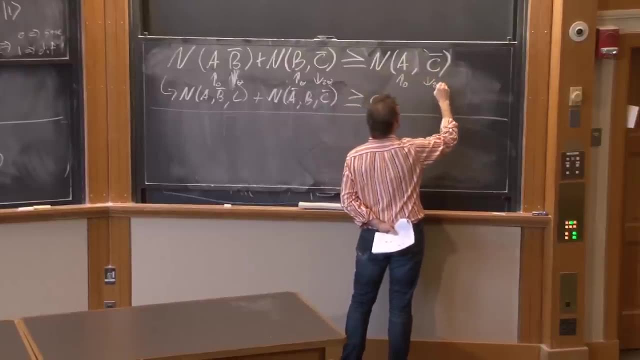 Not B is down at theta, B is going to be up at theta And C is going to be down at 2 theta And A again up at 0. And not C is down at 2 theta. OK, So we can rephrase this as the probability. 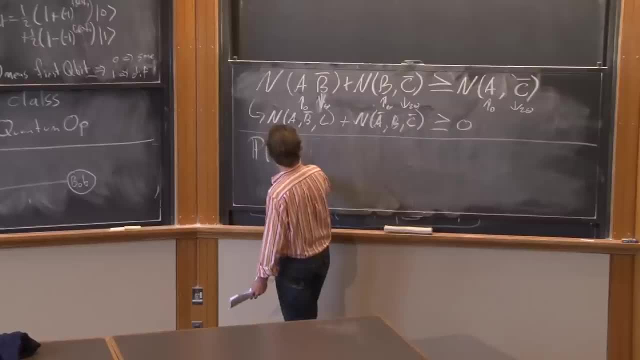 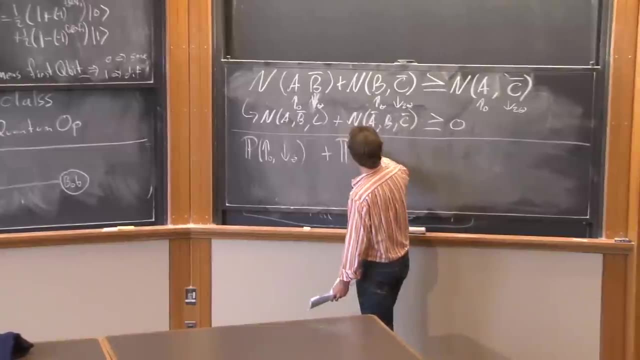 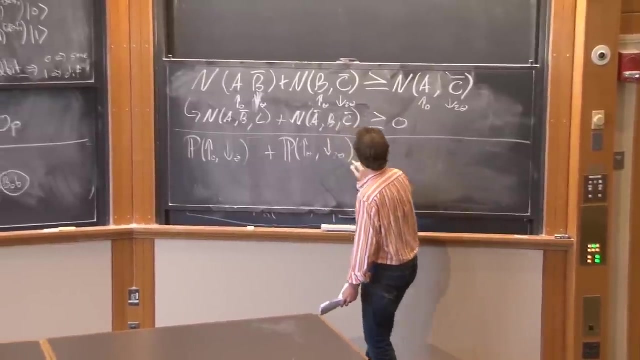 that, given that we are up at 0,, what is the probability that we are subsequently down at theta, Plus the probability that we are up at theta? What is the probability that we are up at theta and subsequently down at 2 theta, And then the probability that we are up at 0 and down at 2 theta? 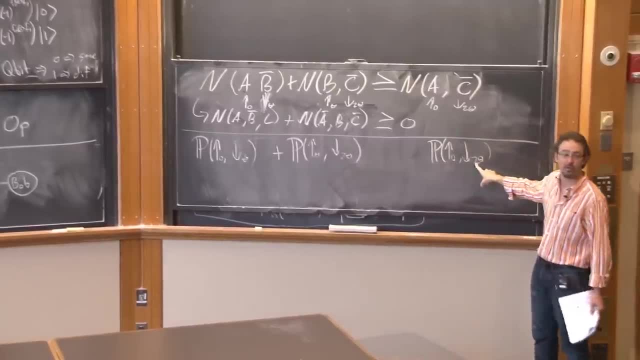 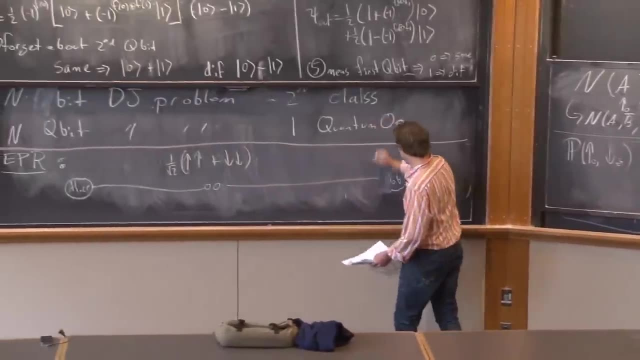 using an EPR measurement, Where one is performed by Alice and the other is performed by Bob, Exactly as EPR wanted, And we computed this last time. In fact, I just erased, because I'm excited about this, I guess I just erased- the wave function that we needed. 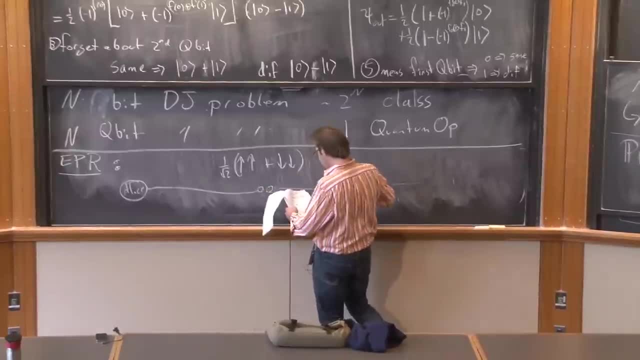 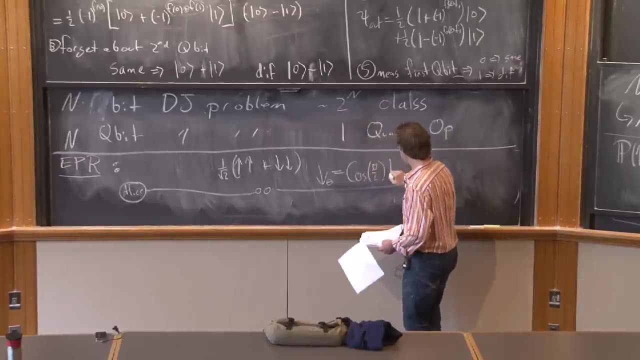 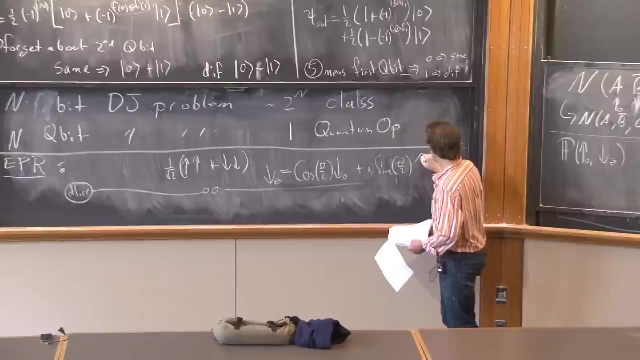 the state we needed. And the state that we needed was that if we are down at the angle theta, then this is equal to cosine of theta upon 2, down at 0, plus i sine theta upon 2.. OK, Up at 0.. 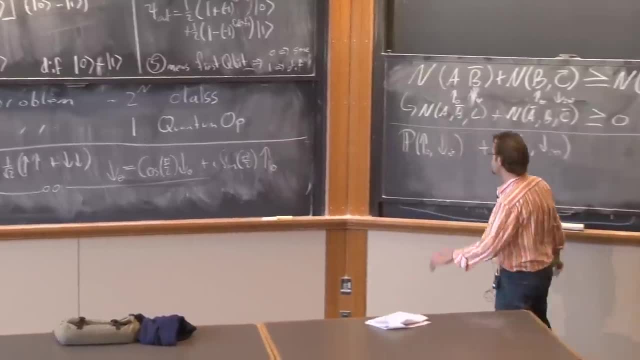 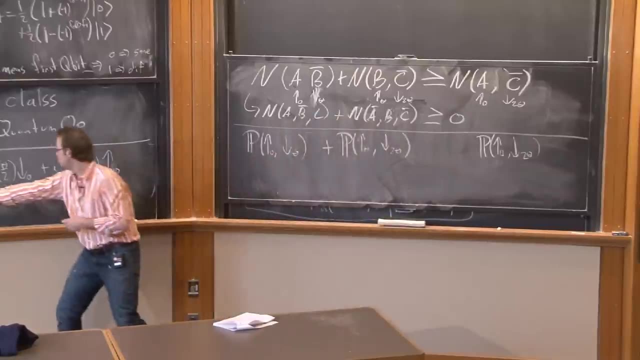 And this is enough to answer our question. This is the quantum mechanical prediction. What's the probability that, given that we're down at the angle theta, we're up at the angle 0?? Well, if we're down at theta, the probability? 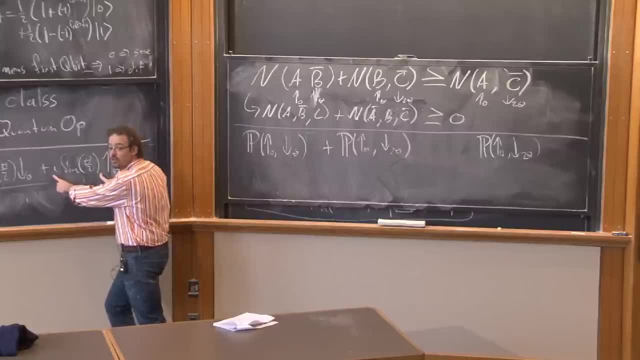 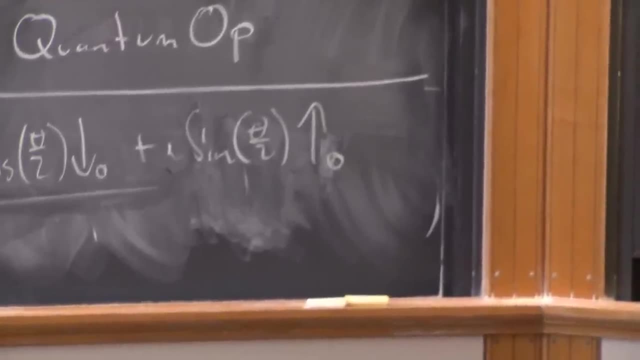 that we're up at 0, the coefficient is i, sine theta upon 2.. And the probability is the norm squared of that expansion coefficient. So the probability is sine squared of theta upon 2.. Similarly, the probability that we're up at theta 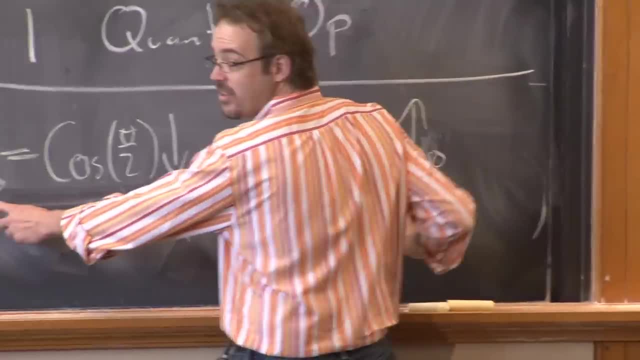 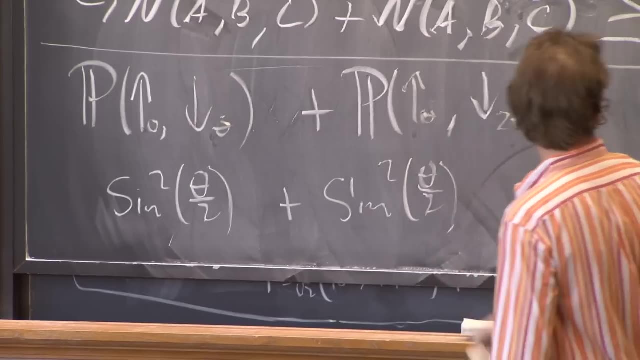 and down at 2 theta. well, by a rotation by theta, this gives me exactly the same thing. So it's again going to be sine squared theta upon 2.. The probability that we're up at 0 and down at 2 theta. 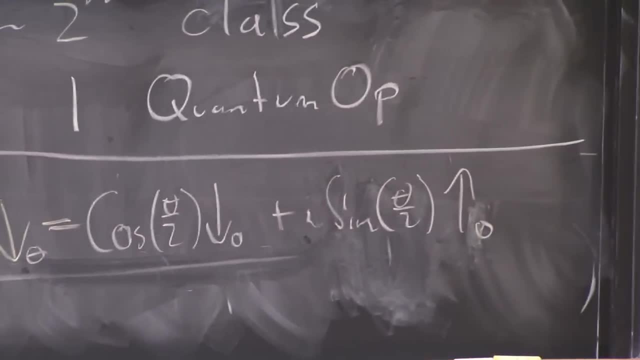 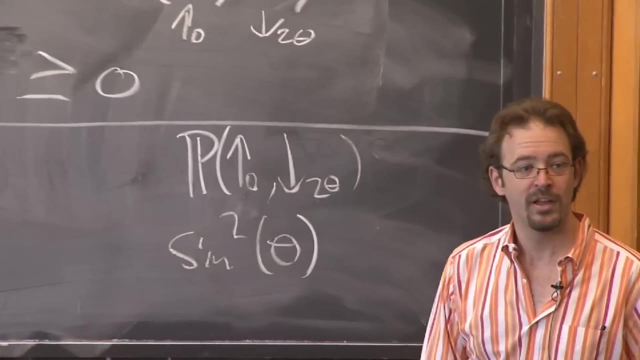 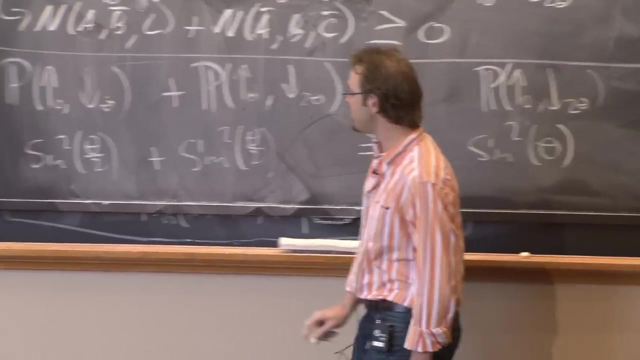 well, just stick in a factor of 2 for theta everywhere, And that gives me sine squared of theta. Now I ask you, is the left-hand side always greater than or equal to the right-hand side? And this is easy to check. 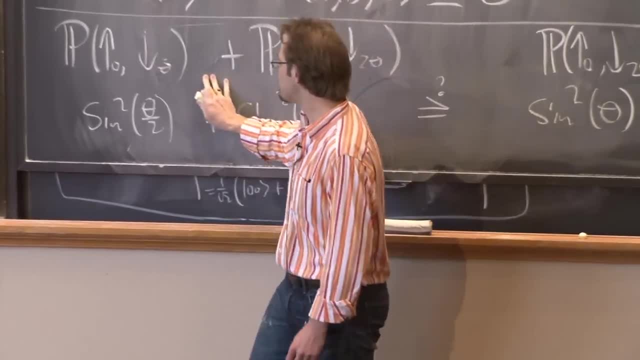 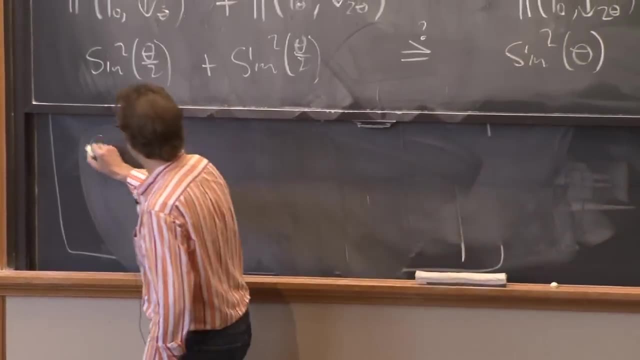 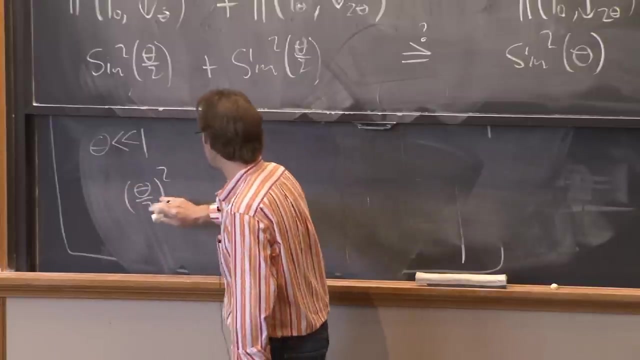 Let's do this for a very small reason, For a very small theta: sine squared theta. so for small theta, much less than 1, sine theta squared is theta upon 2, the angle squared which is equal to theta squared upon 4.. 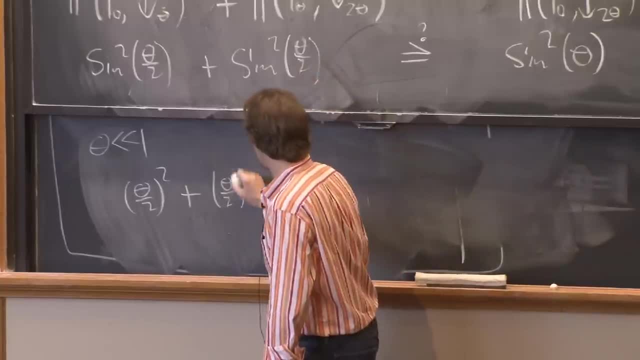 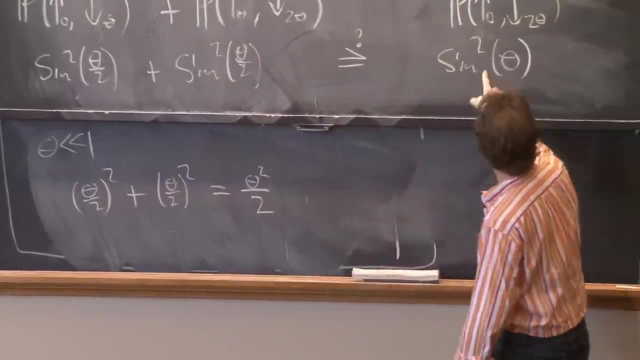 And the next one is the same thing, plus theta upon 2 squared, which is equal to theta squared upon 4, theta squared upon 4, so theta squared upon 2.. And the right-hand side, It's sine squared theta, which is theta squared. 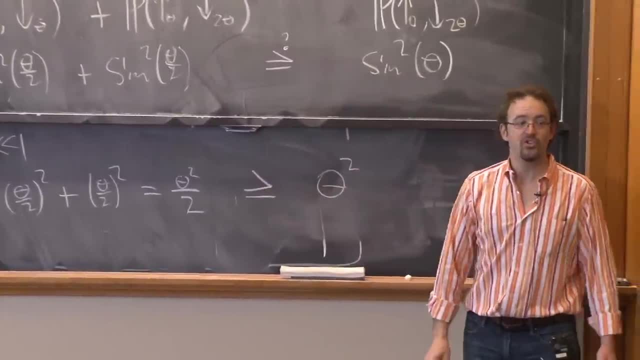 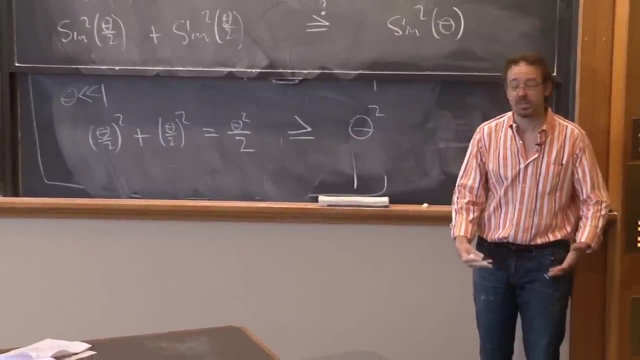 And is theta, squared upon 2, greater than or equal to theta? Certainly not, So. quantum mechanics predicts that if we do the EPR experiment using these observables repeatedly and build up statistics, what we will find is an explicit violation of the Bell inequality. 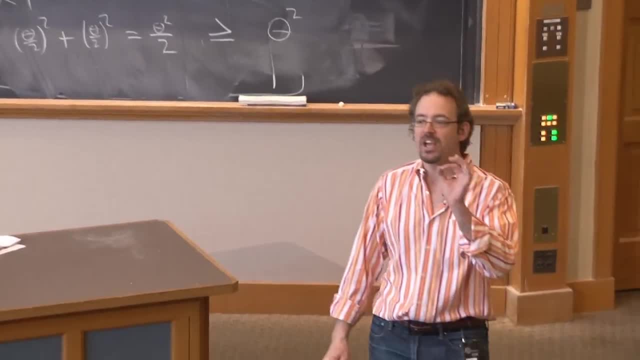 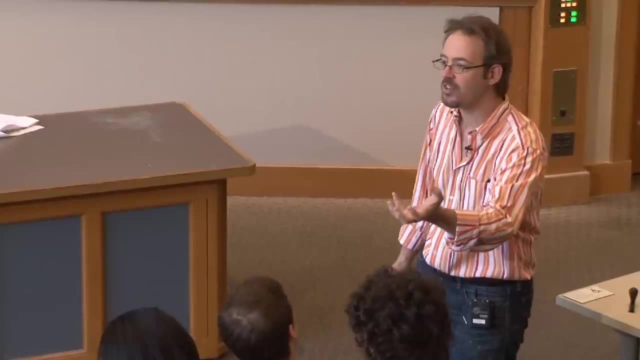 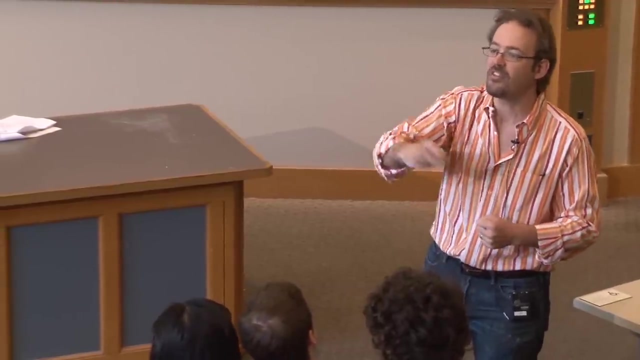 And what that would represent if it were actually true, if we actually observed. it would be a conclusive empirical proof that there are no classical, definite configurations underlying the probability of quantum mechanical events. It would say that it's impossible to build a classical theory with hidden variables that are randomly.